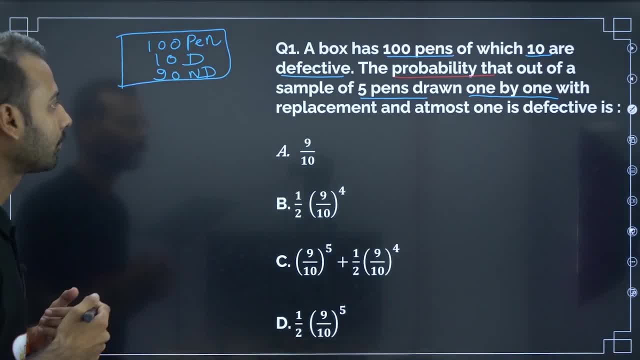 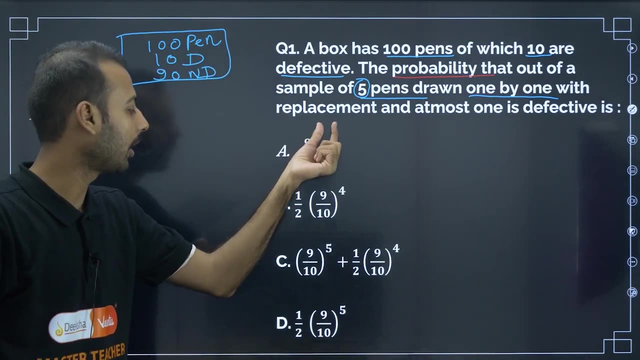 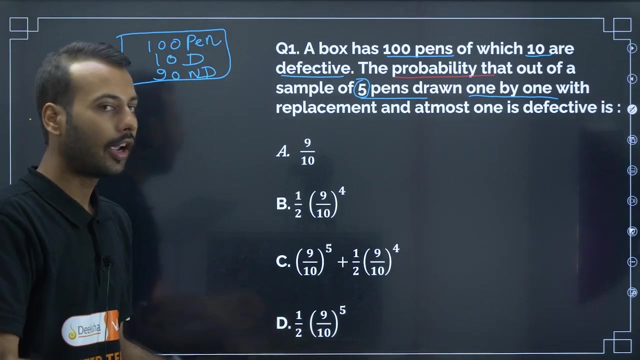 The probability that the probability that out of sample of 5 pens- Suppose, if I am considering 5 pens drawn one by one, Sample of 5 pens means we are drawing 5 pens One by one. we are drawing with replacement. With replacement means one pen we have drawn and then we have kept back Again one more pen we have drawn Again. we are keeping it back Means try to recall. try to recall the concept of non defective. 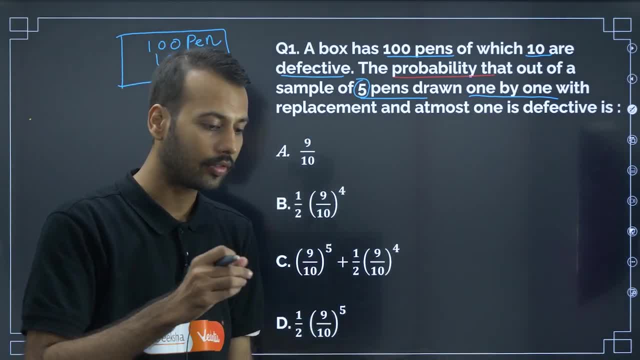 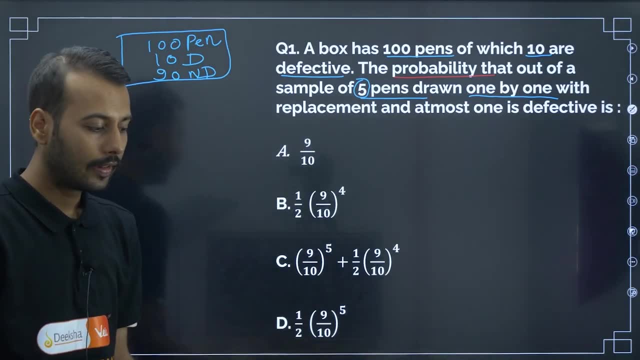 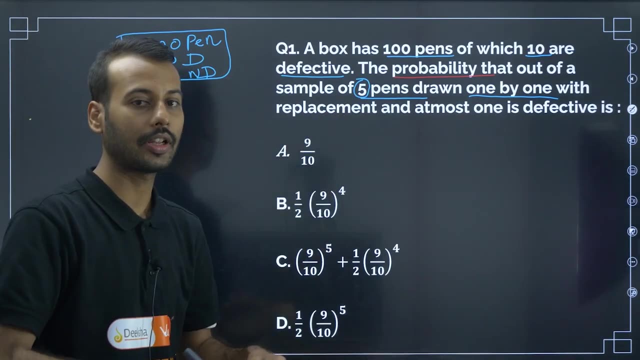 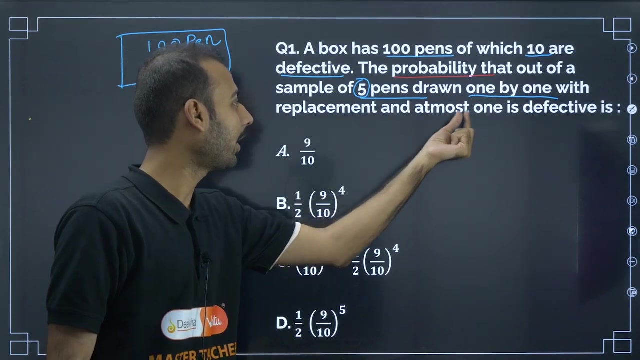 Related with 5 pens are drawn with replacement means one pen. we have drawn Again. we are keeping back. Again we are drawing one pen. Now we are doing this 5 times. 5 times means 5 times means one concept. Bernoulli trials concept should come to your mind at this point because repetition of experiment we do in Bernoulli trials. So drawn one by one, with replacement, With replacement, And at most one defective is, At most one defective is So. 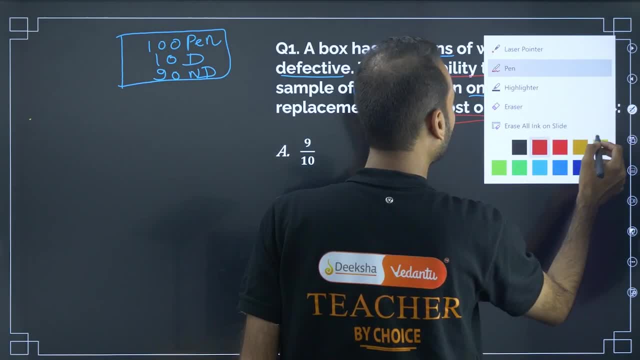 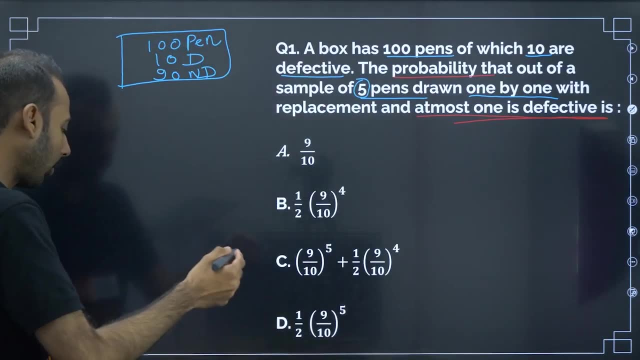 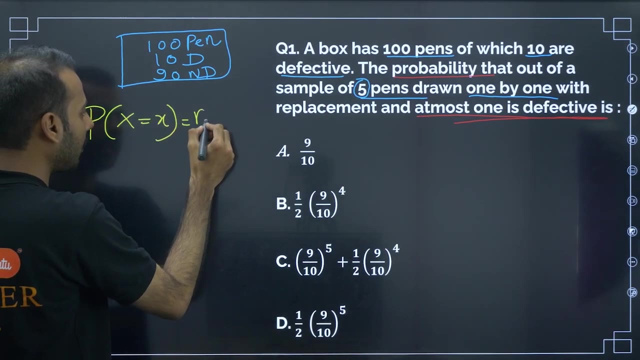 one defective is there, One defective is So for this, So for this. how to approach this problem? Now, Bernoulli trials. Now try to recall Bernoulli trials. There is one formula: X is equal to X, N, C, X, N, C, X, P. raise to X, Q. raise to N minus X, Q. raise to N minus X. Sample of N. Now, 5 pens means N is equal to: 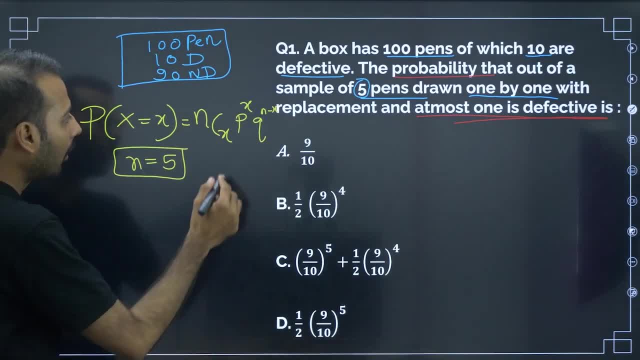 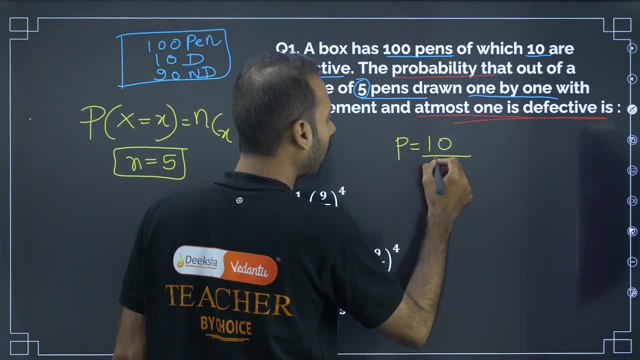 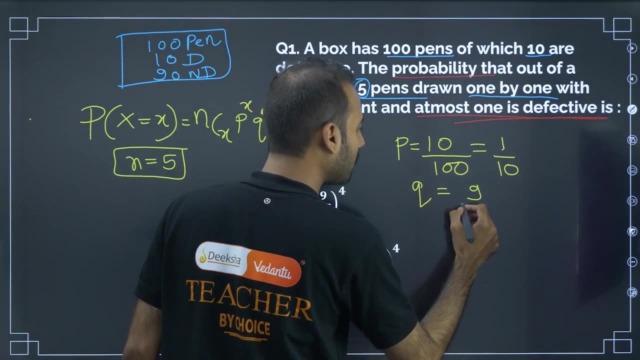 5 they have given us n is equal to 5. also defective they are talking about. defective means success. how many defective are there? there are totally 10 defective, and out of how much so? defective means 1 by 10. 1 by 10: if p is 1 by 10, q is equal to 9 by 10. automatically 9 by 10. 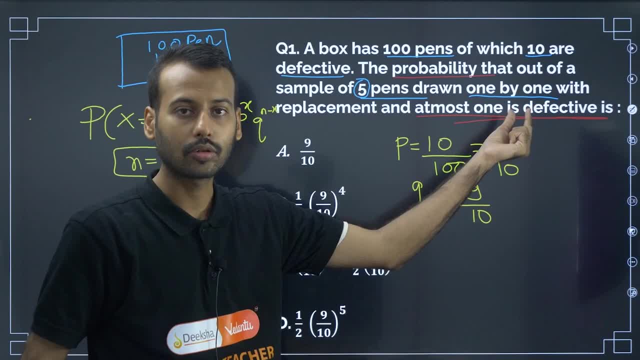 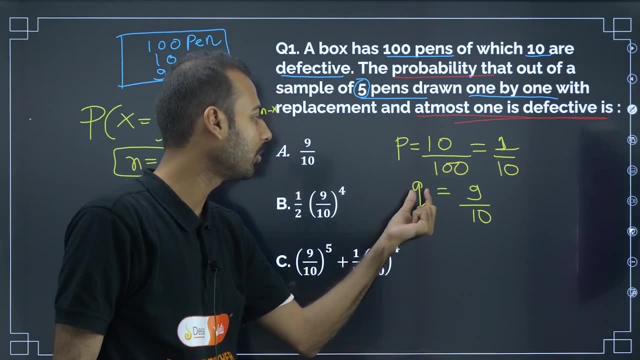 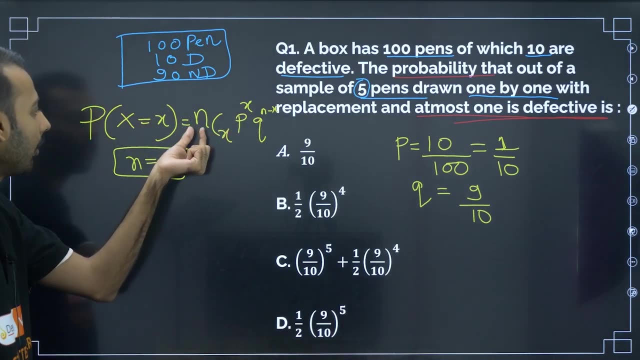 because we are considering defective as success. listen to my words. we are considering defective as success. success probability is denoted by p. p success is 1 by 10 means failure is 9 by 10. so p and q value we got now. x is equal to. we already know n value, we already know p value, q value we 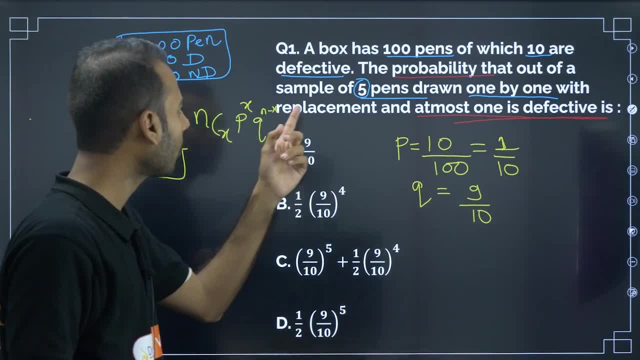 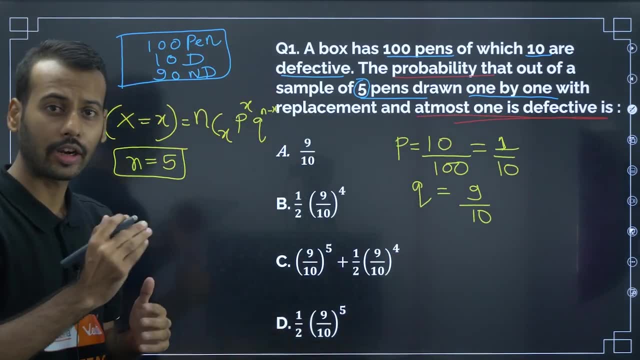 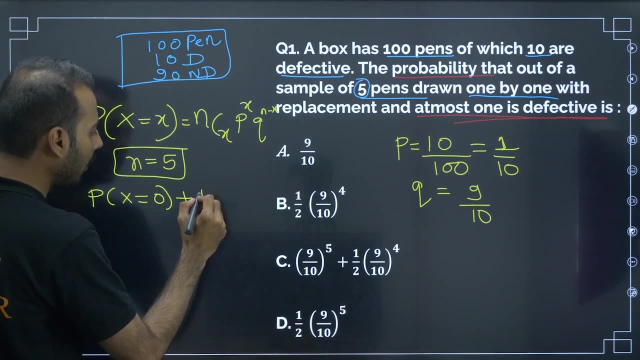 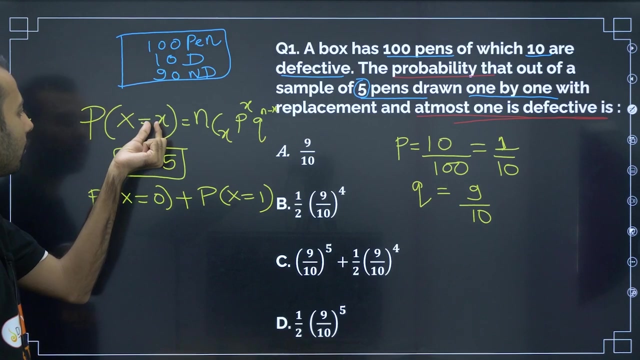 just have to know x value. what is this x? what is this x? now, if you go through the question, and at most one defective, at most means maximum one defective. so can it be zero defectives, at most one defective. so can it be zero defectives? yes, it can be 0 defectives, or it can be maximum 1 defectives. So at most, at most 1 defective. 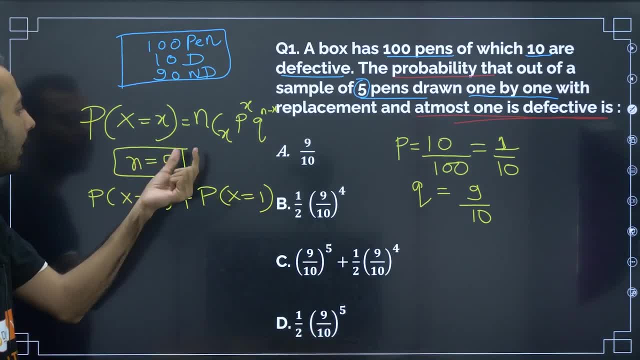 means 0 defective or 1 defective. these two we have to find. Now we just have to substitute this. So here we will get phi c 0, phi c 0. p. value is 1 by 10, 1 by 10, x is 0, q is 9 by. 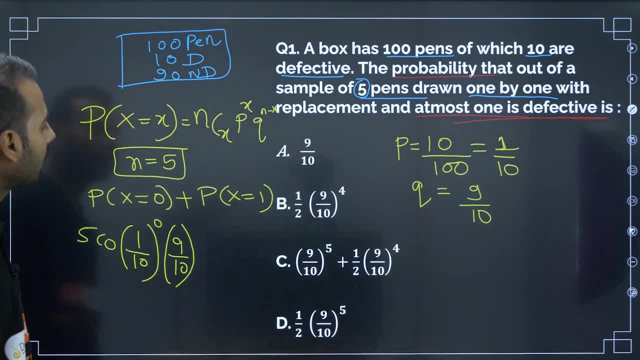 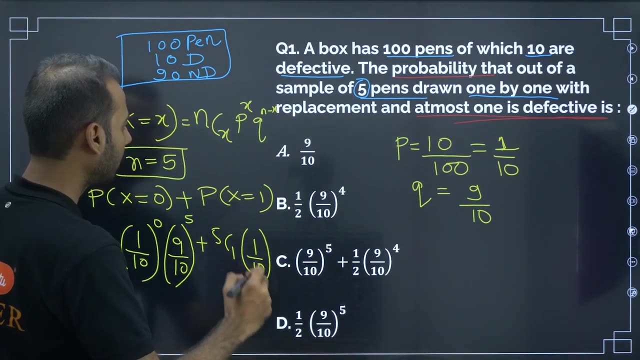 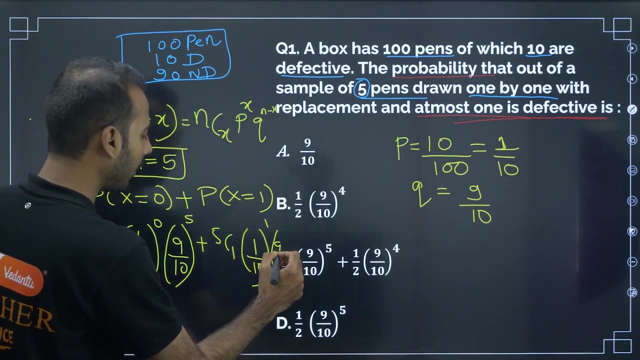 10. 9 by 10. n minus x. n minus x is n is phi minus x is. So this is phi plus p in place of n, c, x, phi c, 1, phi c: 1. p is 1 by 10, p is 1 by 10, x. x is x is 1. q is 9 by 10, 9 by 10. 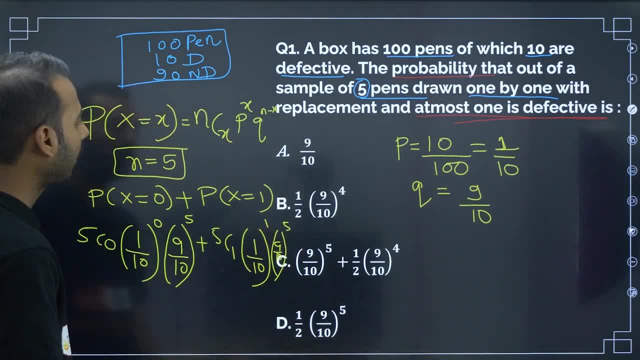 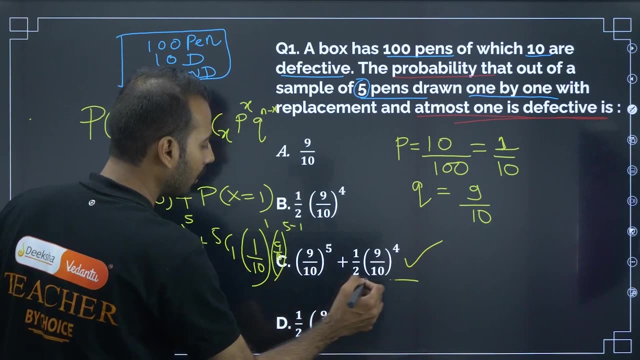 and n minus x is n minus x is n minus x is 1 by 10.. So here, what are we left with? 9 by 10 power phi, and if you see this, this is phi phi by 2, 9 by 10 power 4.. So answer for this is c. So Bernoulli trials, this question is based. 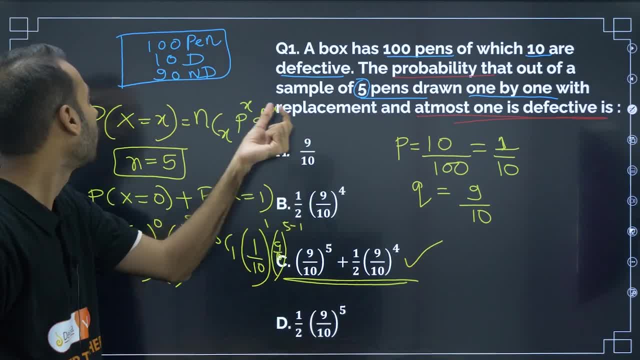 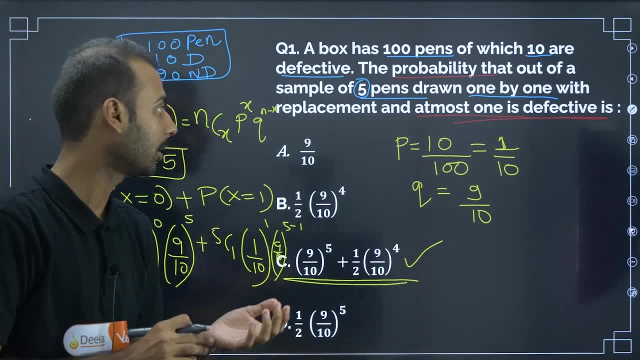 on Bernoulli trials. Bernoulli trials is important concept So you should be knowing Bernoulli trials concept. Please go through the synopsis in textbook Bernoulli trials, that concept and try to solve. try to memorize this concept and try to solve this concept. 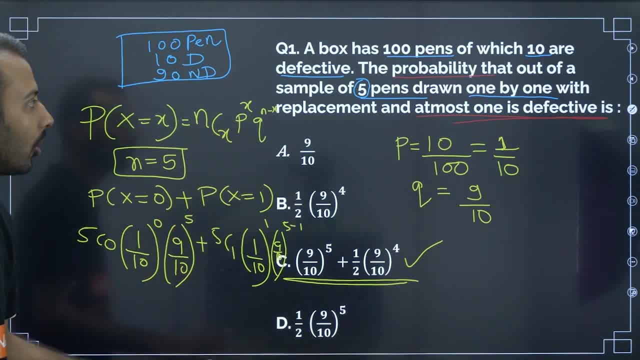 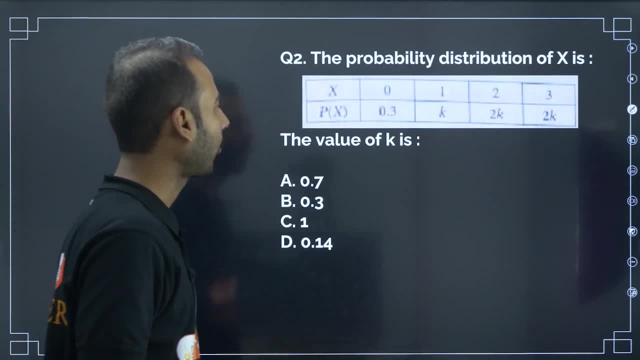 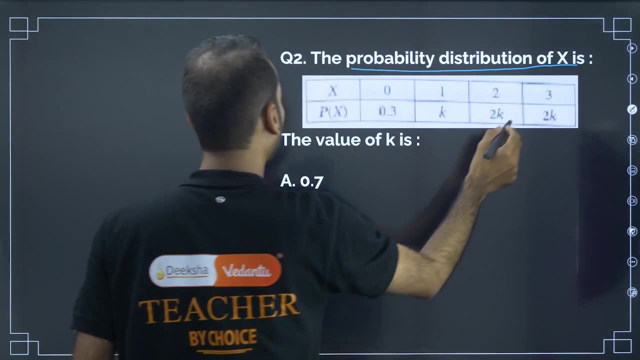 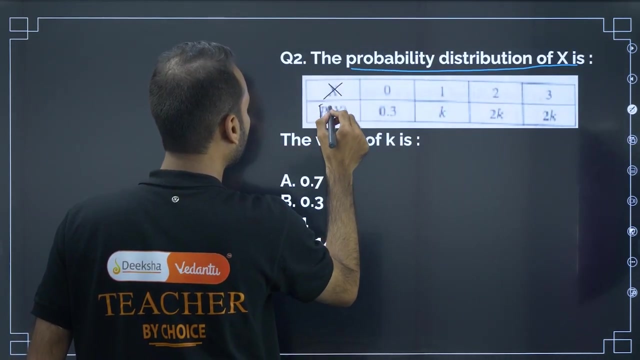 This formula and try to solve some problems. that is important. Bernoulli trials is important. Moving on to next question, The probability distribution of x is the probability distribution of x is So probability distribution. they have given like this: the probability distribution of x is here. let me write, since it is not clear: this is x, this is p of x: 0, 0.3, 1 is. 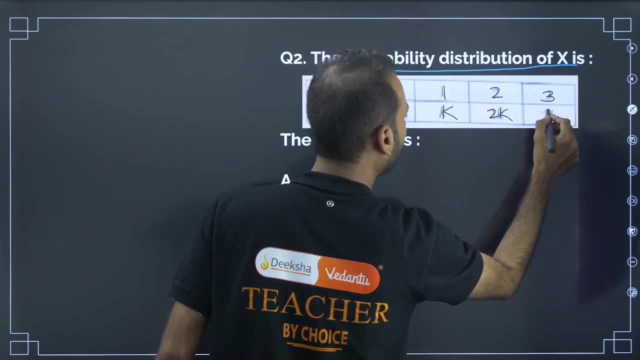 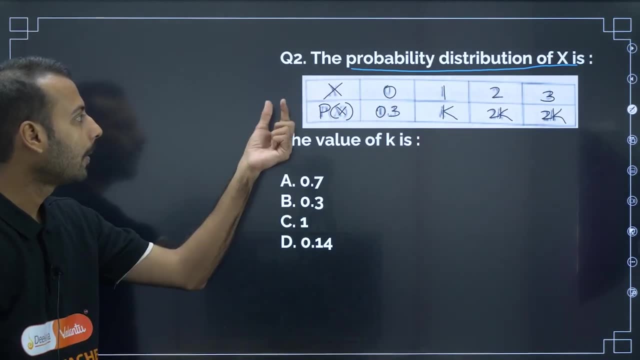 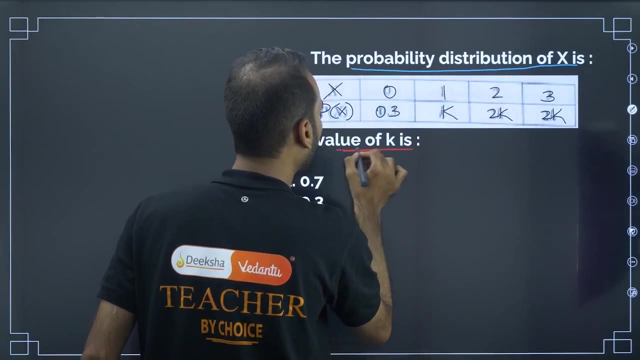 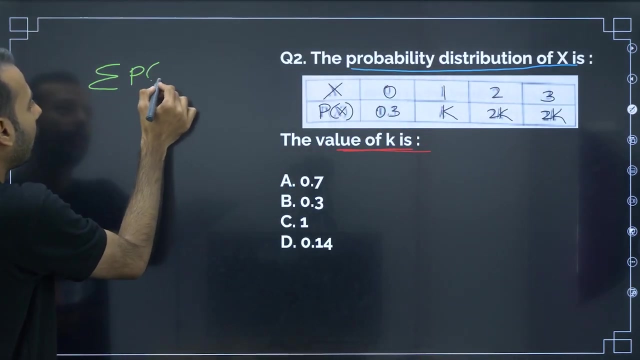 k 2, 2 k, 3 and 2 k. The probability distribution of x is. they have given like this, the value of k. is what are they asking? they are asking to find value of k. Now, one point you should be knowing, one point you should be knowing: summation of p of x is summation of p of x. 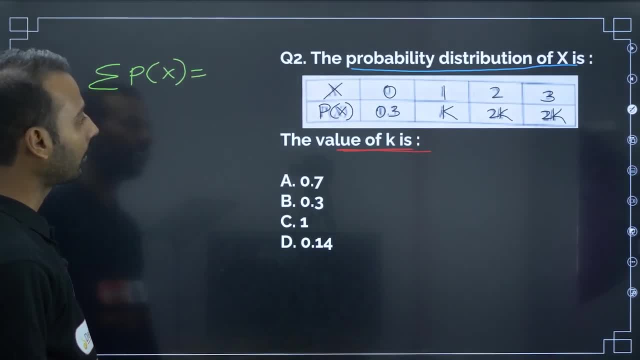 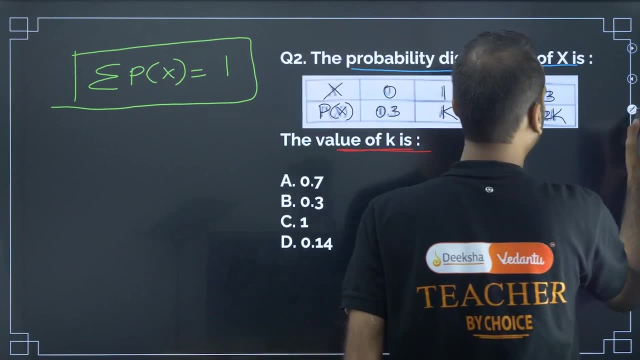 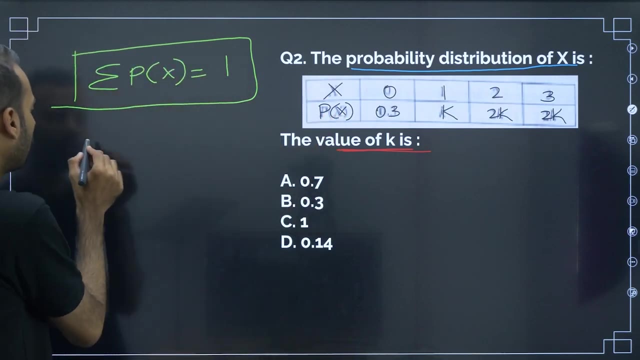 is This you should be knowing. you consider this as synopsis point. Synopsis point: knowing is your responsibility. Now, if you know synopsis point, then we just have to: summation: of p: x means 0.3. 0.3 plus 4 plus 5 k is equal to 1.. So 5 k, 5 k is equal to 0.7. that means k. 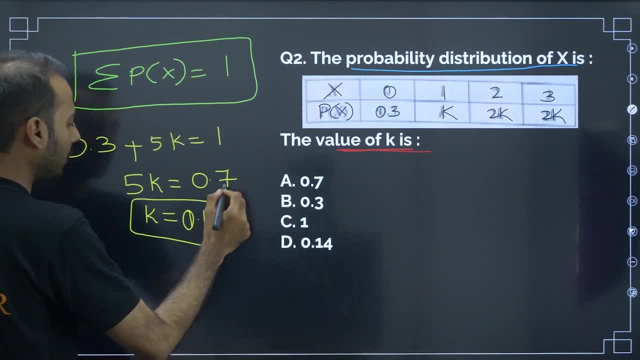 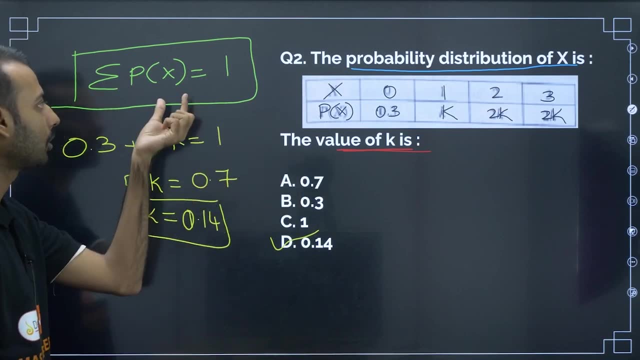 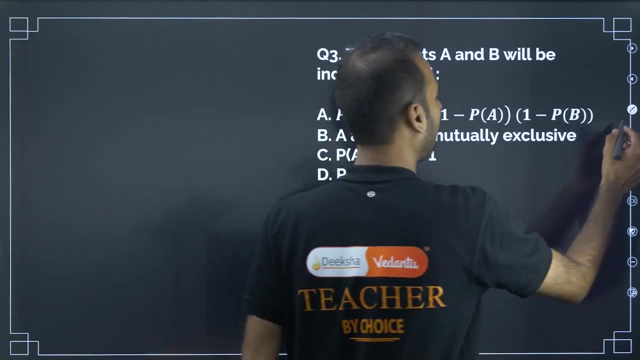 is equal to 0.14, k is equal to 0.14.. So answer for this is 0.14. only based on this. this was a easy question. only this point, if you know you are able to solve this. Moving on to next question, Two events, A and B, will be independent. if so, two events, what? 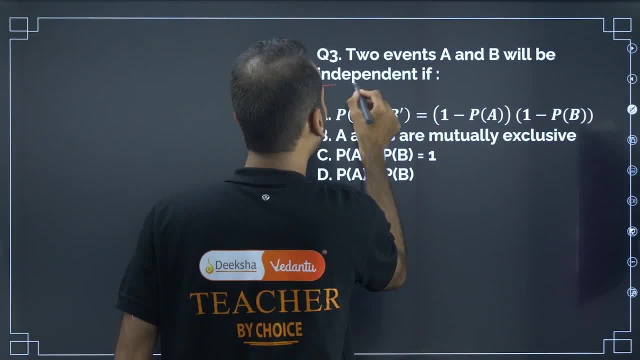 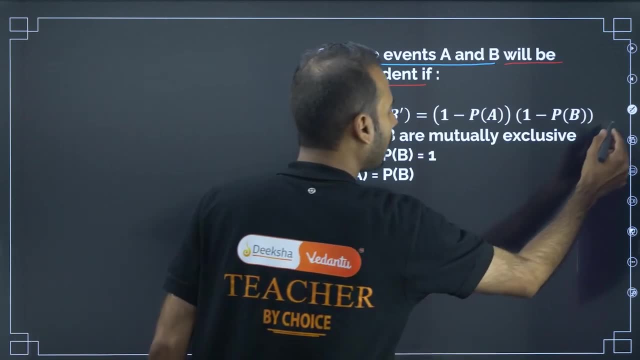 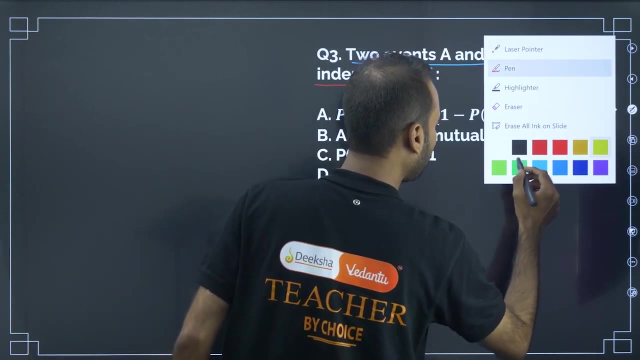 are they talking about two events. A and B will be independent, will be independent. Now, if you observe this, they are talking about two events: a and b will be independent. if a and b are independent, a and b are some synopsis point you should be knowing to solve this. 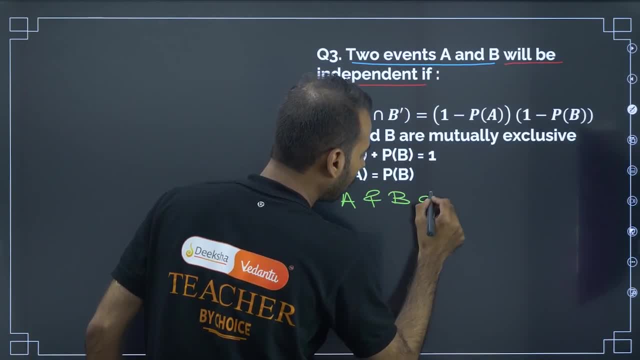 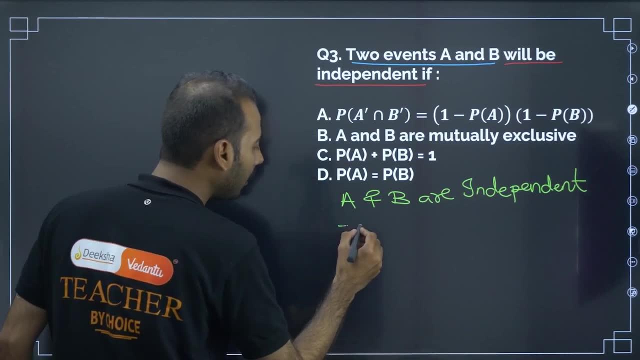 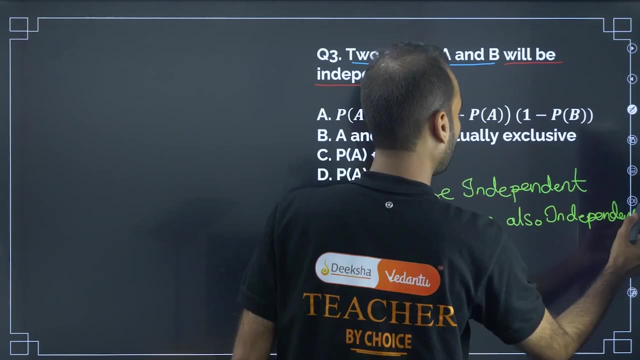 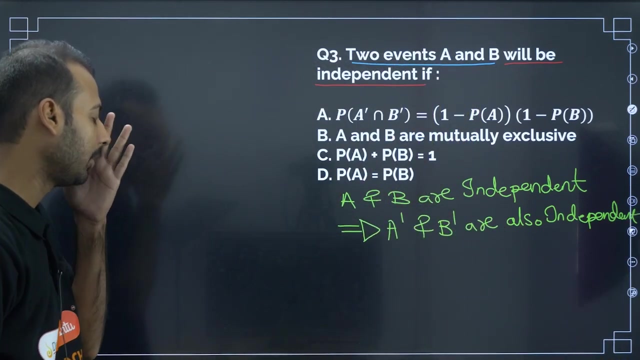 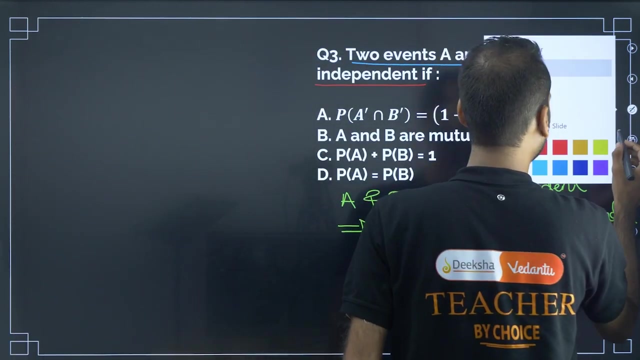 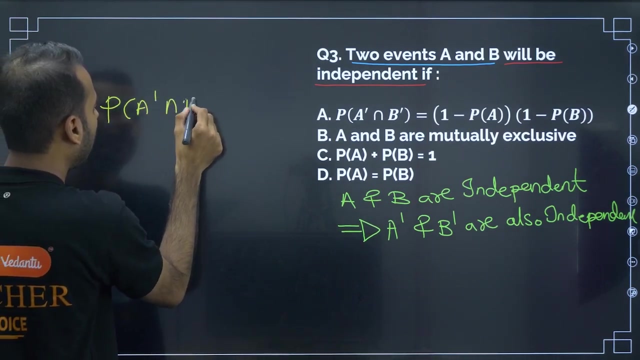 problem. a and b are independent implies a dash and b dash are also independent. so you take this as synopsis point in book. already it is there. if a and b are independent events, then this implies a dash and b dash are also independent. Now if I go through first option: a dash and b dash are independent. that means p of a dash. 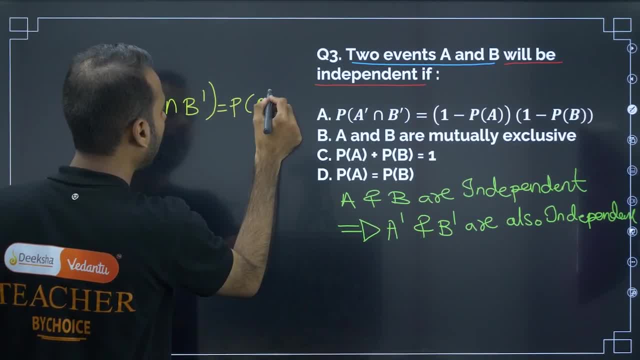 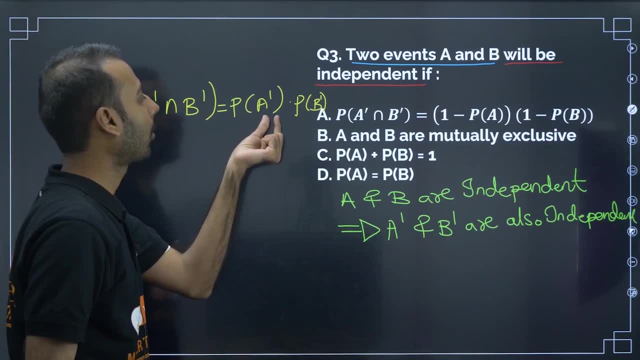 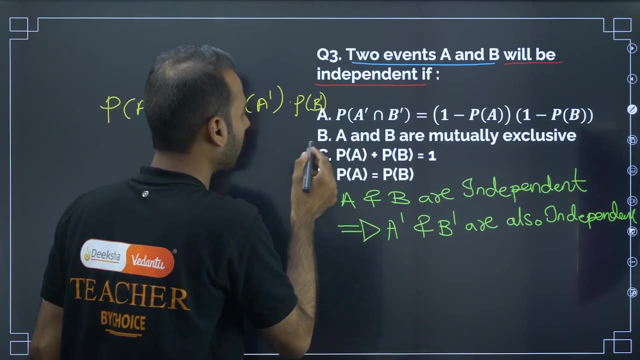 and b dash can be written as p of a dash, p of b dash. independent events means a dash and b dash. probability of a dash, probability of b dash. So independent events. this is the condition for even you can take this as synopsis point. so probability of a dash and b dash. 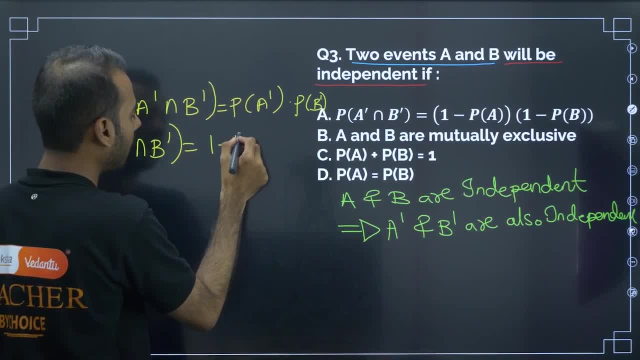 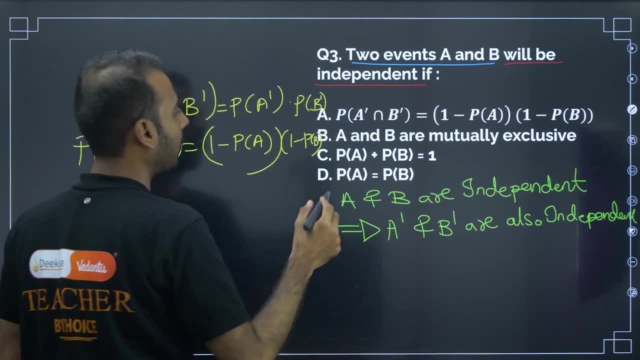 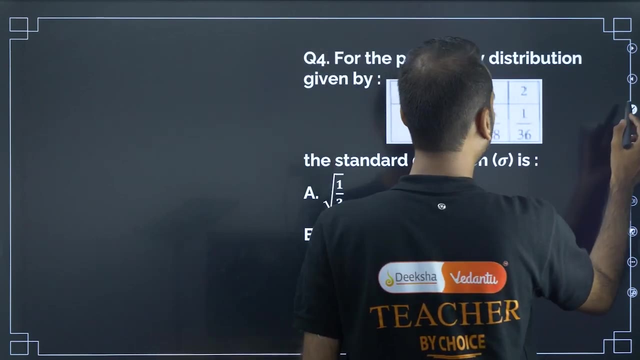 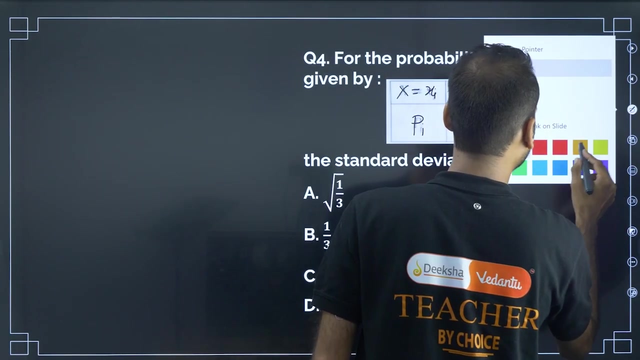 So a dash and b dash is equal to 1 minus p of a, 1 minus p of b. so all this is synopsis points only. So answer for this is a. Moving on to next question, the probability distribution. for the probability distribution, they have given some probability distribution. for the probability distribution, one probability: 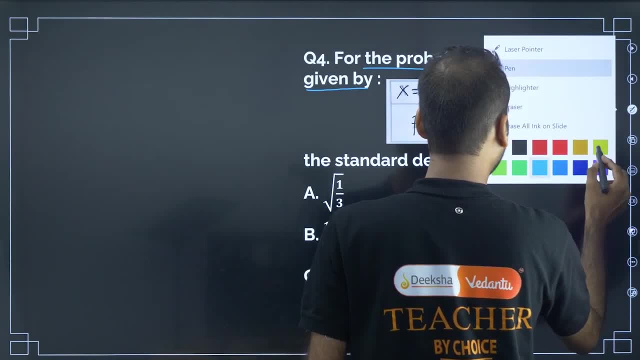 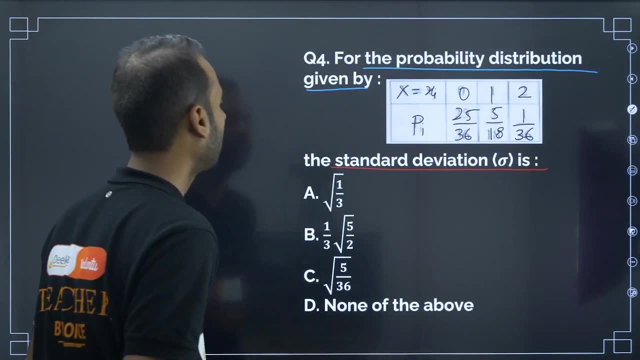 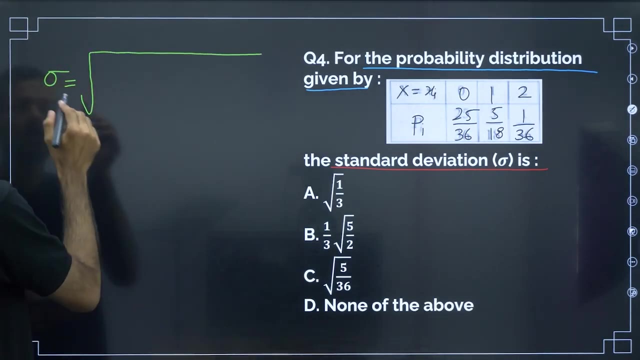 distribution they have. Yes, standard deviation is what is that Standard deviation is? standard deviation means for this now one synopsis point, or in fact you can say this as formula: sigma is equal to under root of standard deviation. sigma is equal to under root of summation xi square. 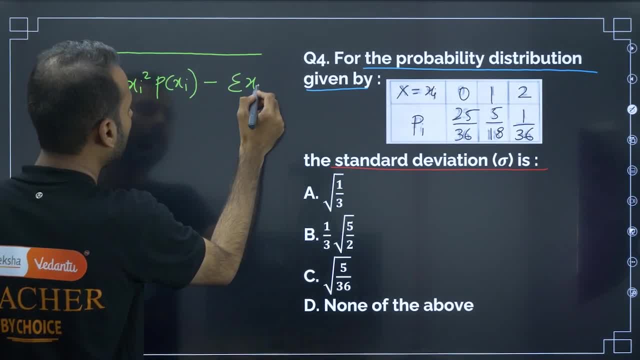 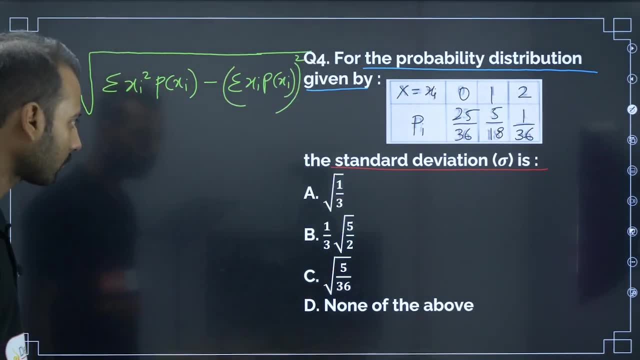 p of xi, p of xi minus summation, xi, p of xi, p of xi square summation. this standard deviation is this: So the formula to find standard deviation is given by this. Now standard deviation formula is this for this. now, if I use this formula to simplify, sigma is equal. 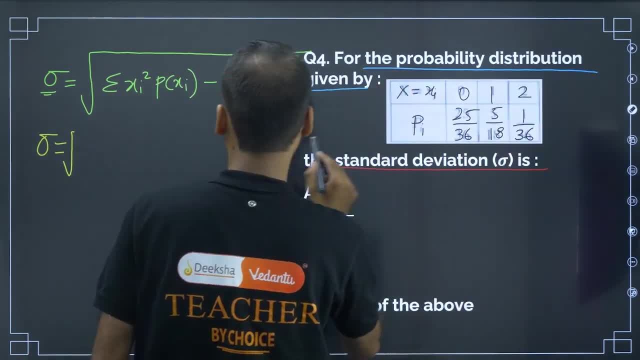 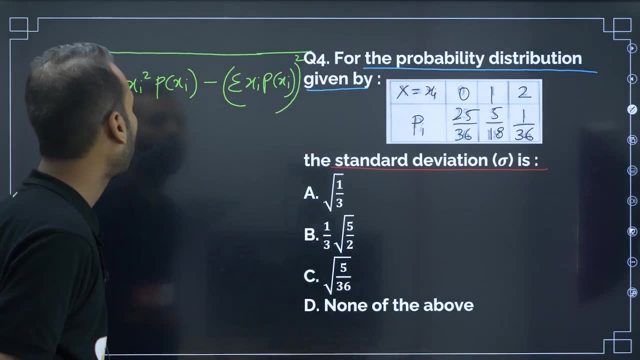 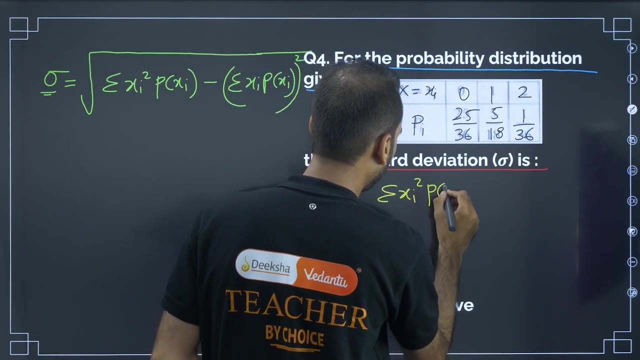 to under root of alpha. Let me calculate it before only, and then I will go for substitution. So xi square is 0, p of xi is: if you multiply this summation, xi square p of xi, p of xi is equal to 0, and 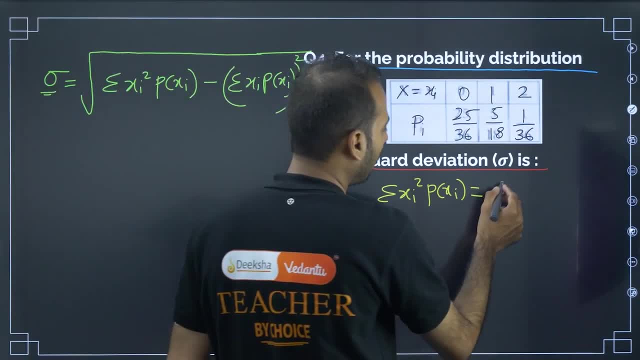 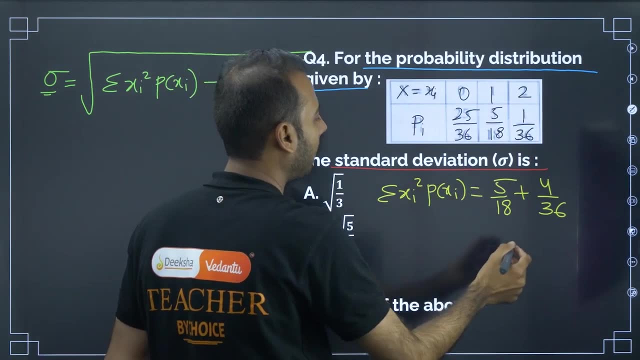 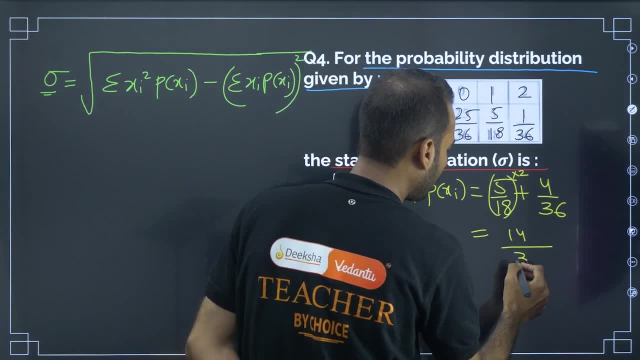 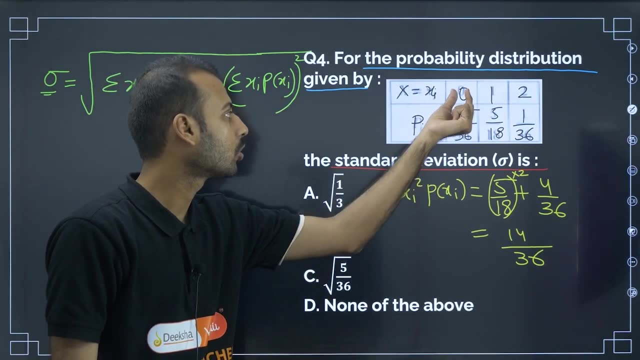 2. So you will get 14 by 36.. Summation xi square p: i means we have to square xi and then multiply with this, So 0. I am not writing 1 square 1,, 1 multiplied by 5, by 18,, 5 by. 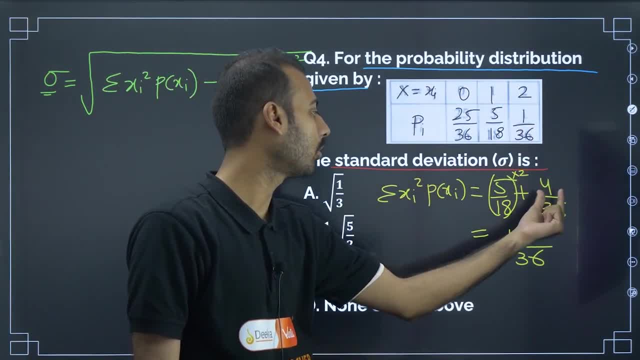 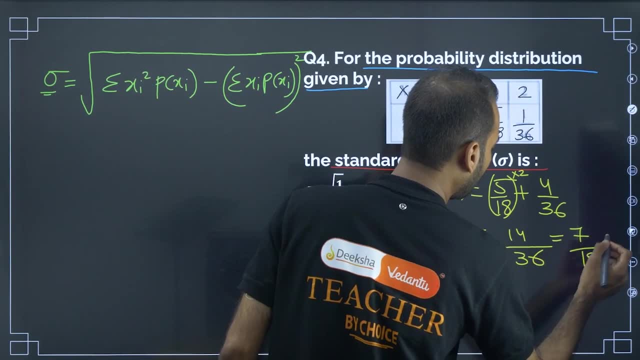 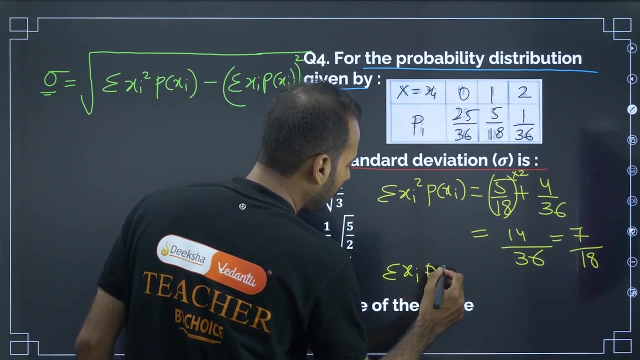 18.. Next xi square is 4,. 4 into 1 by 36 is 14 by 36.. So 14 by 36 is equal to 7 by 7 by 18.. Next summation xi p of xi. Summation xi p of xi. So here summation means addition. 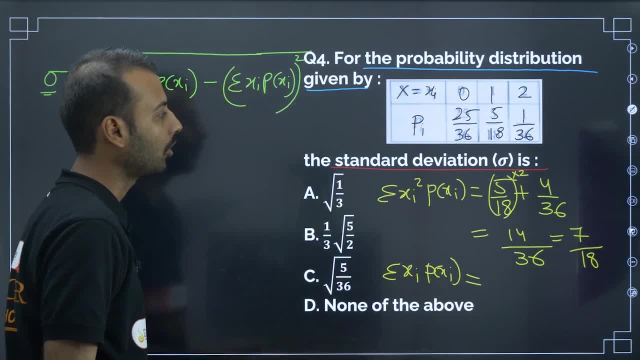 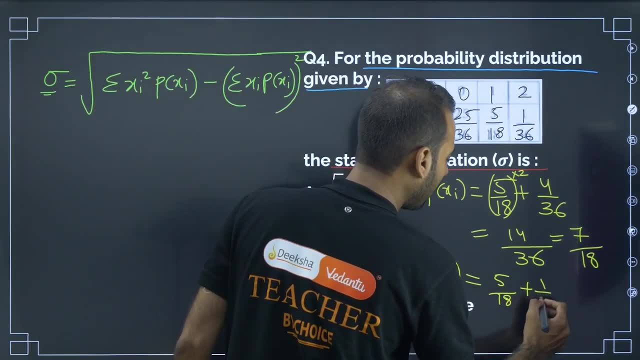 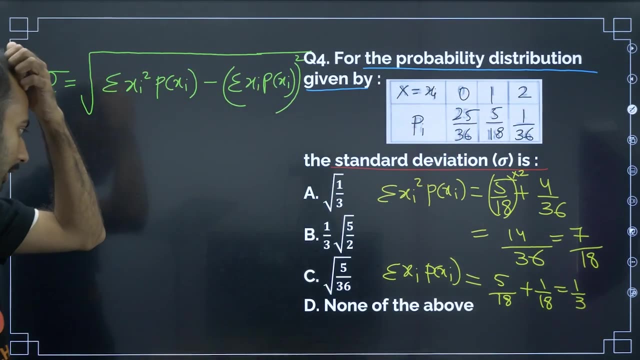 xi. p of xi. we have to multiply this and this. you multiply 0.. Next, 5 by 18, 5 by 18 plus 2 by 36 is 1 by 18 is equal to 6 by 18, is by 18 is 1 by 18.. Next, 5 by 18 plus 2 by 36. 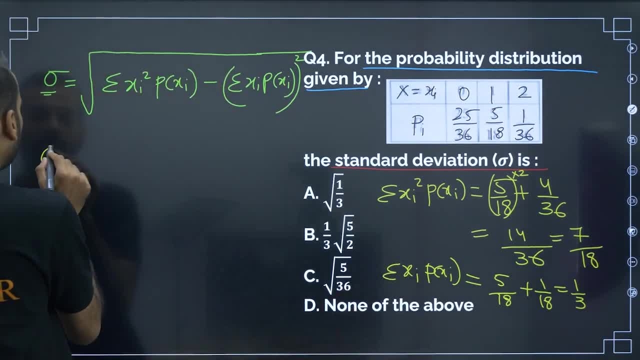 is 1 by 3.. Now, if you square this, now let me substitute. let me go for substitute: under root of: under root of 7 by 18, under root of 7 by 18 minus 1 by 3, minus 1 by 3 square. 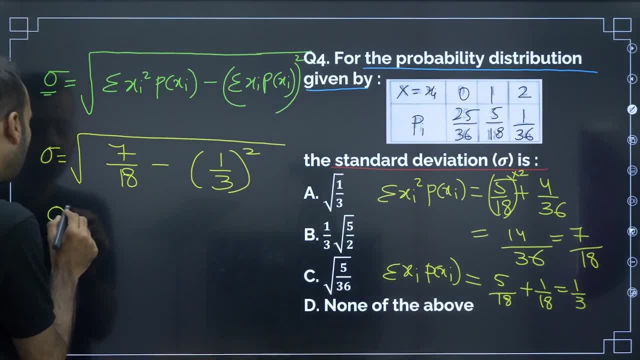 minus 1 by 3 square, So sigma is equal to. sigma is equal to 7 by 18 minus 1 by 9, 7 minus 1 by 9.. For this let me multiply by 2.. So sigma is equal to 5 by 18.. Is there? 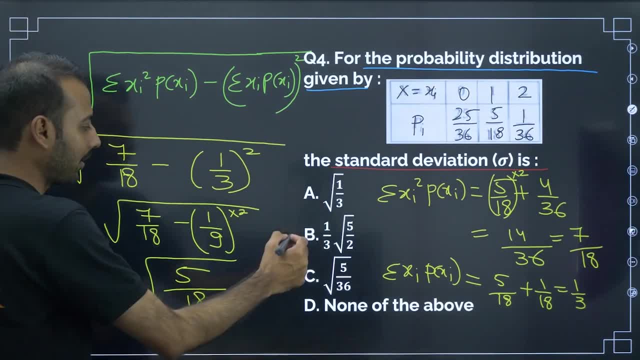 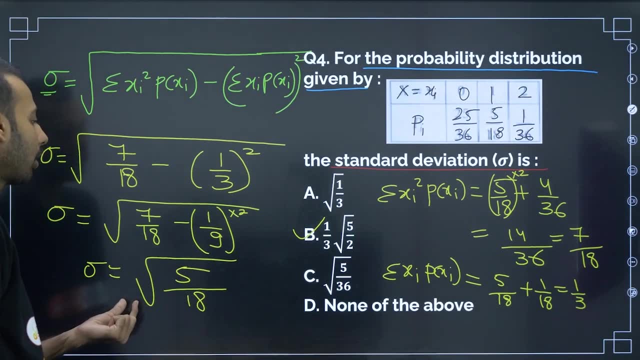 any option like 5 by 18?? Yes, B is the answer for this. Just simplify. readymade it is not available. 18 can be written as 9 into 2.. 9: if I keep outside of bracket, I will get. 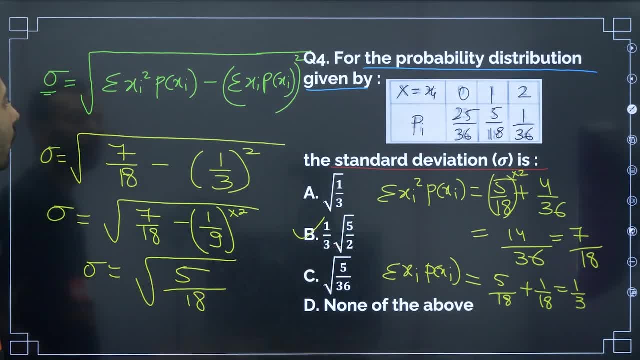 3 and inside it is 2.. So the answer for this is So very easy question: What was the thing? What knowledge was required? Only this much of knowledge was required to solve this problem. That's it, Nothing else. 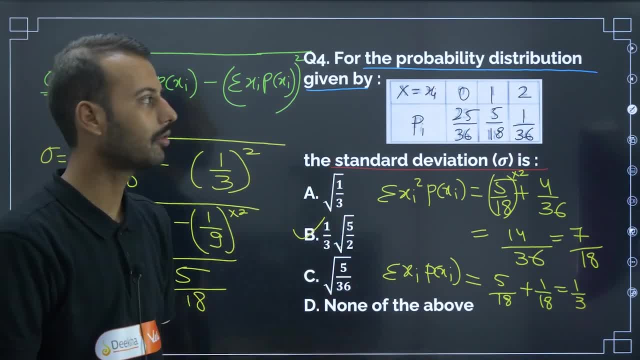 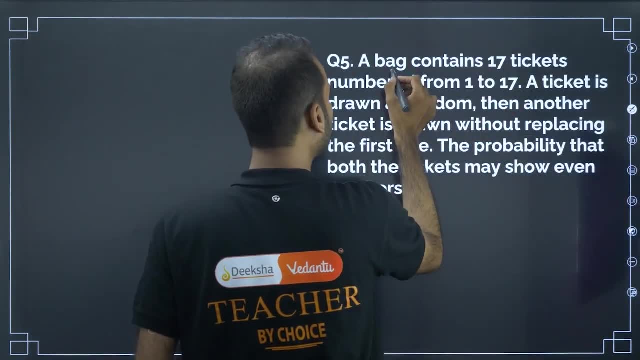 Only this knowledge Remaining: calculation, addition, subtraction, multiplication, division- that you should be known. Next, moving on to next question: A bag contains. what does a bag contains? A bag contains 17 tickets numbered from 1 to 6, 17.. Let me draw the. 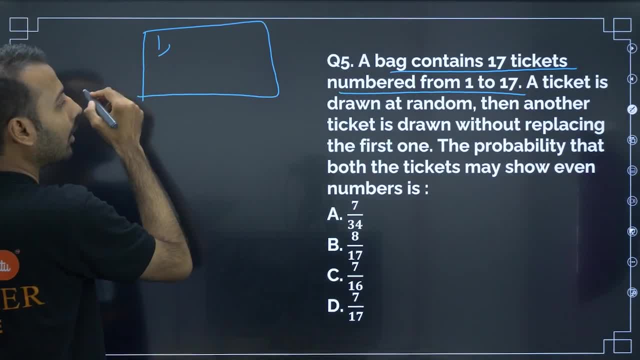 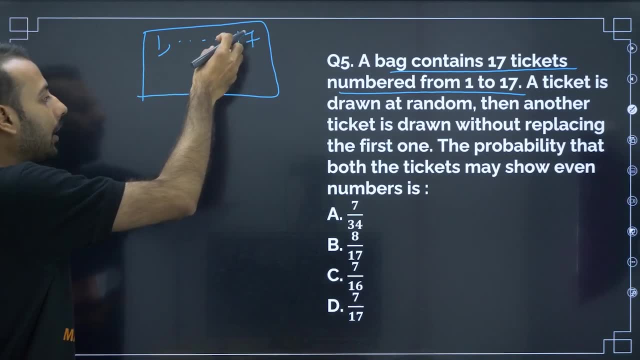 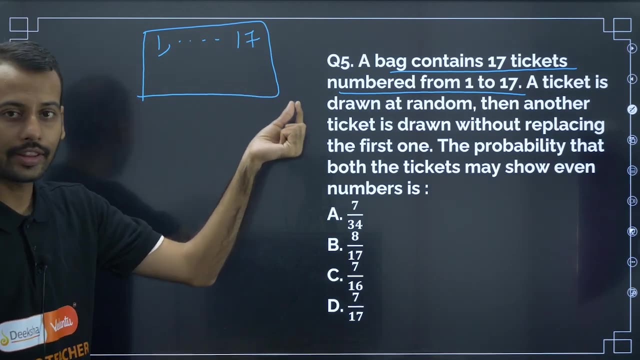 graph box for that: 17 tickets from where to where, 1 to 17, from 1 to A ticket is drawn at random. They are drawing one ticket at random, Then another is drawn without replacing the first. That means a ticket is drawn, One ticket they have drawn and another ticket is drawn without. 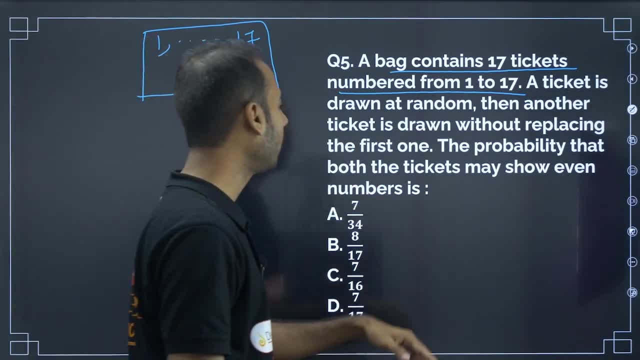 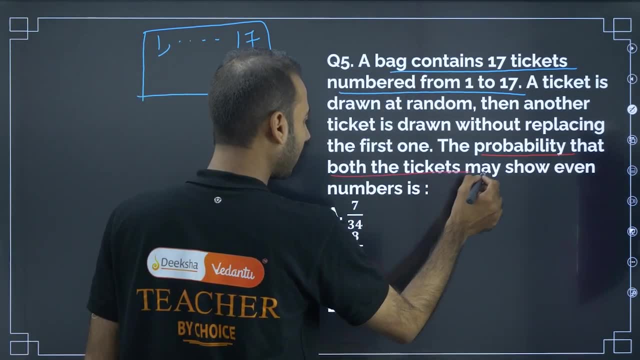 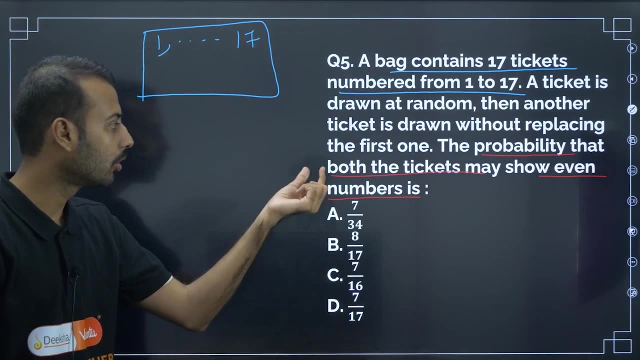 replacing means: first ticket is outside, only next ticket. The probability that? what is the question? The probability that both the tickets, both the tickets may show even numbers, may show even numbers, is the probability that both the tickets. The probability now, what is the question? 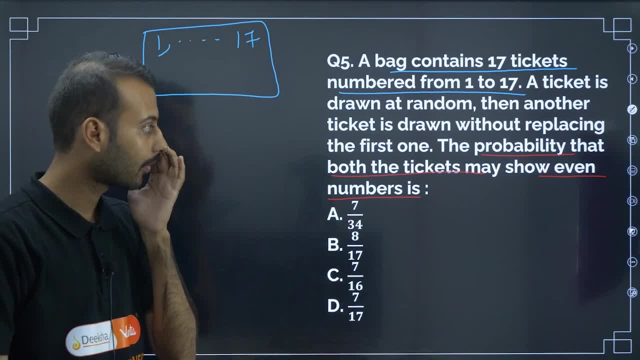 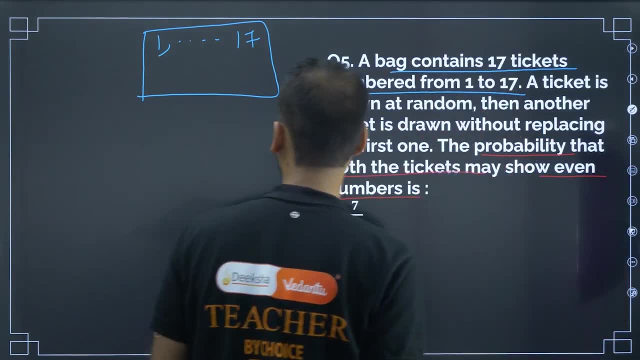 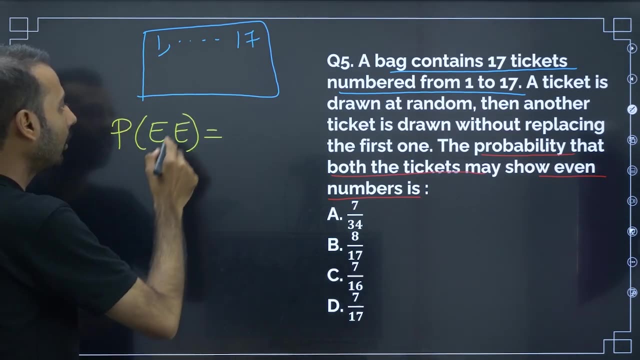 The probability that both the tickets may show even number is: both may show even number is. So how to approach this problem? So probability that both, even, even, even for first, even totally 8 are there and then favorable 8 by second. 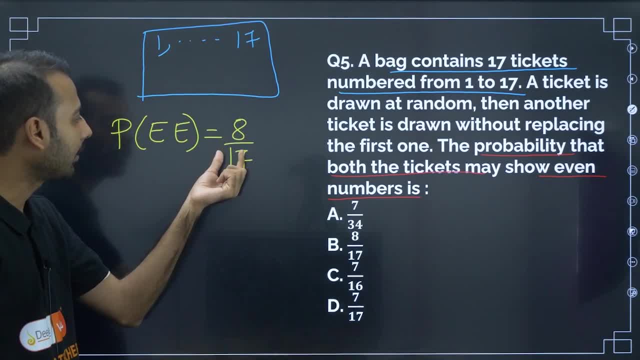 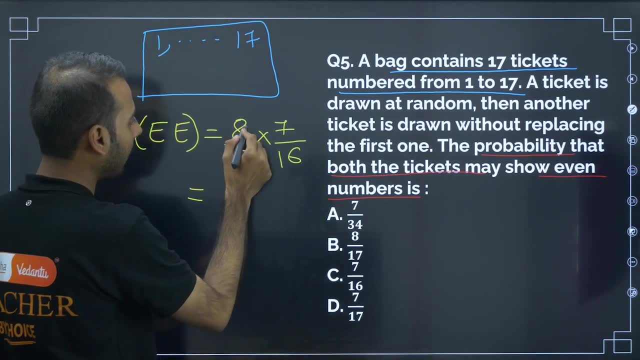 Using classical definition of probability, we can write favorable case 8 by 16.. In the next case there are only 7 and there are only 16 left. So for this I can write this as by 2, 7 by 34.. 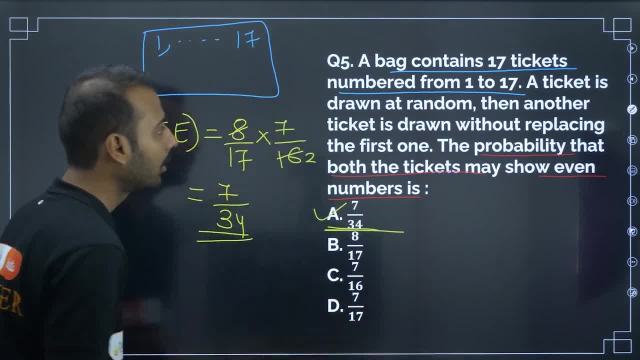 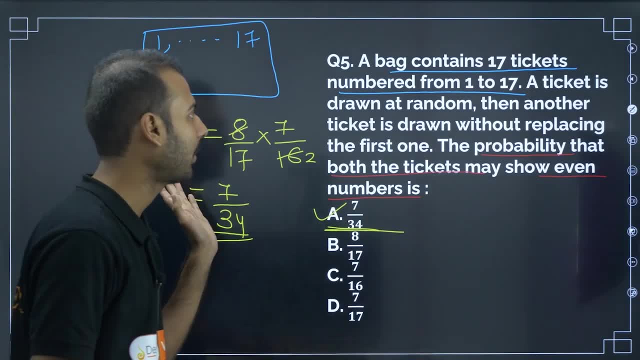 So is there any option like 7 by 34,? yes, see here again. easy question, very easy question. just you just have to do this calculation. hardly, I will say 10 or 15 seconds maximum to solve this question. Moving on to next question, 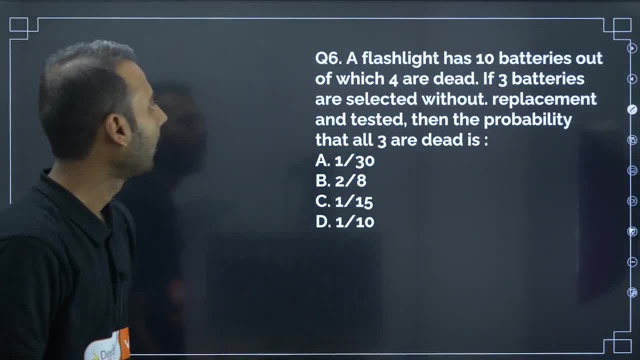 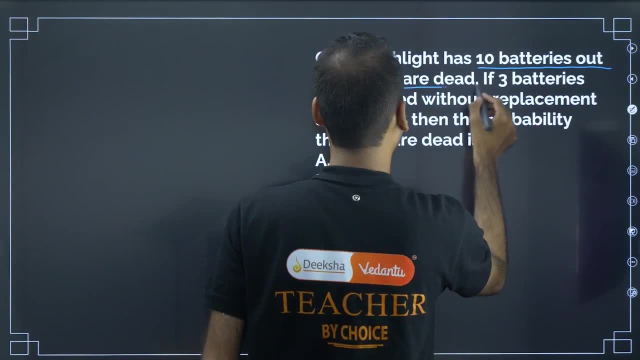 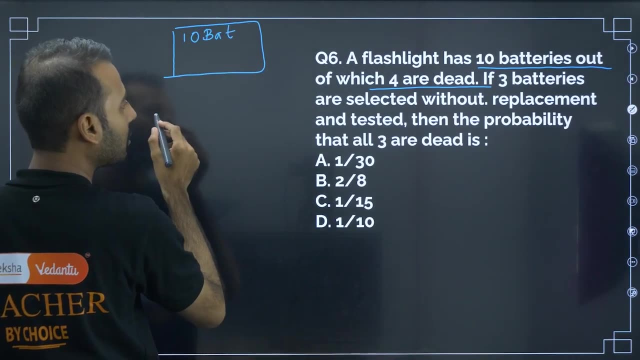 A flashlight has 10 batteries. A flashlight has 10 batteries, out of which 10 batteries out of which 4 are dead. So let me draw. has 10 batteries, 10 batteries out of which 4 are dead batteries, 4 dead. 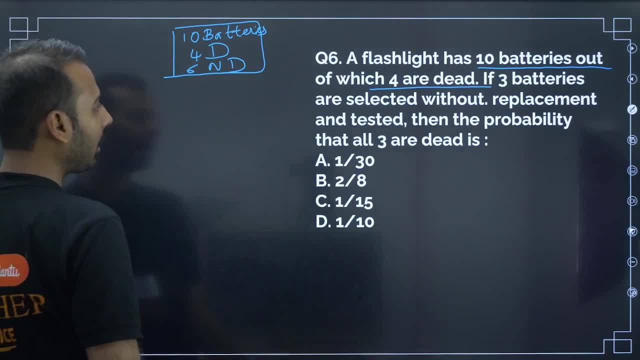 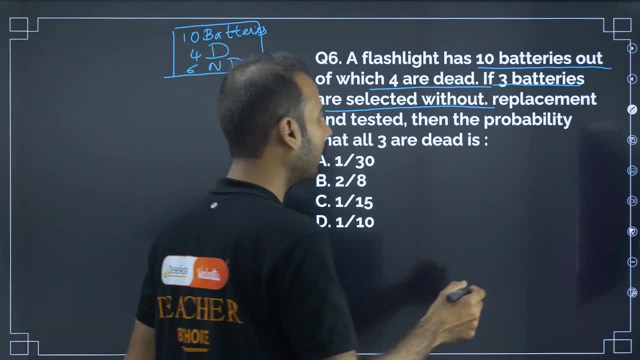 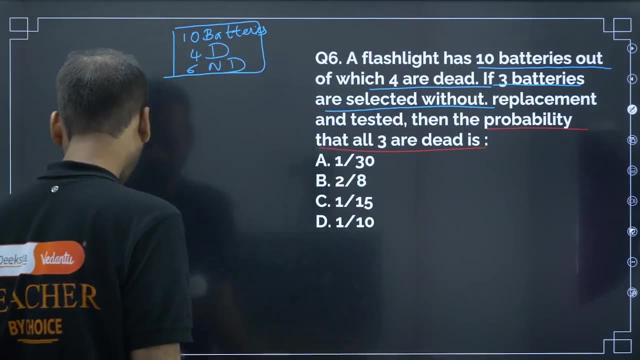 means 6: non-dead. non-dead: If 3 batteries are selected, 3 batteries are selected without replacement and tested, then all 3 dead. all 3 dead. probability that all 3 are dead is probability of all 3 are dead. 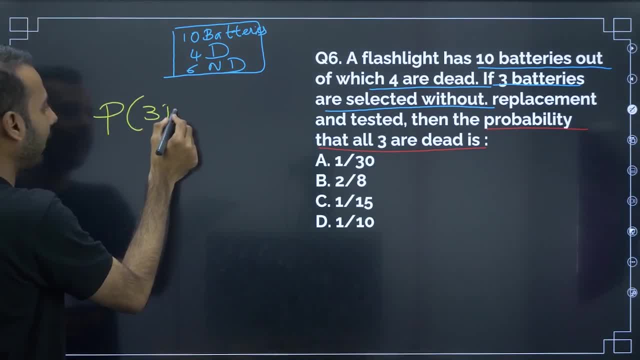 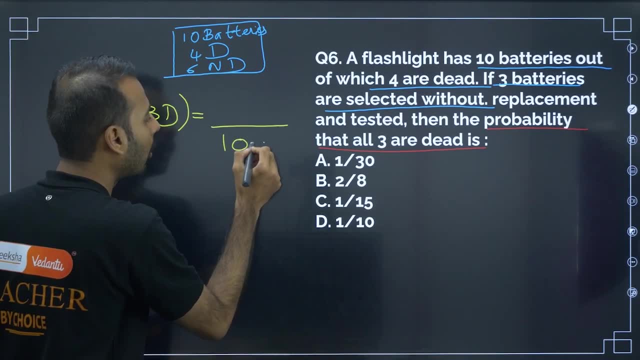 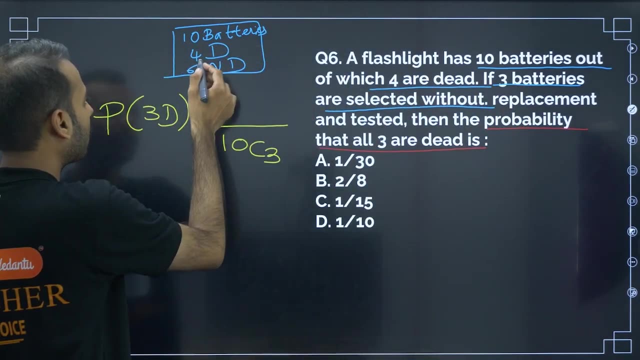 is probability. all 3 dead is now total favorable cases by total cases total. how many batteries? 10 batteries, out of which we have to choose 3 batteries. So next, if 3 batteries are selected, 3 batteries out of dead only we have to select. 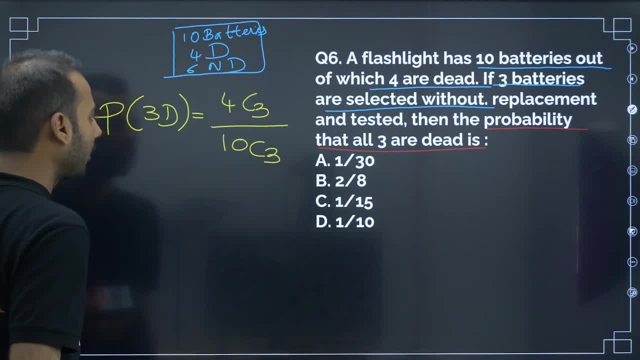 So 4 dead, 4 dead, 1 dead, 2 dead, 3 dead, 1 dead. So that is correct. so shall we write: 4 C, 3 divided by 10 C. Now NCR, formula N factorial. 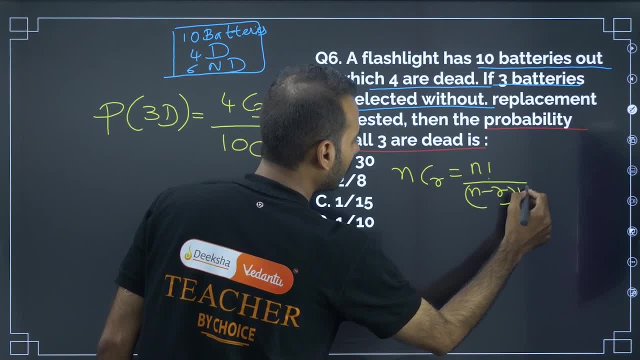 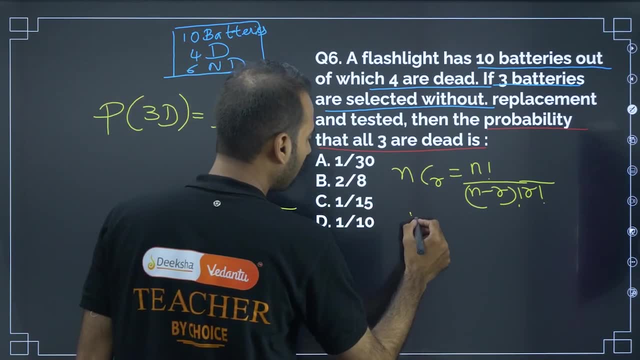 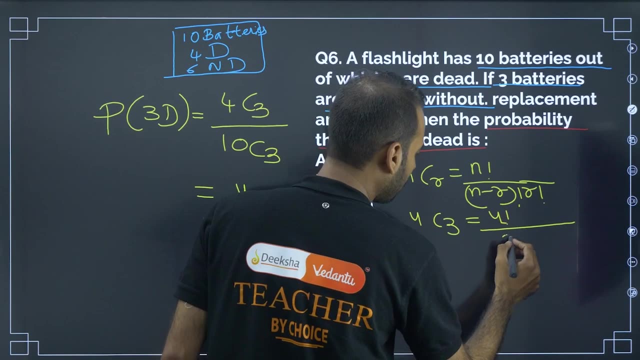 by N minus R factorial into R factorial, So 4 c 3 is 4.. How to calculate: 4 C 3 is 4 factorial by 4 minus 3, 1, R is 3 factorial, So 4 C 3 is equal to 4.. 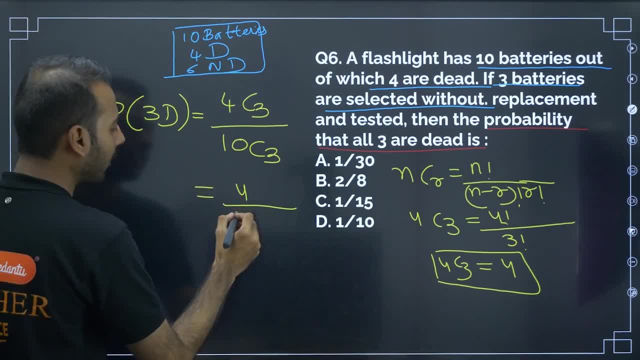 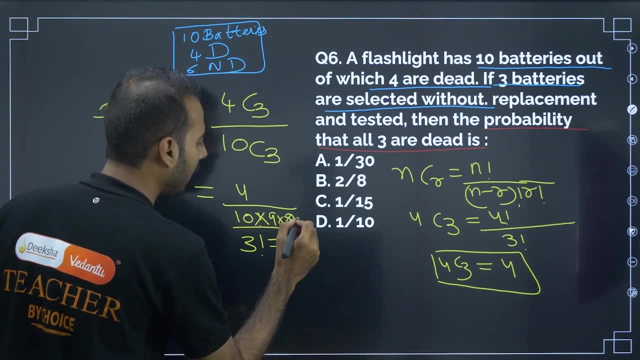 4 C 3 is equal to 4.. 4 C 3 is equal to 4.. to 4. in the same way, 10 factorial, 10 factorial by 3 factorial, 7 factorial, So 10 into 9, into 8, into 7 factorial, 7 factorial, 7 factorial gets cancelled. 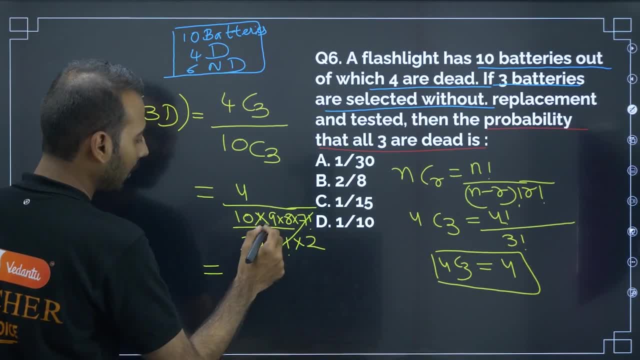 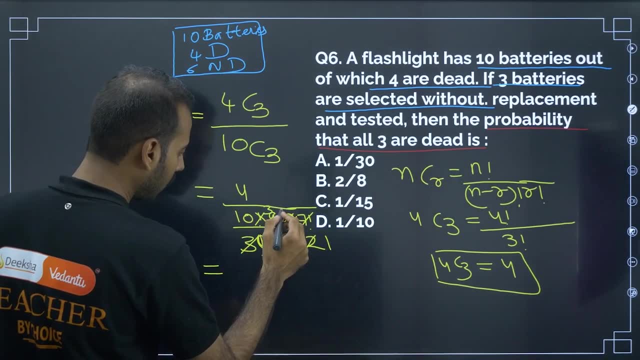 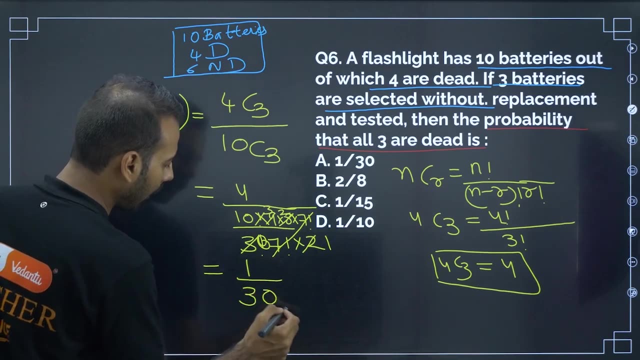 So here we are left with 3. factorial means 3 into 2, 3 ones are 3, threes are 2, ones are 2, ones are 2, twos are. so, after cancellation, here we are left with 1 by 30 after simplification. 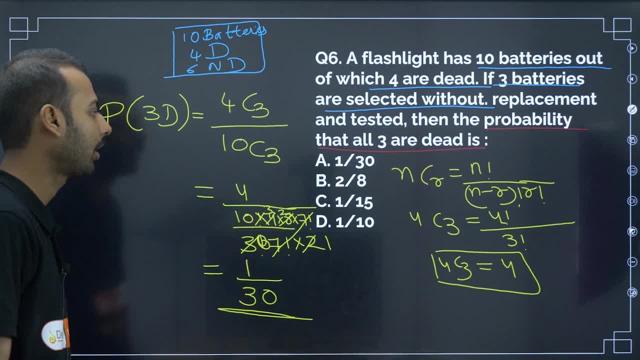 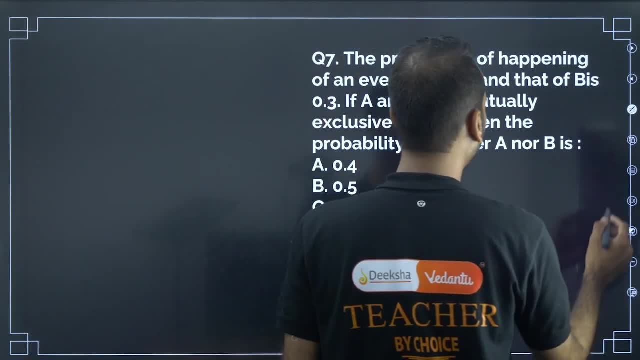 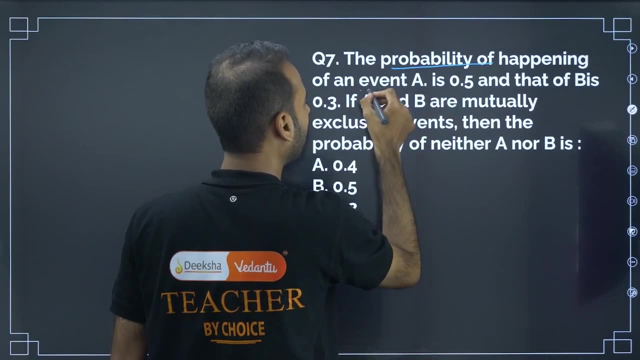 we just have to simplify this: 10, C, 3, all this we are left with 1 by 30. So answer is 1 by 30. moving on to next question, The probability of happening of event A is of an event A is 0.5 probability of happening. 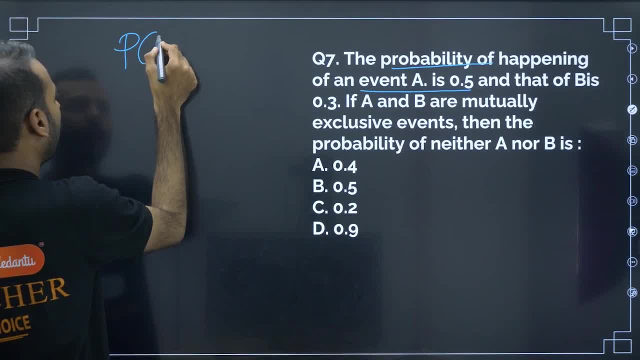 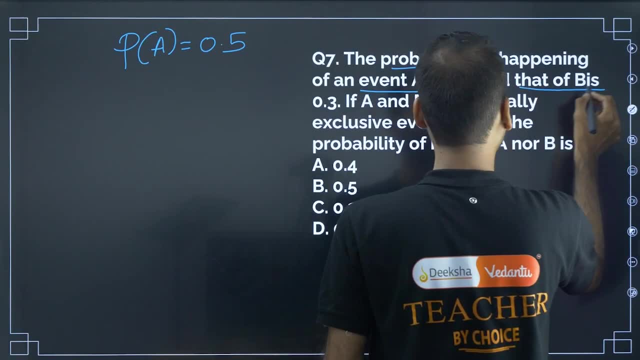 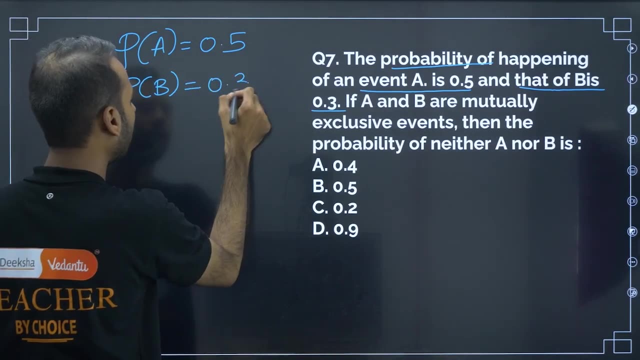 of an event. A is 0.5. So probability of happening of event is 0.5 and that of B is 0.3 and that of B is 0.3. probability of happening of B is 0.3 if A and B are mutually exclusive. next statement: 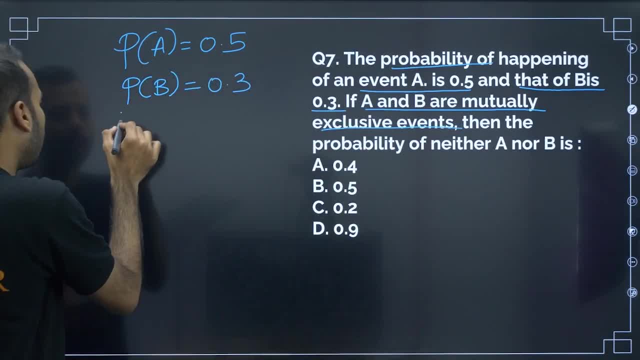 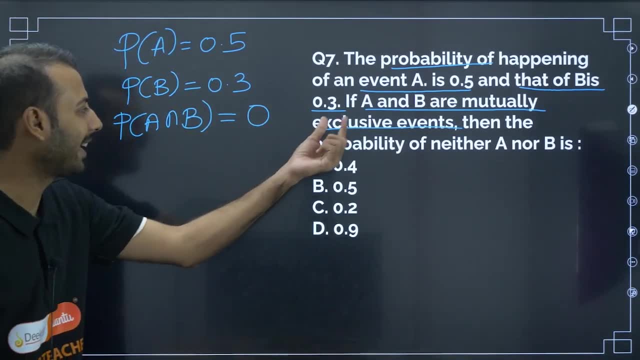 A and B are mutually exclusive events means what A and B are: if one occurs, another does not occur. So the probability of either A and B is 0.. Mutually exclusive means probability of A and B is 0. then probability of neither A nor. 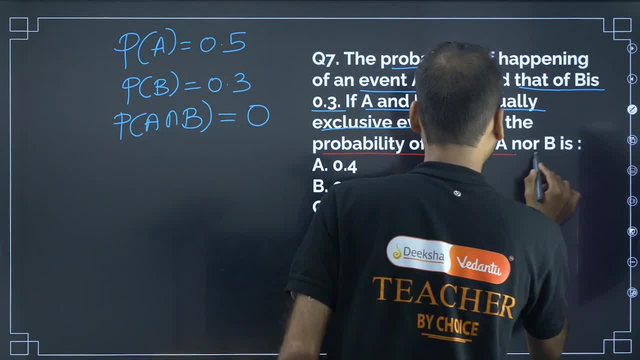 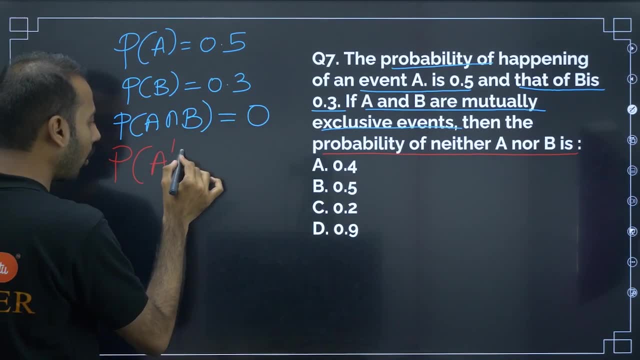 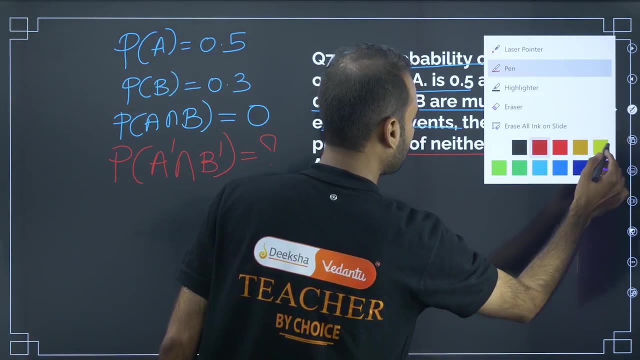 B is. what is the question? Probability of neither A nor B. Probability of neither A, neither A nor B. nor B is what? this is the question. Now some synopsis with basic knowledge. this p of A, intersection A, dash intersection B, So which is the같 amount of affordability? 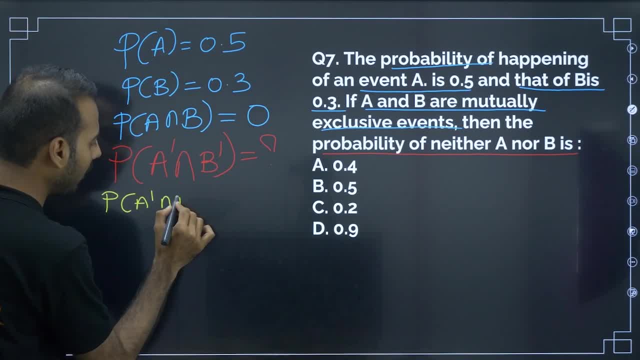 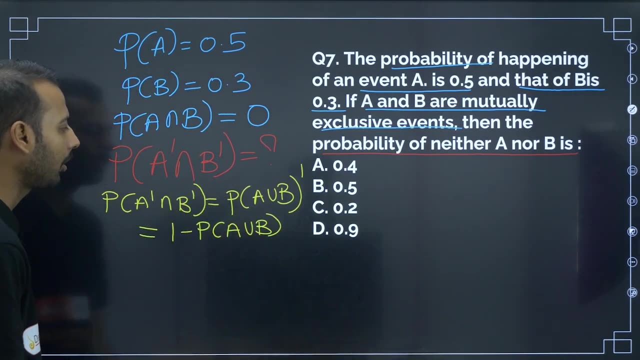 A Elliot, Then this is left as an asymptotic. these numbers are ad Shakespeare spanning books, no difference. 21 and 4 is what A dash intersection B dash can be written as P of A union B. dash is equal to 1 minus P of A union B, 1 minus A union B. from synopsis, from synopsis, I am dragging all the knowledge. 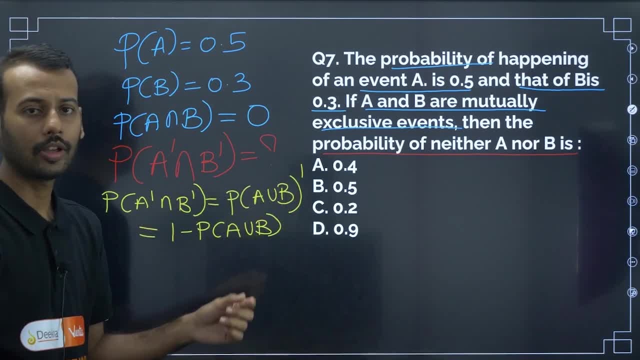 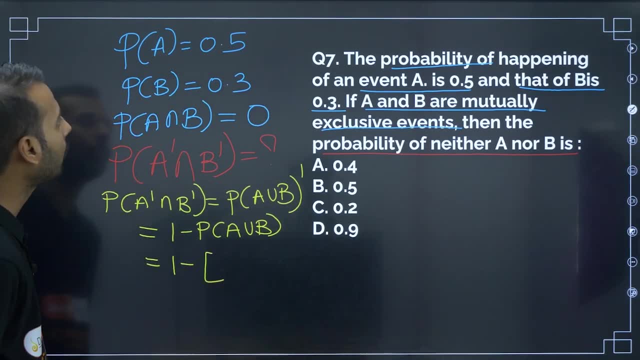 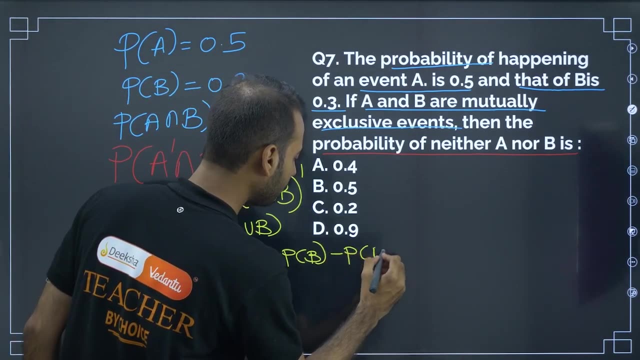 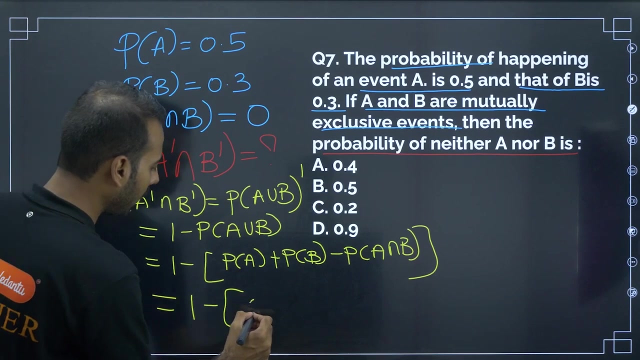 from synopsis: A union B dash: 1 minus B of A union B. if you do not know synopsis, please go through it. if you know, it is a good thing. next: 1 minus 1 minus P of A union B is P of A plus P of B, minus P of A intersection B. so 1 minus P of A is 0.5, P of B is 0.3. this: 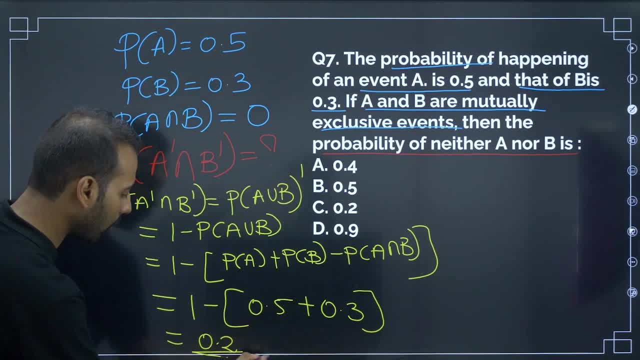 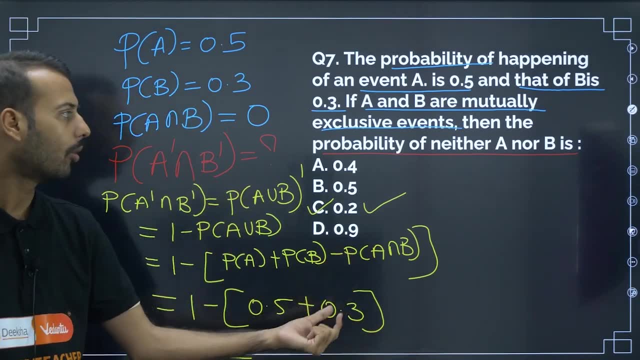 is 0, so I am not writing. so finally we are left with 0.2. is there any such option? yes, C is the answer. see here again. easy level question, only nothing complicated if you know basics, basics like this one, only this formula was required to solve this, so this is a basic. 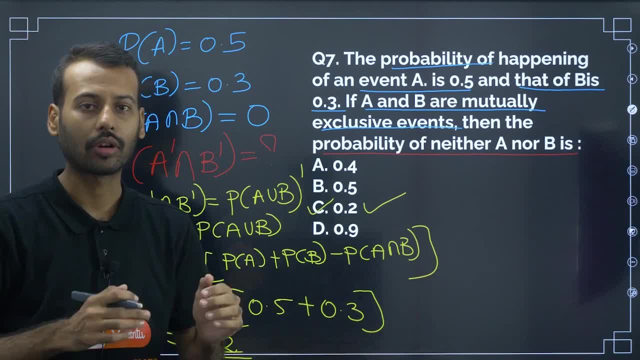 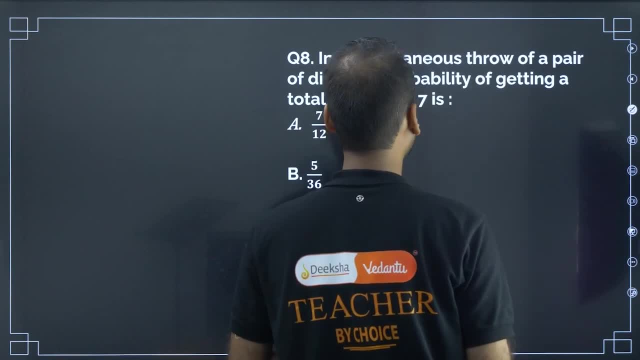 formula. please go through ncrt synopsis very well: A to your soul, A to your DNA. this synopsis points next. move on to next, in a simultaneous throw of pair of dice, the probability of so one random experiment. they are performing in a simultaneous throw of pair of dice, so 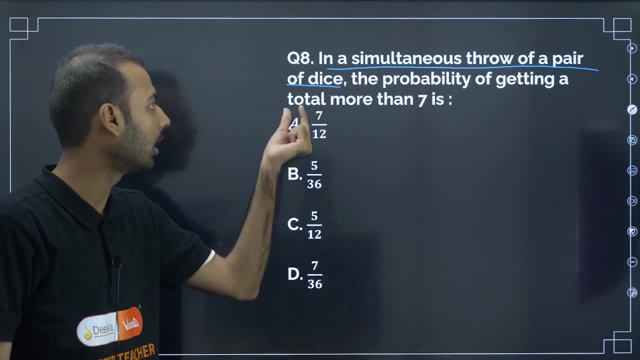 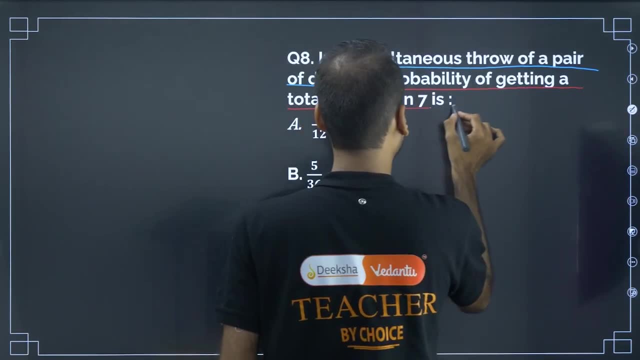 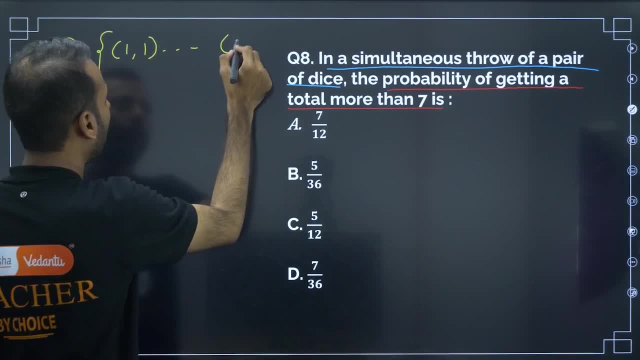 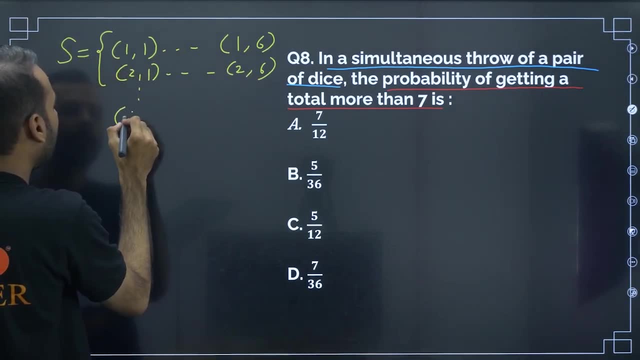 two dice are thrown. this everybody should be knowing: 1, 1, 1 up to 1, 6, 2 1 up to 2, 6. next, in the same way, 6, 1 up to 6, comma 6 total more than 7.. 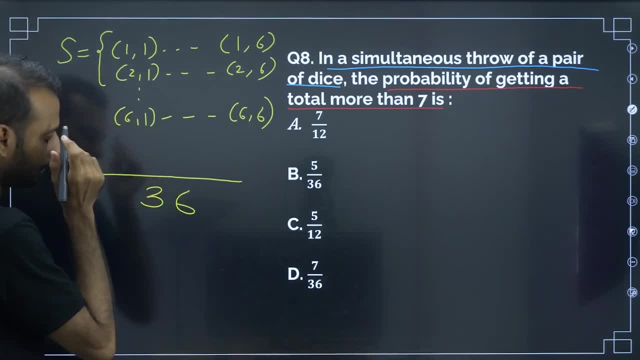 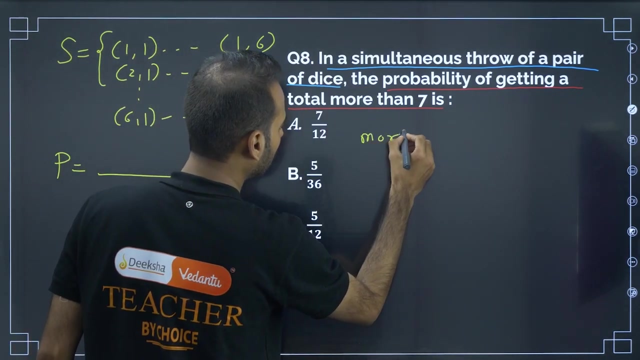 probability is equal to total is 36. total is how much? 36 total is how much? 36 more than 7. total more than 7 is more than 7 means here only one possibility is there. so more than more than 7 more than. 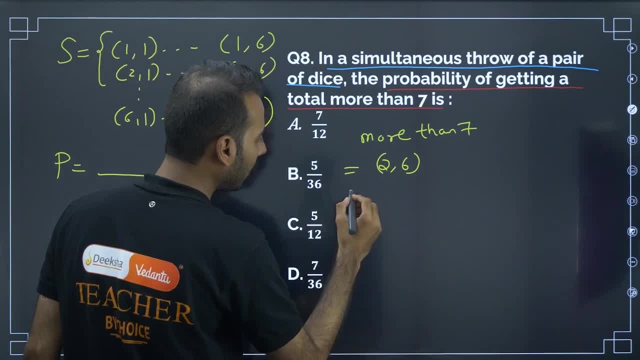 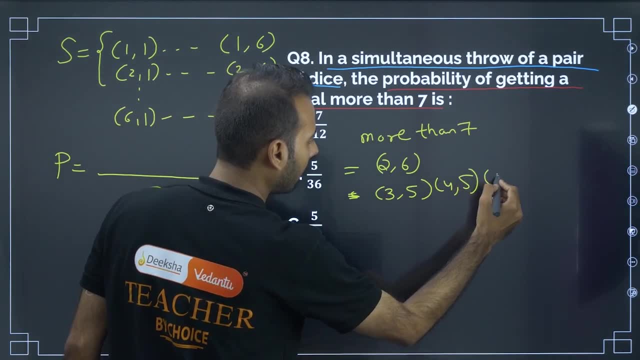 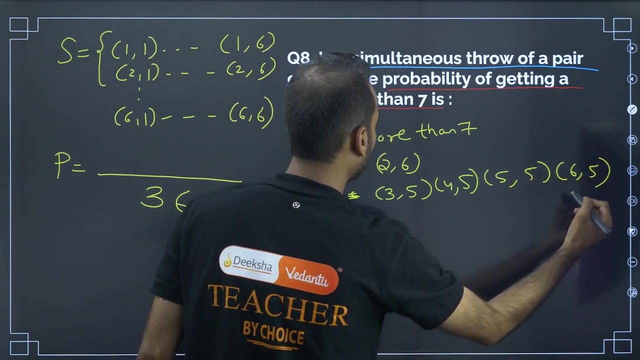 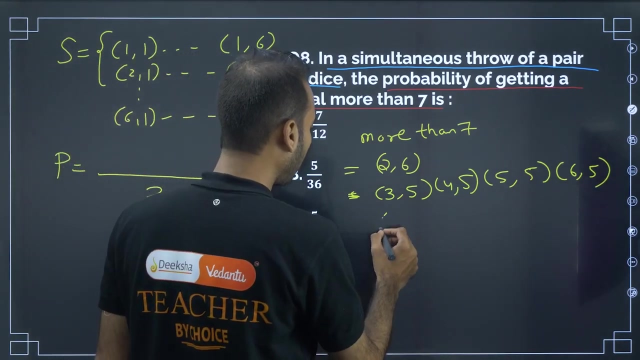 7. are there 2 comma 6, this is one possibility. Next, 3 comma 5, 4 comma 5, 4 comma 5 and 5, 3, 5, 4, 5,, 5, 5, 6, 5, 2, 6, 3, 5, 4, 5, 5, 5, 6, 5.. Next for this, 4, 5.. 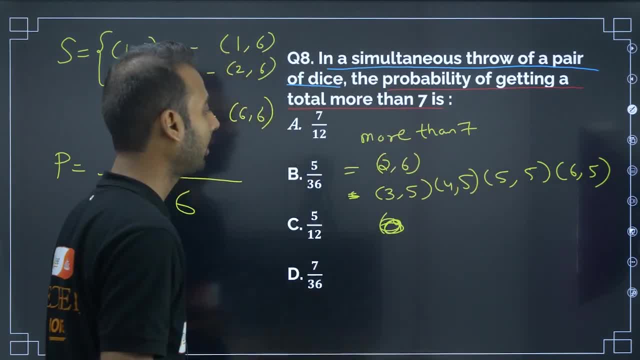 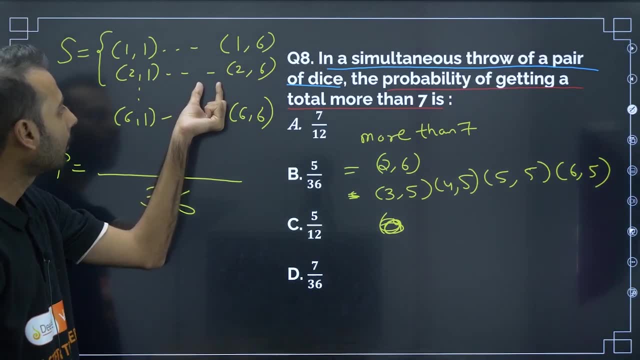 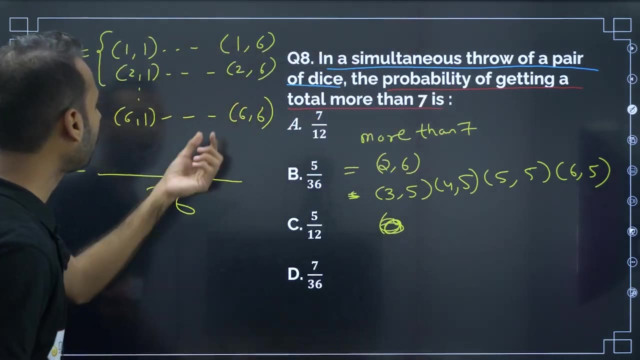 Next, if you count more than 5,, more than 7 means 2- 6,. here we will get 2- 6,. in the next one, we will get here. in the next from here, we will get 2 comma 6, only this is possibility. 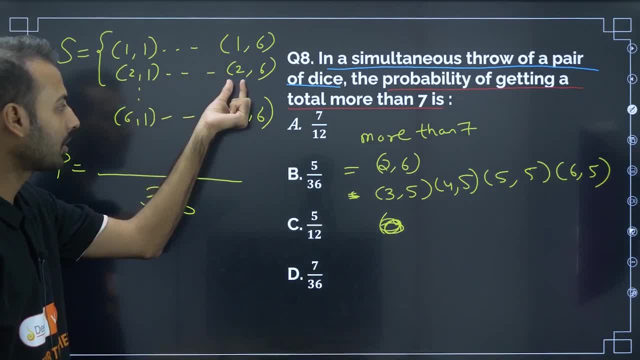 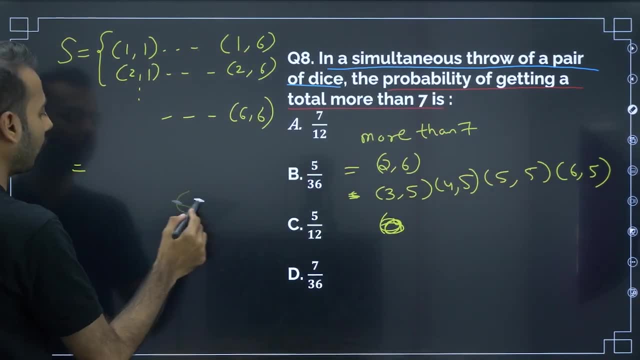 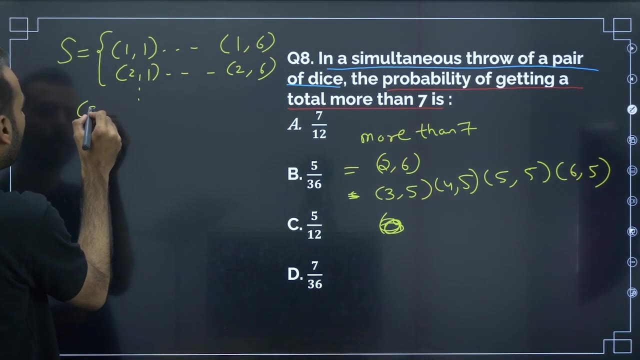 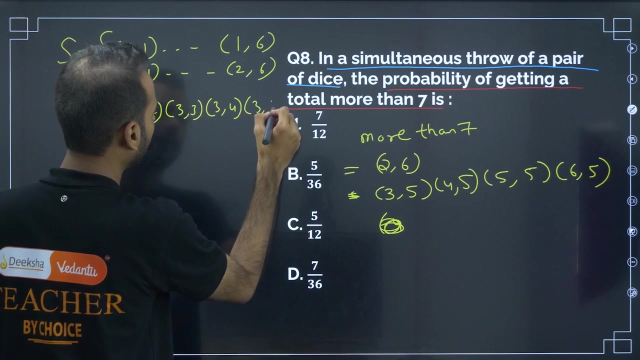 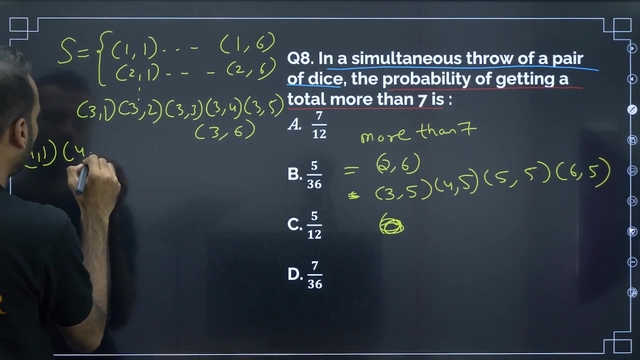 in the next 3, 6, we will get 4, 6. also we will get 5, 6, 6, 6.. Let me write this properly so that you can understand. It will be easier for us to get those. So: 3, 1, 3, 2, 3, 3, 3, 4, 3, 5,, 3, 6.. Next, 4: 1, 4, 1, 4, 2, 4, 3, up to 4, 6.. Next, 5: 1 and then 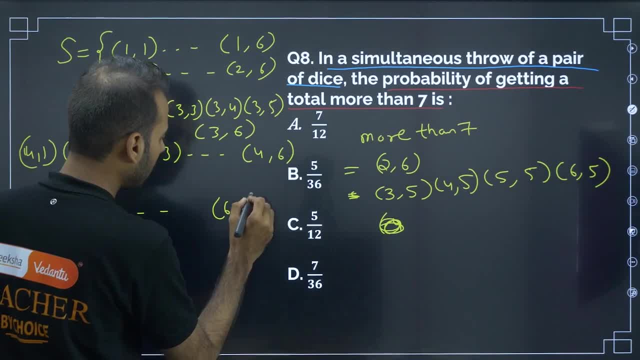 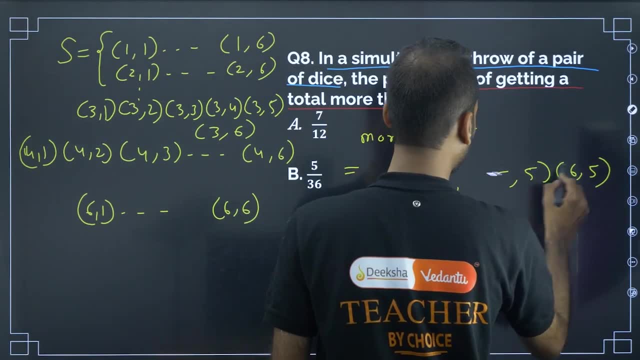 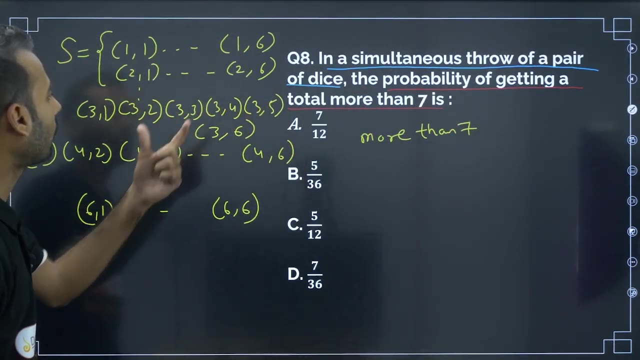 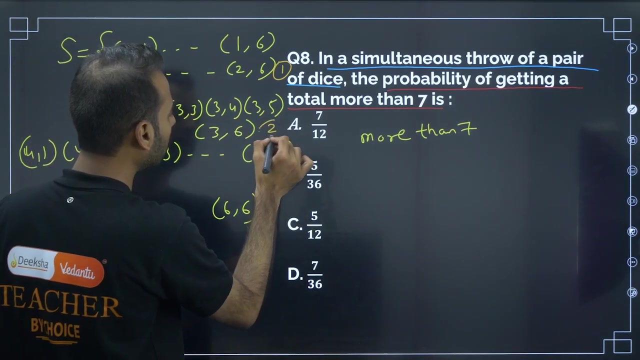 6, 1 up to 6, 6.. Now, if you observe, if you observe more than 7 or more than 7.. So, if you observe more than 7, how many more than 7 here? Here, 2 comma 6, only 1, you will get Next here. if you observe 3, 5, 3, 6, here you will get 2.. 4, 1, here you. 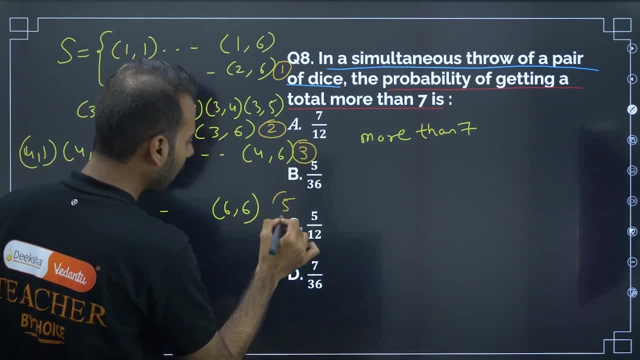 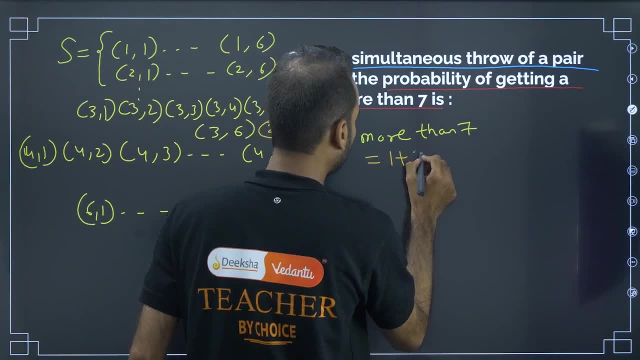 will get 3.. Next, 4, 5, 3, 6.. Next, 3, 1 to 3. here we will get 3.. And in the same way, finalized you way. finally, we will get 5 here, because 6, 2, 6, 3, so on. So more than 7, how many 1 plus. 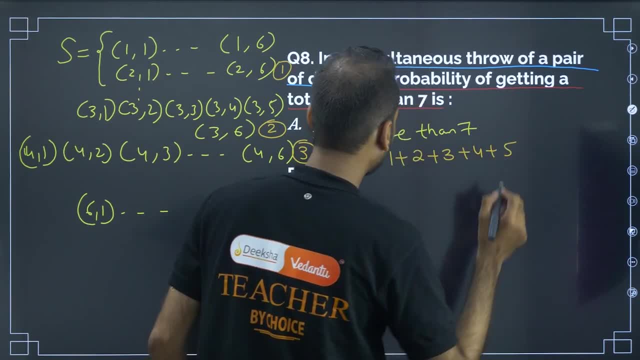 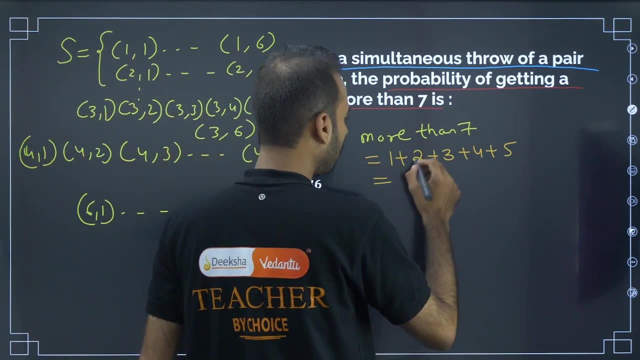 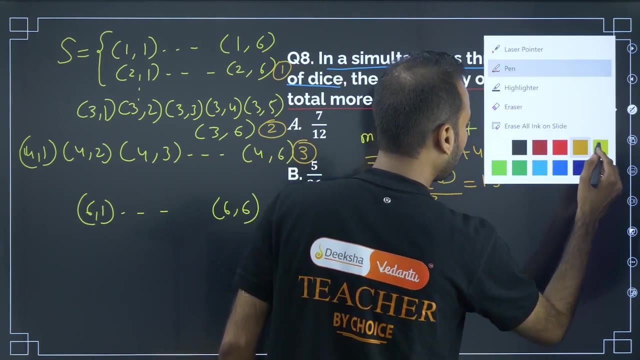 2 plus 3 plus 4 plus 5.. So here, in this row 1, in this row 2, this row 3.. So what is this 5?? So, if I take summation of this, 6 by 3 is equal to 15.. Now, favourable probability. 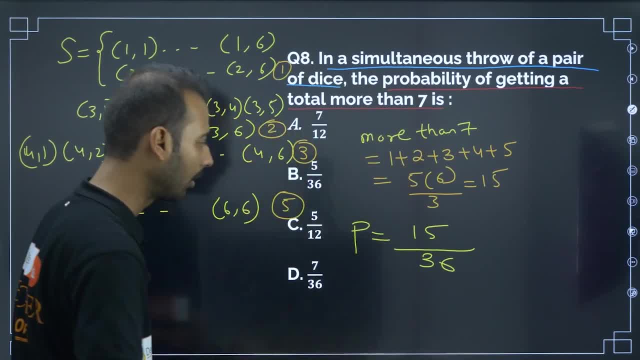 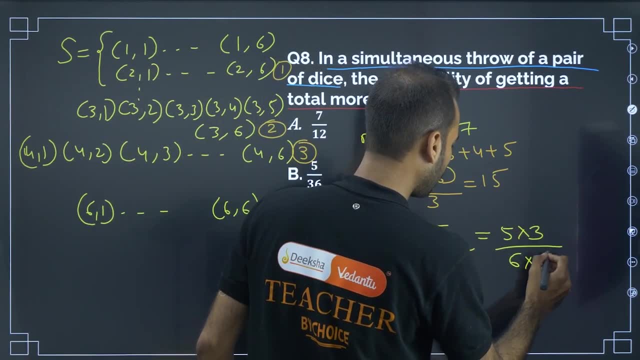 is equal to favourable 15 cases. total 36: total 36 favourable 15.. So 15: 15 can be written as 5 into 3, 5 into 3, 6 can be written as 6 into 6, 6 into 6, or else 5 by 5 into 3, 2 L. 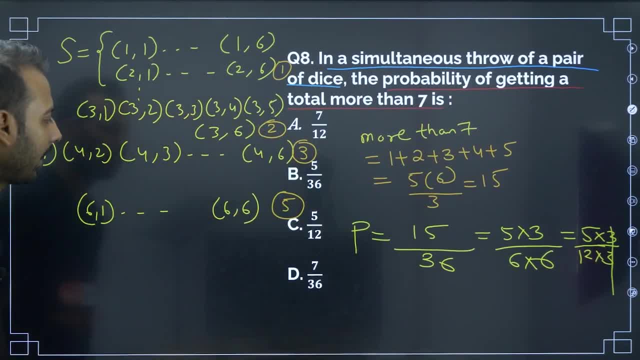 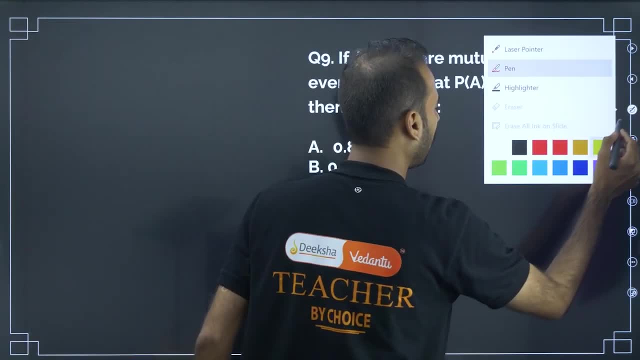 into 3.. So if I cancel 3 and 3, 5 by 2, L, is there any such option? Yes, C is the answer for this. Moving on to next question, If A and B are mutually exclusive events, what? 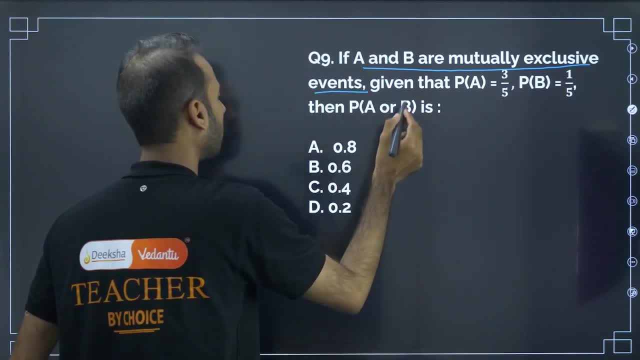 are they talking about? A and B are mutually exclusive, So they are mutually exclusive events. So let us see So. A and B are mutually exclusive events, So let us see So let's. mutually exclusive events. mutually exclusive events means if one event happens, other does. 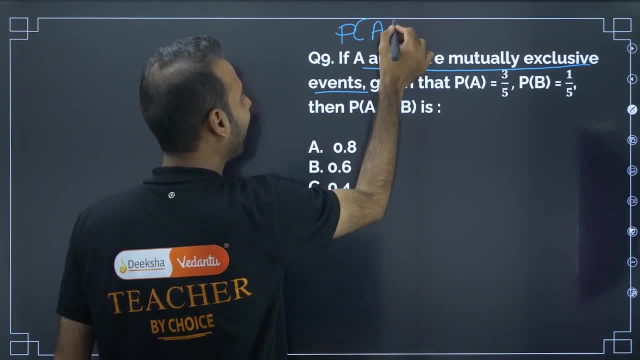 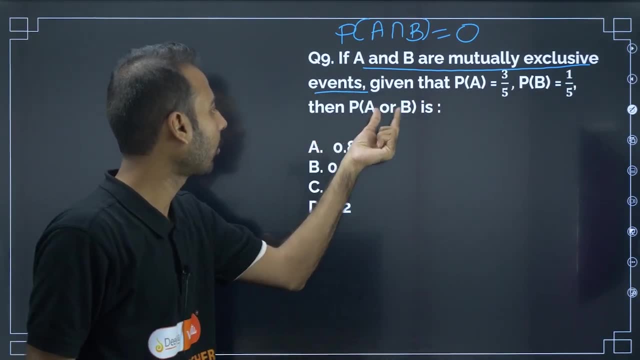 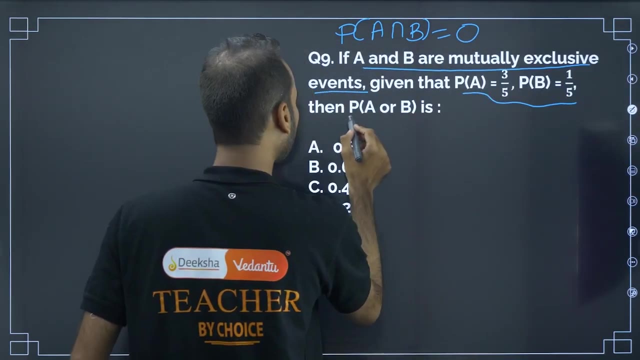 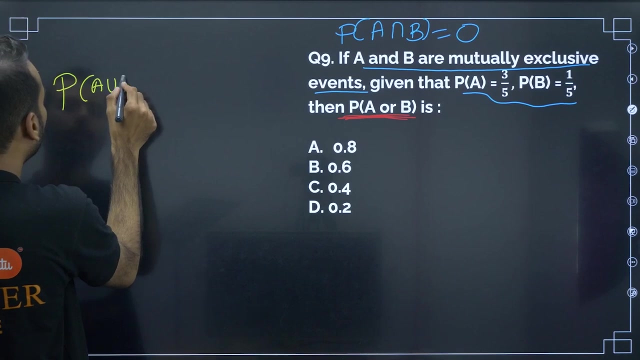 not happen. that means what probability of a intersection b is 0, mutually exclusive. given that a is equal to 3 by 5 b, then probability of a or b is what are they asking? they are given this much of data and they are asking this: p of a or b. so p of a or b is p of a union. b is equal to. 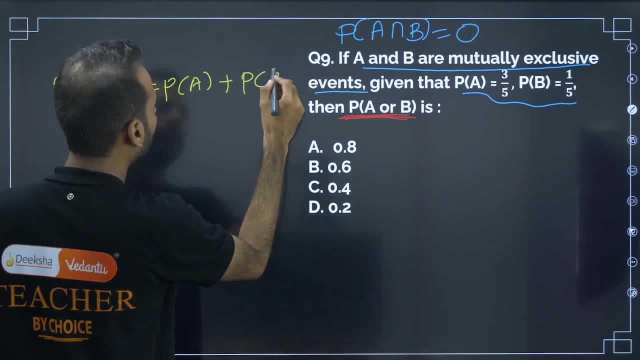 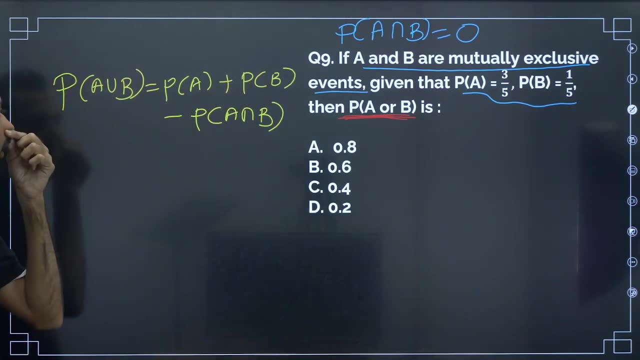 p of a plus p of b minus p of a. intersection, b, addition, theorem of probability: this is very, very important, very, very important formula. so everybody should be knowing this. p of a or b is: p of a value is 3 by 5. p of a value is 3 by 5. 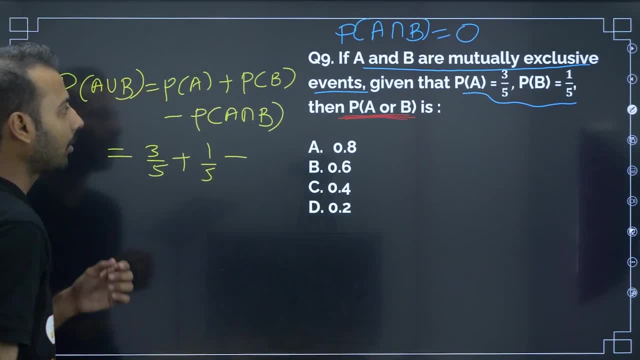 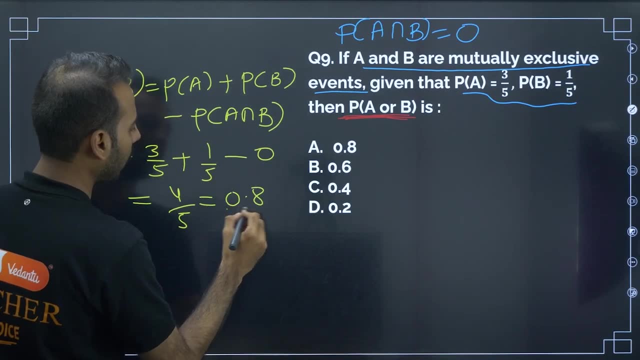 p of a value is 3 by 5. p of b value is 1 by 5. a intersection b: this is 0, so answer is 4 by 5, which is equal to 0.8. so if i know this formula, only one formula. 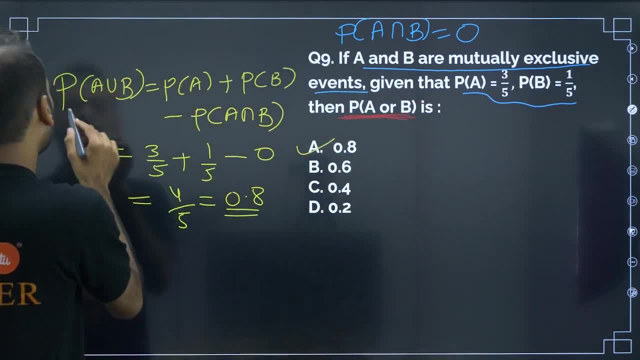 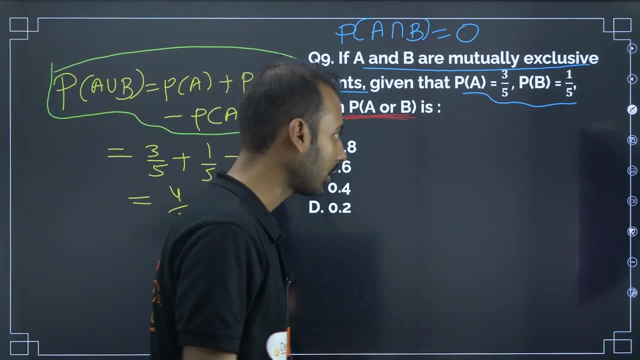 i was supposed to know. with that only we are able to solve this. so this: you take this as synopsis: p of a union b is equal to p of a plus p of b minus p of a intersection b. so 0.8 is the answer for this. moving on to next question: two letters are chosen. two letters are chosen. 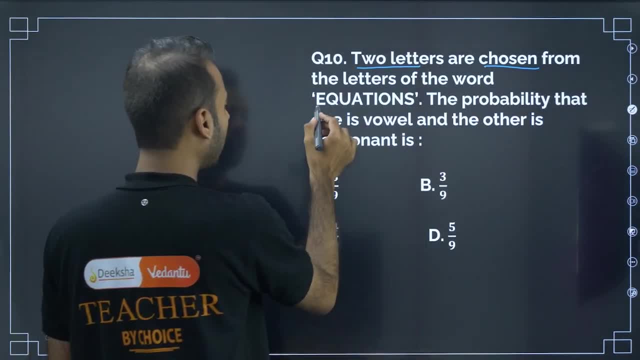 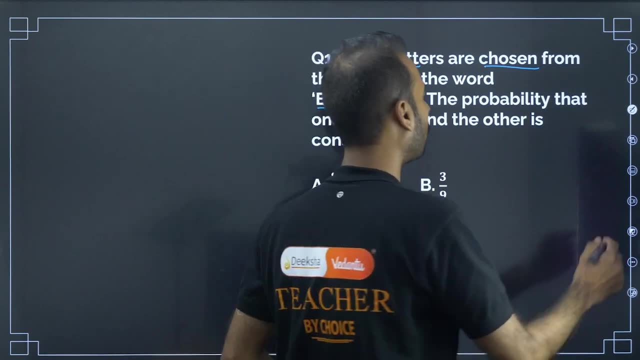 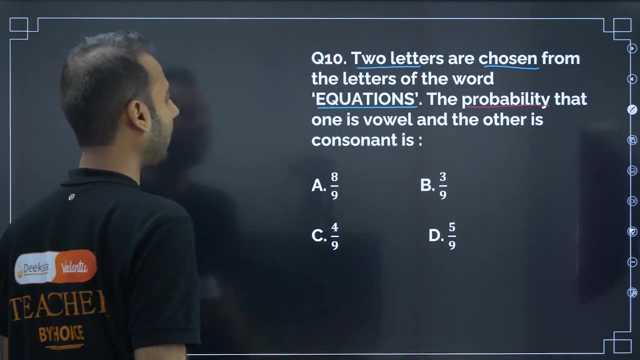 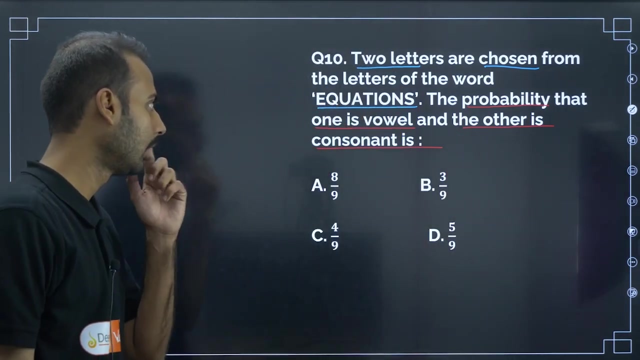 from letters of the word equations, equation from two letters. they are choosing from this equation the probability that one is oval. the probability, what are they asking? probability that one is oval and other is consonant. probability that one is oval and other is consonant. so for this, how to approach this? 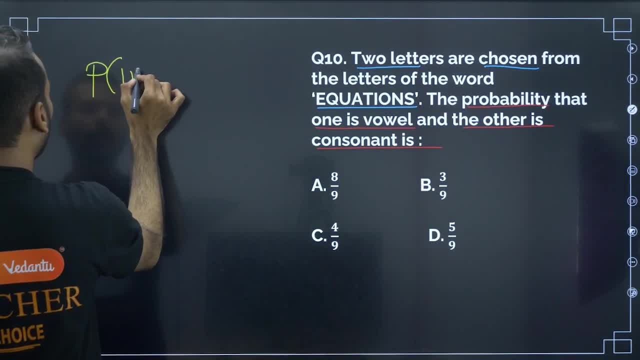 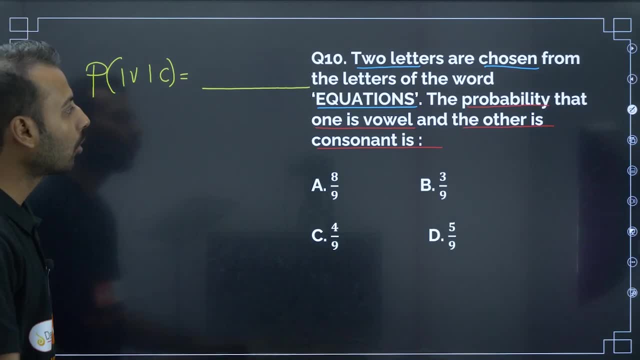 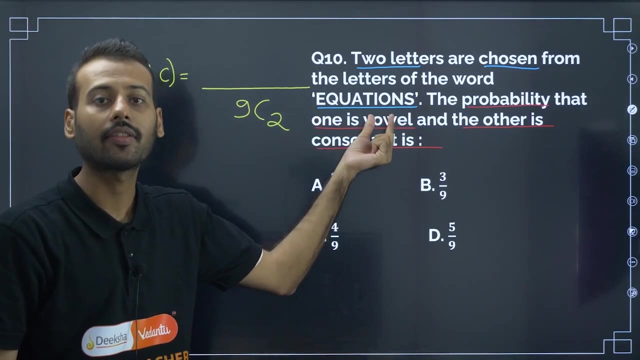 problem. see here probability of one oval. one consonant is two letters are chosen again here: favorable cases by total cases total. how many letters are there? three, three, nine. from this we are choosing two total nine letters are there from this i am choosing two, uh, two, so nine c two. total nine c two. 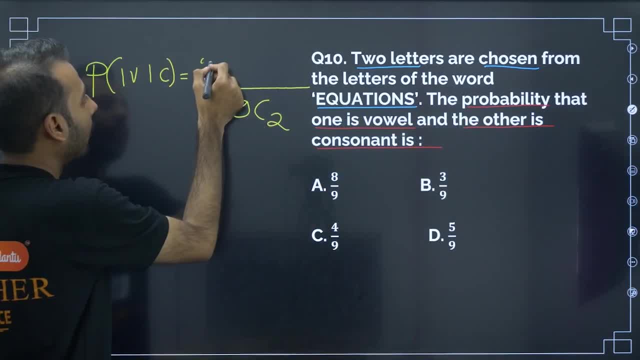 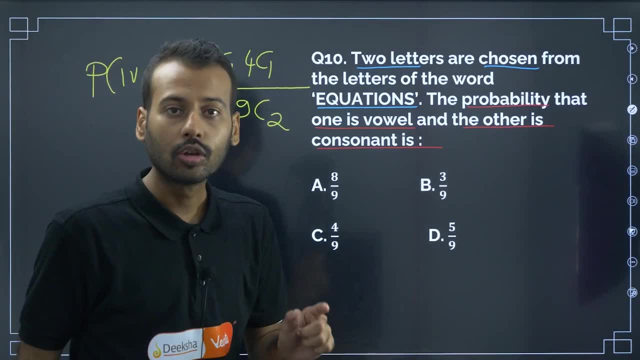 next one is oval. how many vowels are there? five ovals are there, from that, one is oval. 5 c, 1. next, four consonants are there, from that we are choosing one. so 4 c, 1, 5, 4 za, 20, divided by 9, factorial 2. 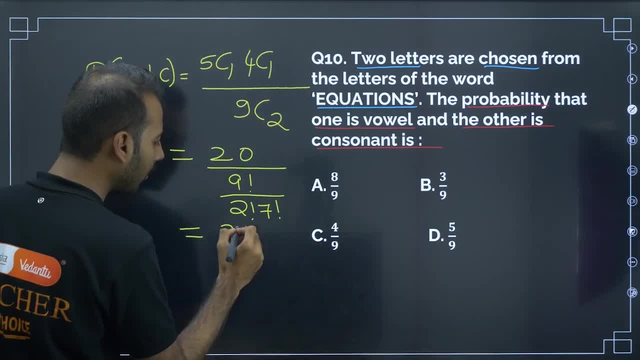 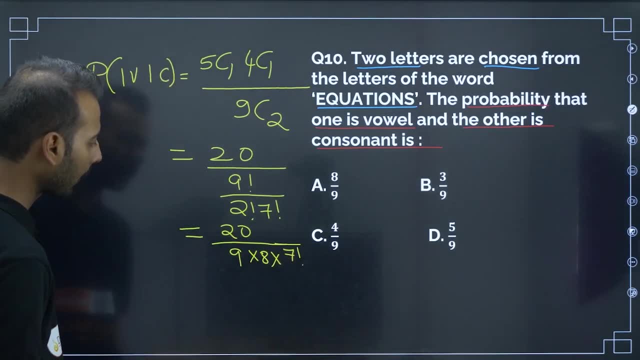 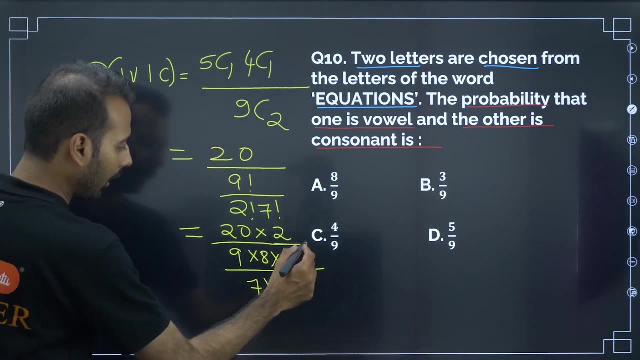 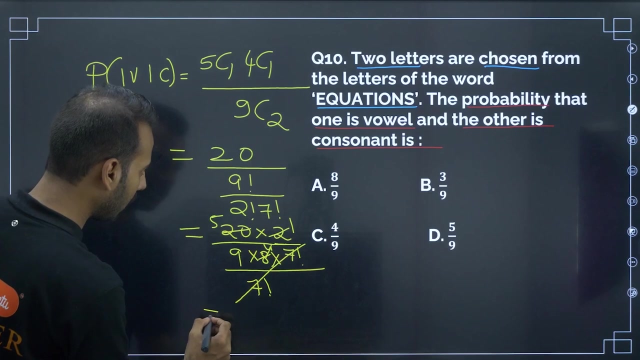 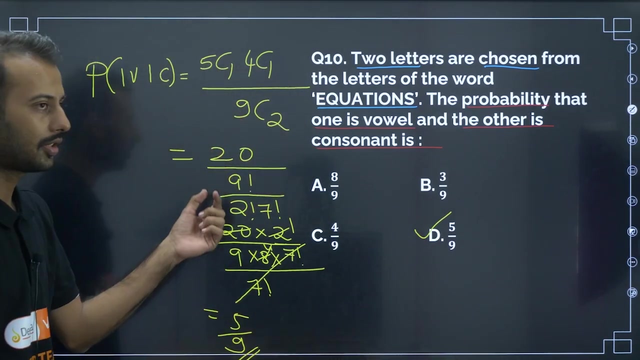 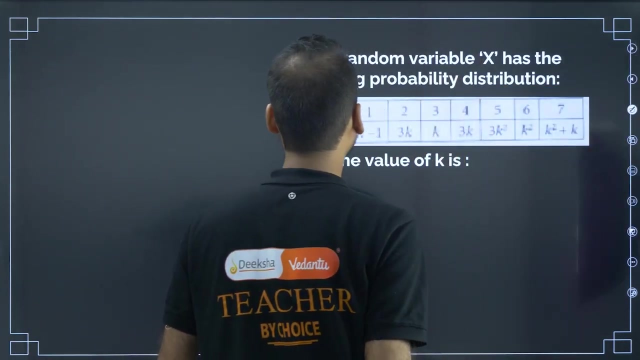 factorial, 7 factorial. so 20 divided by 9 into 8 into 7 factorial by 7 factorial into 2 factorial into 2. i am writing here: let me cancel this and this one: za. this is 4 za. so 20, this is 5, 4. so here we are left with 5 by 9. just simplification, i am leaving it to you. so d is the answer. again, this is a very easy question and less time consuming. within 20 seconds we are able to calculate this. moving on to next problem, the random variable. 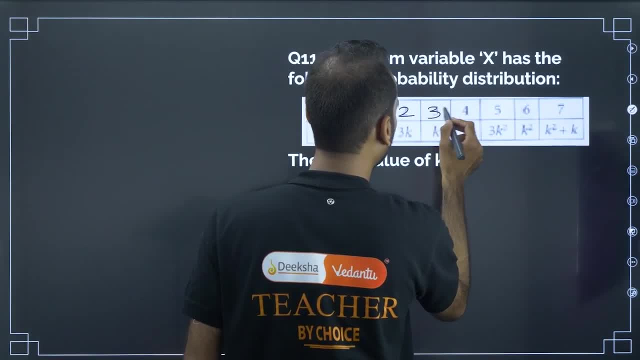 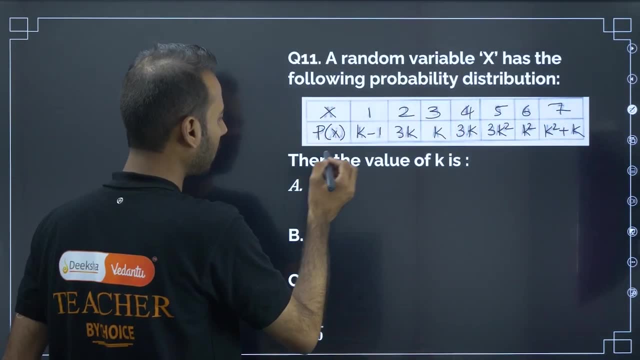 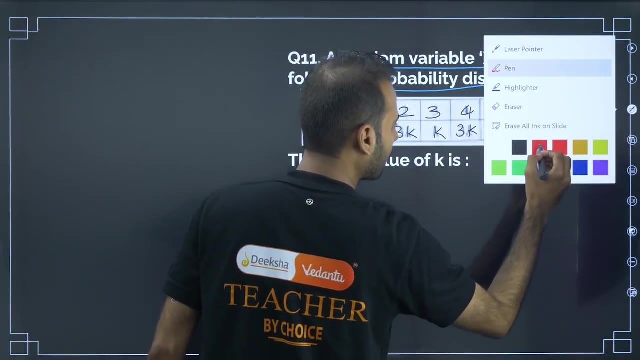 so they are talking about one random variable. one random variable, variable x, has the following probability distribution: then the value of k is a random variable. x has following probability distribution. then what are they asking? they are asking to find the value of k. So how to find the value of k for this one? 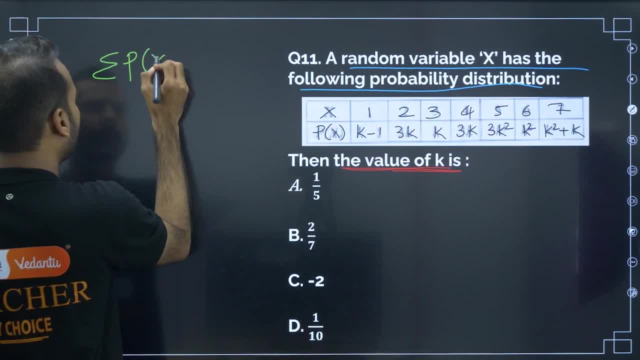 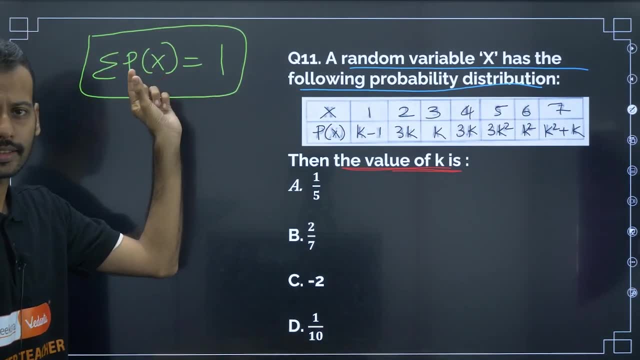 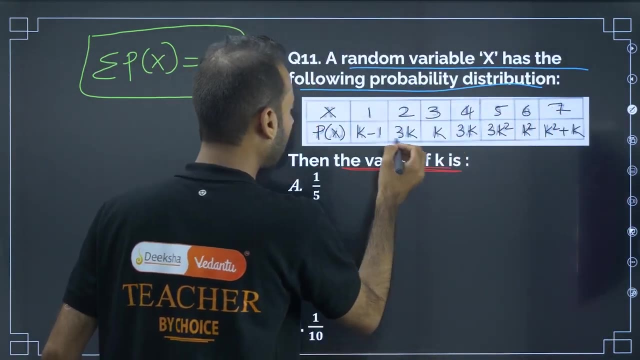 synopsis point: just now I have explained p of x. summation of p of x is equal to 1.. So, if you know this synopsis, only one, only one statement, one equation. if you know this problem is done. So how to use this problem? how to use this equation now? if you observe k, 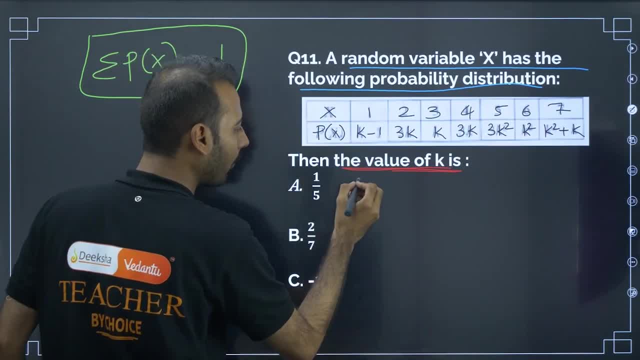 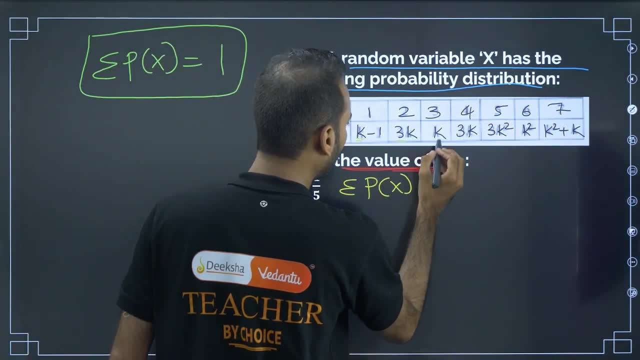 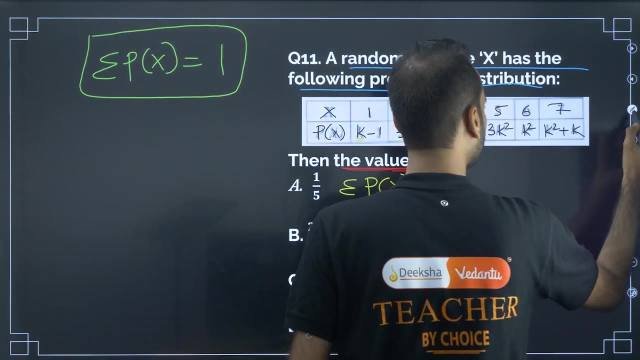 minus 1. if I add all this summation, if I do summation of p of x, summation of p of x is equal to k. Now, if I add all this, k, 4, 5, 5, 3, 3, 4, 5, 3, 9. 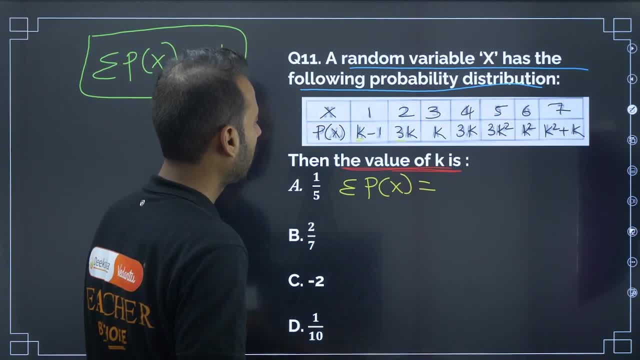 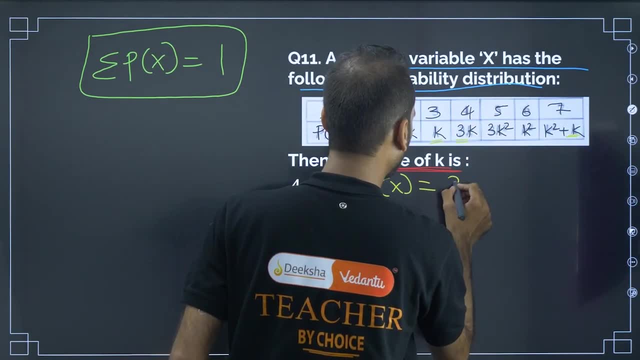 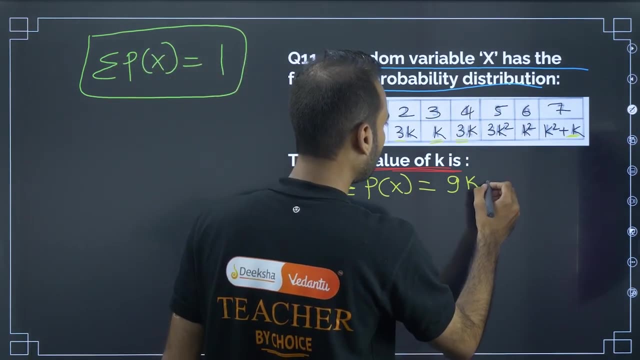 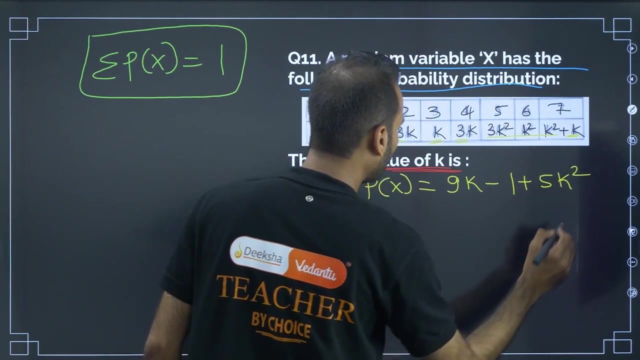 3, 4, 5, 3, 9, 4, 3, 3, 3 and 3 and this 3.. So total 9 k. total 9 k. just I am doing summation. next minus 1, I am keeping minus 1, only minus 1, 3 k k square, 5 k square, totally 5 k square. So p summation. 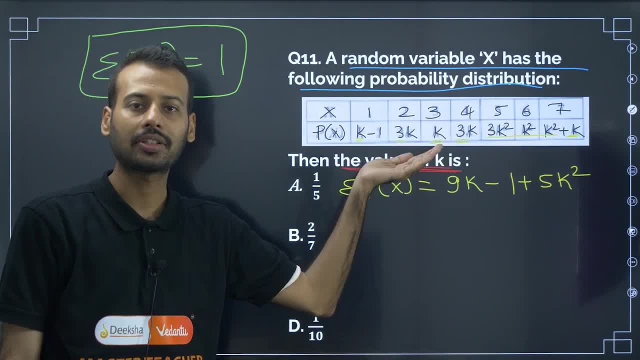 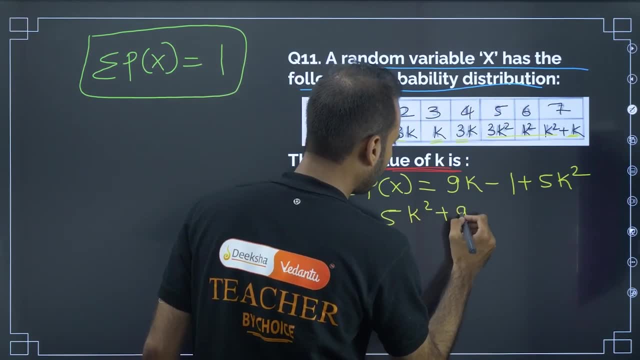 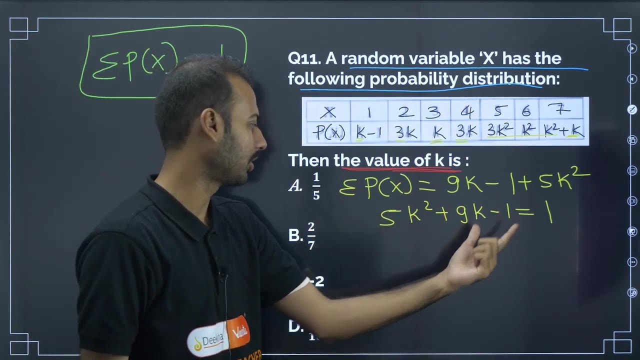 p of x is equal. to just add this addition and subtraction of terms they will teach in 7th standard, 8th standard, So next: So 5 k square plus 9, k minus 1 is equal to 1. I am just placing summation of p of x is: 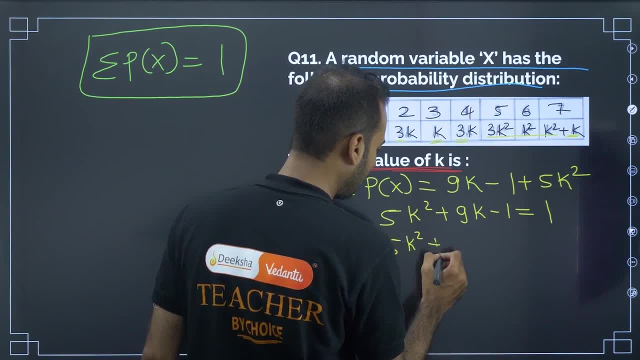 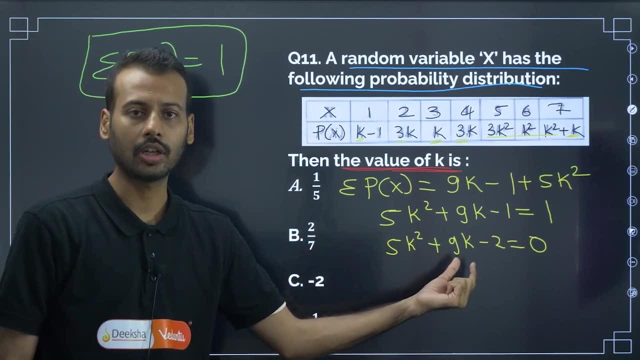 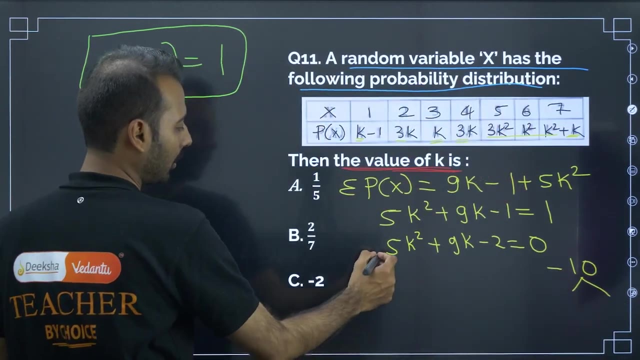 equal to 1.. So 5 k square plus 9 k minus 2 is equal to 0. this is the quadratic equation. Now we have to find 2 roots. what are the 2 roots minus 10? minus 10 for this, this and. 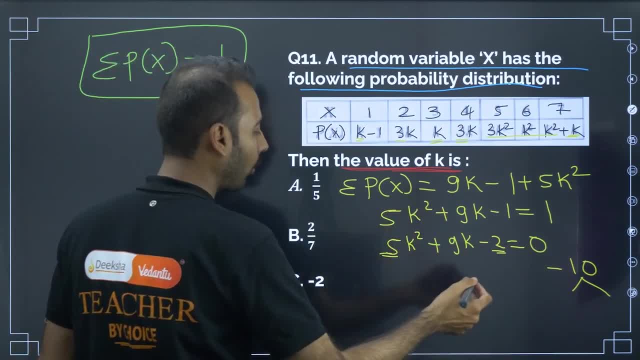 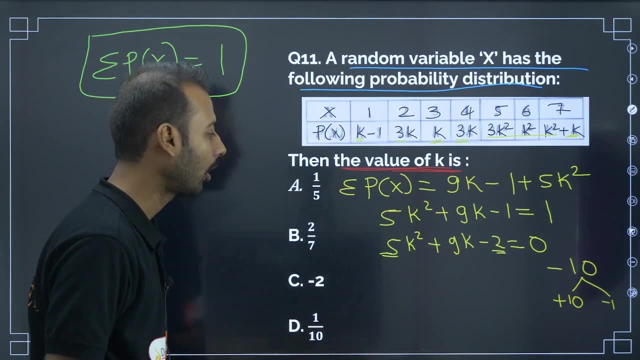 this: you have to multiply, You will get minus 10, and then for this minus 10, I will write minus 10 ones, or else 10 into minus 1.. So that I will get k. now what I have to do to find. I have to change its sign, change its. 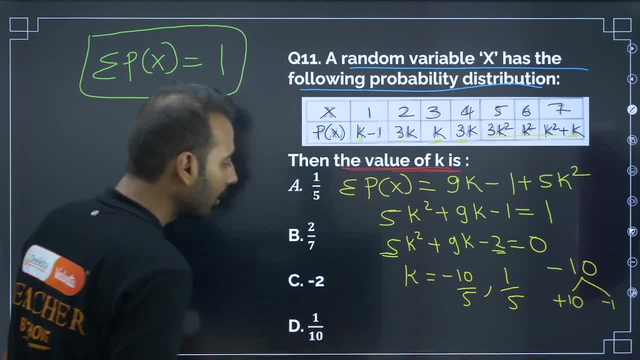 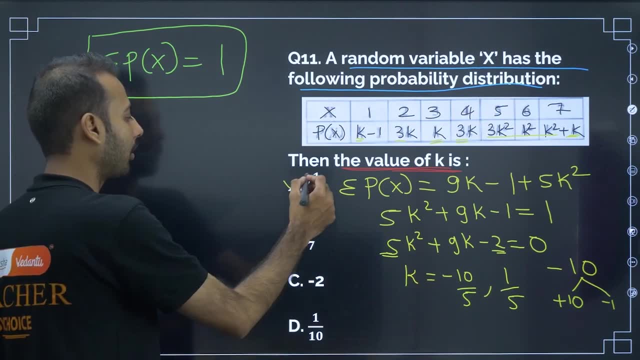 sign and divide by this. So change its sign and divide: k is equal to minus 10 by 5, 1 by 5.. So is there any such option? 1 by 5? yes, a is the answer for this. So only one synopsis. 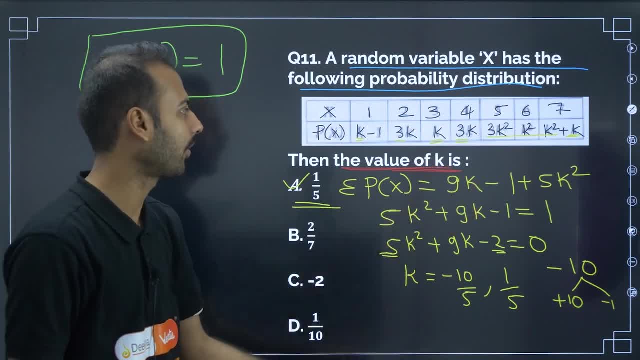 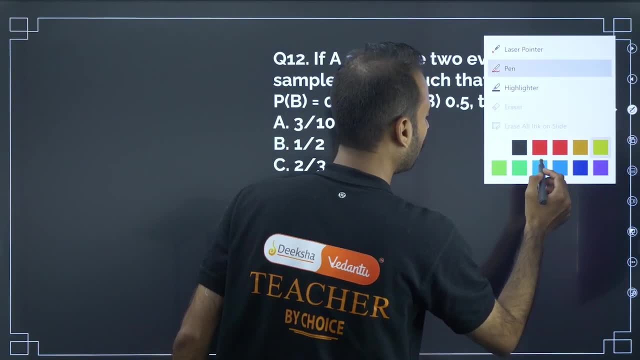 point. If you know. So this calculation will take 10 or 15 seconds, So within 15 seconds you are getting moving on to next. If a and b are events of a sample space, So if you go through this question, a and b are: 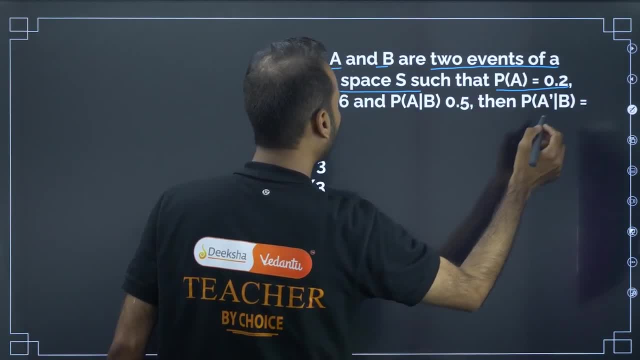 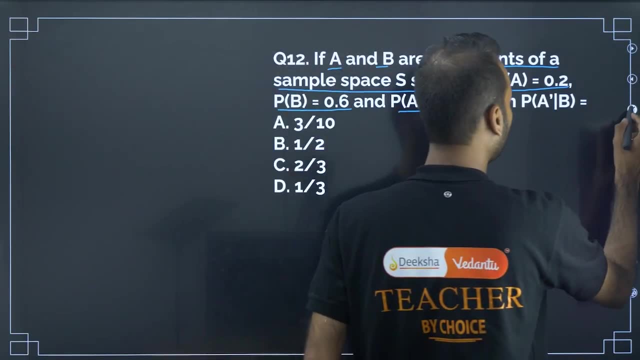 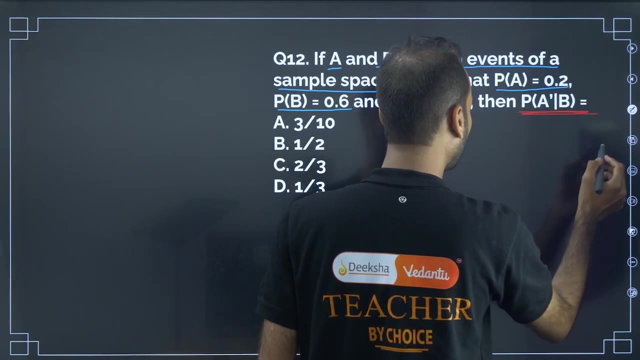 two events of a sample space. yes, p of a is this much. p of b is this much? p of a given b is this much, then? p of a dash given b is what? p of a dash given b is what. how to approach this problem: See here. 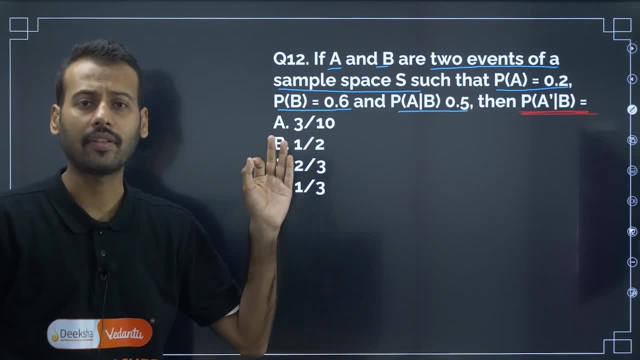 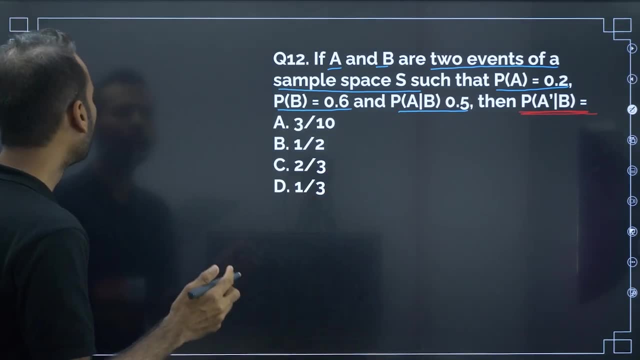 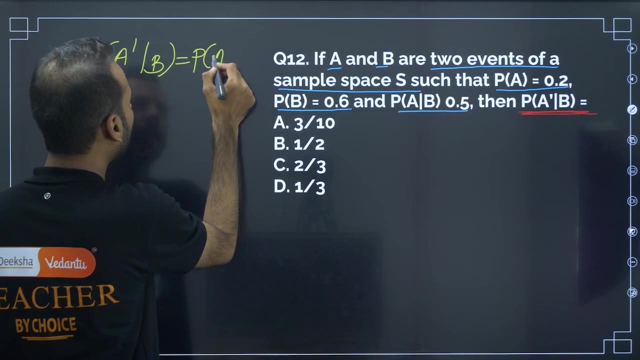 So what we are saying is: So this condition- conditional probability- very, very, very important topic: conditional probability. please go through the synopsis. If you do not know synopsis, if you know a synopsis, then it is a good thing. Now, probability of a dash given b is equal to probability of a dash and b divided by 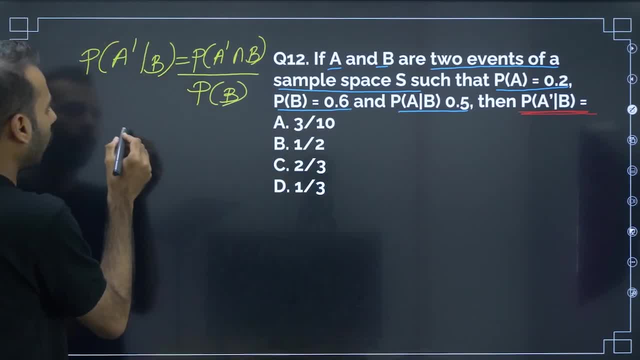 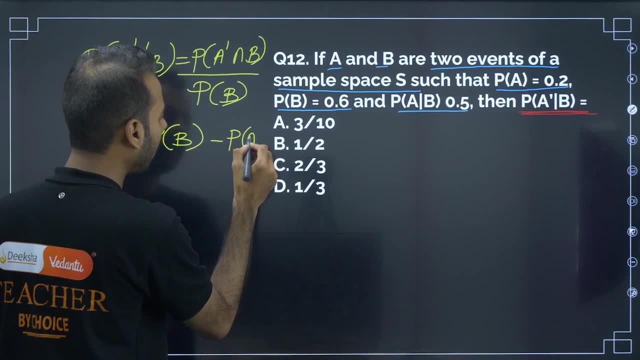 probability of b. So probability of b is 0.6.. Probability of a dash given b is equal to probability of b given Okay. probability of A minus probability of A and B. A and B divided by probability of B: probability. 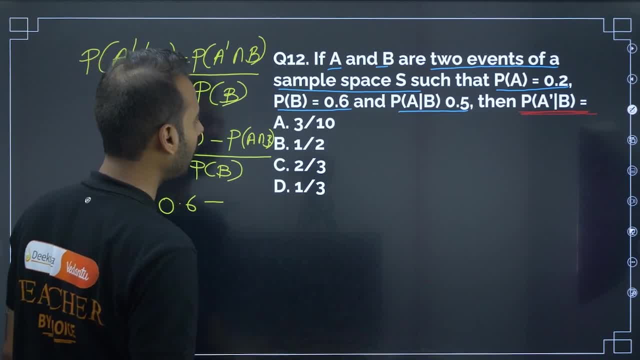 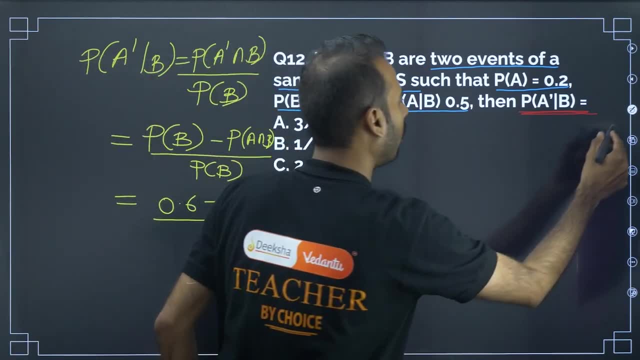 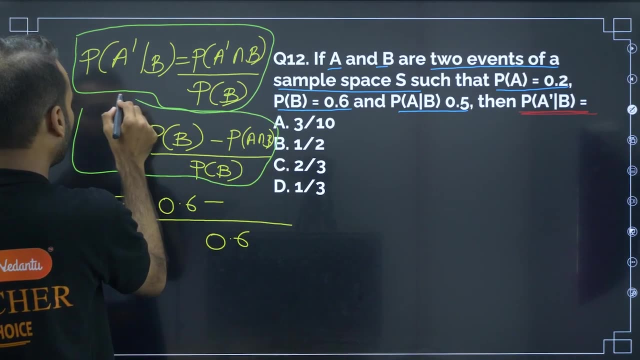 of B is 0.6 minus A intersection B, so probability of B is 0.6,. what about probability of A and B? now, all these are synopsis points. so you consider this much as synopsis, this also you consider as synopsis, so this is a part of synopsis. now, further, we want probability. 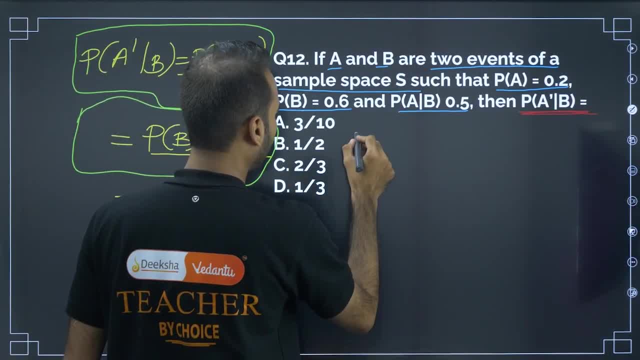 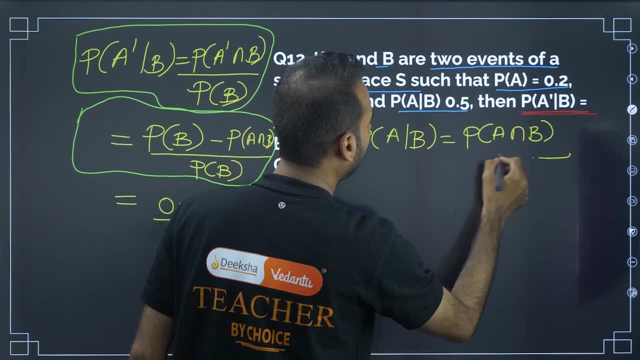 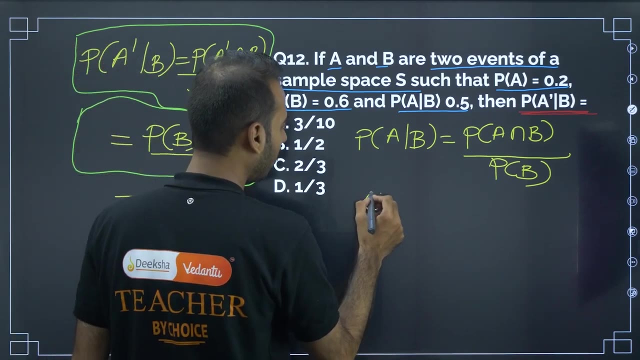 of A intersection B. so how to find A intersection B. probability of A given B is equal to probability of A intersection B divided by probability of B. probability of A given B is 0.5,. probability of B is 0.6 is equal to. 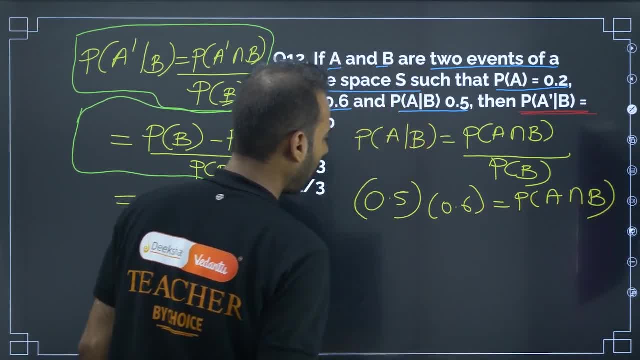 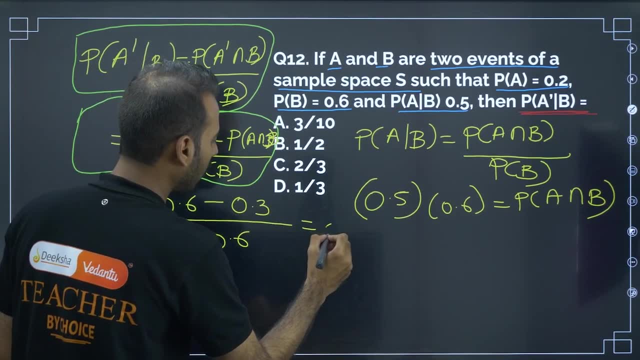 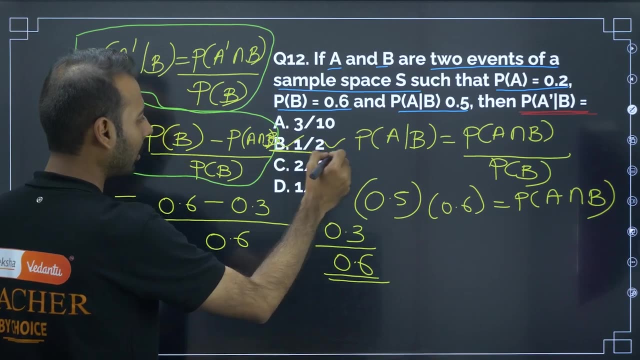 So probability of A intersection B. so probability of A intersection B is 0.3,. so 0.6 minus 0.3 divided by 0.6, which is equal to 1 by 2, so the answer for this is 1 by 2.. 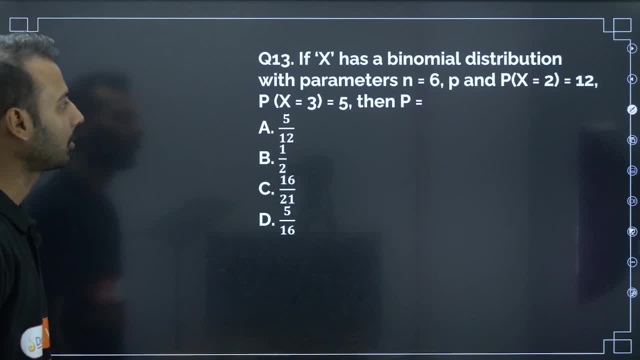 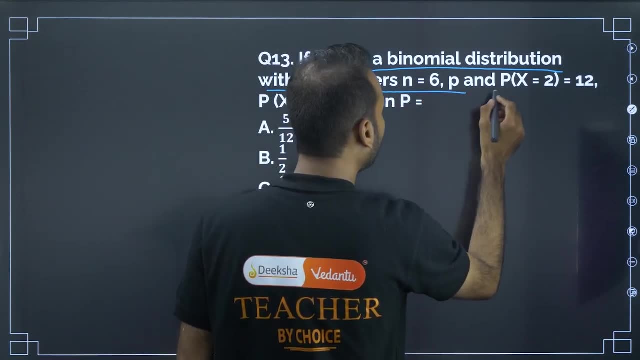 Moving on to next question, if x has a binomial distribution with parameters, so some information they have given x as a binomial distribution with parameters, parameters and p of x is equal to this much and p of x, then p is equal to the question. 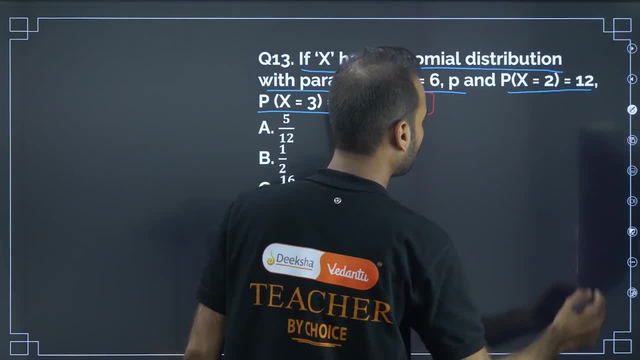 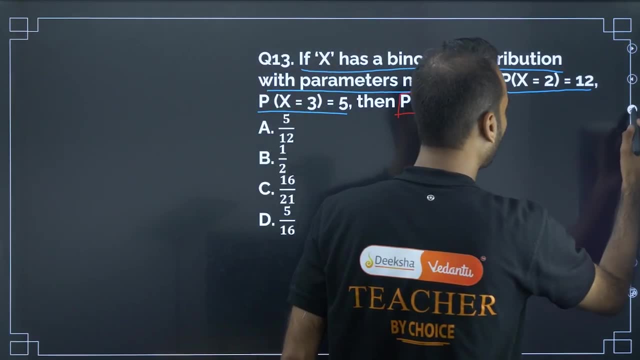 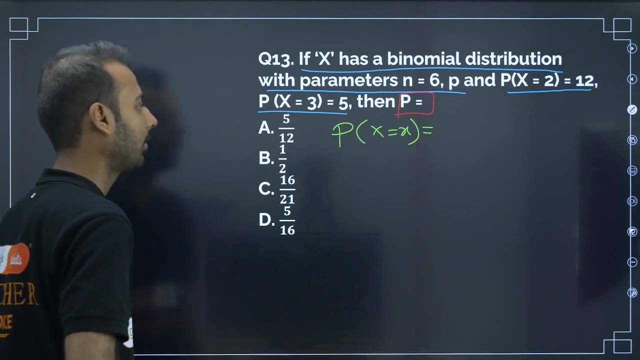 they are asking, p is equal to now in this question. in this question, then, p is equal to now. try to recall one synopsis point. what is that synopsis point related to Bernoulli trials? x is equal to x. probability of x is equal to x, n, c, x, n, c, x. probability of x is: 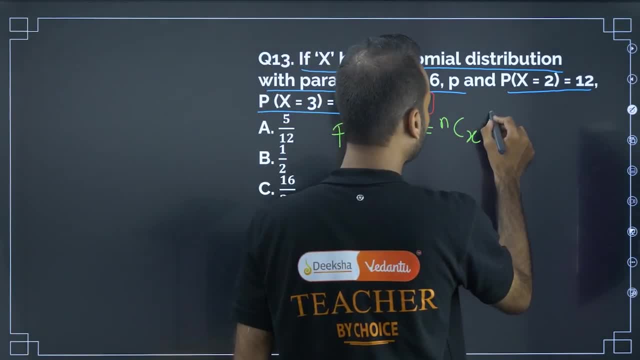 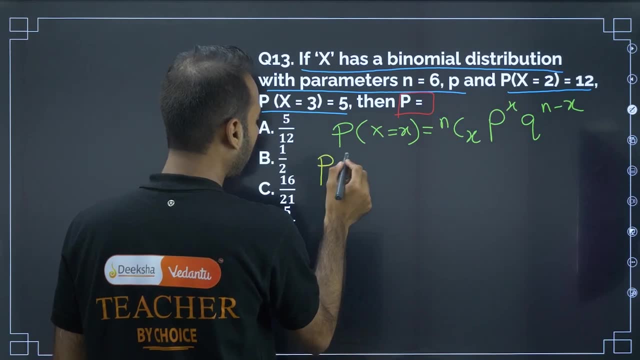 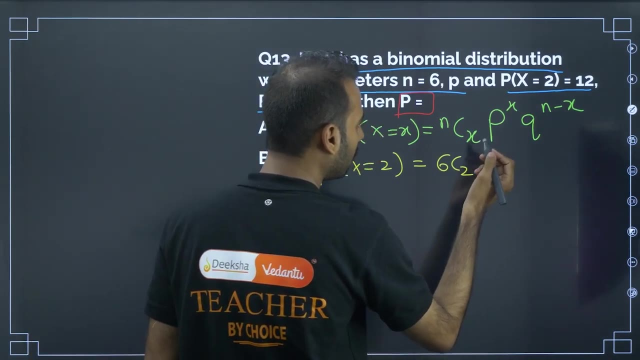 equal to x, n, c, x, p. raise to x, q. raise to n minus x. the synopsis point. try to recall Now: probability of x is equal to 2, is equal to 6 c, 2, 6 c, 2, p, p. raise to n minus x. 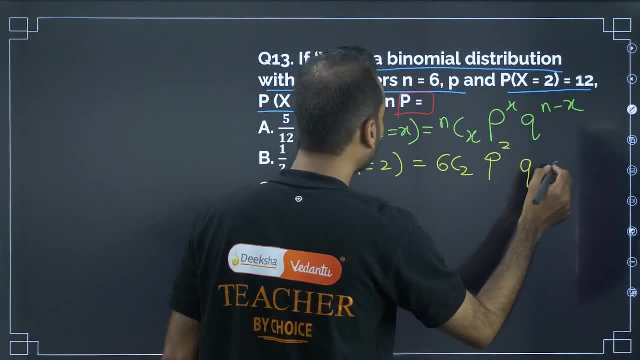 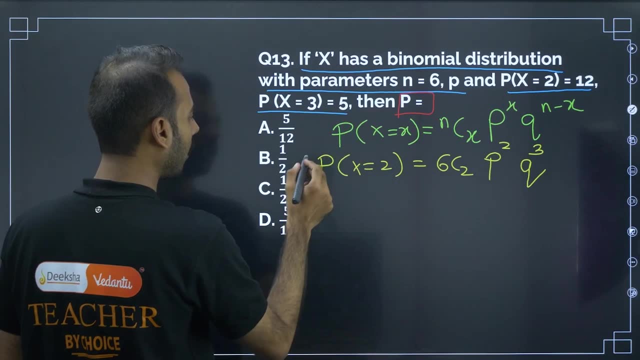 So this is the one we are looking for. This is the one we are looking for. So this is: in place of x, we are keeping 2, in place of q. q. n minus 3 is 3.. So this p value also. 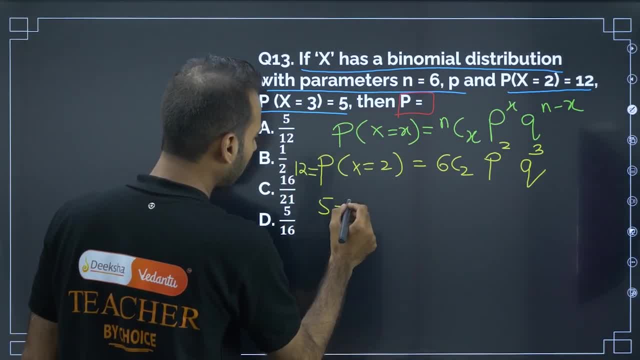 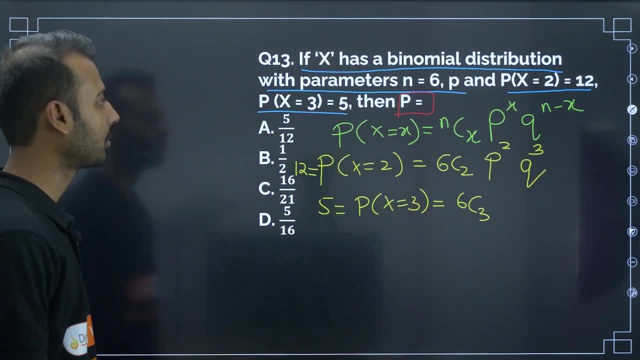 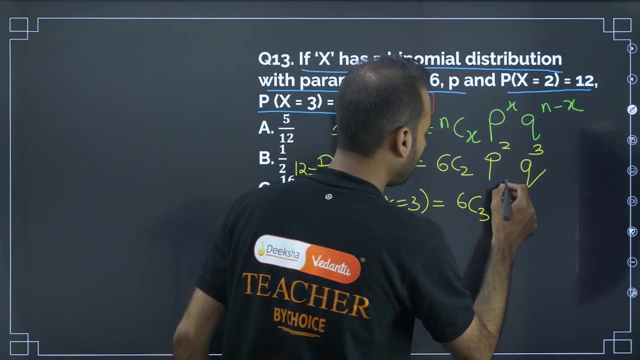 they have given this as to. well, next, phi is equal to p of. x is equal to 3, is equal to 6 c. 3 is equal to 6 c 3 p. p raise to x, x value is 3, q value is, So this is also. 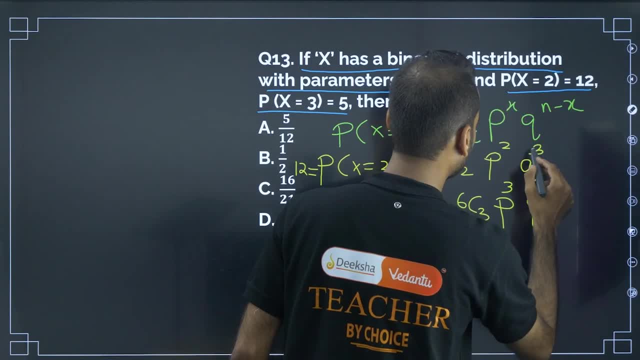 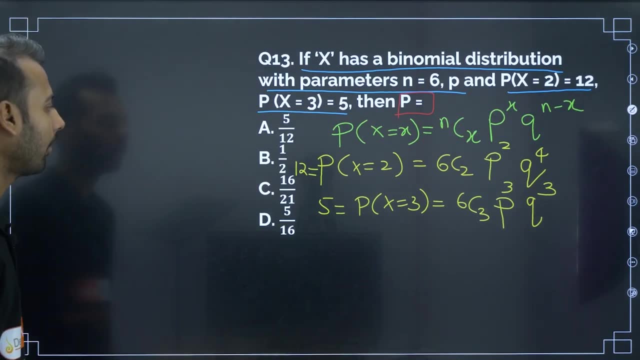 3 n minus x. I think it should be 4, n minus x, n minus 2 is 4.. Now everything is fine. So 2 l by phi, go for dividing of this equation. then I will get 2 l divided by 2 l minus 2. 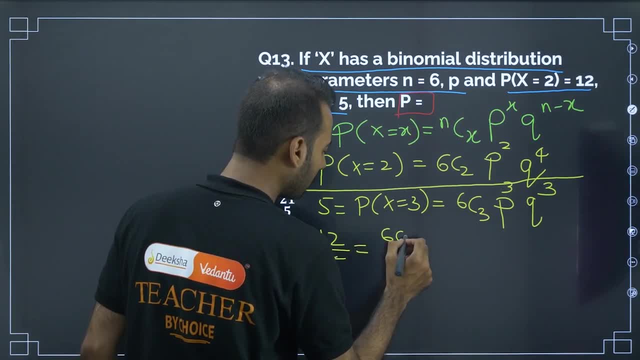 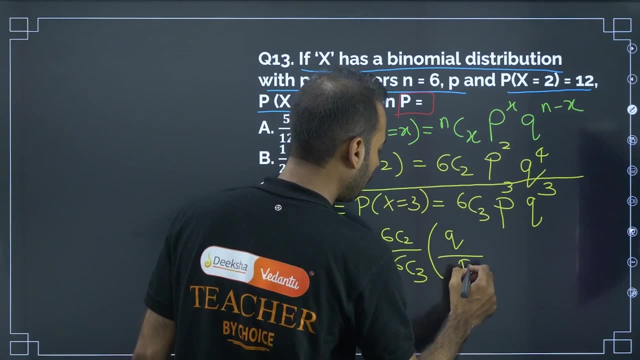 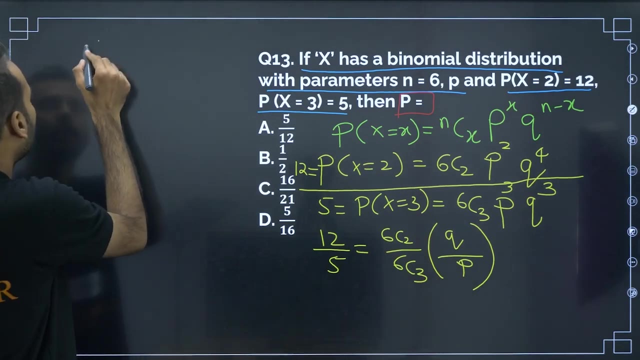 divided by 4 is equal to 6 c 2 divided by 6 c 3,. 6 c 2 divided by 6 c 3 q divided by p. So q divided by p. next, 6 c 2 value is 6 c 2 value is 6 factorial by 2 factorial. 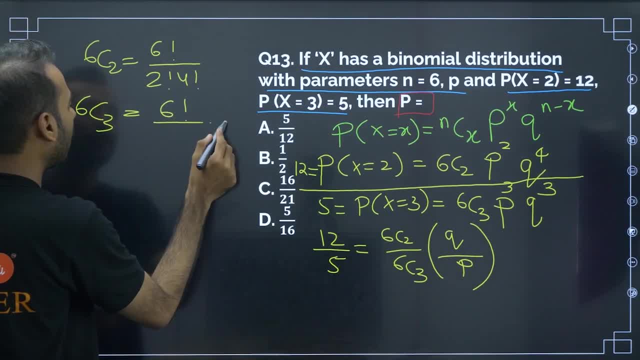 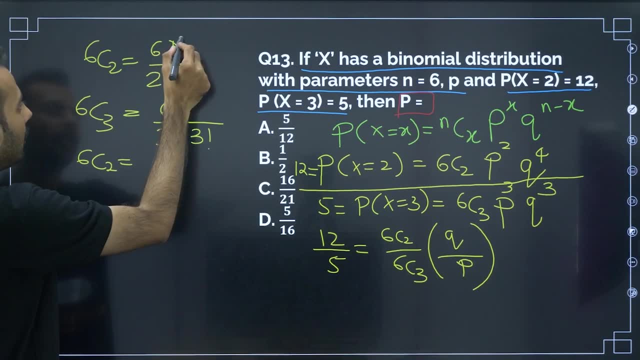 4 factorial 6 c. 3 is 6 factorial by 3 factorial, 3 factorial factorial. so 62 is equal to 6, 6 into 5 into 4 factorial, 4 factorial 4, 3, 5, 15, 63 is equal to. 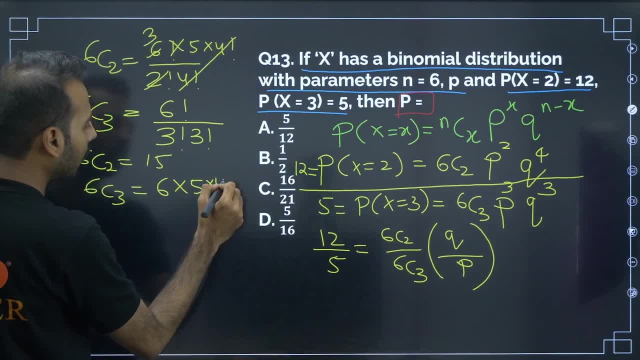 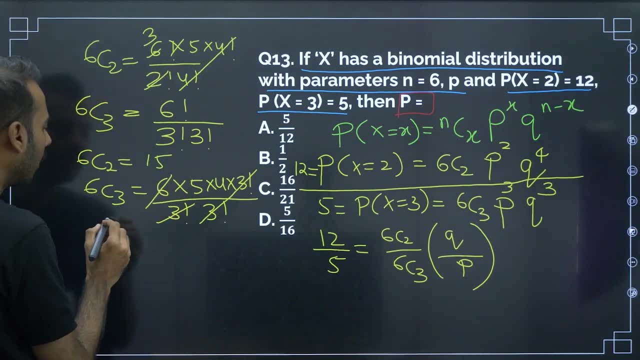 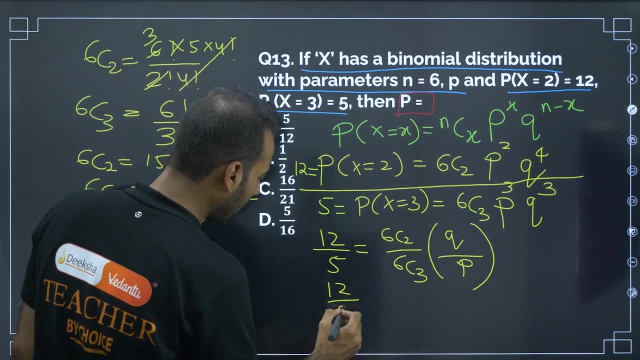 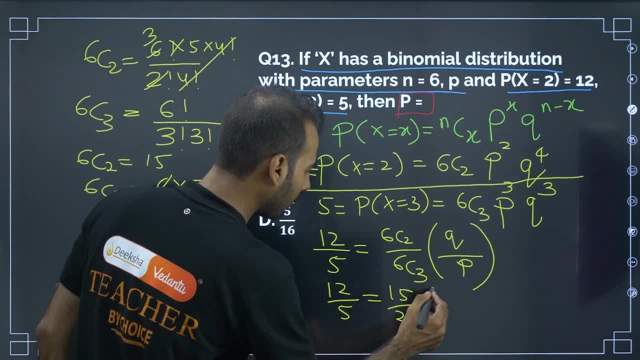 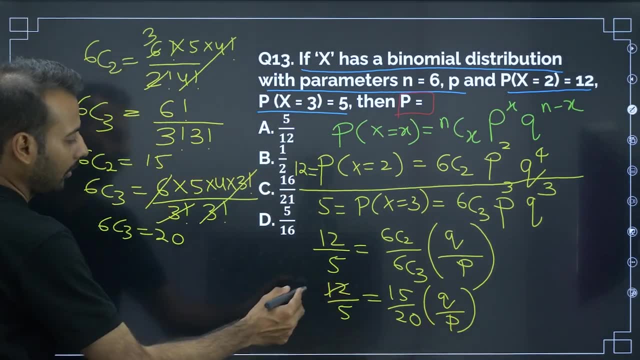 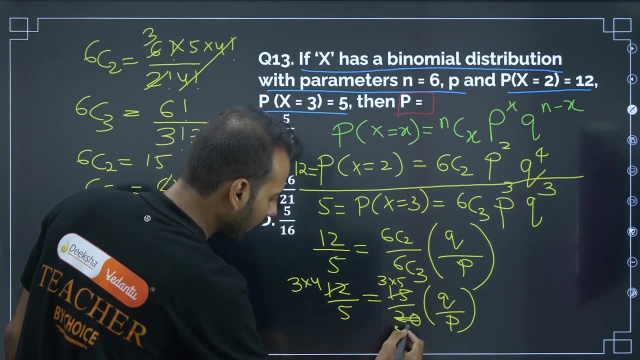 15 by 20, 15 by 20, q by p, q by p. so phi. this is: this can be written as 3 into 4, and here this side. this can be written as 3 into 5. here, 5. this can be written as 5. 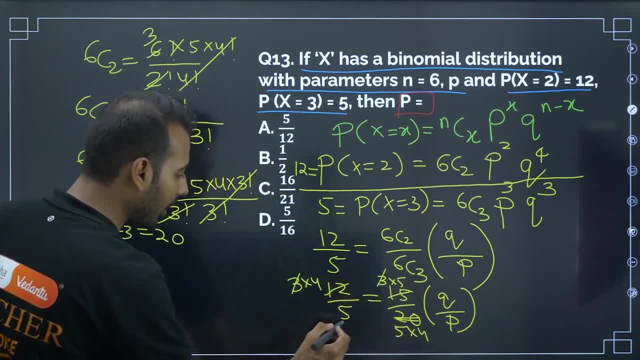 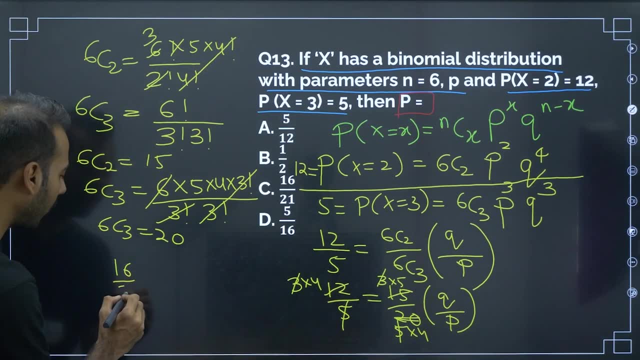 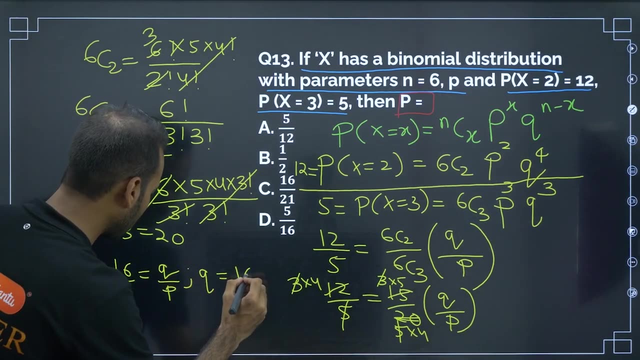 into 4. so if i cancel this 3 and this 3, if i cancel this 5 and this 5, so what i am left with here? i am left with: 16 divided by 5 is equal to q divided by p, which implies q is equal to 16 p. 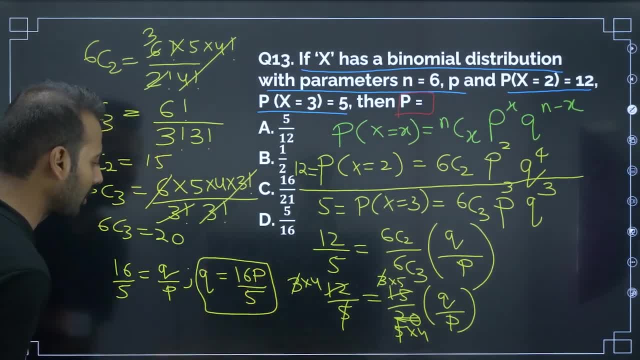 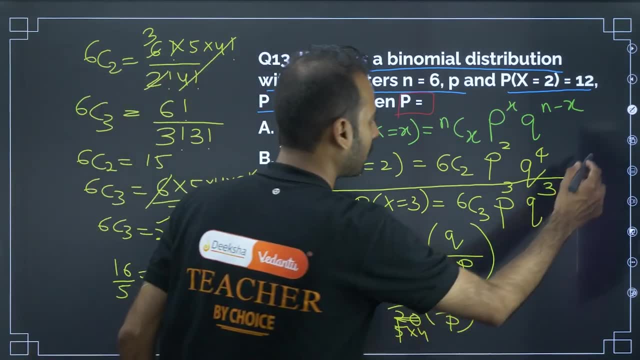 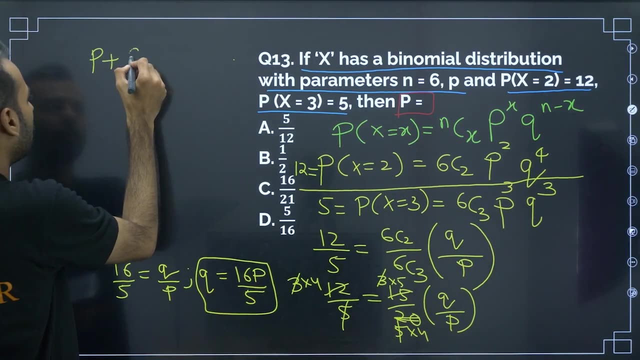 divided by 5, q is equal to 16 p divided by 5. if you want to make a note of this, you make a note of this. i am going to erase because of space constraint. moving on to next, q is equal to 16 p divided by 5. p plus q is equal to 1. this is a synopsis point, so in 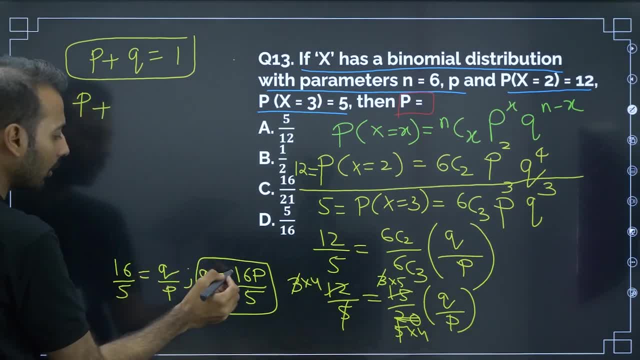 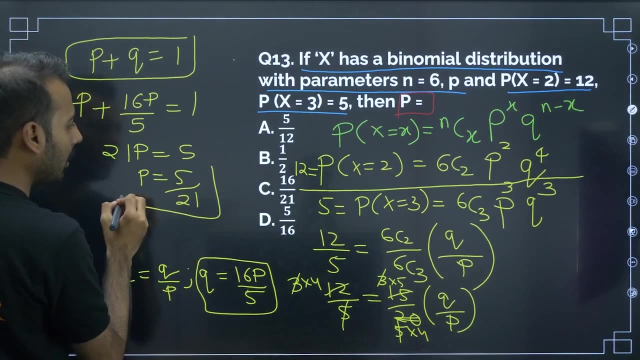 place of p. i am keeping p only in place of 16 q. i am writing: 16 p divided by 5 is equal to 1. if i take lcm 21, p is equal to 5. so p is equal to 5 divided by 21. is there any such option? p is equal. 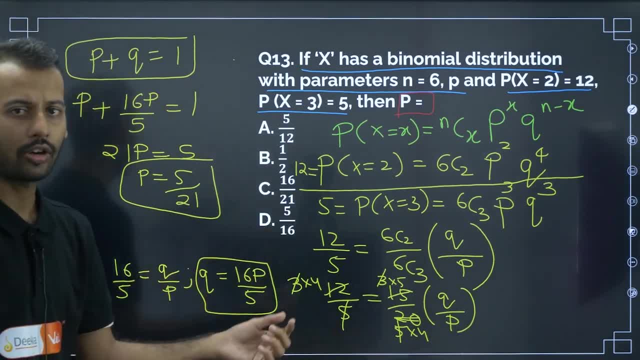 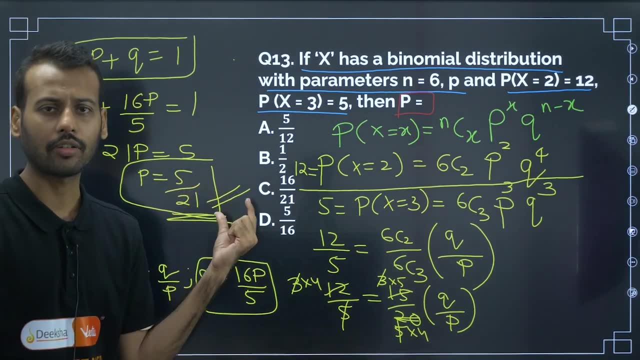 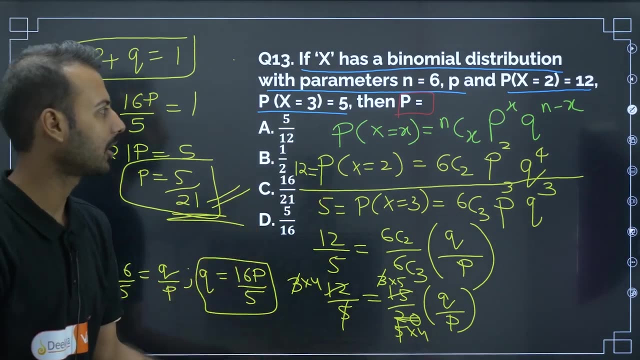 equal to 5 divided by 21.. This option is not there, So you can consider this as a grace marks. the correct answer for this is: P is equal to 5 by 21. is the correct answer in exam. If they have not given any options, you just take one option randomly. that will be considered as a 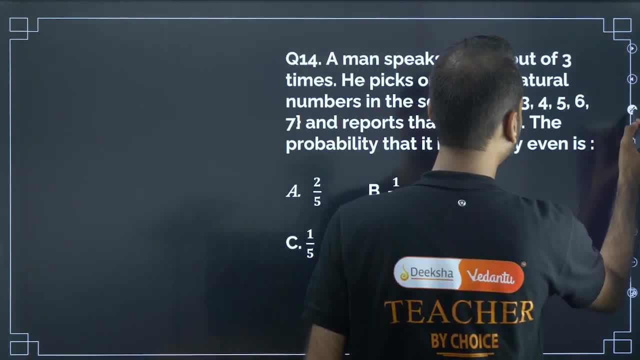 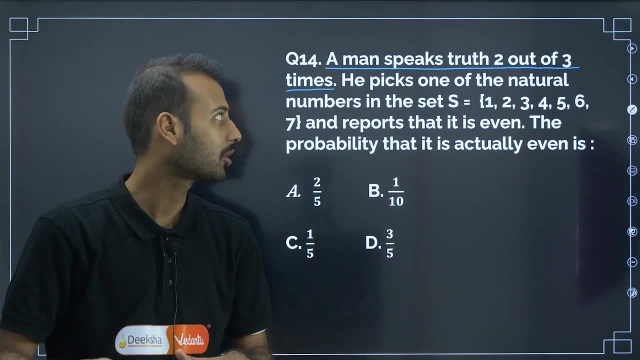 grace question. Moving on to next question, a man speaks truth 2 out of 3 times. There is one man he speaks truth 2 out of 3 times. That means sometimes he is lying 1 out of 3 times he is. 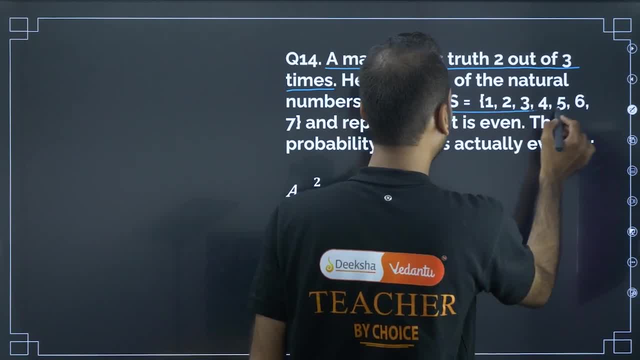 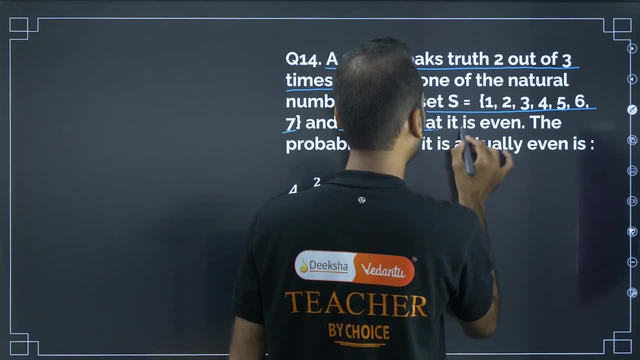 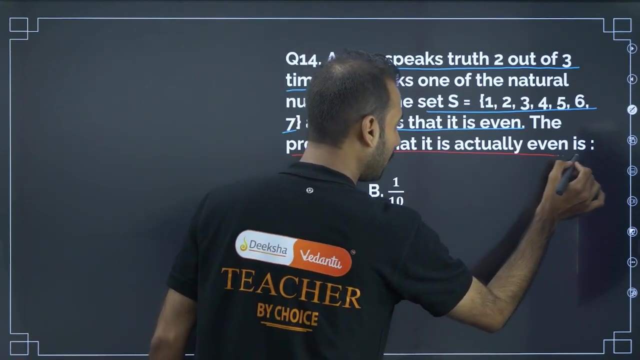 lying. He picks one of the natural numbers in the set. From the set he is picking one natural numbers and reports that it is even and report the probability and reports that it is even The probability. what is the question? The probability that is actually even is They. 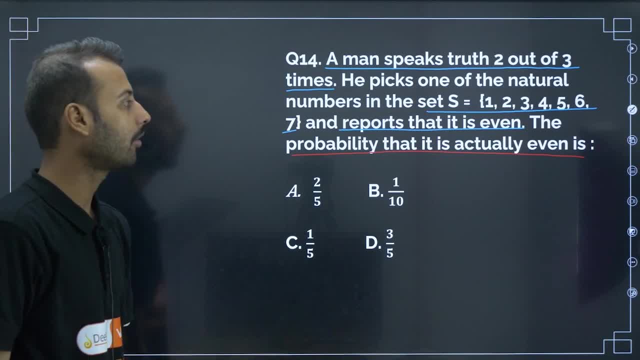 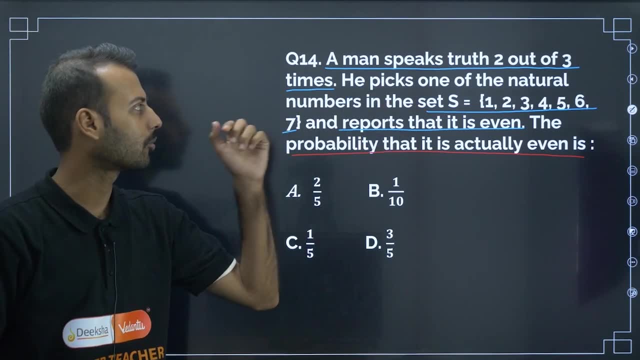 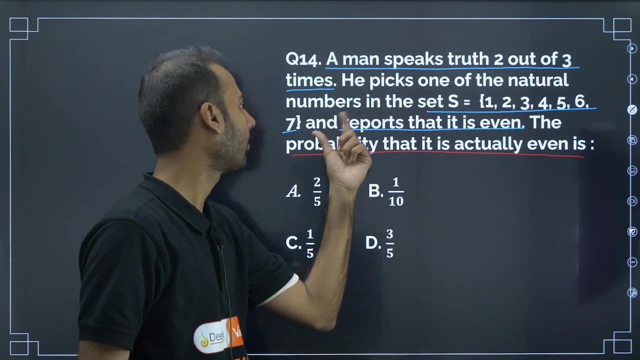 are asking: probability that it is actually even is. Now I will go through the question and I will try to extort some data. A man speaks truth 2 out of 3 times. He picks one of the natural numbers. So random experiment here is picking of natural numbers in the set. So probability of even number. 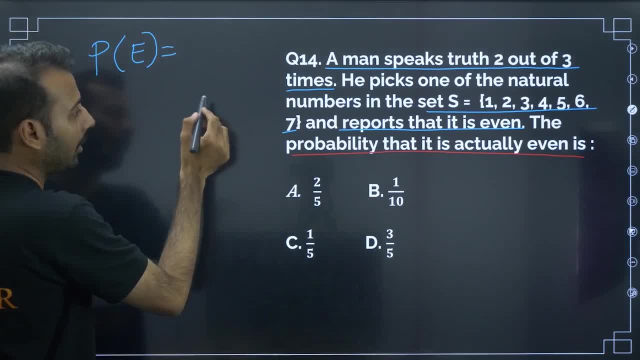 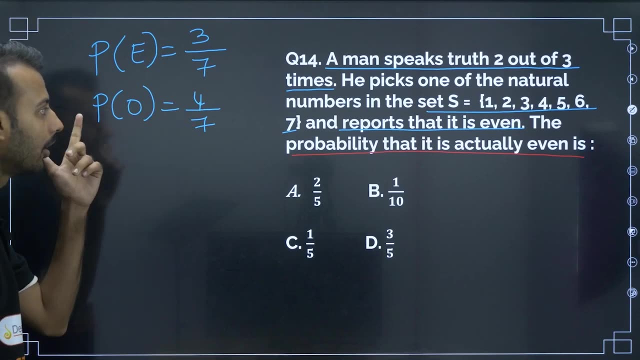 probability of even number is: how many even numbers are there? 3 even numbers are there? How many total Total 7 numbers? Probability of odd: How many odd numbers are there? 4 divided by total? So probability, this much of information I will get from here Next r be the event r be. 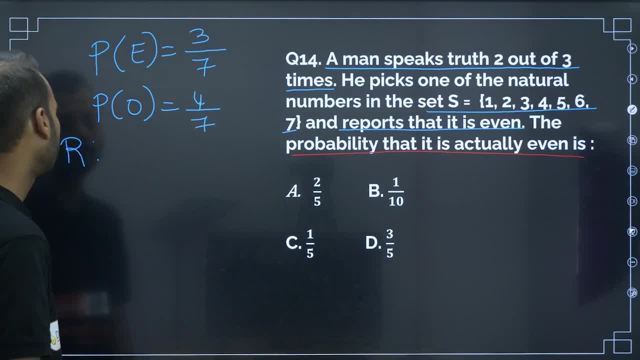 what The probability that it is actually even is. r is one event. What is this event Probability that actually even is Reports? r be the event that reports, even That man is reporting, even That event. let me name that as r. Let me name reports, even Reports, that it is even That event I am. 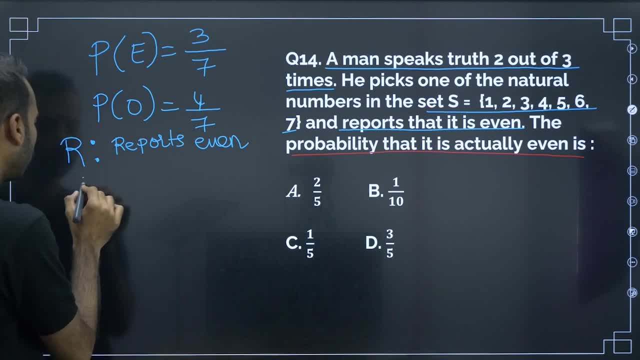 naming this as r. Now, if I go, if I try to understand this probability of reporting, even given that it is actually even is, Once again, I will go through the question, I will go through this Probability of reporting, even given it is even. So, that means it is truth Probability. 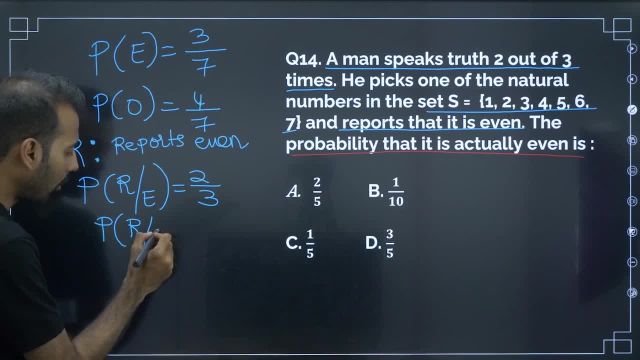 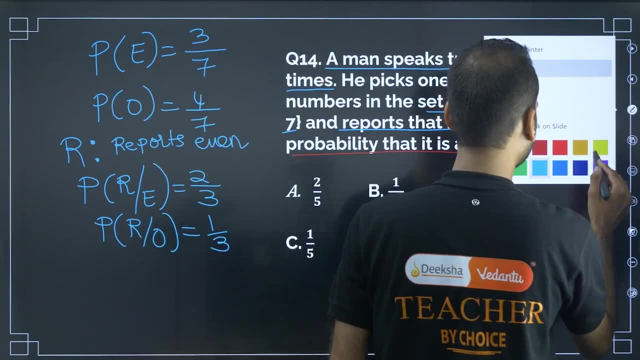 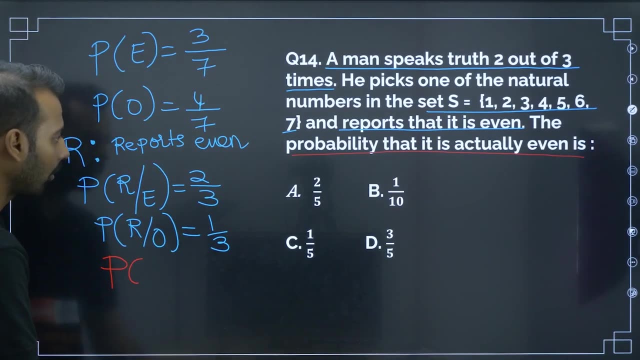 of reporting odd is Next, probability of reporting odd means he is false. Now what is the question? that actually even The question is: probability of the question is probability of actually even Reports, that it is even Actually even Reports. even The question is this: See here: 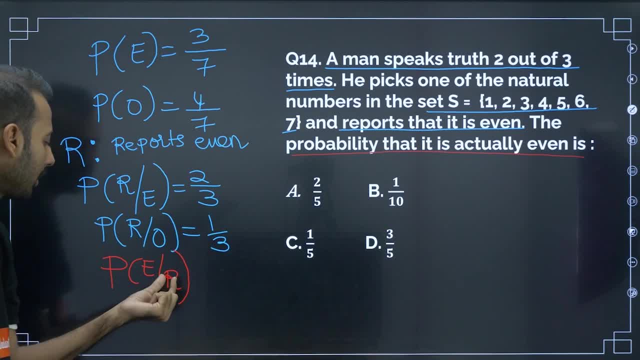 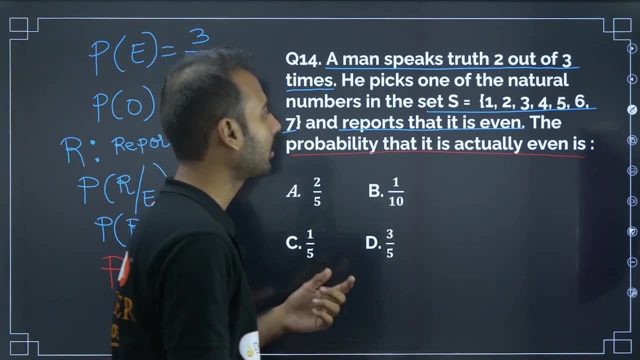 here the probability that it is actually even reports, that it is even given that reports, that is even So already is reporting even. the probability that it is actually even actually even given reporting even is Now with this information, if you go through this information, given data they are asking. 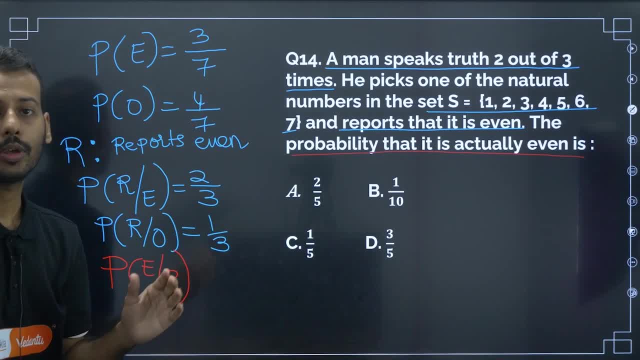 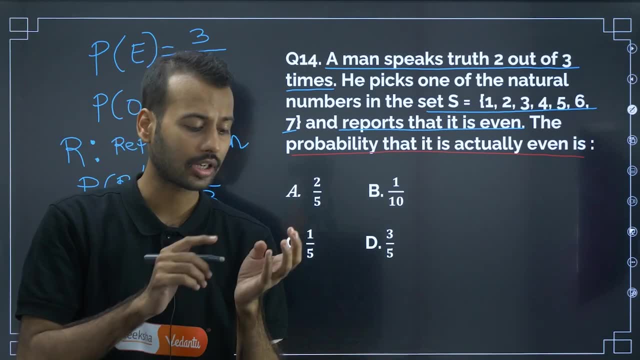 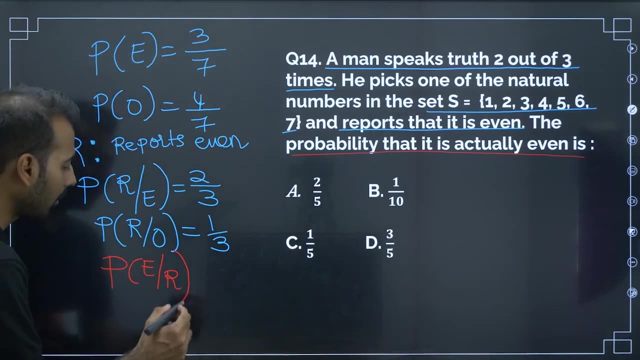 to find this Now, this data, you try to relate it with Bayes theorem. so Bayes theorem is very important. what all the important things? conditional probability, Bayes theorem, total theorem and Bernoulli trials. these are the most important. So probability of E given R for this formula is probability of R given E, R given E dot. 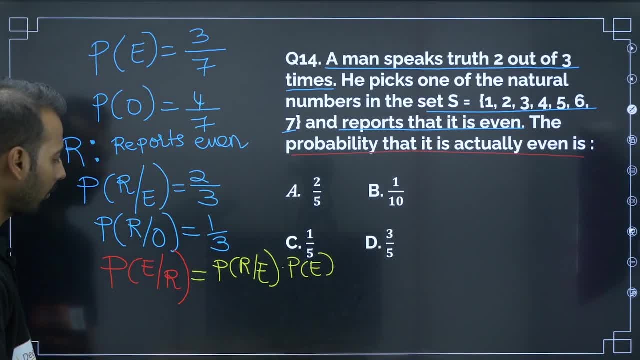 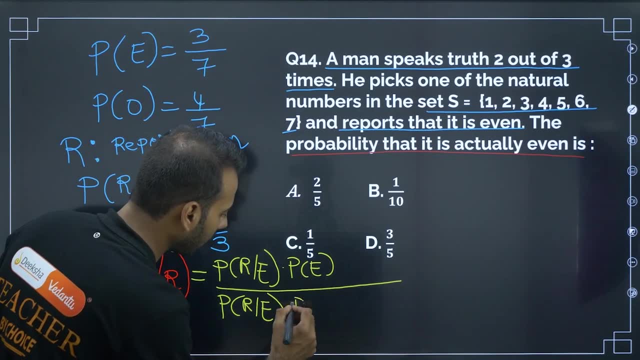 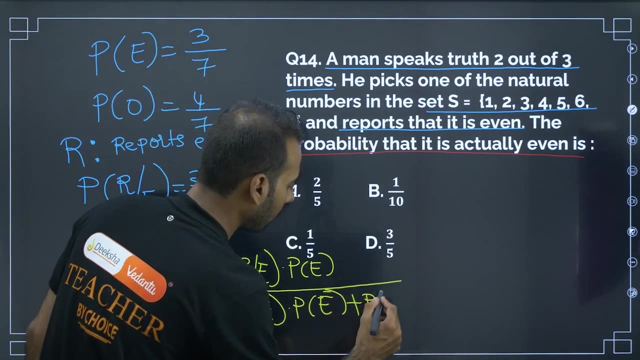 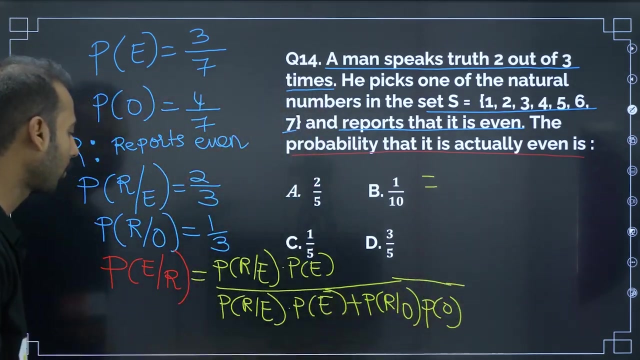 probability of E, Probability of R given E divided by probability of E. So R given E dot probability of E, plus probability of R given O, probability of R given O dot probability of O. So this is equal to R given E. from Bayes theorem, I am writing this: 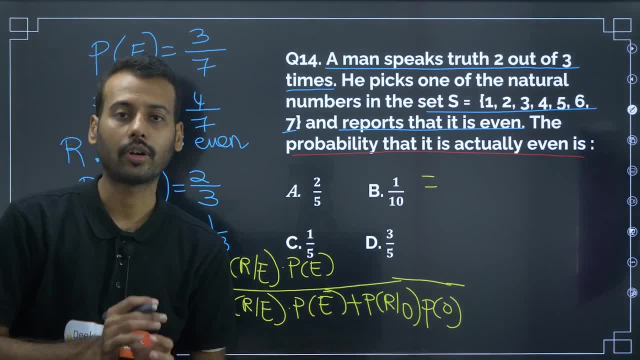 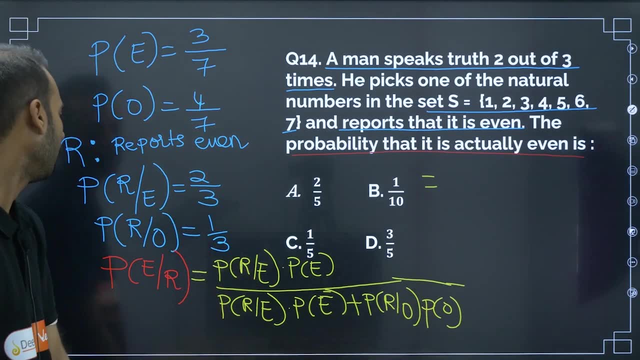 So this Bayes theorem, please, very important. I am saying, I am requesting you, Bayes theorem is very important in CET that will definitely come, So you please pay attention to it, Practice it. R given E. R given E is 2 by 3, 2 by 3. probability of E: 1 is 3 by 7, 3 by. 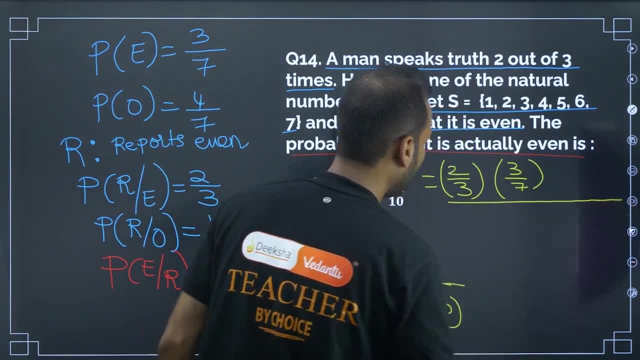 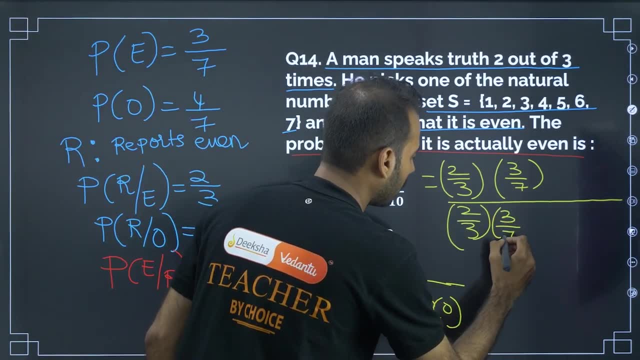 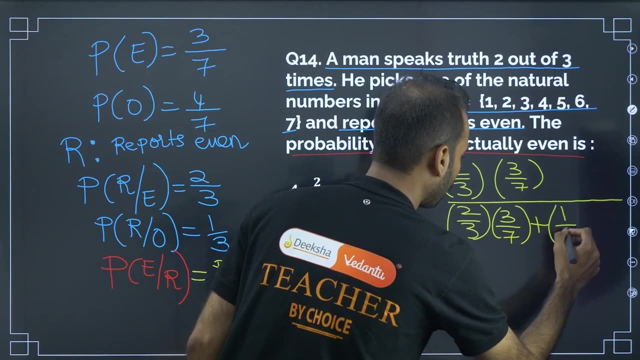 7, 3 by 7 divided by R given E, 2 by 3, 3 by 7, 3 by 7 plus R given O, R given O is 1 by 3, 1 by 3.. 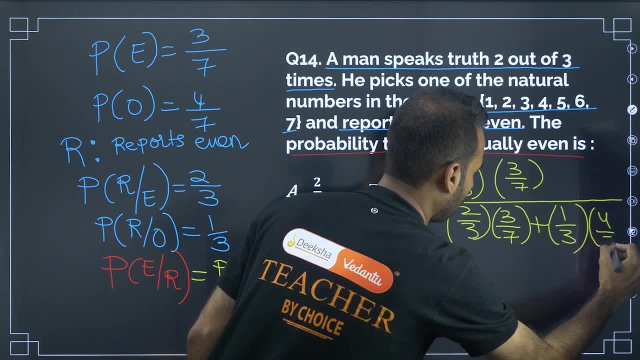 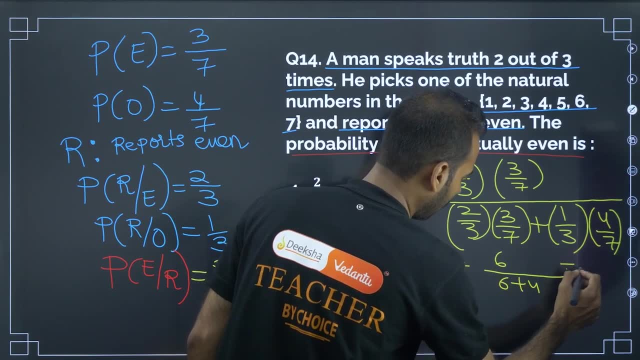 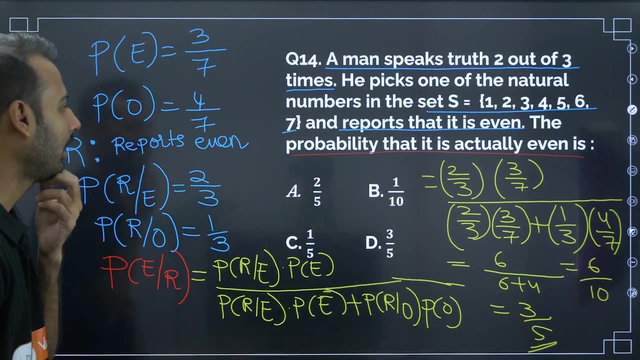 So probability of R 4 by 7,, 4 by 7 next. so if I calculate this, what I am left to 6 divided by 6 plus 4, 6 divided by 10,, 3 by 5,, 3 by 5, so is there any option like 3 by 5,? yes, 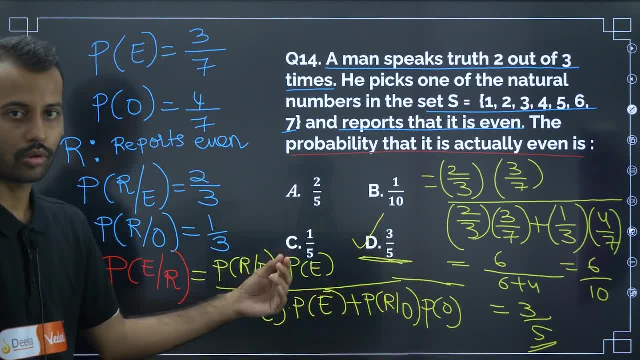 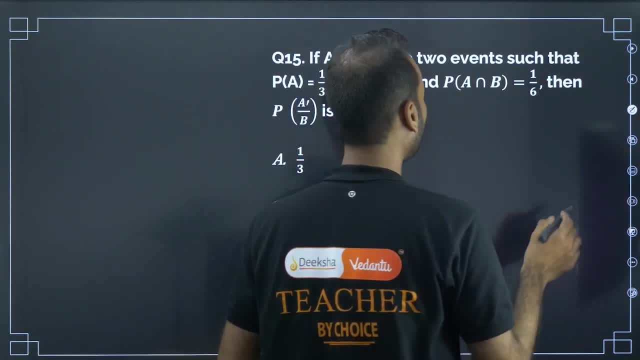 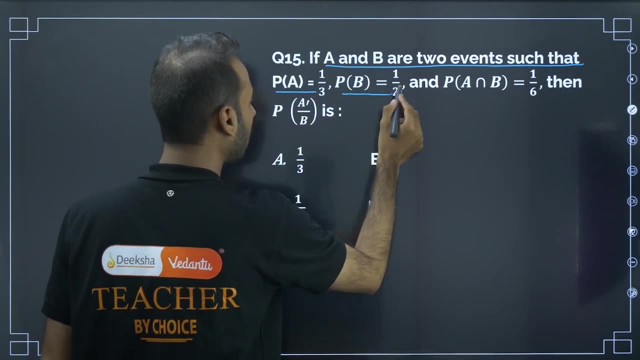 D is the answer for this? again, a easy question. if you know Bayes theorem, then it is easy. if you do not know Bayes theorem, then it will be tough. moving on to next question: If a and b are events, if a and b are two events such that p of a is this much p of 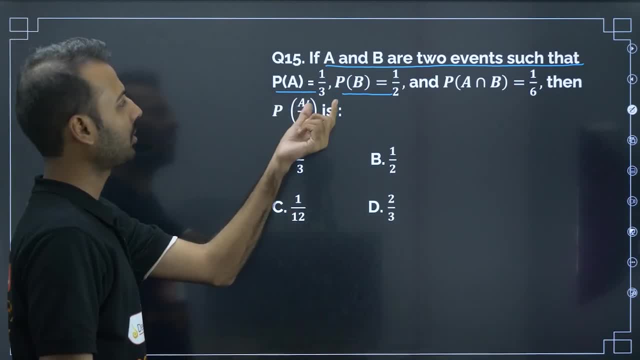 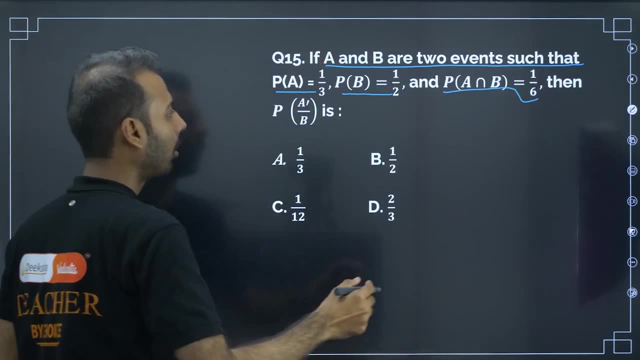 b is this much? If a and b are two events such that p of a is this much, p of b is this much and p of a and b is this much, then, p of a dash given, b is what is the question? p of a dash given. 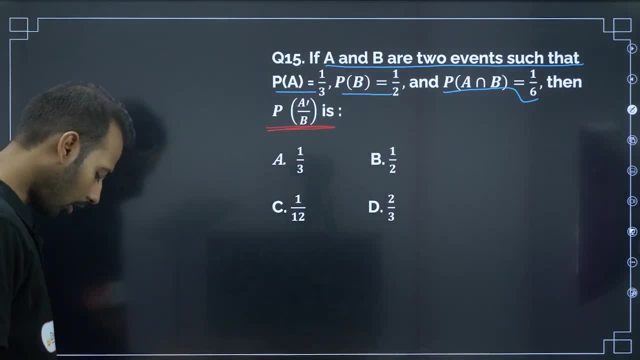 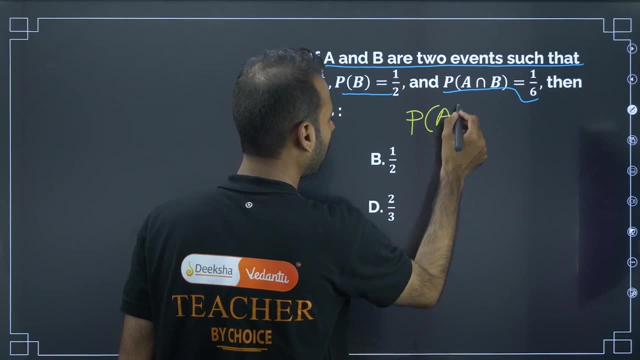 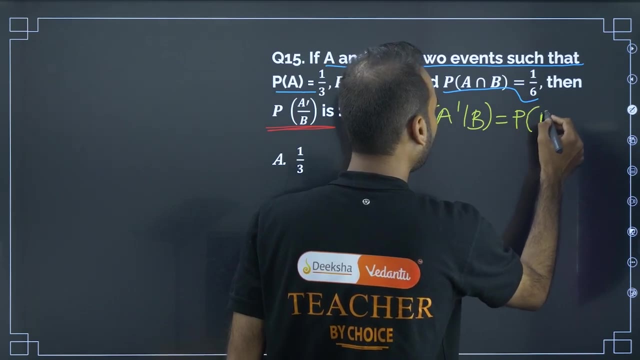 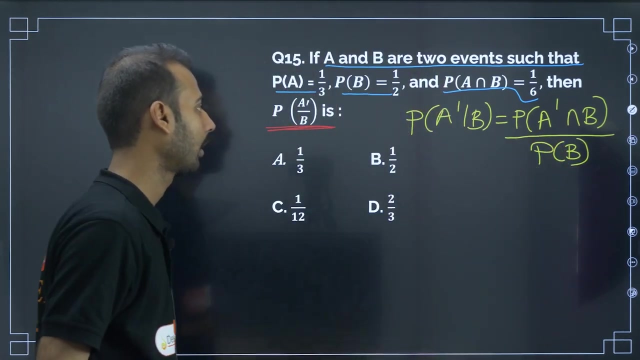 b is how much? So how to approach this? a dash given b, probability of A dash given B. Now, what is the formula to find? probability of A dash given B is probability of probability of A dash intersection B divided by probability of B A dash intersection B. This is synopsis. please add to your memory. please add to your. 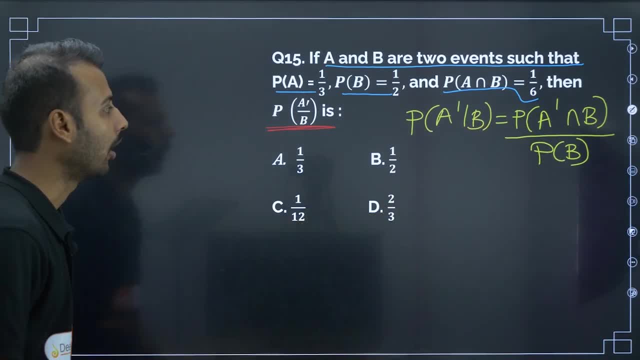 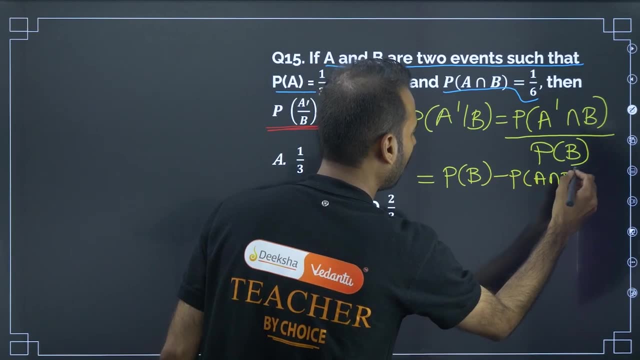 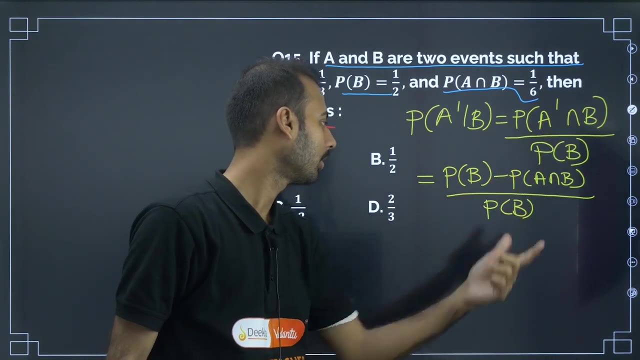 soul. this point is very important. A dash given B conditional probability. Now probability of this can be written as probability of B minus probability of A and B by probability of B. Again, this also from synopsis: A dash, intersection B is probability of B minus. 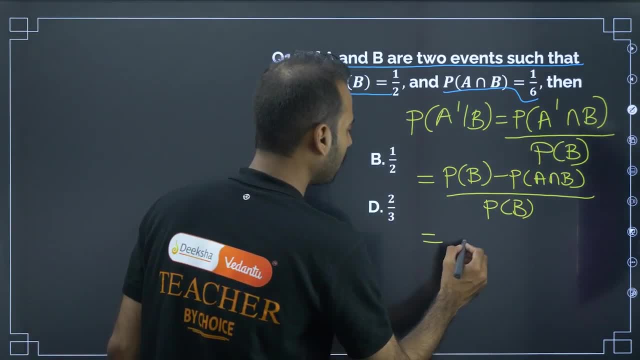 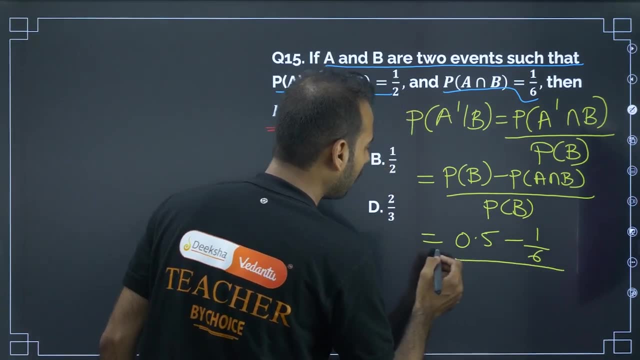 Next, probability of B is how much probability of B is 0.5? here it is given minus A intersection. B is 1 by 6. by probability of B is 1 by 2. let me erase this. let me erase this: 1 by 2. 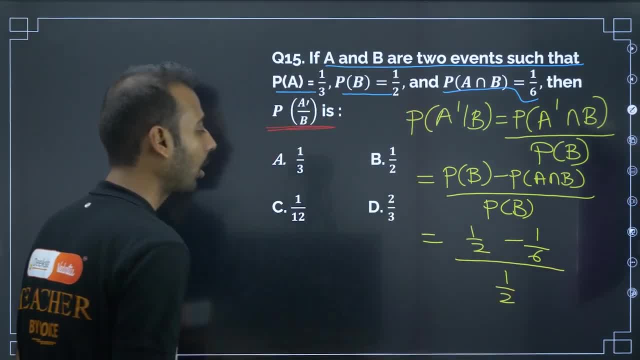 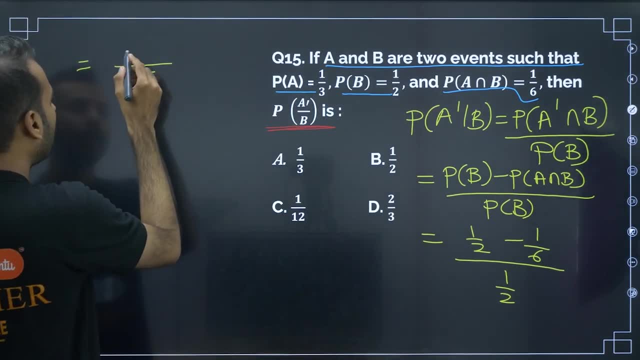 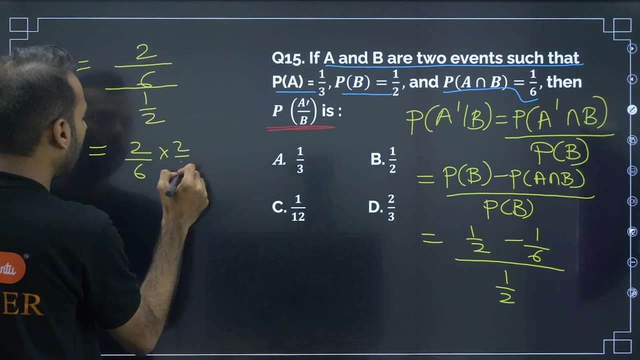 2 and let me write this as 1 by 2.. 1 by 2 minus 1 by 6 is 1 by LCM. if I take LCM, 6, 3 minus 1 is 2 by 1 by 2.. So this is 2 by 6. 2 by 1. 4 by 6 is equal to 2 by 3.. Is there any such option like? 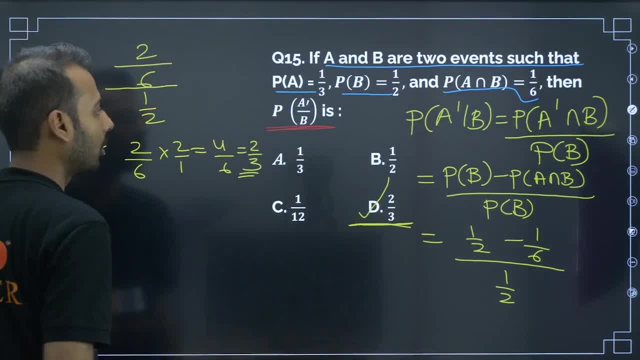 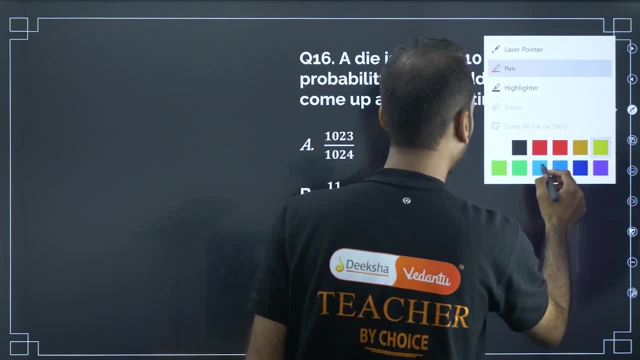 2 by 3, then a dash given b. 2 by 3 is the answer for this. Moving on to next question, A die is thrown 10 times. A die is thrown 10 times. So from Bernoulli trials we can say n is equal to 10.. 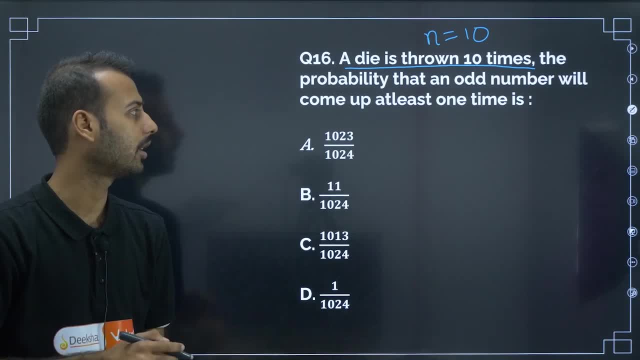 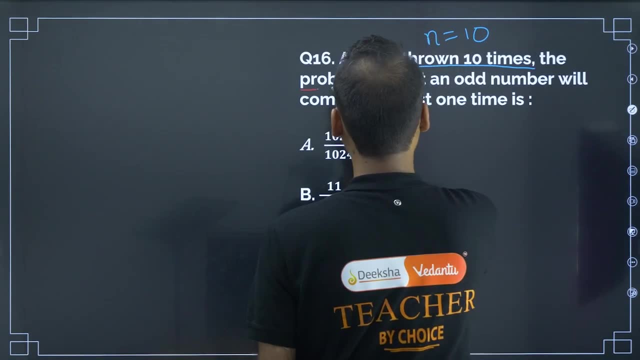 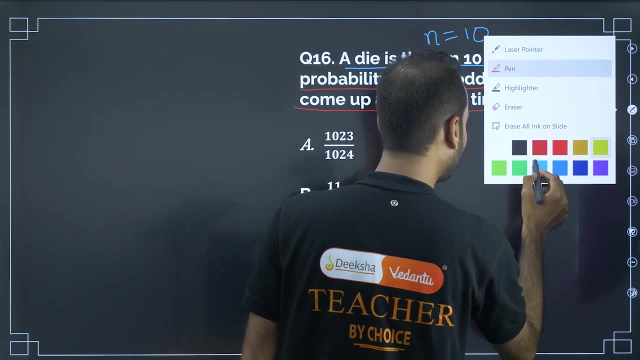 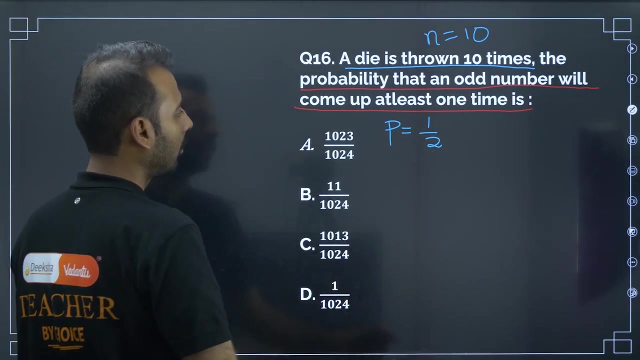 The probability that an odd number will come up at least one time is. the probability that an odd number will come up at least one time is So getting odd number is success. So success is denoted by p. Getting odd number success is 1 by 2.. Next, q is equal to 1 by 2.. Automatically q will be 1 by 2.. 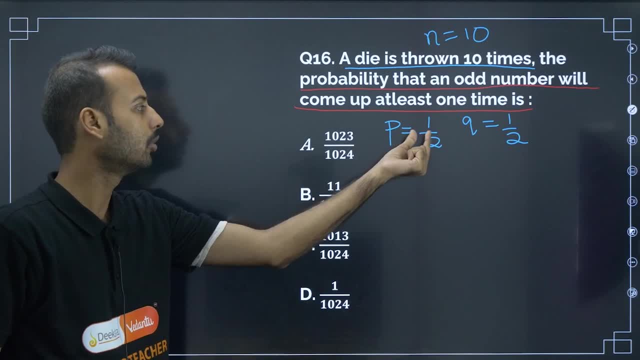 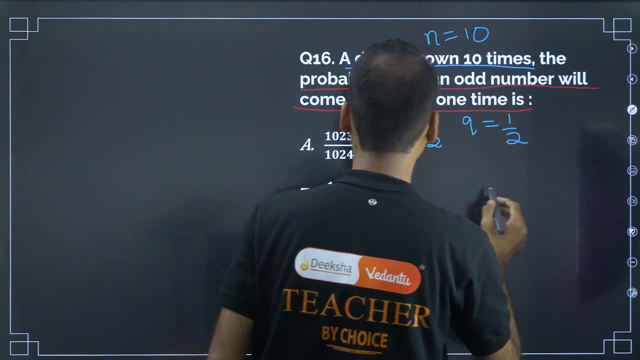 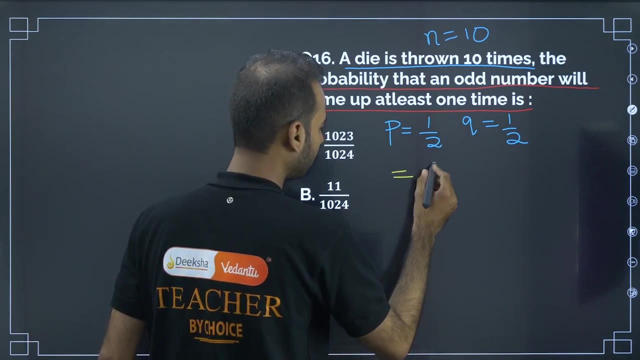 Probability means odd number is success. Success is 1 by 2.. So failure will also be 1 by 2.. At least one time. now, if you go through this, if you go through this probability that an odd number will come up at least once- At least once means required probability is equal to 1. 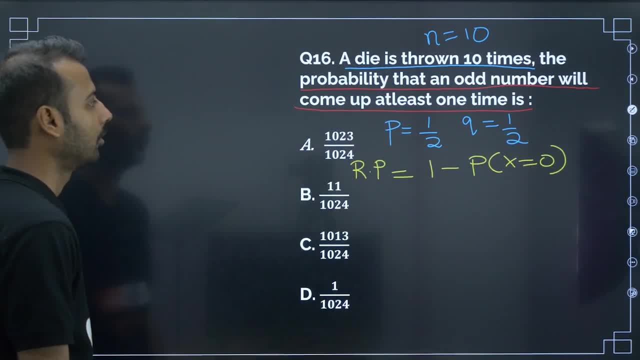 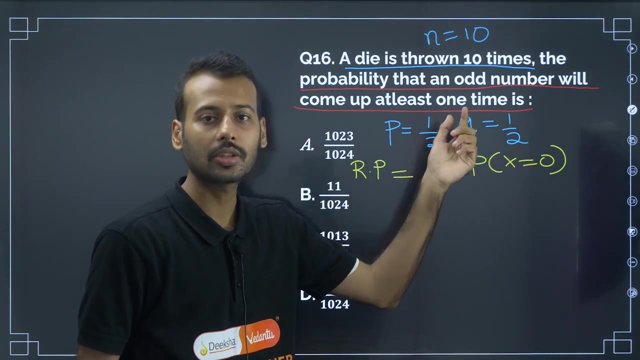 minus probability of x is equal to 0.. Probability that an odd number will come up at least one time Probability. So this will be 1 minus probability of 0.. At least one time means 0 time should not come. One time it is ok, Two times, more times it is ok, But one time should. 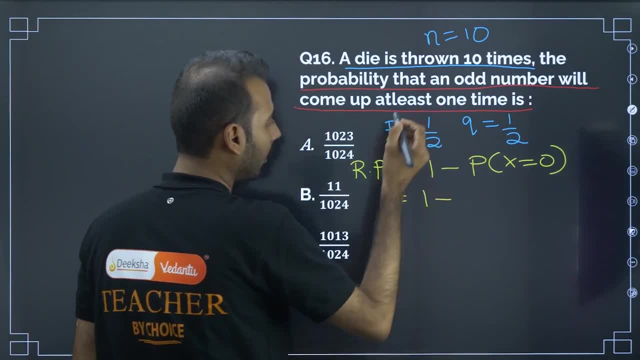 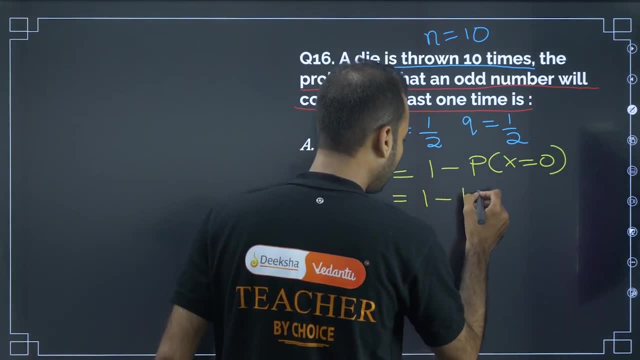 not come means 0 time should not come Now 1 minus. try to recall that Bernoulli n c x, p raise to x, q raise to n minus x. that formula you try to recall. So n in place of n, I am writing n c x p raise to. 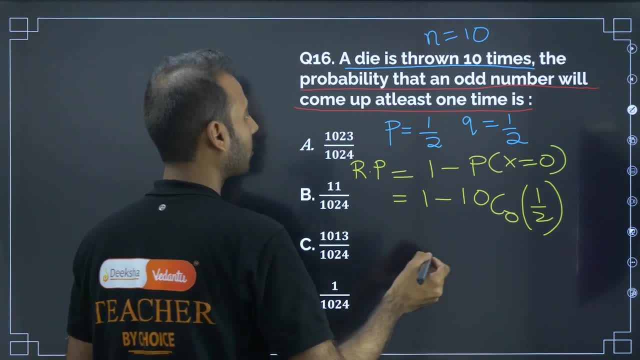 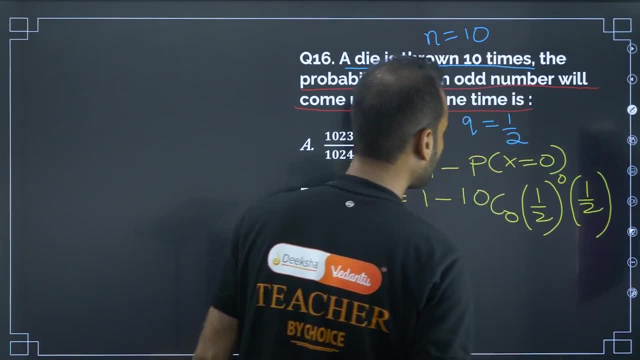 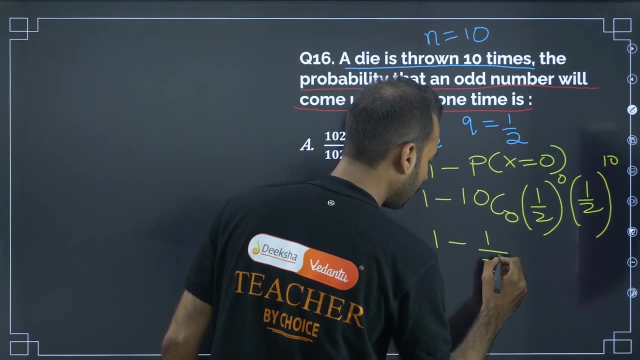 p. raise to x In place of x. what should I write In place of x? 0. q. raise to n minus x. n minus x is n is 10.. So here we are left with 1 minus 1 by 2, 10. So this is equal to 2, 10. So 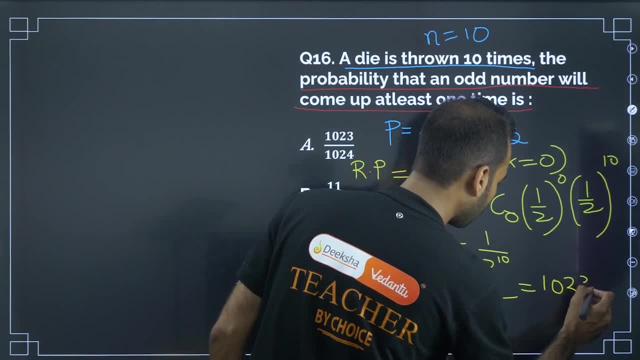 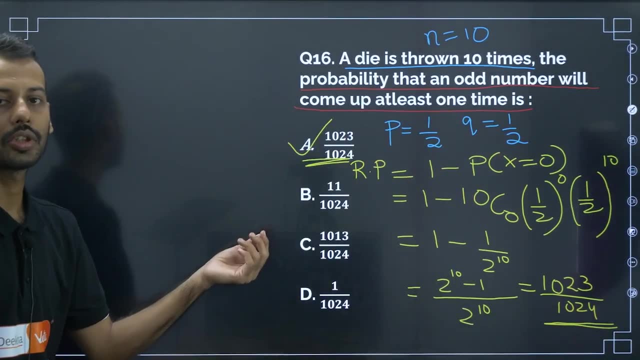 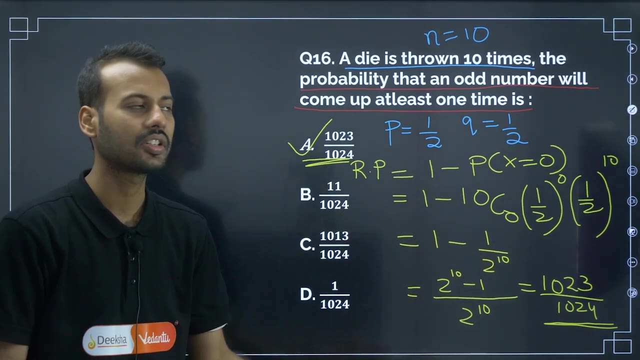 2, 10 minus 1 is equal to 1023 divided by 1024.. So a is the answer for this. Again, easy question: Basic calculations like Bernoulli trials. if you know small calculations, you know within 30 or 40 seconds you can handle this question. Moving on to next question: The probability of solving. 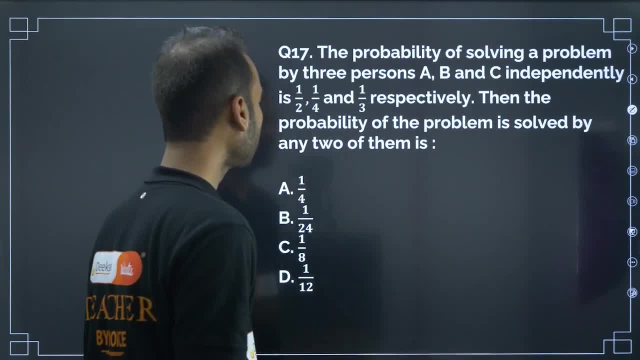 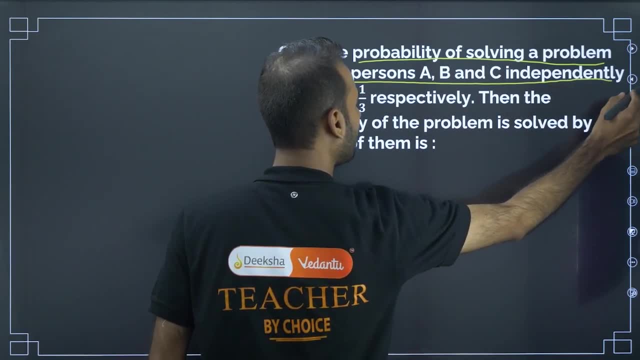 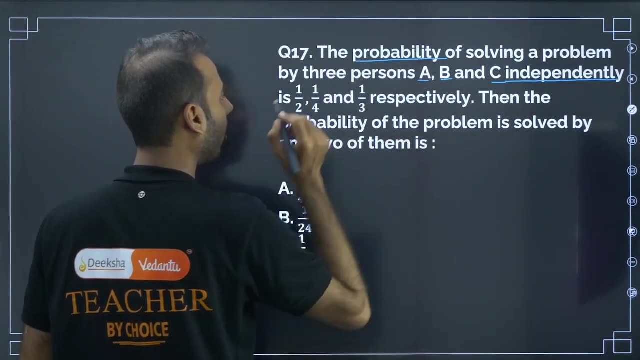 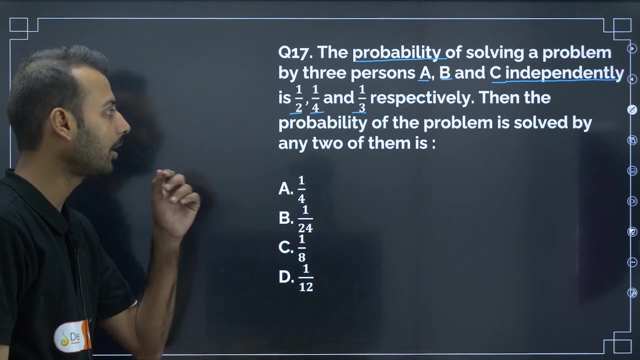 a problem by three persons- a, b and c independently. probability of solving a problem By three persons- a, b and c independently. a, b, c probability of solving a problem. is this much, this much, Then? probability of problem is solved by any two of them. Now, what is? 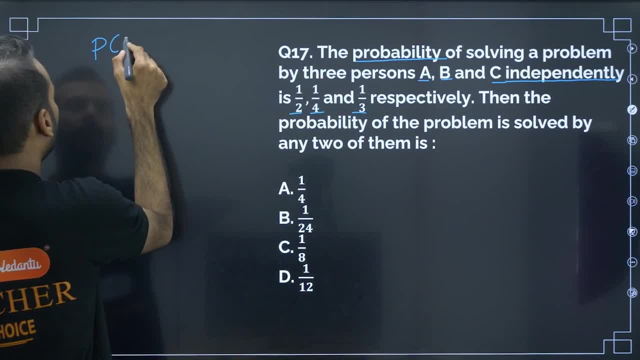 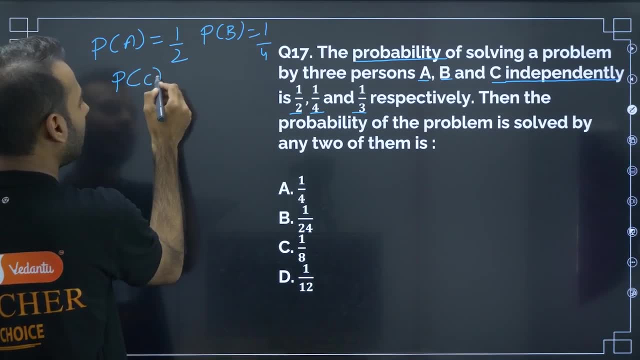 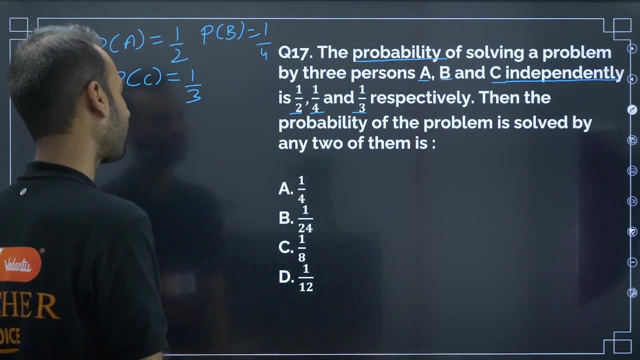 the question. let me write the given data first. A is 1 by 2, b is 1 by 4, c is 1 by 3, c is 1 by 3.. Then the probability of problem is solved by any two of them. probability of them solved. 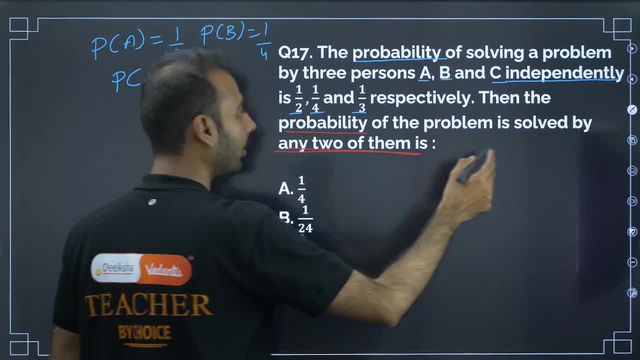 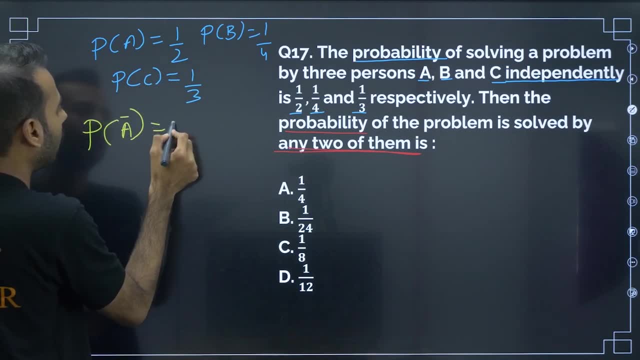 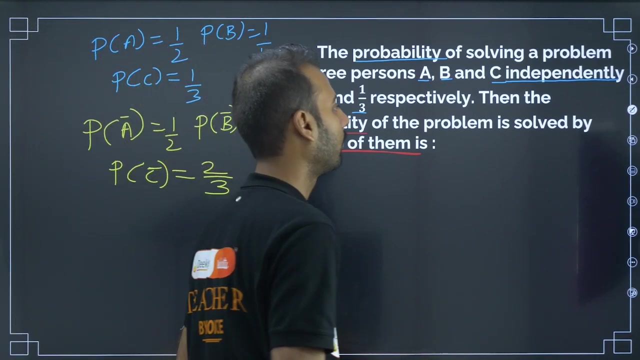 by any two of them. they want probability solved by any two of them. Now, from here remaining data what I can extort: p of a dash is 1 by 2, p of b dash is 3 by 4, p of c dash is c dash is 2 by 3. problem is solved by any two of them. 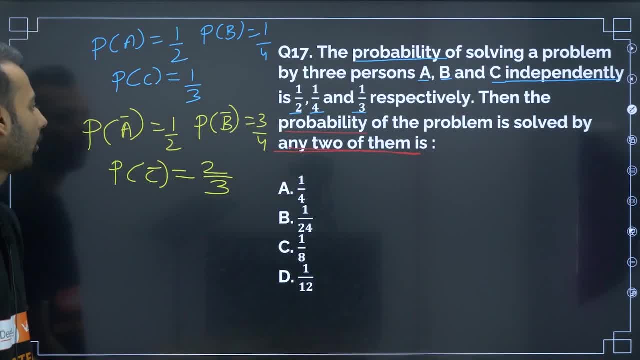 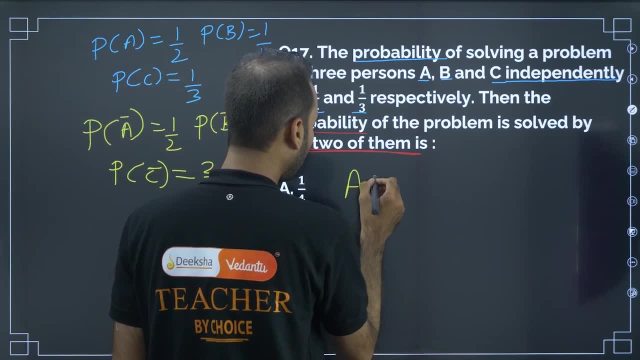 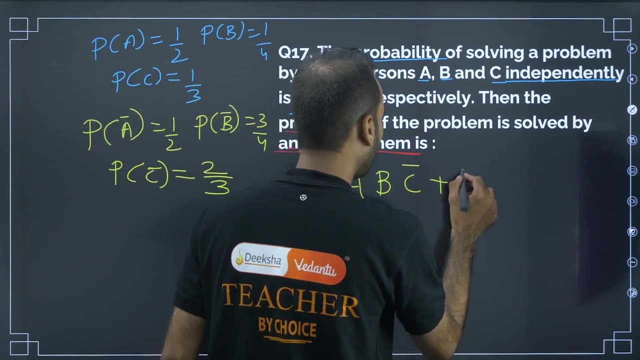 Next, how to approach this. probability of a dash is 1 by 2. this problem is solved by any two of them. means a, b has solved, c has not solved. a, b have solved, c has not solved. Next: a has solved. b has not solved. c has solved a dash: b, c. 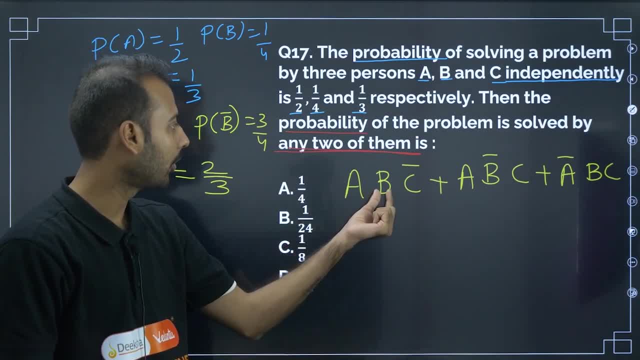 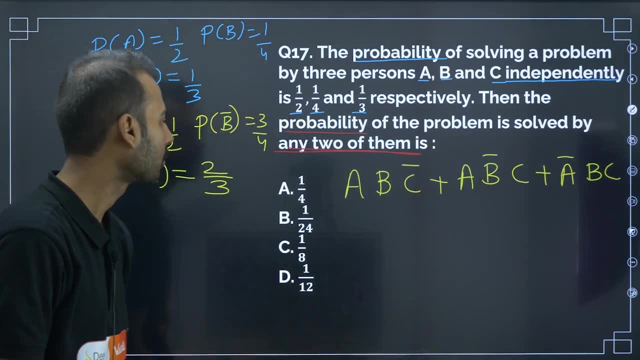 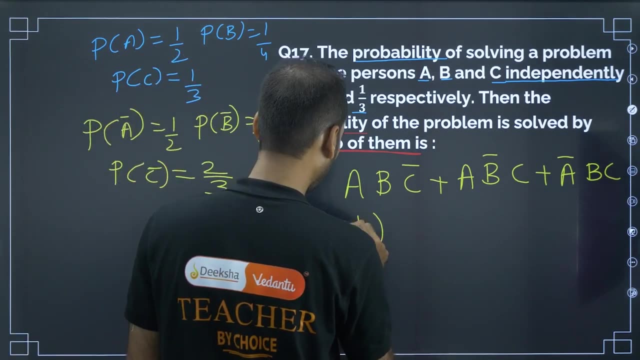 So a- b have solved. at least two of them have solved. problem is solved by any two of them. this and this solved, this not solved. this and this solved, not solved. So you might have understood a- b. a is how much a is 1 by 2, b is how much 1 by 4, 1. 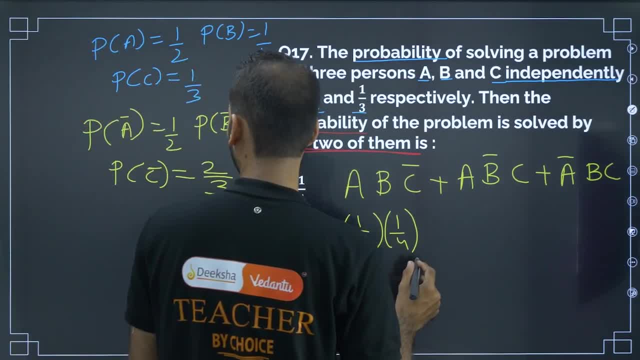 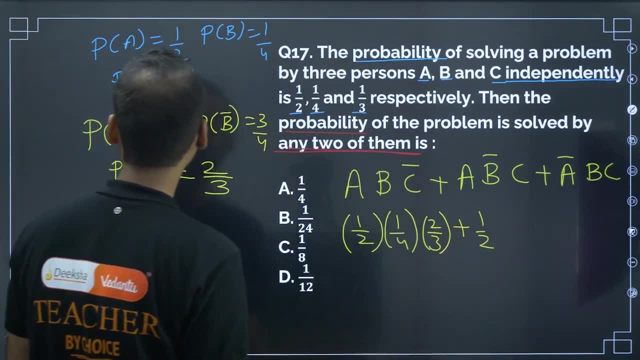 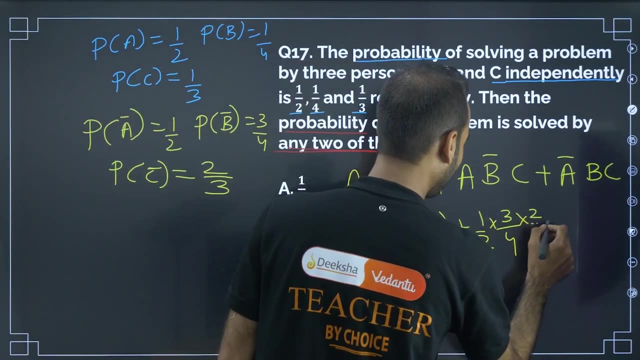 by 4, c dash is how much c dash is 2 by 3, 2 by 3.. A is how much a is 1 by 2, b dash is how much b dash is 3 by 4,. c is how much 2 by 3, 2 by. 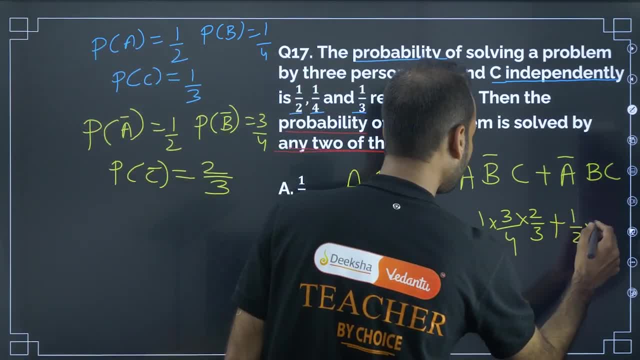 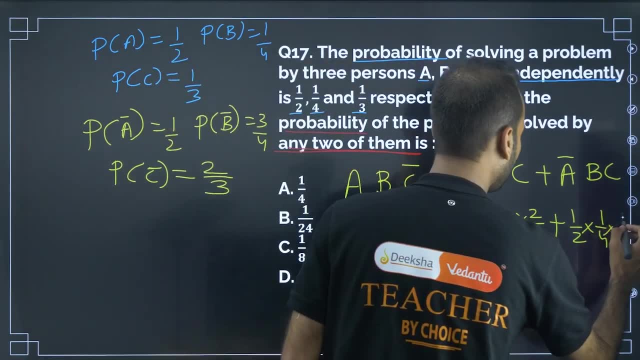 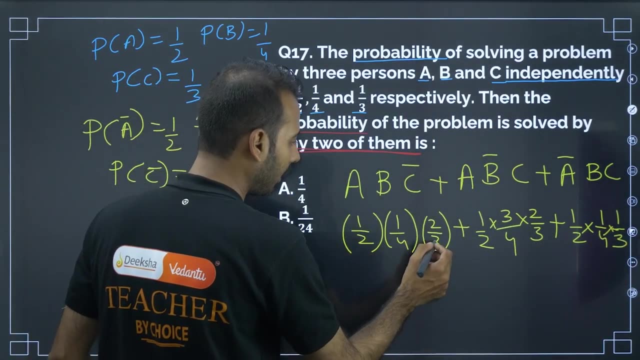 3 plus a. dash is how much 1 by 2, b is b is 1 by 4, c is how much c is 1 by 1 by 3.. So if you do calculation, two fours are. 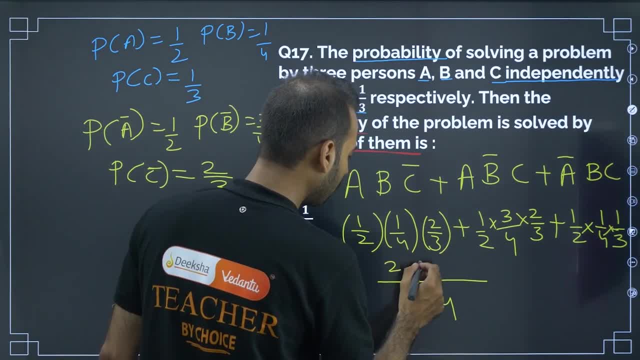 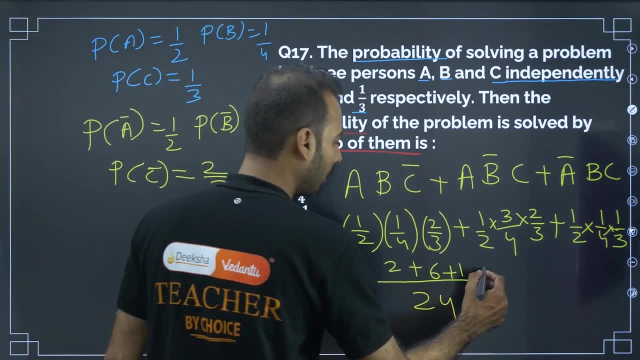 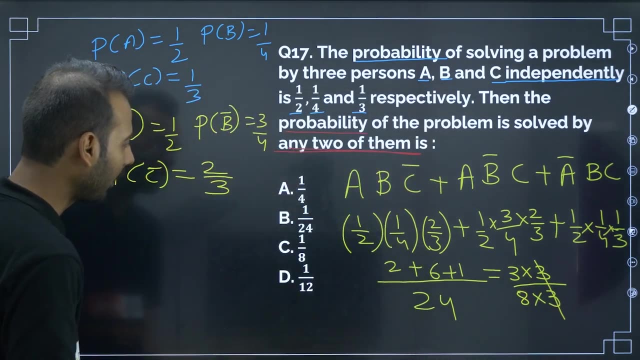 a 24 denominator: 24. 2 plus 6 plus 1, 7 to 9, 9 by 24. 9 can be written as 3 into 3 and 24 can be written as 8 into 3.. So 3 and 3 if I cancel 3 by 8. is there any such option? 3 by the probability. 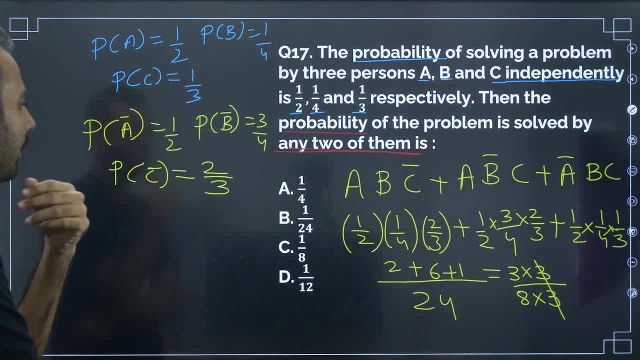 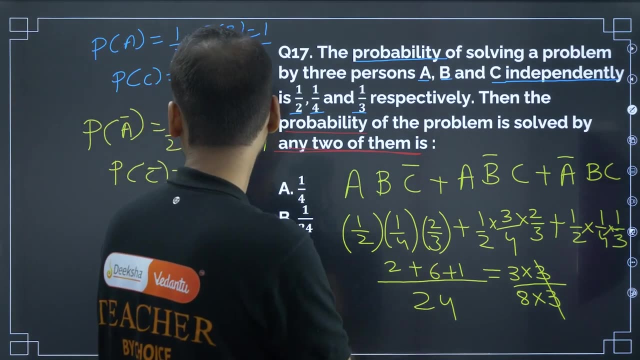 of solved by them is 3 by 8. there is no such option like 3 by 8.. So once you check whether all our calculation is correct or not, a is ok. b is ok, c is also ok. a b: 1 by 2, 1 by 4, c. dash is how. 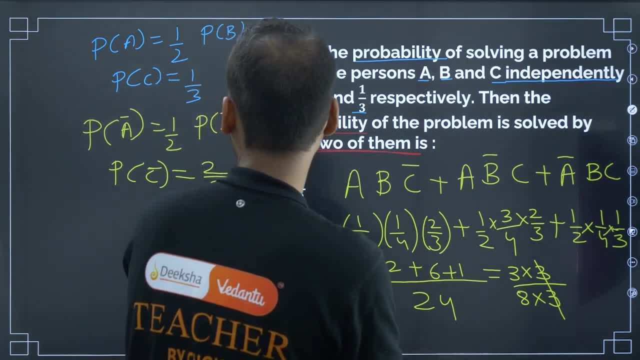 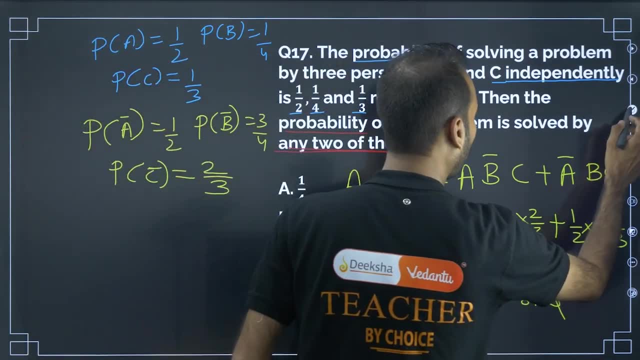 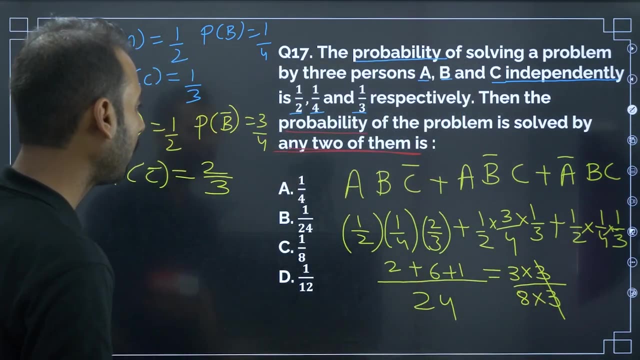 much. 2 by 3. a is 1 by 2. b dash is 3 by 4, c is 2 by 3, c is 1 by 3.. So here one small calculation mistake we did In hurry in exam. do not do such mistake. c, what about a? a dash is 1 by 2, b, c. 3 by 4. b, c. b is 1. 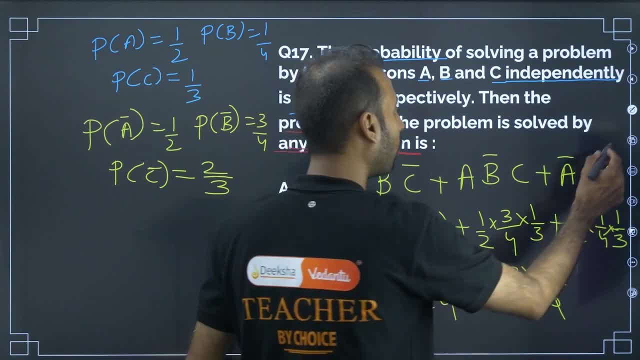 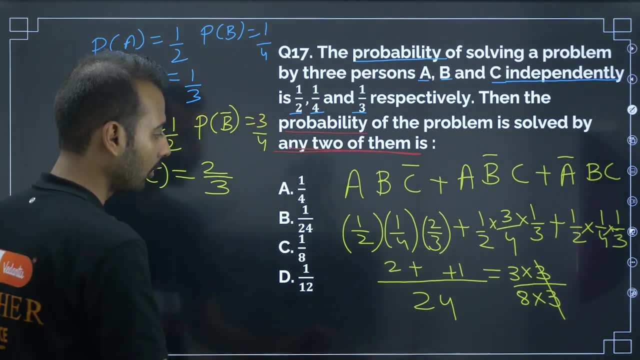 by 4, c is 1 by 3.. So one small mistake. we did one calculation mistake. do not do such calculation mistake in exam. here you do while practicing, you do no problem. So 3 plus 3, 6, let me erase this. 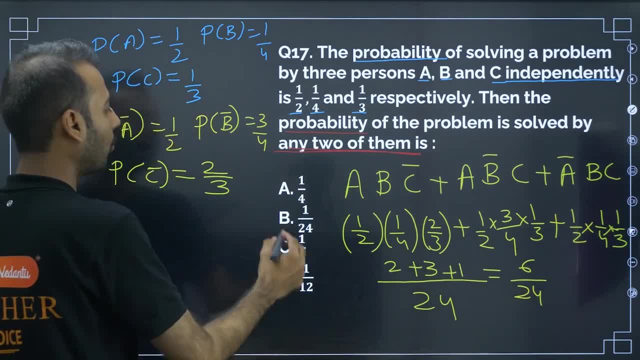 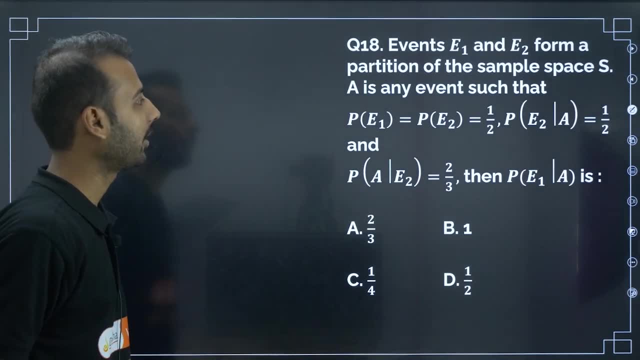 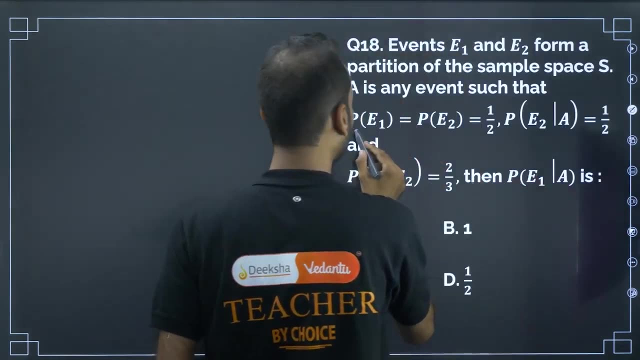 6 by 24.. So this is equal to 1 by 4.. So 1 by 4 is the answer. moving on to next question: events e 1 and e 2 form partition of sample space. yes, a is any event such that such that they have given. 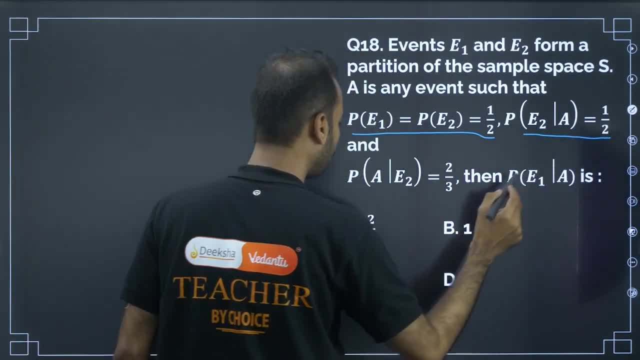 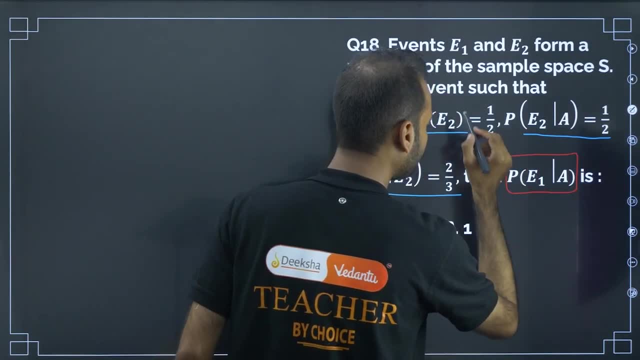 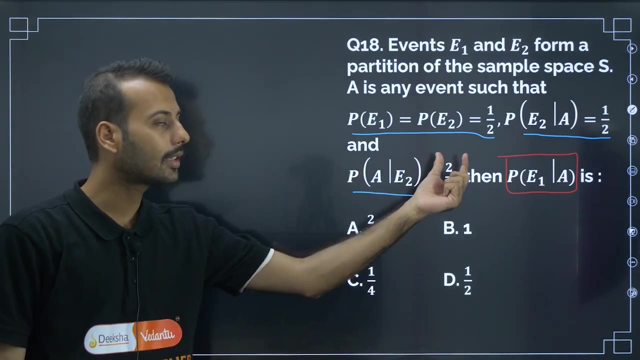 this much of information, and this also they have given and a given to. then what are they asking? ultimately, their target is this one: E 1, e 2, partition of sample space. this say goose, any event. So all this is related to base theorem, open base theorem, sample space, partition of sample. 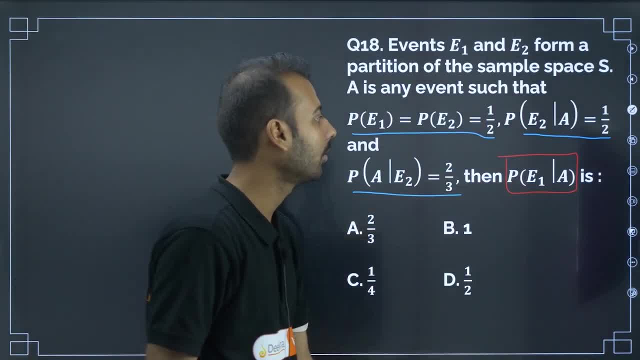 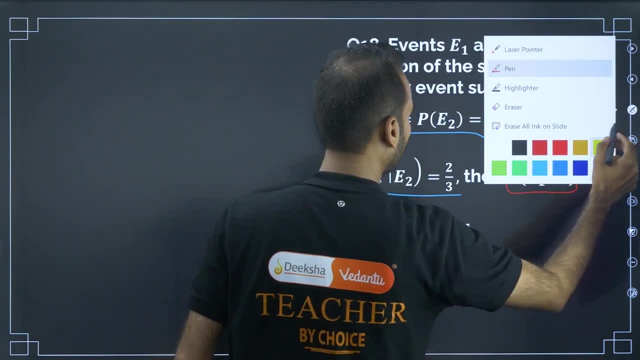 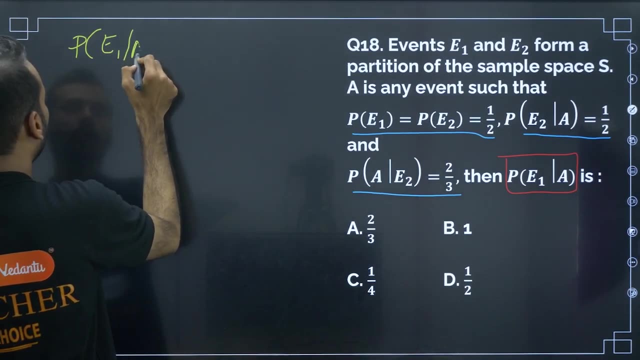 space, everything it comes there only So p of even given a. they are asking to find this probability of even given a. Now, how to solve this problem? probability of even given a. For this probability of e, 1 given a is equal to. 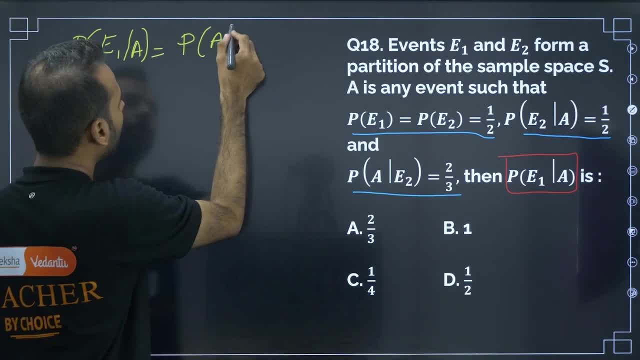 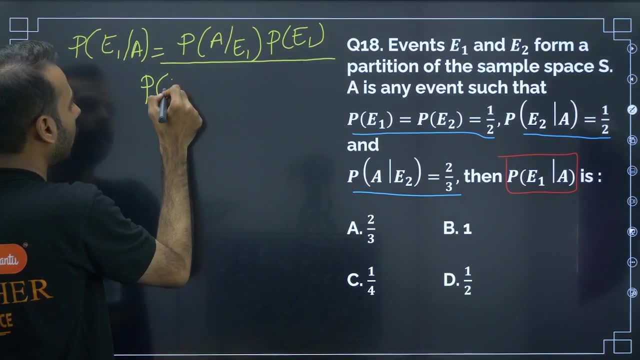 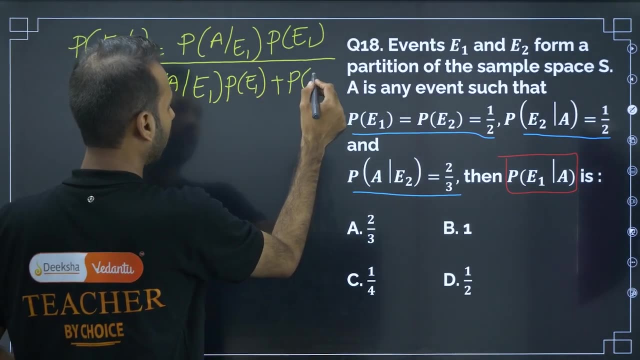 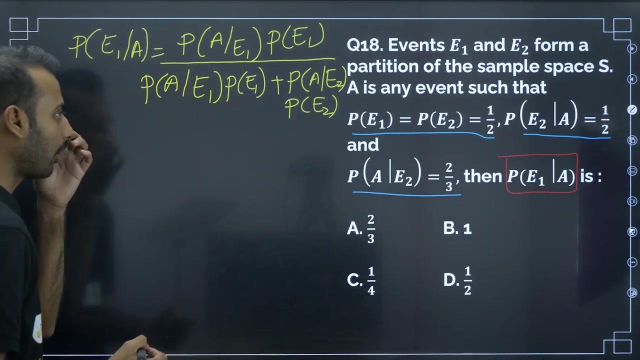 probability of a given E1: dot probability of E1. by probability of a given E1. by probability of E1 plus probability of a given E2: dot. probability of E2.. So probability of a given E1 is of a given E1 is- we do not know this one also. 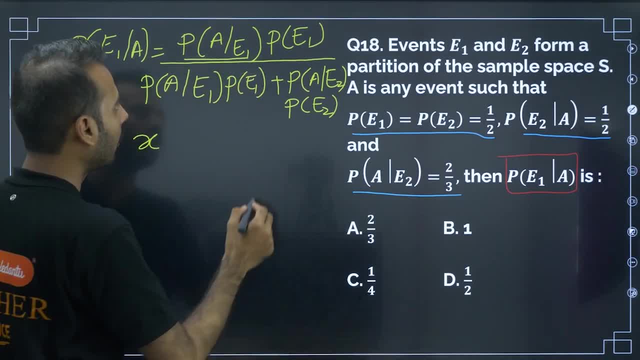 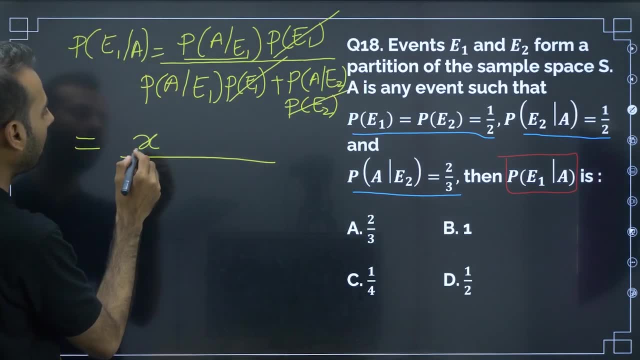 So for a moment, let me name that as x probability of E1. I will cancel off this, this and this. So finally, what are we left? a given E1 is so that for that I have assigned x. next, probability of a given E2 is 2 by 3.. 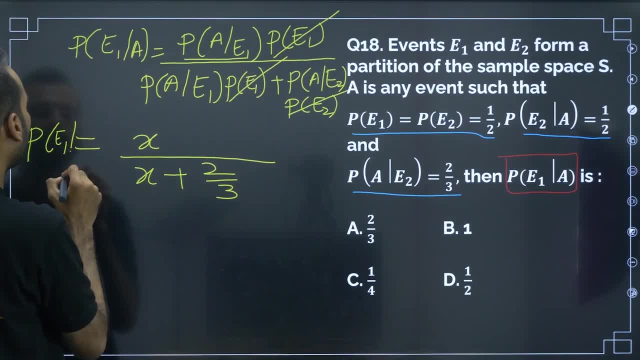 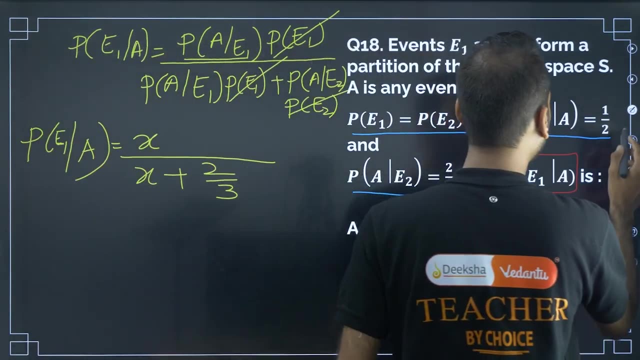 Now we are supposed to find this: E1 given E2.. E1 given A, E1 given A. This we are supposed to find: x is equal to x divided by x plus. Now, what is that we are supposed to find here? 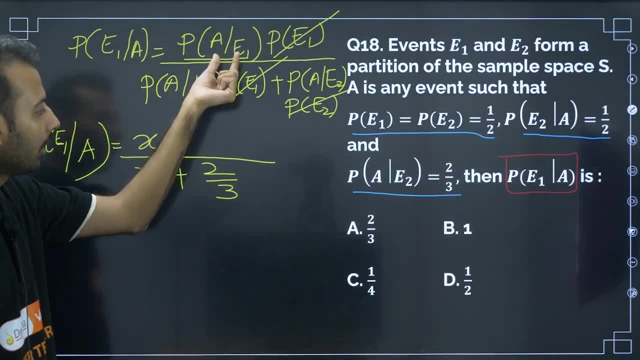 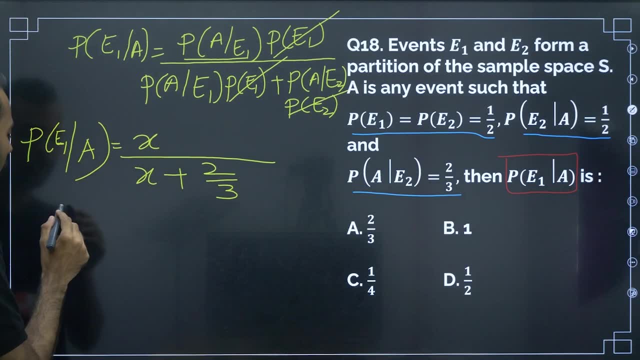 So what is that? a given E1, we have to find. A given E1, we have to find. So for this let me write one more formula using Bayes theorem: E2 given A, E2 given A, E2 given A can be written as if I use a given E2 dot. probability of. 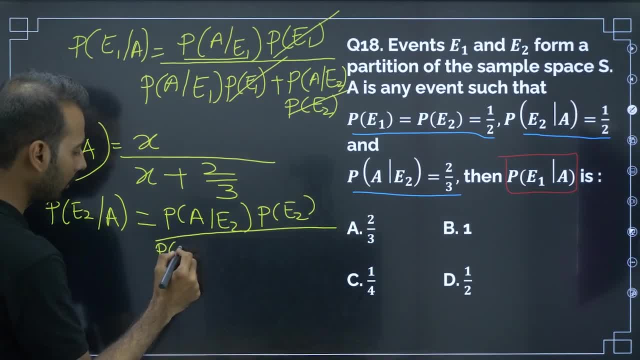 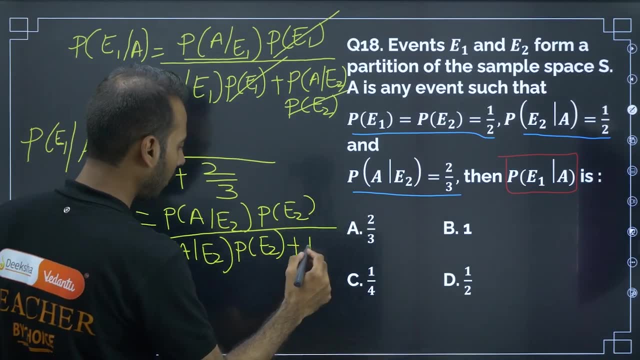 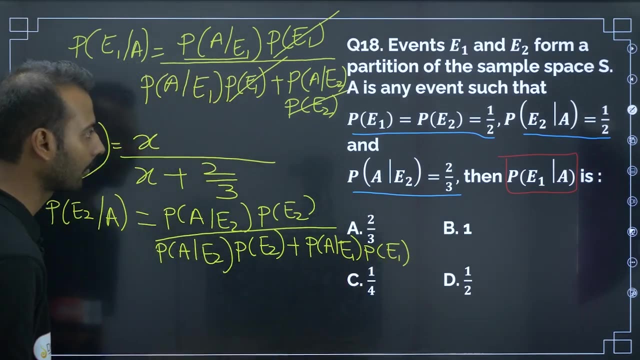 E2.. Next a given E2 dot probability of E2 plus probability of a given E1 by probability of E1 dot probability of E1. this much Now again E2, E2, E1 I will remove off. a given E2 is 2 by 3 by 2 by 3 plus a given E1 is how: 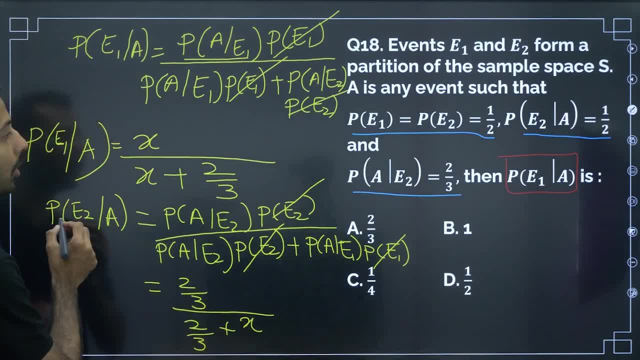 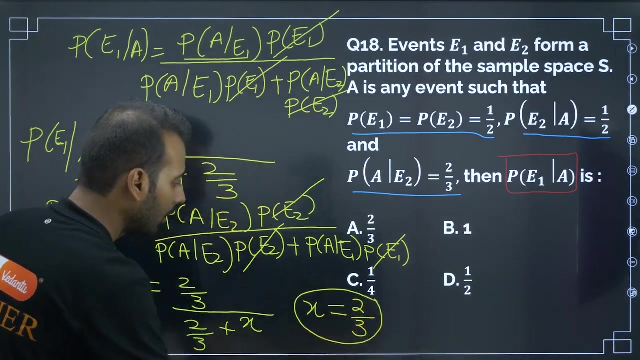 much. let me write that as x, E2 given A, is how much 1 by 2, 1 by 2.. Now we have to find this x from this equation. So how to find x? this entire, I will place it here. So 2 by 3 plus x is this, if I transpose 4 by 3 minus 2 by 3, after solving this equation. 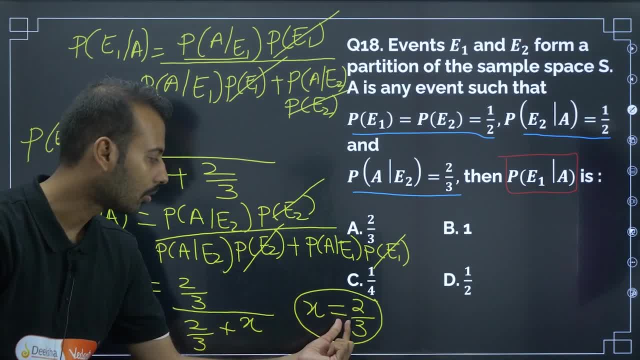 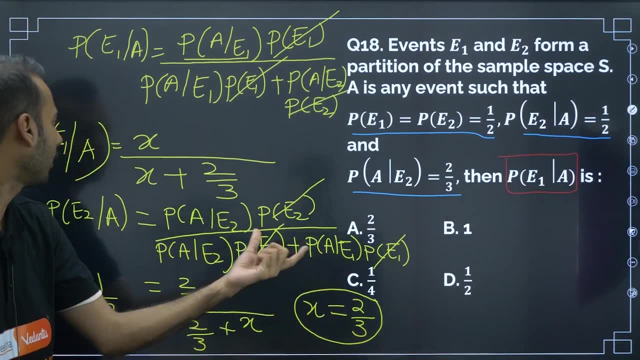 see here. after solving this equation, we will get: x is equal to 2 by 3.. Now this x is equal to 2 by 3. if I place here: what is that? x is what? a given E1. a given E1, a given. 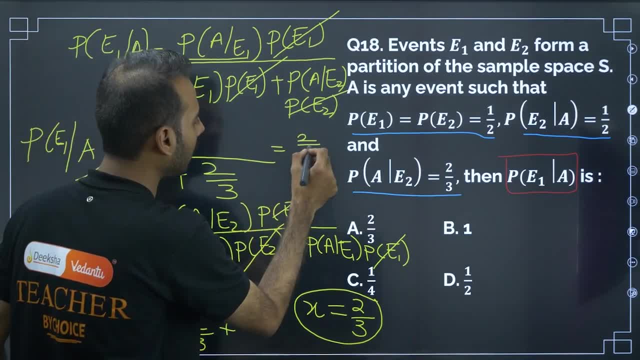 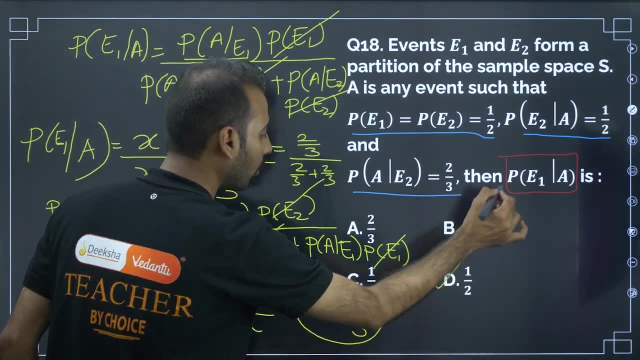 If I place here x is equal to 2 by 3.. This is 2 by 3 by 2 by 3 plus 2 by 3. this is equal to 1 by 2. why it is equal to 1 by 2: 1 quantity divided by quantity plus quantity here 1, quantity here 2 quantities. so answer: 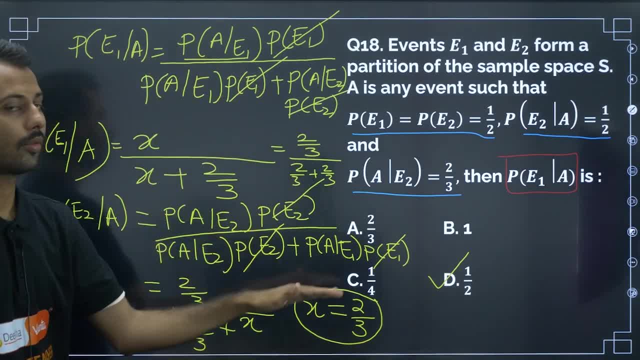 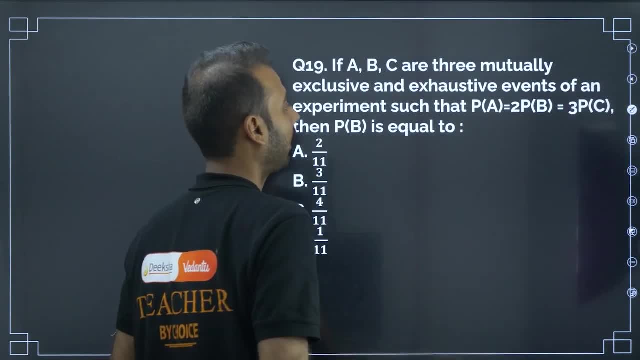 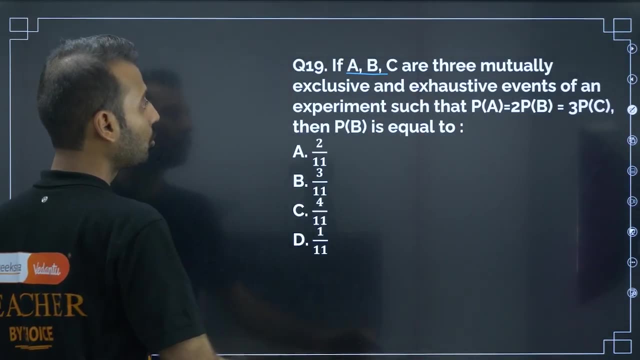 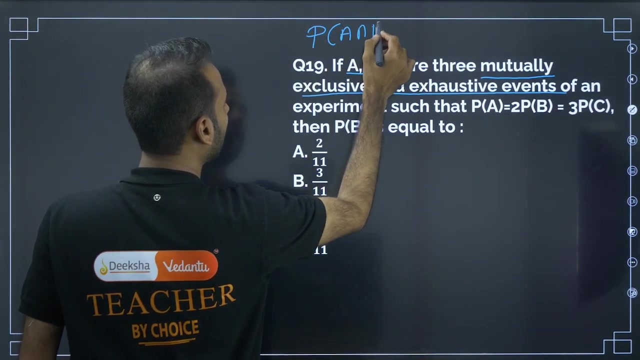 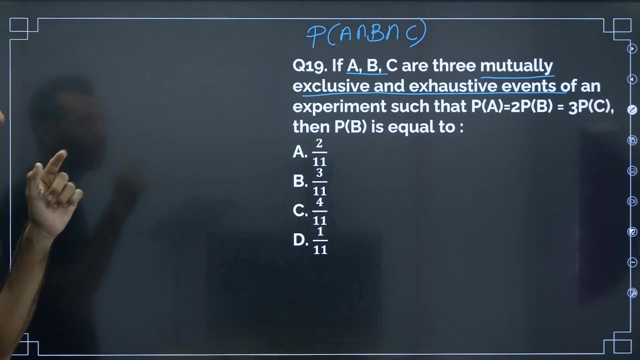 is d. So only simplification, only one formula, Bayes theorem formula and simplification. that is it. moving on to next question, if A, B, C are 3 mutually exclusive and exhaustive events, So if A, B, C, A B C are three mutually exclusive and exhaustive events, that means A B C exclusive. 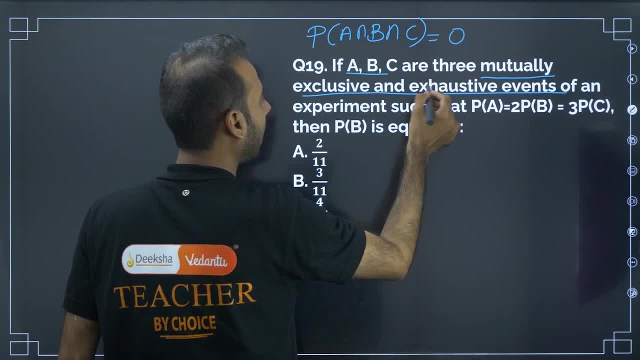 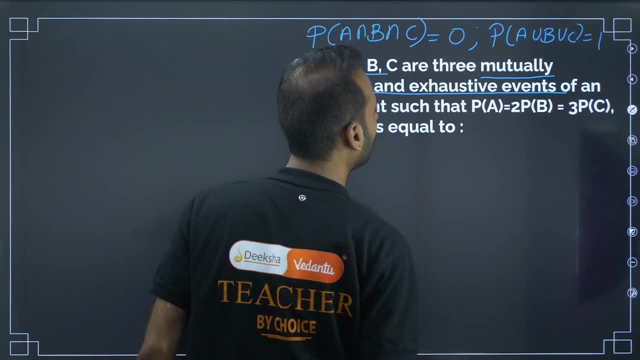 mutually exclusive means. this is 0. Exhaustive means A union. exhaustive B union. C is 1 sign I would say it is total of better Biennials of B hoch B. Humans understand this much. They all are very, very. those are rather 0s. 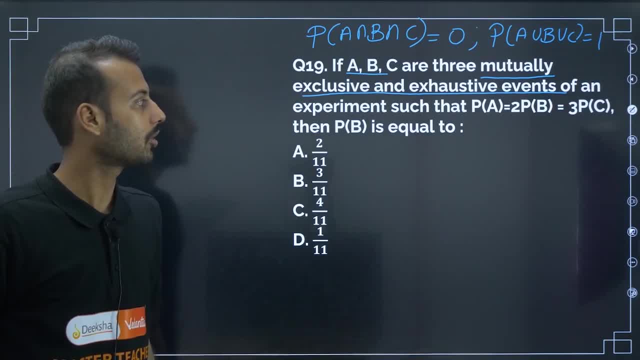 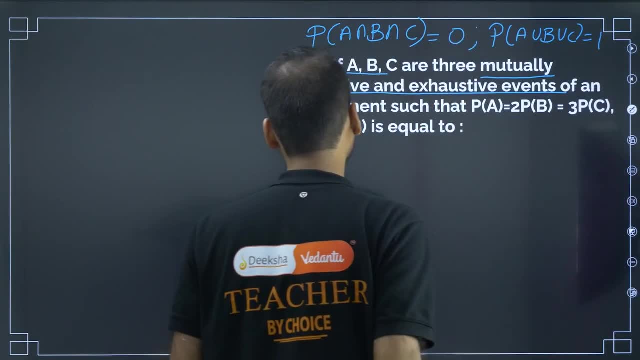 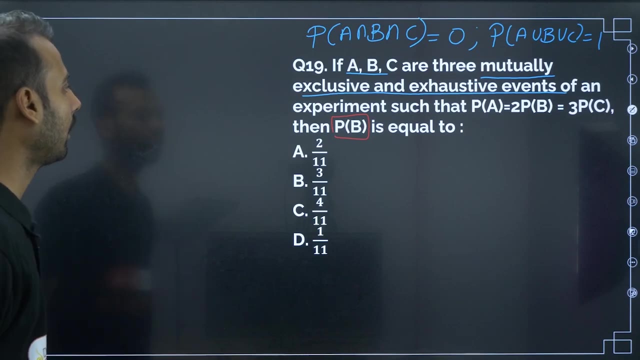 element such that p of a is 2, p of b is equal to 3, then p of b is equal to what? p of b is equal to what? what is the question then? p of b is equal to what they are asking to. 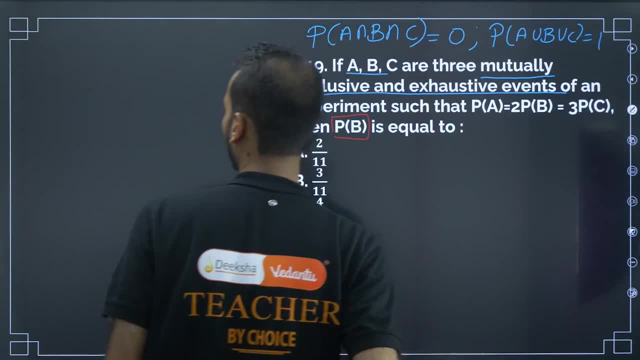 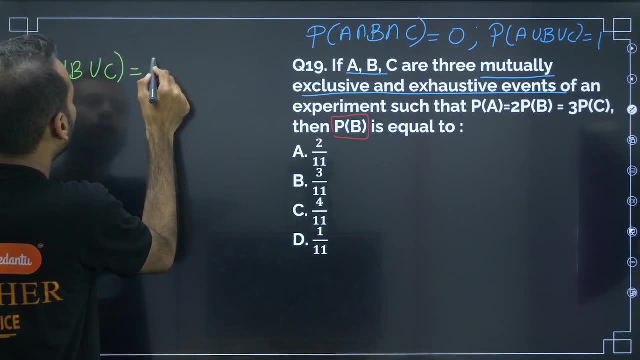 find p of b. Now one synopsis point. you should be knowing what is that synopsis point p of a union b, union c is equal to a, a, b, c minus b, c, c, a, all that. it well be 0 anyways. 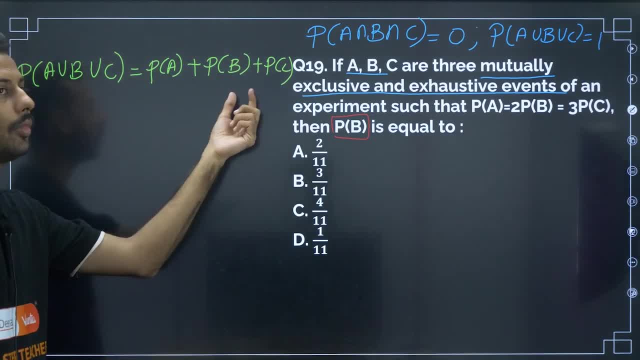 So p of a union b remaining minus a, b, b, c, c, a, all that well, be there 3 mutually exclusive events. So I am not writing remaining things because anyways it will be 0. Okay, only So A union B, union C, value is 1. So I am writing 1 here. P of B is equal to P of 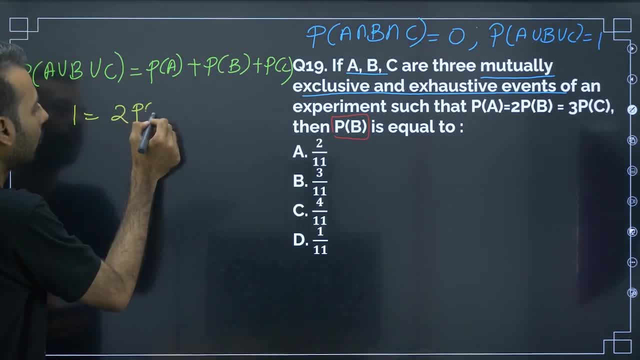 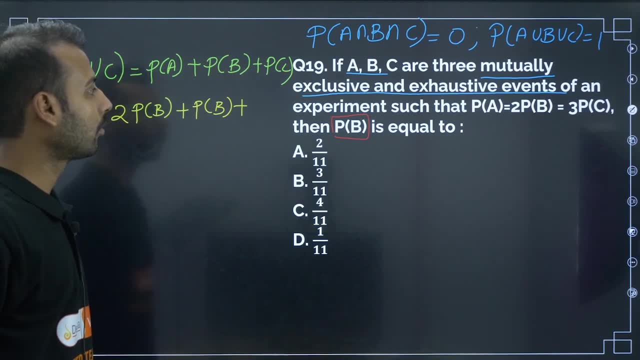 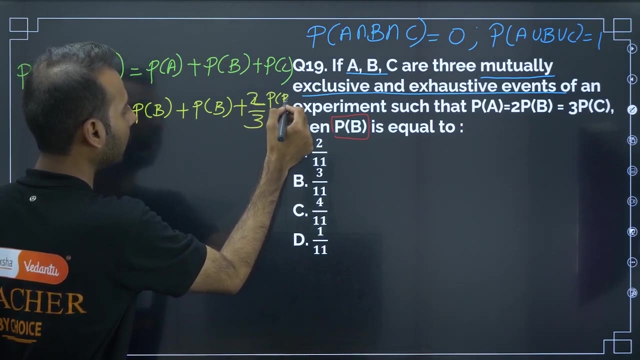 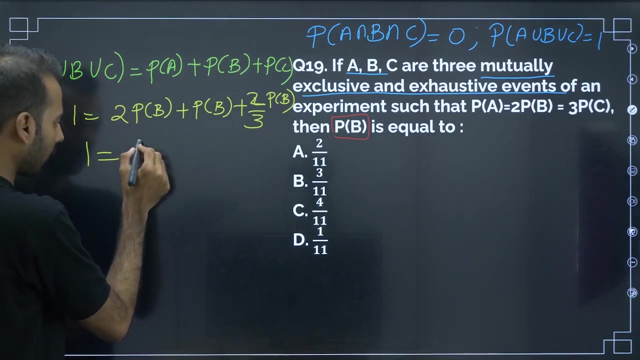 A is 2 times of P of B. 2 times of P of B plus P of B plus 3 P of C is how much? 2 by 3 P of C is 2 by 3, 2 by 3 of P of B. So 1 is equal to 3 plus 2 by 3 is 11 by 3 P of B. if. 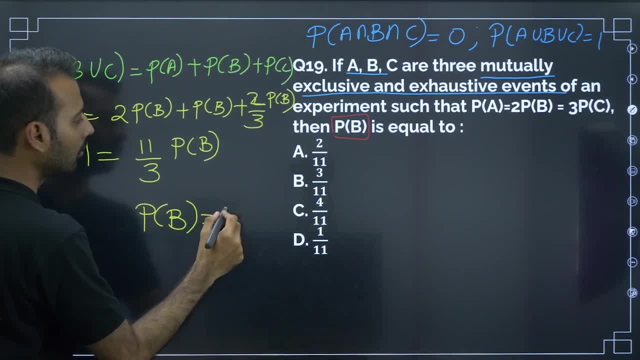 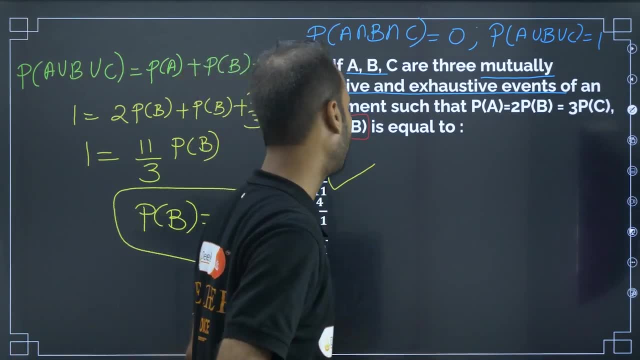 you add this. So finally, P of B is equal to 3 by 11. P of B is equal to 3 by 11.. So is there any such formula? Yes, B is the answer for this. Moving on to next, 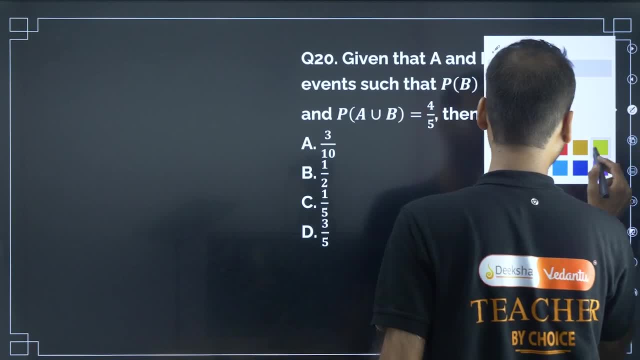 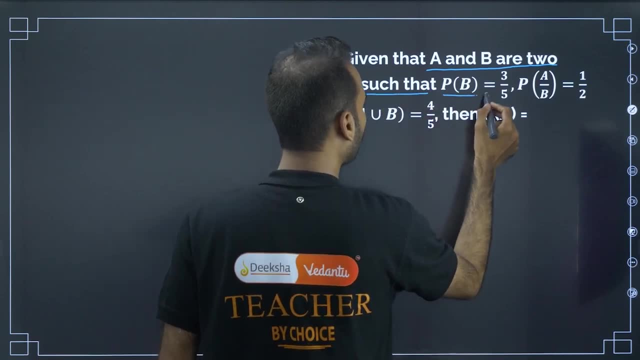 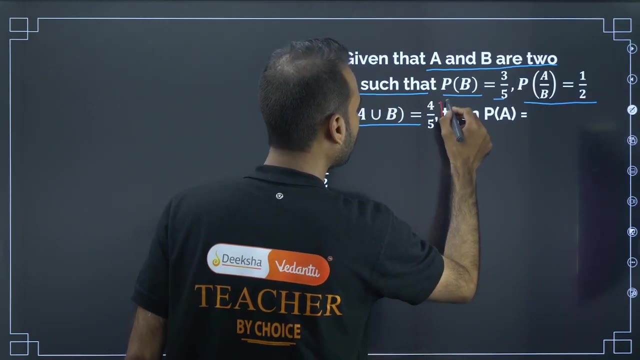 next, Given that A and B are two events, what have they given? A and B are two events such that P of B is this much, P of A given B is this much, and then P of A is: what are they asking? P of A is how much they are asking this. So how to approach this? So please, 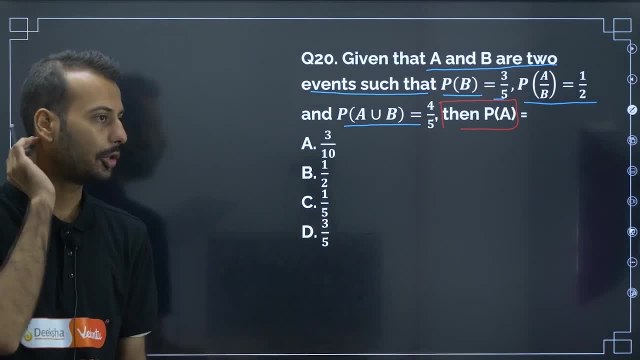 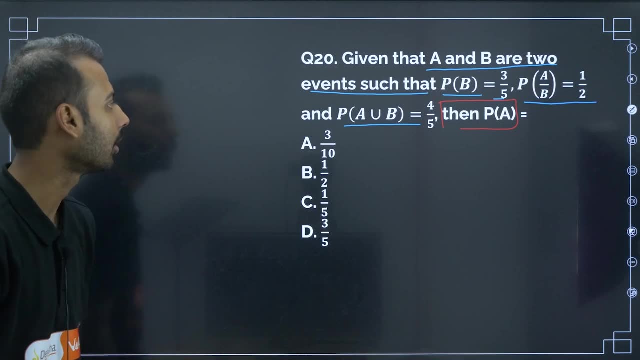 be aware of the synopsis, These many videos I have discussed with green pen, and also probability chapter. you keep aside your that book if you do not know synopsis. if you know, it is a good thing. Next, P of A union B is equal to 4 by 5. So P of A union B is equal to. 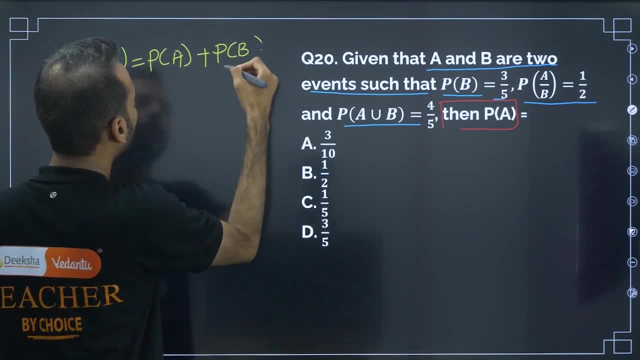 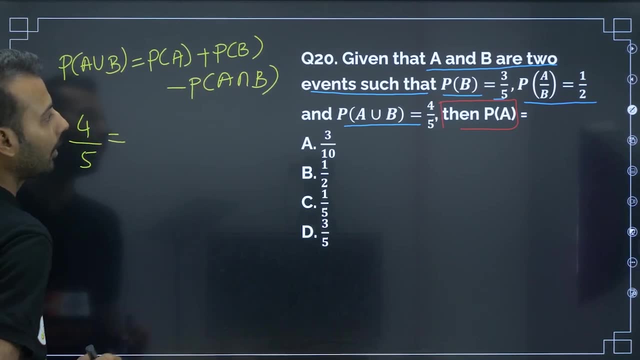 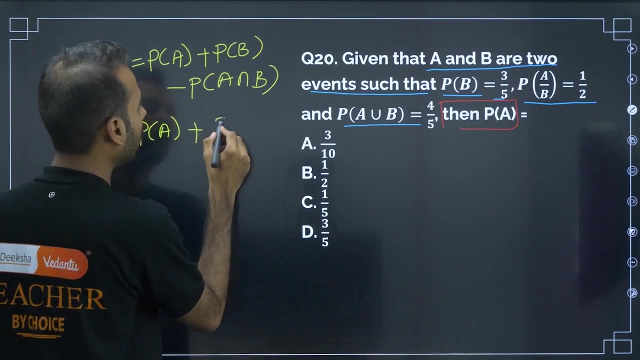 P of A, P of B, P of B minus P of A, intersection B. So P of A, union B is 4 by 5, P of A is P of A. then, ok, we have to find this. So P of A, ok, P of B is 3 by 5, P of A is 3 by 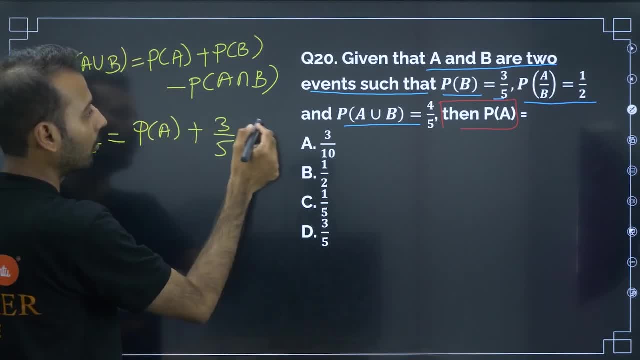 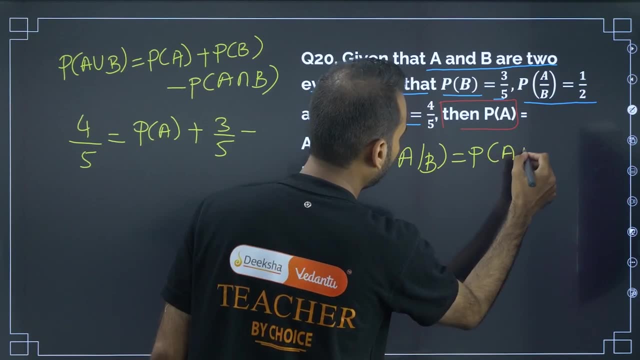 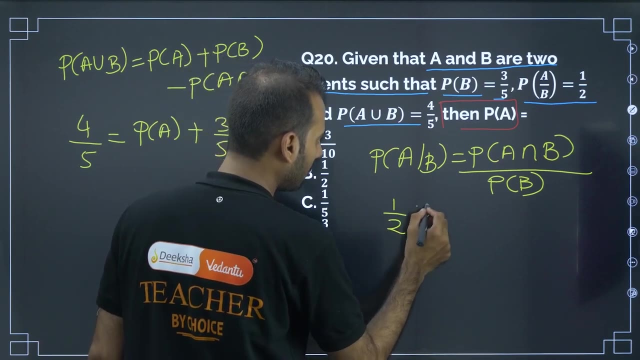 5, P of A intersection B is A intersection B is not known, but one more data they have given: Probability of A intersection B is equal to probability of A intersection B divided by probability of B. So probability of A intersection B is equal to probability of 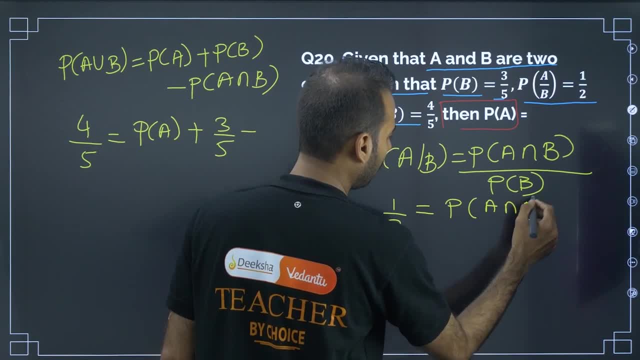 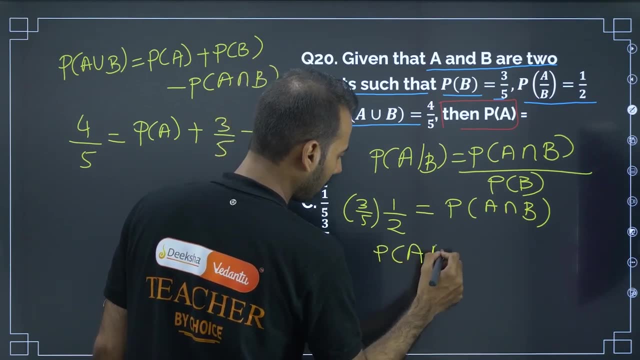 A intersection B. probability of A intersection B. probability of B is 3 by 5.. So if I place this 3 by 5, probability of A intersection B is equal to 3 divided by 10.. So if I place 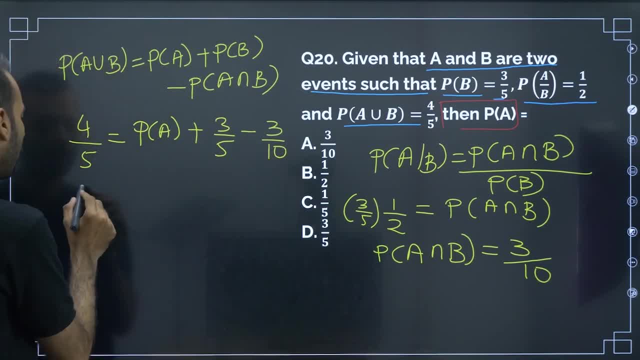 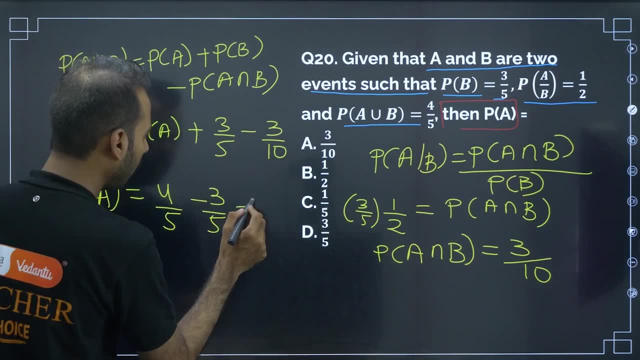 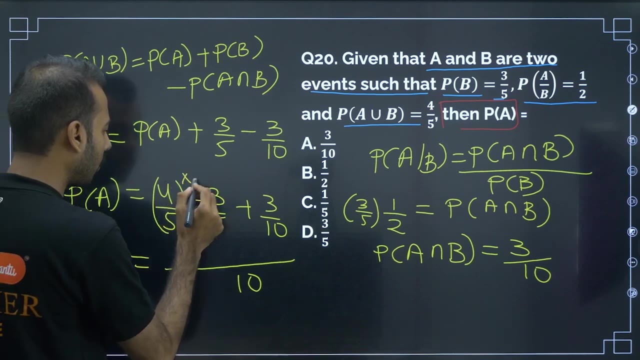 3 divided by 10. here what we have to simplify this P of A is equal to 4 by 5 minus 3 by 5 plus 3 by 10.. So if I take LCM, if I multiply this with 2,, if I multiply this with 2,, 4. 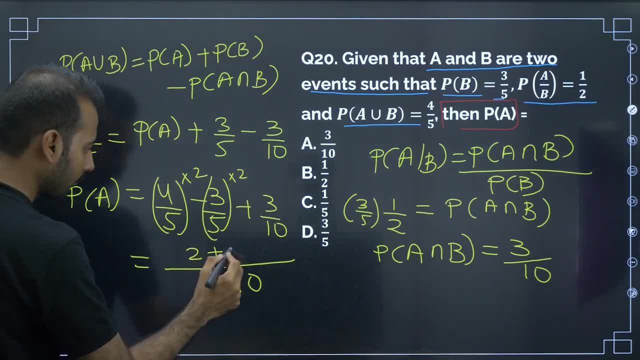 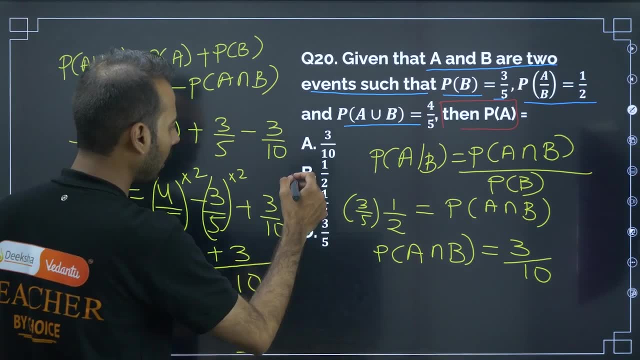 2 psi. 8 minus 6 is 2 plus 3 is equal to 5 by 10, which is equal to 1 by 2.. Is there any such option like 1 by 2?? Yes, B is the answer for this. 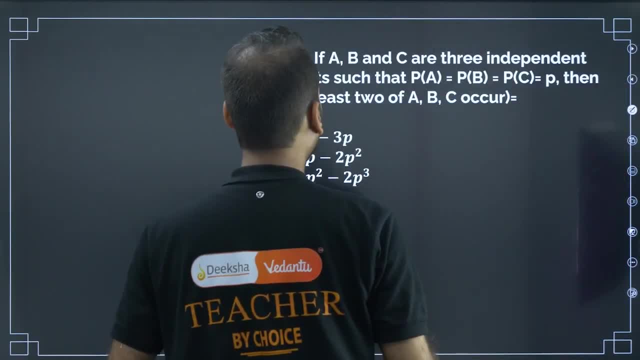 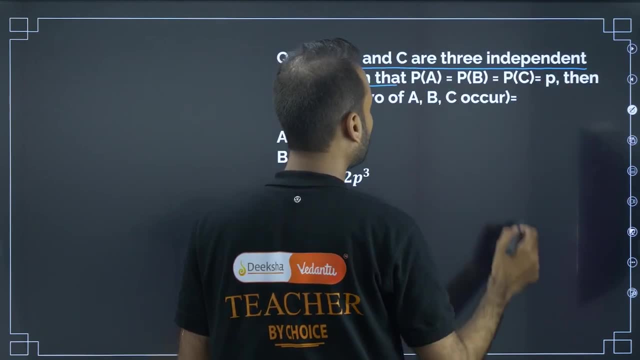 Moving on to next question, If A, B, C are three independent events, A, B, C are independent events such that P of A is equal to P of B, is equal to some information they have given. they have named that. P of A is equal to that. P of B is equal to some information they have. given. they have named that P of A is equal to some information. So it is, as like many of them, as much as it became כן, So that P of A is equal to, so that P is equal to, so that 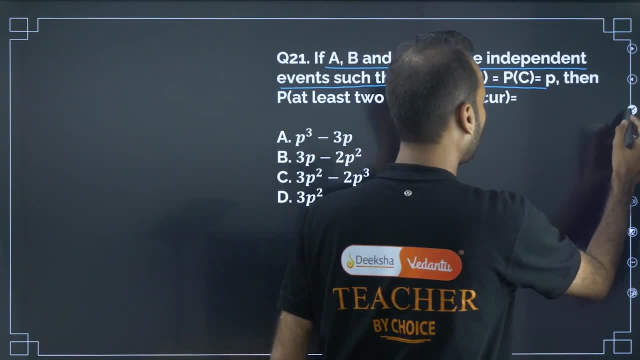 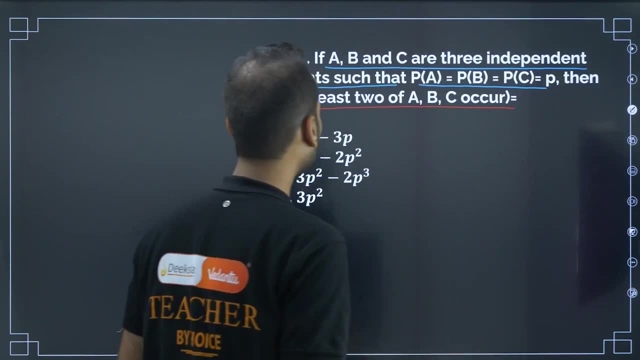 a, then p of at least 2 of a, b c occur is equal to. what is the question? p of at least a, b c occur is equal to at least a b c should occur. that means a b occurring c. 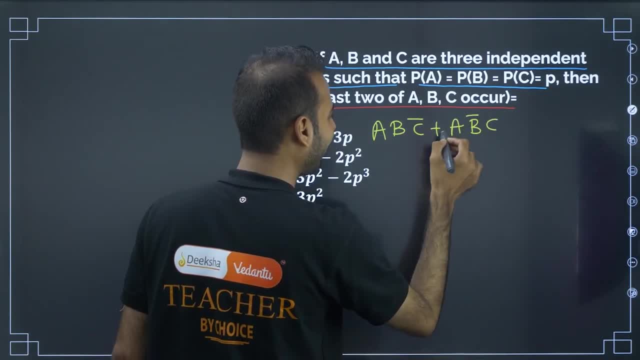 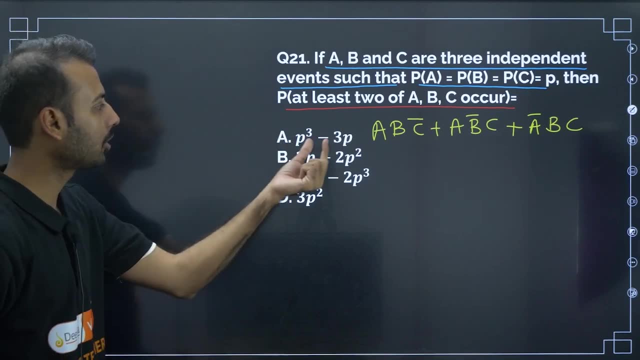 not occurring: a, b, dash, c, a, c occurring, b not occurring. next a not occurring, b, c occurring. So at least 2, at least 2 means these 2 are occurring. this one is not occurring. 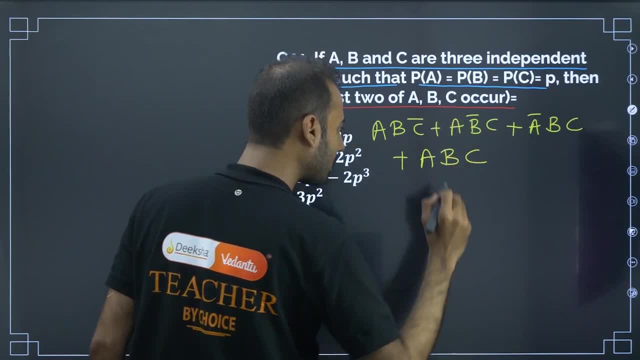 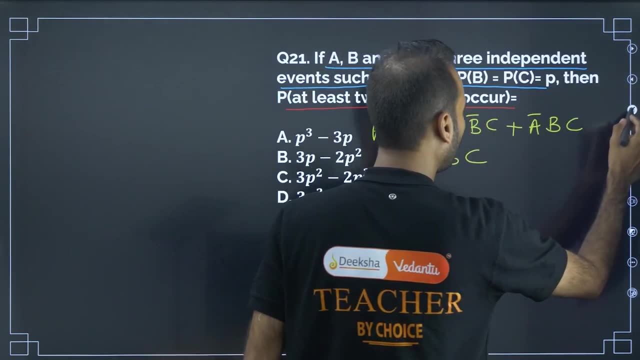 next, at least 2 means all 3 occurring. that also. we have to consider that also. if all 3 are occurring, then also it is ok. Now if I go for substituting their probabilities, probability of A is b, probability of b is also p. 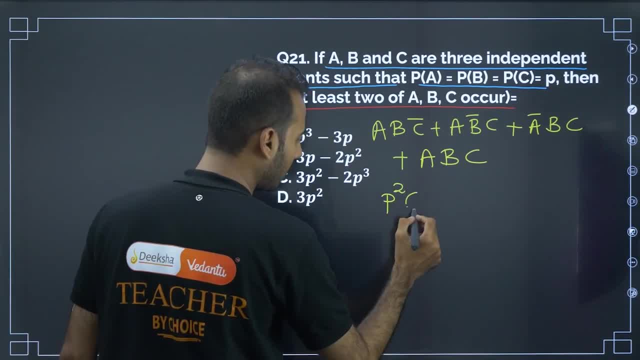 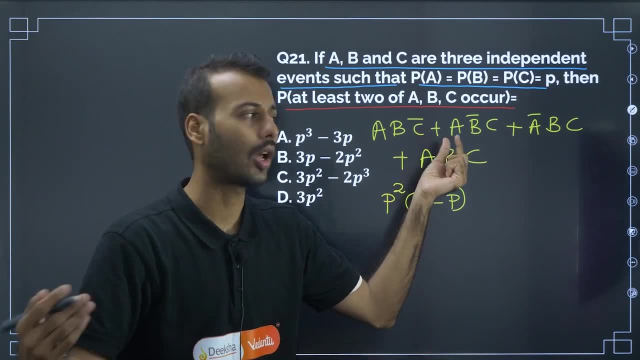 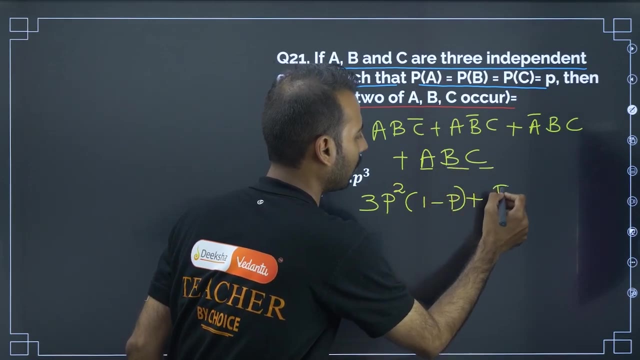 So that is equal to p square. probability of C is 1 minus p, because probability of occurrence is p. then probability of non occurrence is 1 minus p. Same way we are having these three, 3 times plus probability of A, probability of B. this is equal to p cube. so this is: 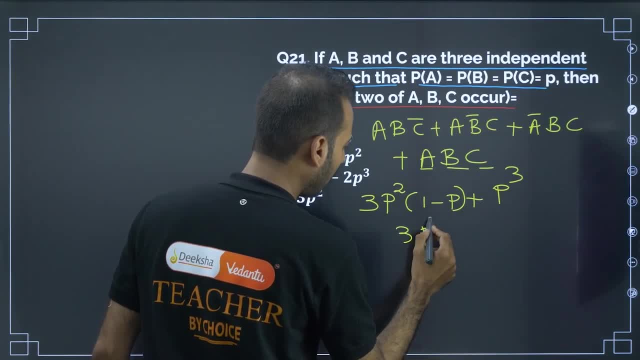 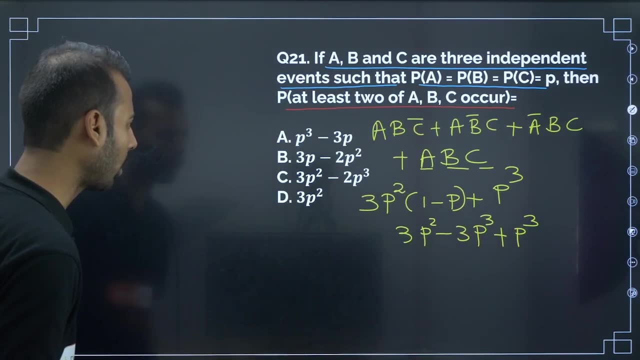 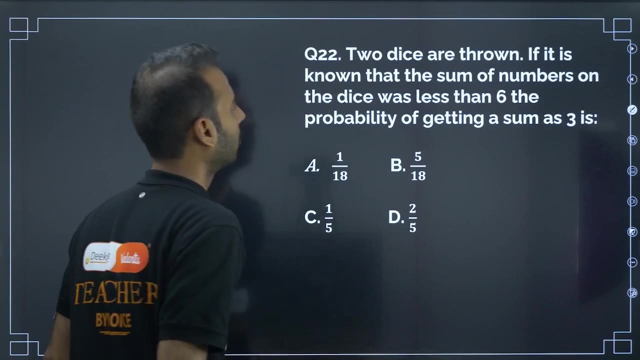 equal to p cube, so 3 p square minus 3 p cube plus p cube. so this is equal to 3 p square minus 2 p cube. C is the answer for this. Moving on to next question, two dice are thrown. 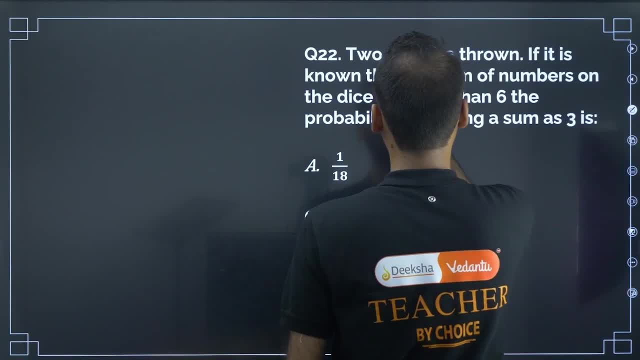 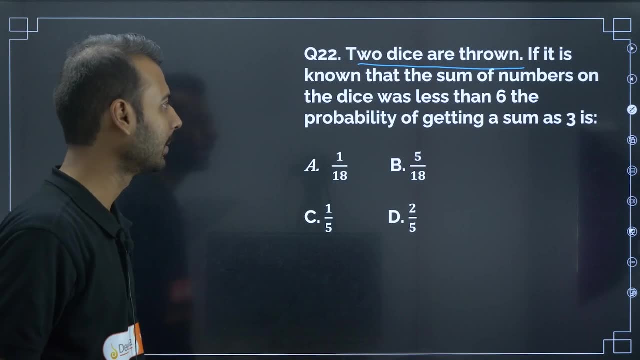 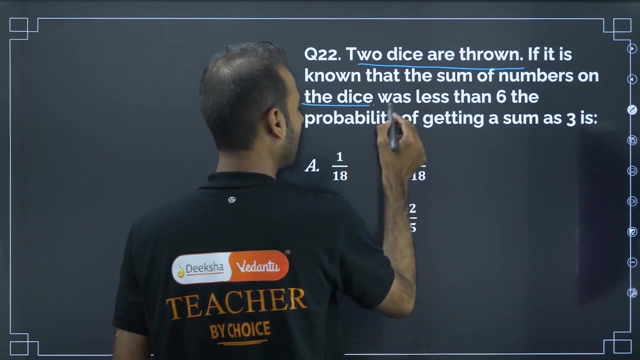 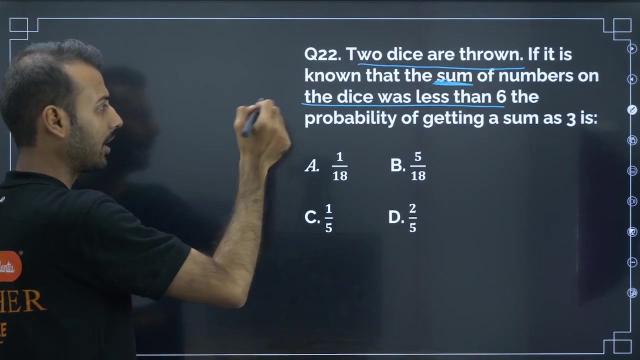 if it is known that two dice are thrown. if it is known that the number. if it is known that sum of numbers on the dice was less than 6, sum of number: the probability of getting sum as 3 is so number was less than 6, probability of sum of numbers. sum of numbers on the dice. 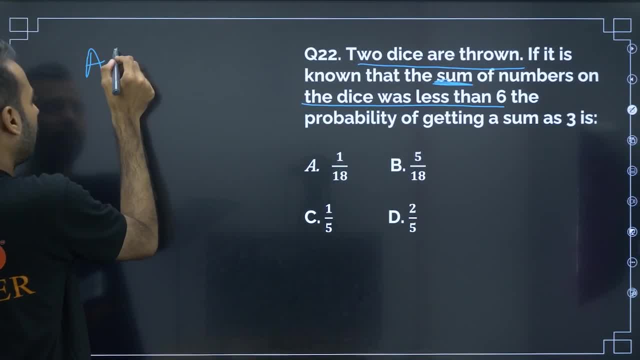 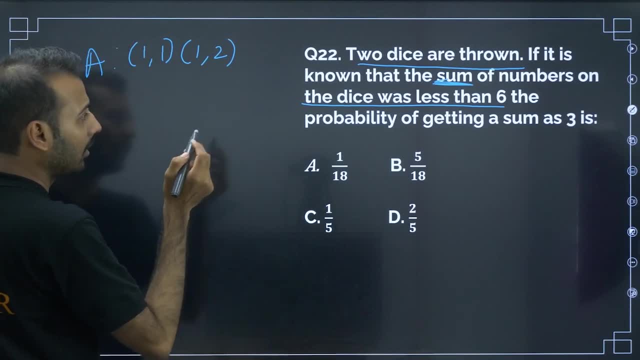 was less than 6, that means if I name that first event as the sum of numbers, then I of 1, 1, 1, 2, this will go till 1: 5. sum is less than 6. 1, 3, 1, 4, 1, 5 is was less than 6: 1- 5. if I take 1. 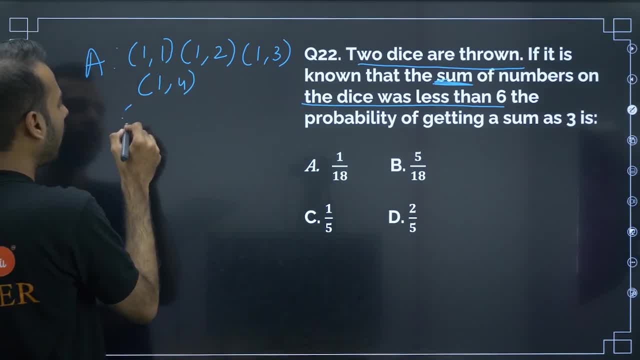 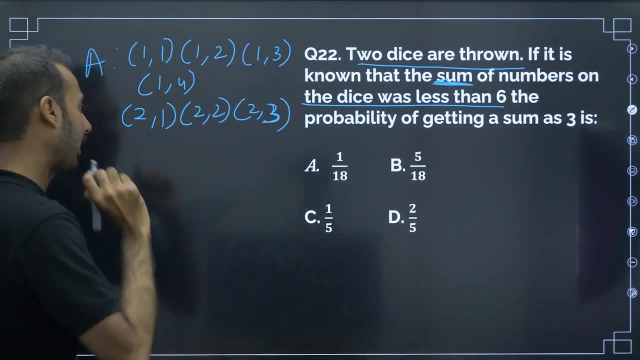 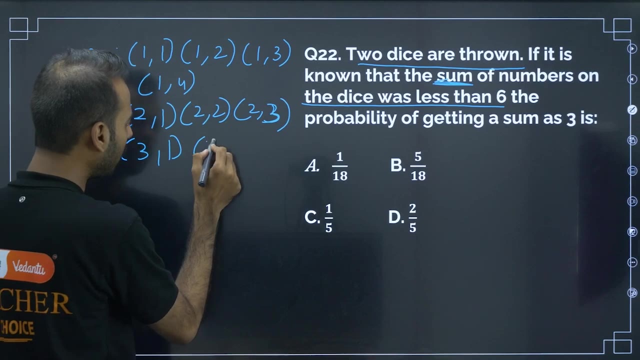 5, 6, it should be less than 6.. So I cannot consider Next: if I take 2, 1, 2, 2, 2, 3, it is ok. 2, 4, I should not take 2, 4. if I take, it will become 6.. So I cannot Next: 3, 1, 3, 2, 3, 3. 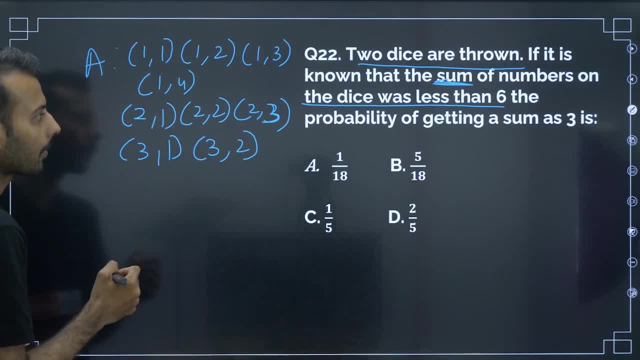 I cannot take 4 1. 4 1: yes, definitely. I can consider 4 1. yes, So 4 1. I can take 4 2. I cannot take 5 1. I cannot take the probability of getting sum as 3 if it is known that sum. 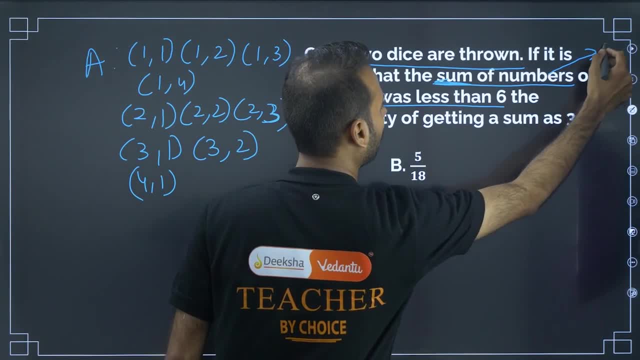 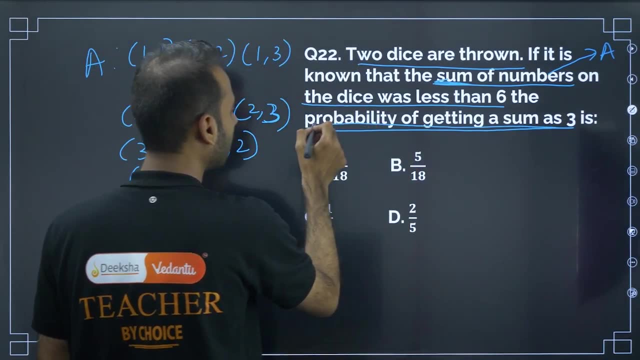 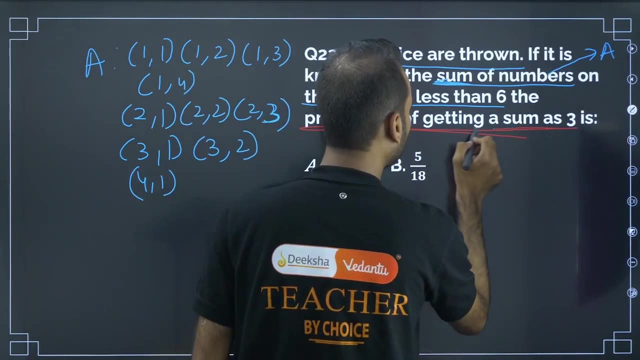 on the numbers: sum of numbers. if I am naming this as a event, If I am naming this as probability of getting a sum as 3, probability of getting sum as 3.. So what is the question? Probability of getting sum as 3 is Now let me write that if I name 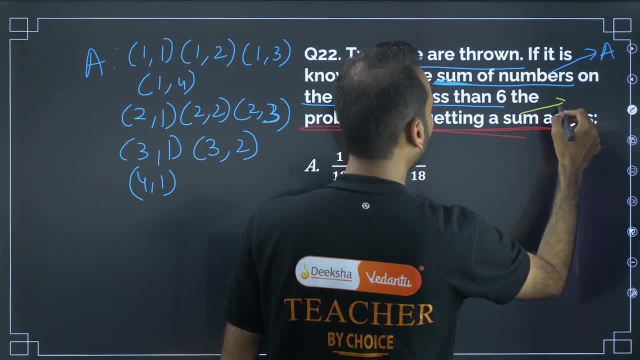 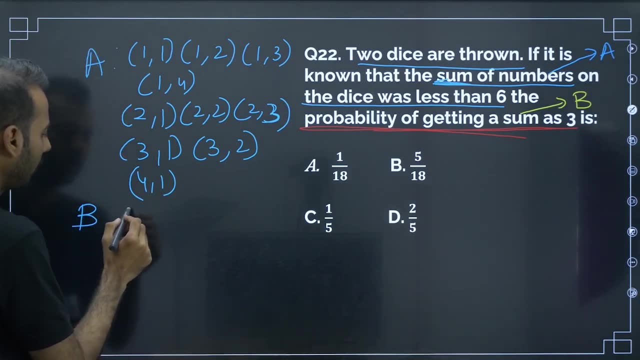 this, as if I name this as b event. then what is that? b probability of getting sum as 3 means 1, 1.. 1 sum is 3. sorry, 1, 2, 1, only this many possibilities are there. Now what is the question? Probability? 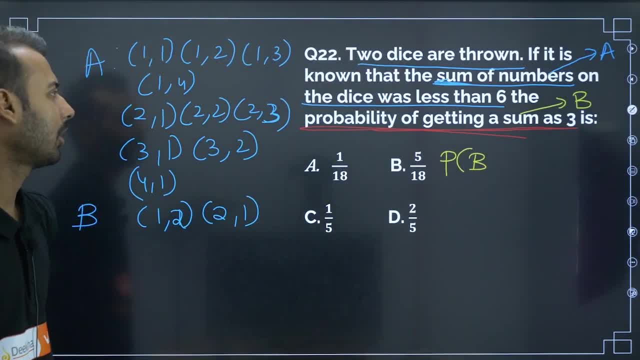 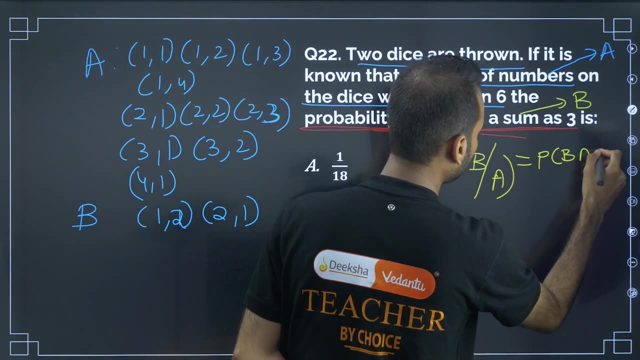 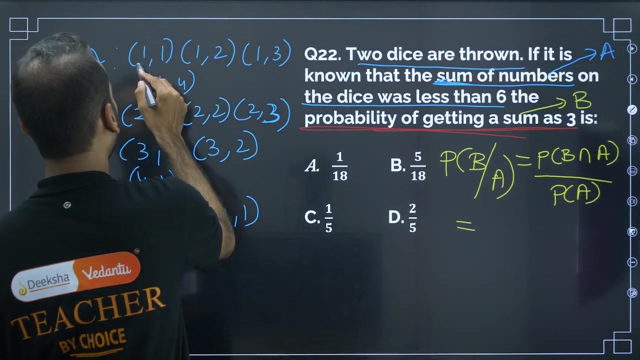 of b, 2 dice are thrown if it is known that sum of numbers on the dice was less than 6, sum as 3, given that dice was less than a. So probability of b intersection a by probability of a, Now probability of a is how much? if I count all this, 1, 2, 3, 4, 5, 6, 7, 8, 9, 10, 10 by? 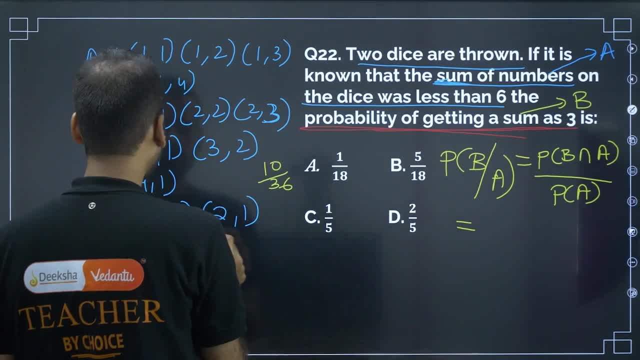 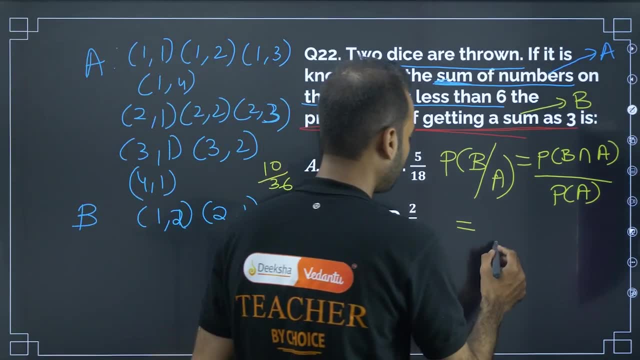 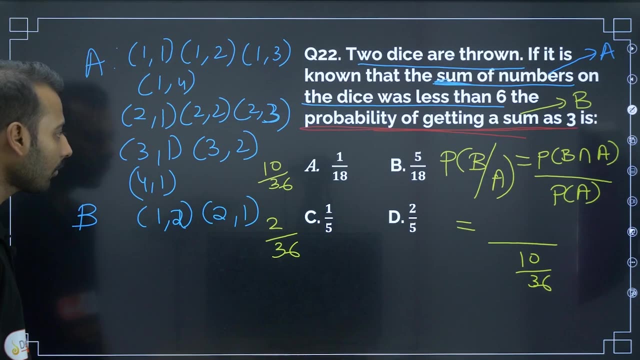 36. this is 10 by 36, this is 2 by 36.. So probability of a is 10 by 36, 10 by 36.. Probability of b intersection a is. intersection a is how much probability of b intersection a. probability of b intersection. 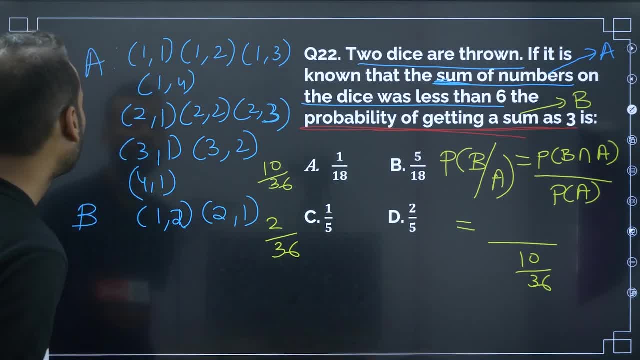 a. what is common between this and this? 1, 2, 2. 1 is common. two things are common. so 2 divided by 36, so if i cancel 1 by 5, c is the answer for this. again, easy question, within 30 seconds we can. 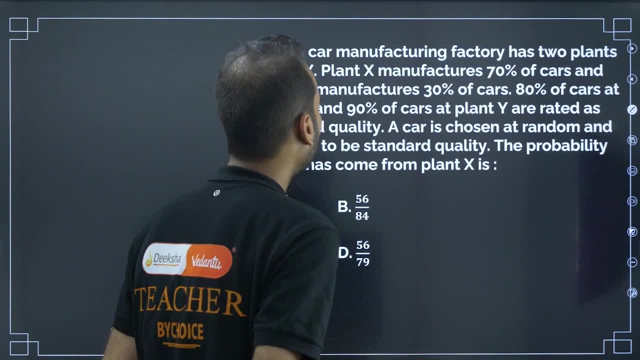 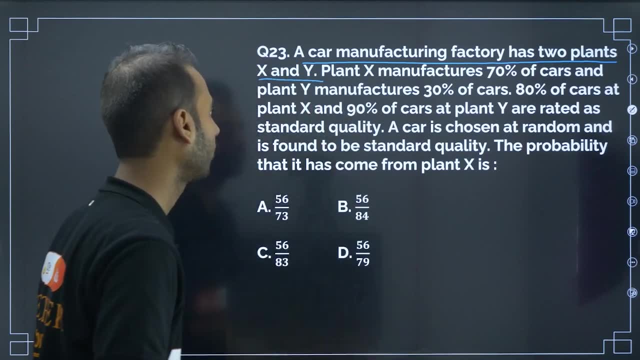 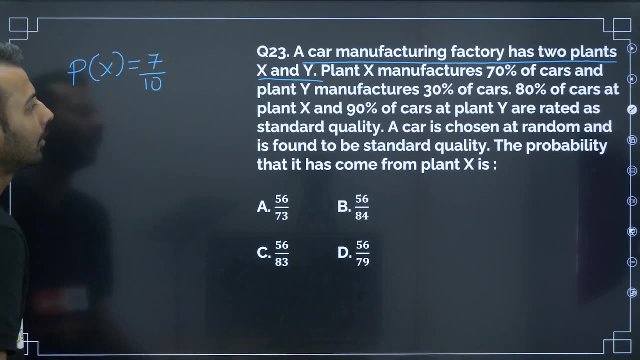 solve this. moving on to next question, a car manufacturing factory has a car manufacturing factory, as has two plants, x and y. there are two plants: plant x- manufacturers- x manufacturers- 70 percent means 7 by 10 manufacturers. and plant y- manufacturers- 30 percent, that means 3 by 10. 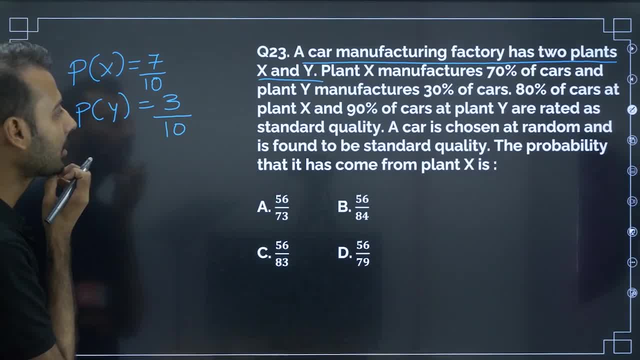 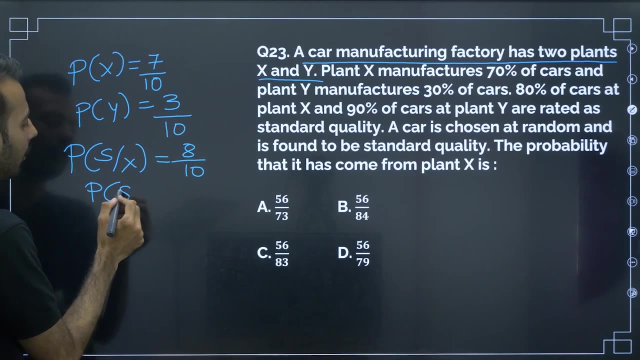 manufacturers. 80 percent of the cars at plant x and 90 are rated as standard quality, standard x. 80 percent of cars 8 by 10 and standard by y. 90 percent of the cars 9 by 10.. A car is chosen at random. so from this data, from given data, I am writing all this. 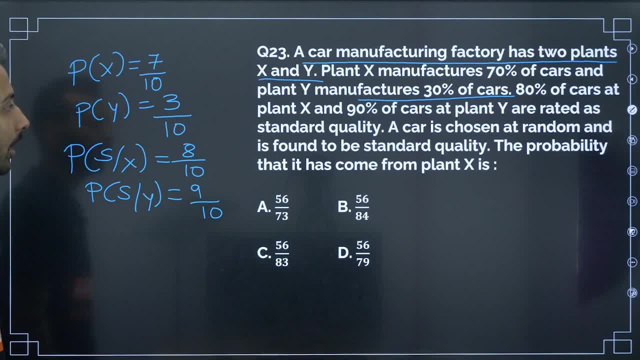 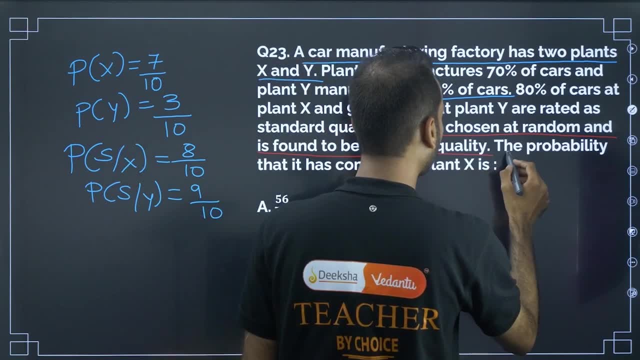 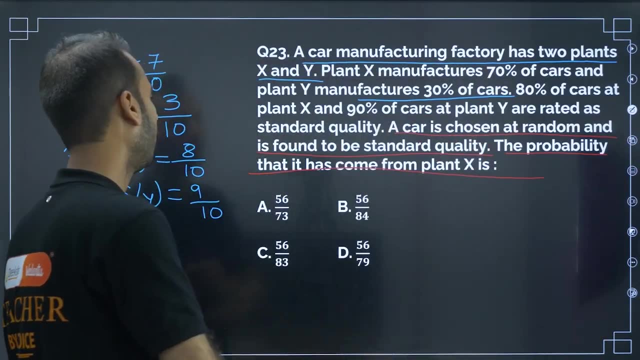 Now what random experiment they are doing. a car is chosen at random. one car they have chosen at random and is found to be standard quality: the probability that it has come from plant x's. a car is chosen at random and is found to be standard quality standard. 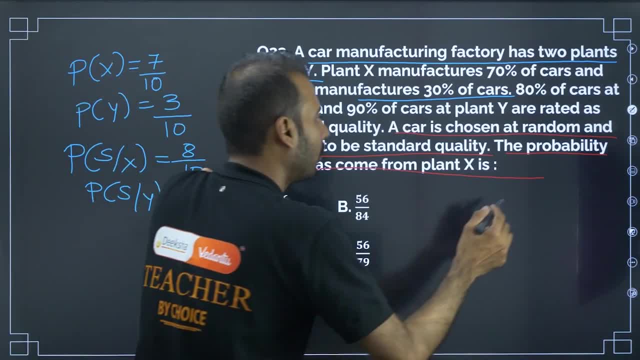 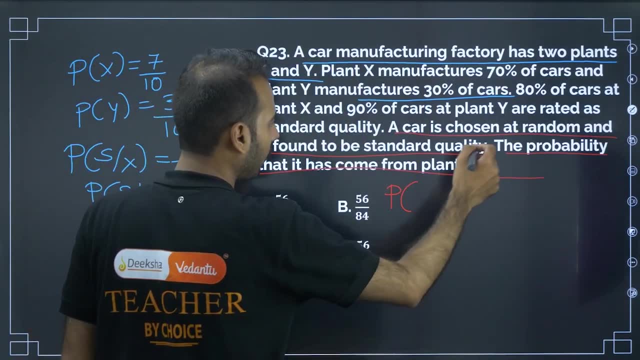 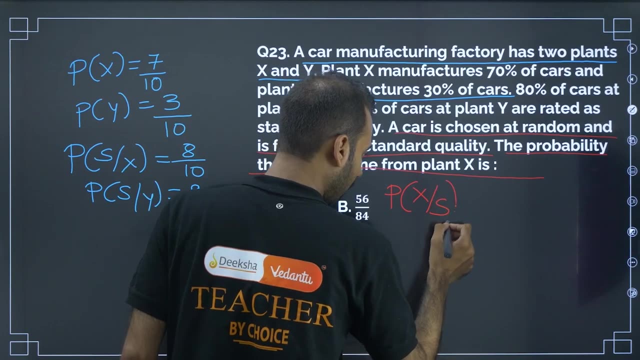 quality. The probability that it has come from plant x's from plant X is. So what are the what is the question? probability that it has come from plant X? is the probability come from plant standard quality, from, given that it is of standard quality? So this is the question. So here the probability that it has come. 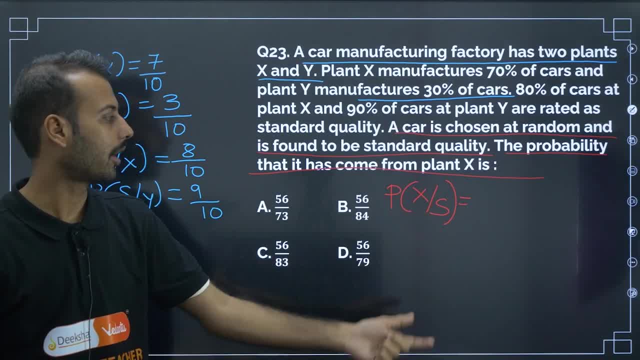 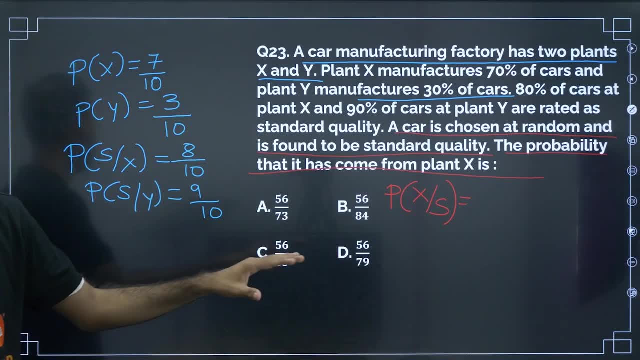 from plant X, given that it is a standard quality standard. Now, how to solve this Now with the given data? if you go through the question, everything properly, this question, we can say that it is based on Bayes theorem, reverse probability. So there are. they are asking: 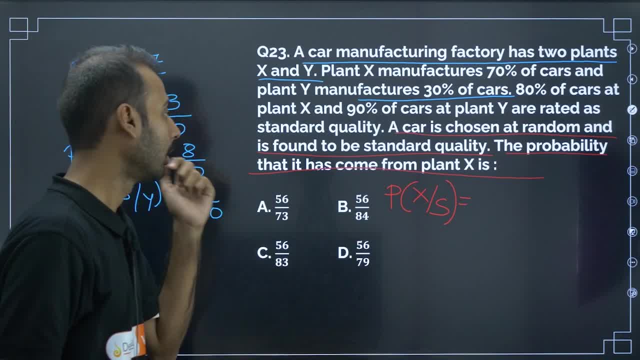 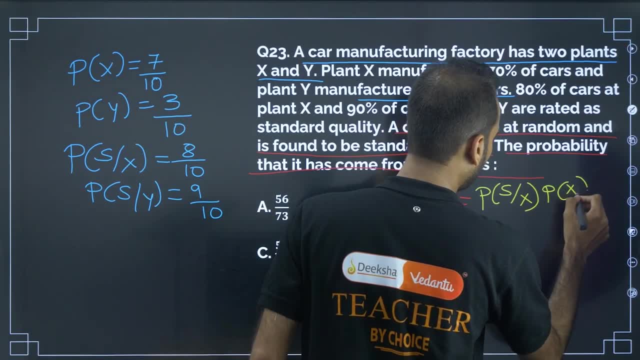 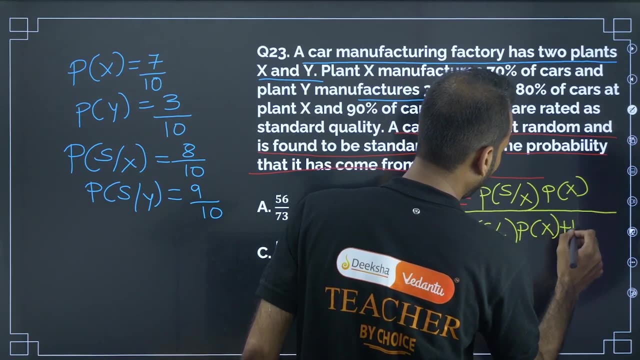 to find probability of one already, one more event has already occurred. So that is why next, Now this: if I frame, if I frame a formula for Bayes theorem: probability of X divided by probability of S given X: probability of X plus probability of S given Y, probability of X. 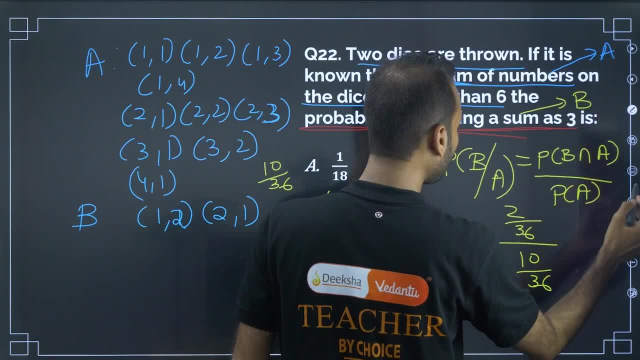 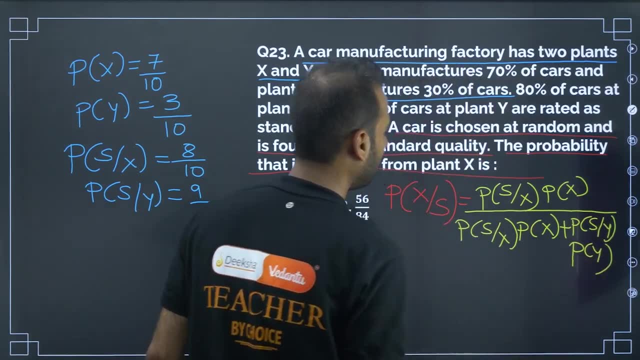 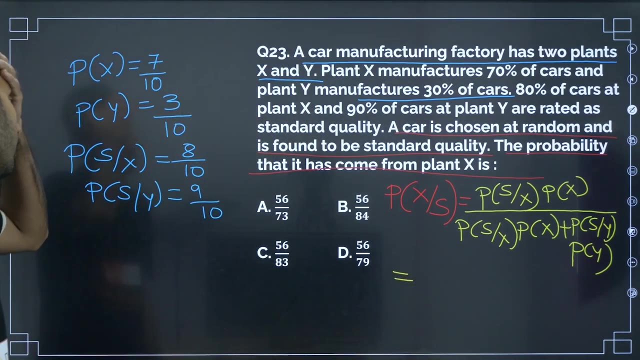 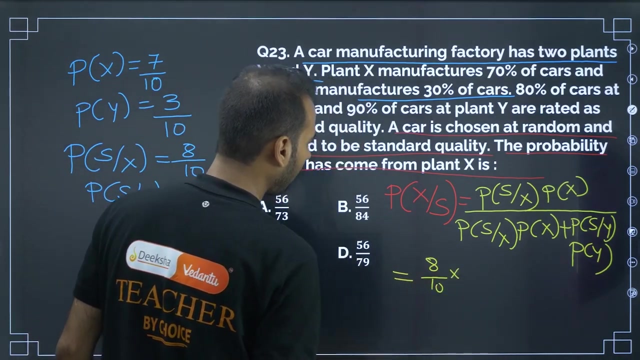 So probability of probability of. so for this probability of Y, if I frame a formula, probability of X given X is equal to probability of S given X. So probability of S given X, already all the data readily it is available, 8 by 10. probability of X is 7 by 10. 7 by 10. 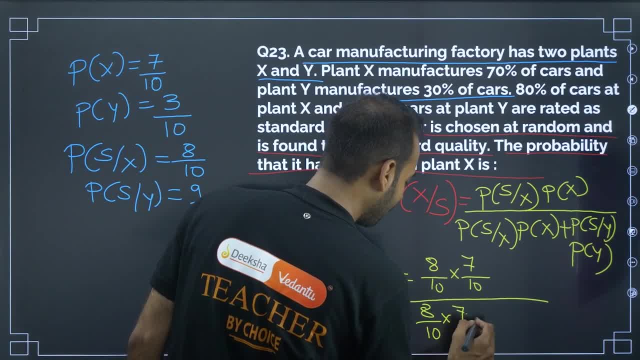 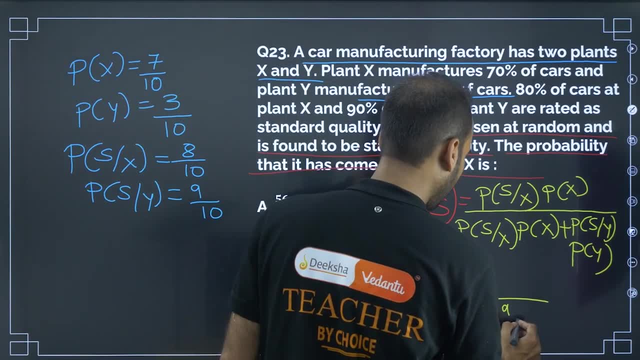 by 8 by 10.. 8 by 10, 7 by 10, 7 by 10 plus S, given Y, 9 by 10, 3 by 10, 9 by 10, 3 by 10.. So if I simplify, 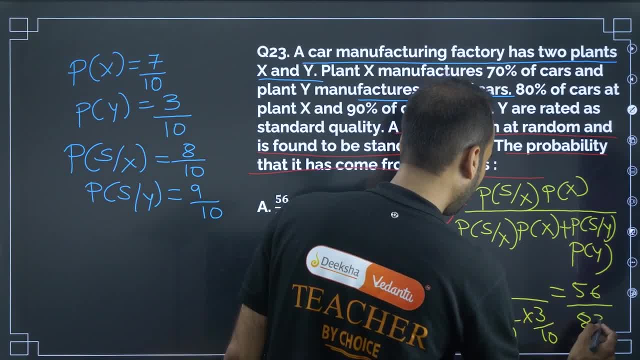 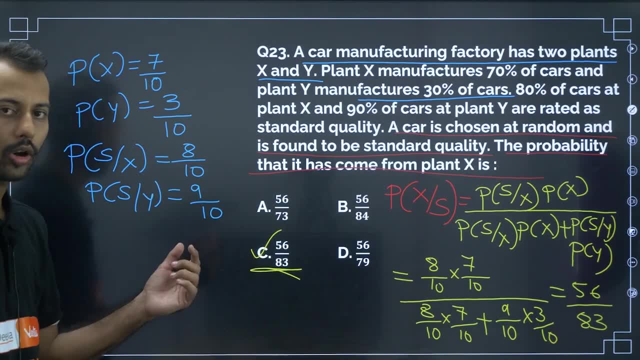 this: 7 x 56, this is 83. if I add all this, 56, 27, 83. So is there any option like 56 by 83?? Yes, C is the answer for this. Again, this problem is based on Bayes theorem, So Bayes. 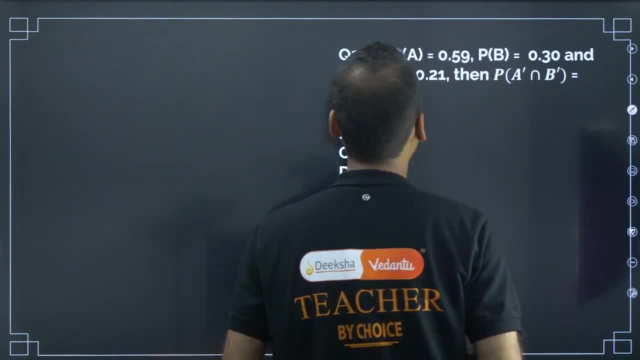 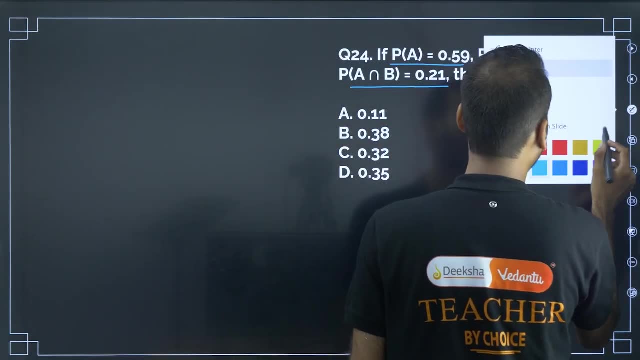 theorem is very much important. moving on to next question, If p of a is equal to some information they have given, if p of a is equal to, this must be of a is equal to and b here, then probability of A dash and b dash is what? So for this? 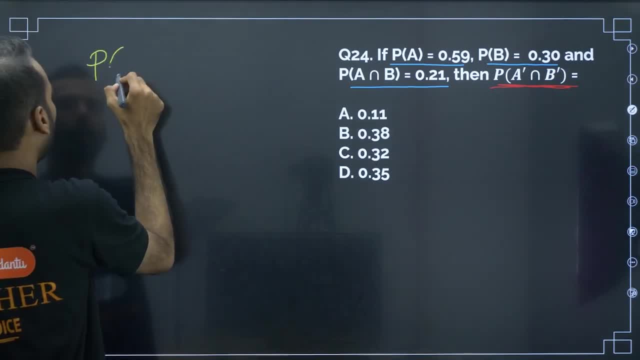 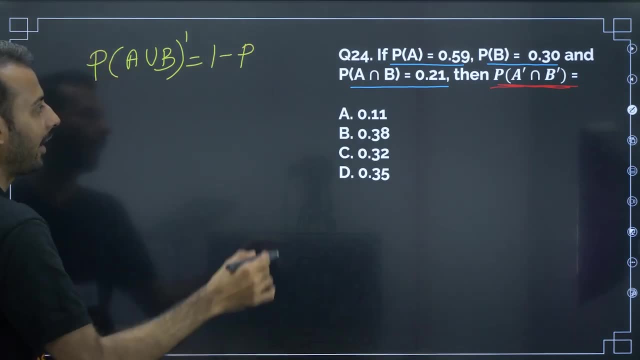 so for this probability of A union B dash is equal to 1 minus A dash. intersection B dash can be written as A union b whole dash, 1 minus probability of A union b. So if if x is greater than or equal to point c, then probably does not matter much f of a. 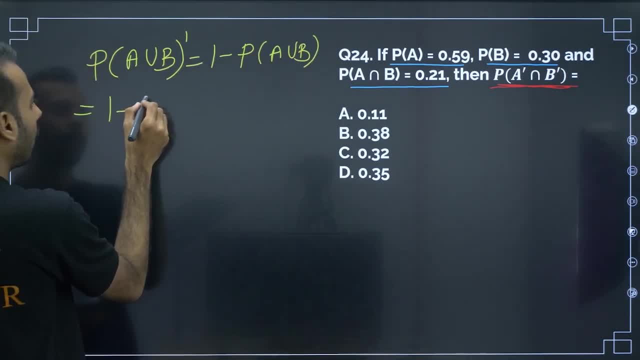 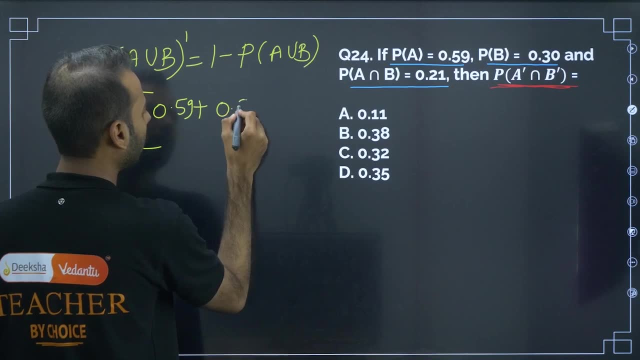 then probably is bigger than or equal to 1 minus this point c, then probably raise to Now further: 1 minus p of A is 0.59 plus probability of B is 0.3 minus A intersection B is 0.21.. 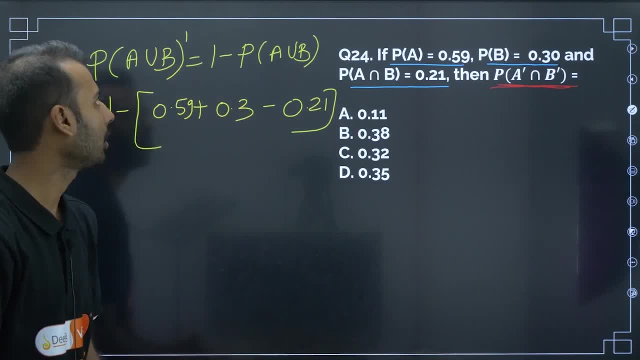 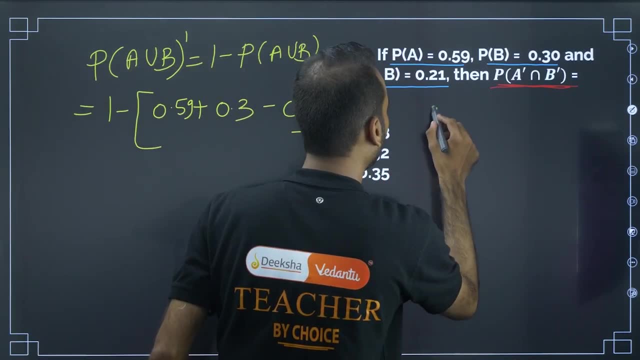 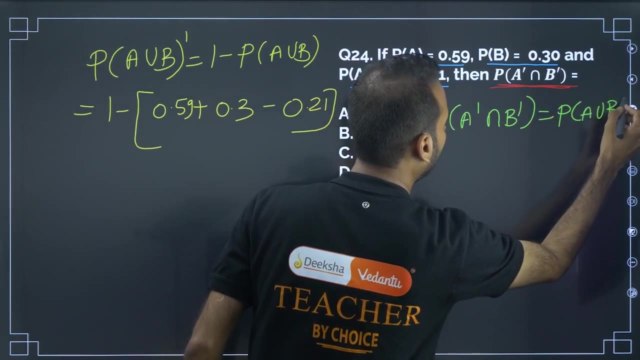 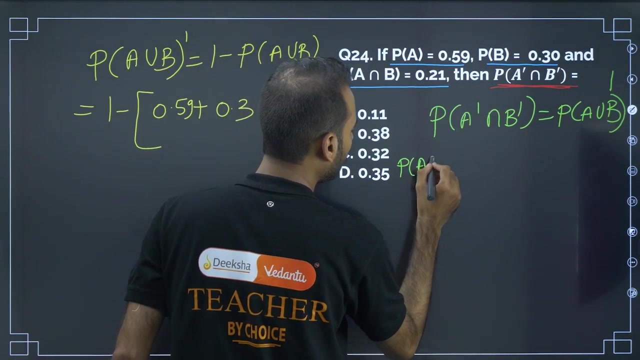 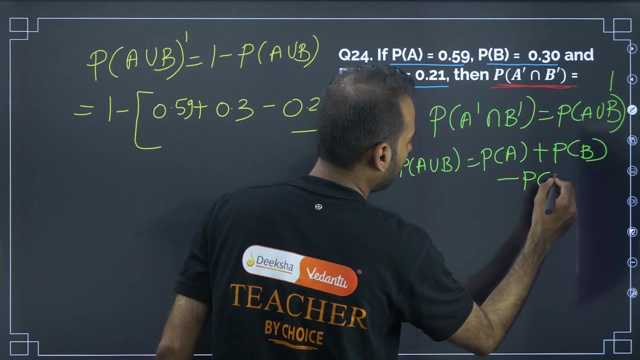 Now just some basic formulas I am using. probability of A union B dash is 1 minus this one, and probability of this formula, A dash, intersection B dash is A union B, whole dash. and then p of A union B is p of A, p of B, p of B minus p of A intersection B. Next p of A union. 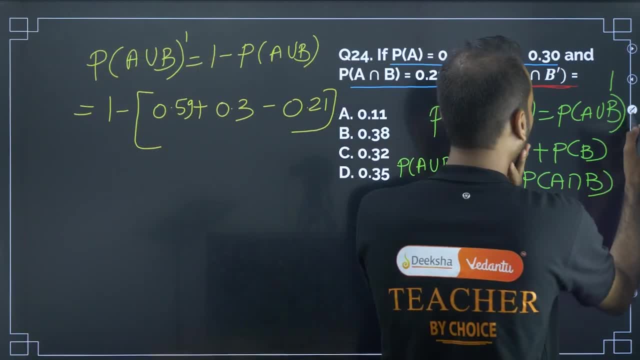 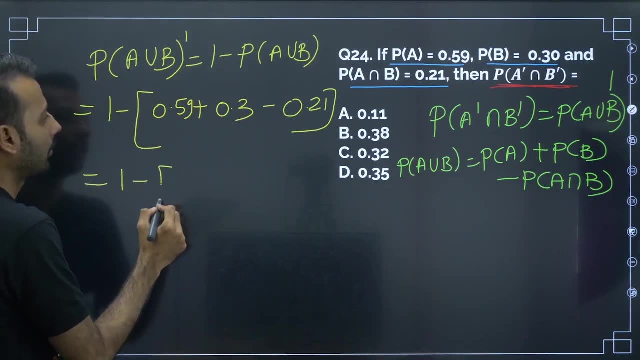 B is this much All this we have done. Now, how to simplify this? how to simplify this: 1 minus, if we solve this, all this, if I solve 1 minus 0.9, if I keep 0.59 plus 0.09, 0.09 means almost 0.68, 0.32 is the answer. 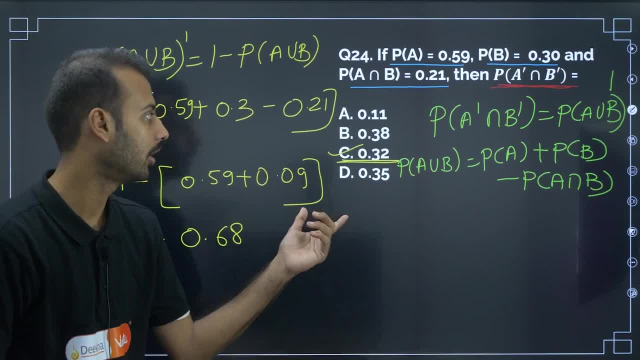 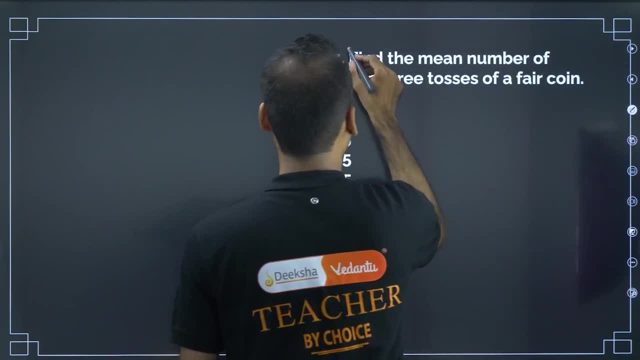 for this. Again, with basic formula, within 30 seconds we can solve this. So probability, do not leave this at any cost. Find the mean number of heads. so what are they asking? Find the mean number of head. mean number of head in how many tosses? 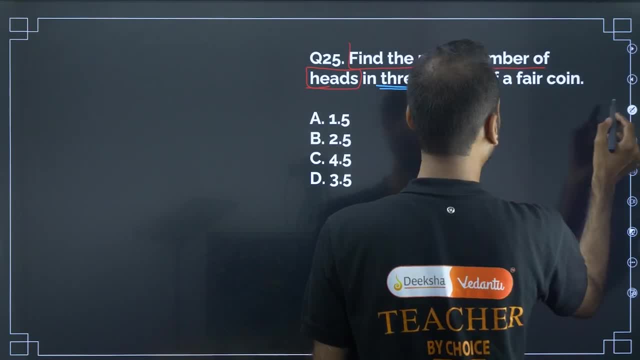 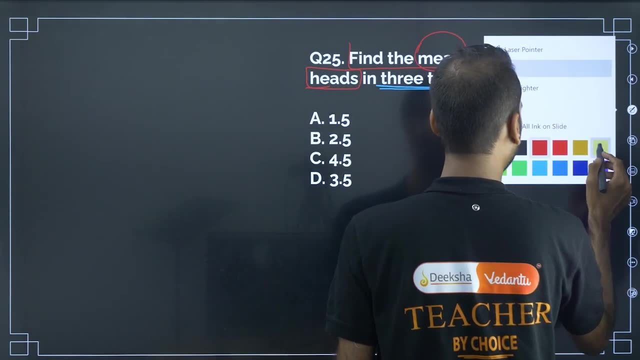 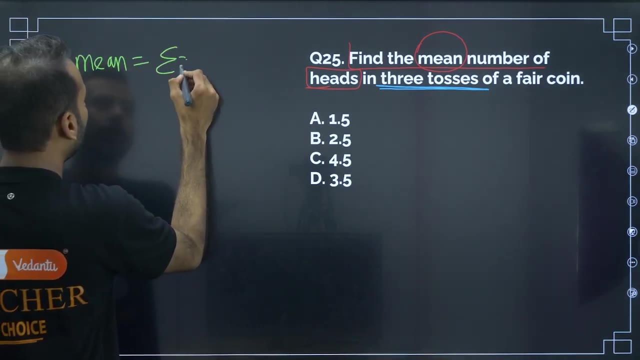 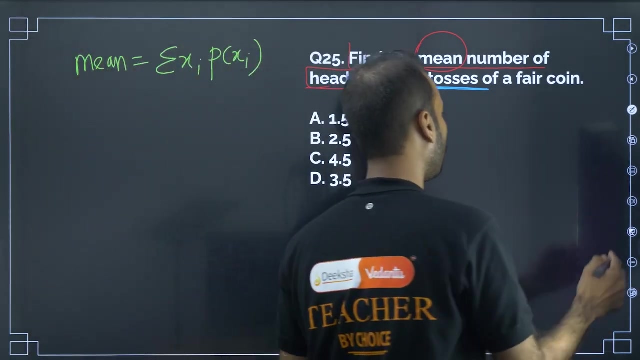 In 3 tosses of a coin. what are they asking to find? Find mean, mean, mean in 3 tosses of a coin. So mean formula. what is the formula to find? mean? Mean is equal to mean is equal to summation xi, p of xi. mean is equal to summation xi. 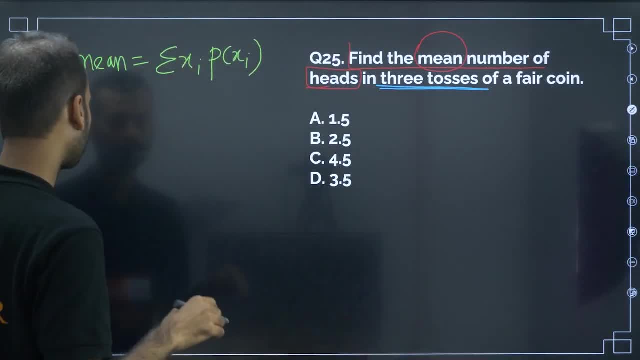 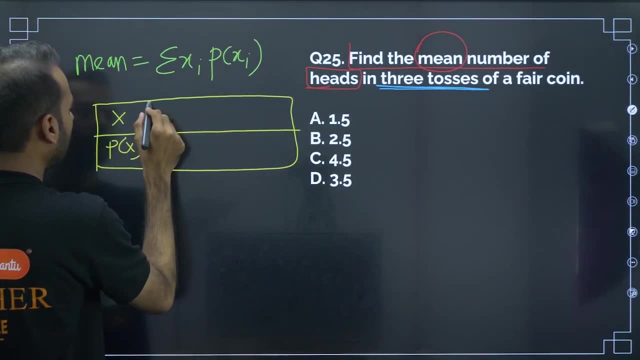 p of xi. So how to solve this problem? x? p of x. so for this: 0, 1, 2, 3, so 0, how many 1 minus 6, 1 plus 3 plus 3 minus 4 plus 3 minus 3? 8 by 8 plus 2 minus 2 by 8 by 8 plus 1 minus. 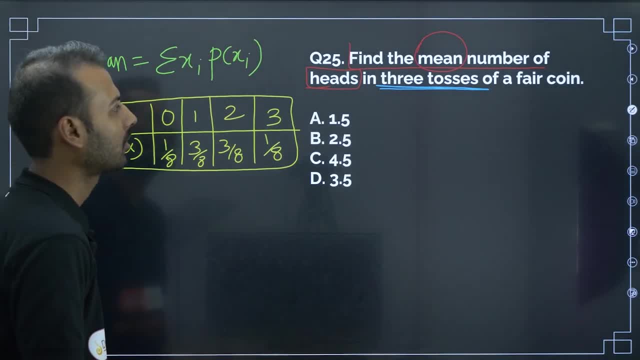 3, find the mean number of heads. find the mean number of heads in places, fair coin. find the mean number of head. So this is x, which is xi, this is xi if I name this as xi. So if I take this: 3 by 8 plus 6 by 8 plus 3 by 8. So which is equal to: 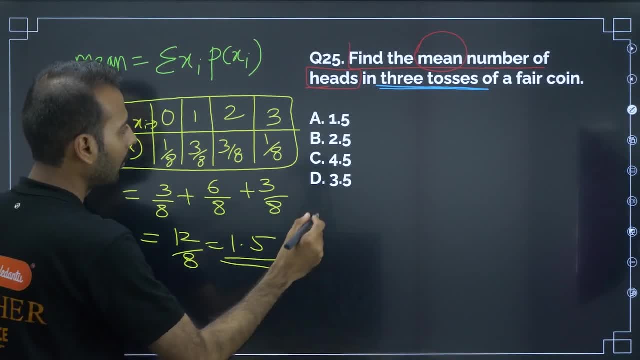 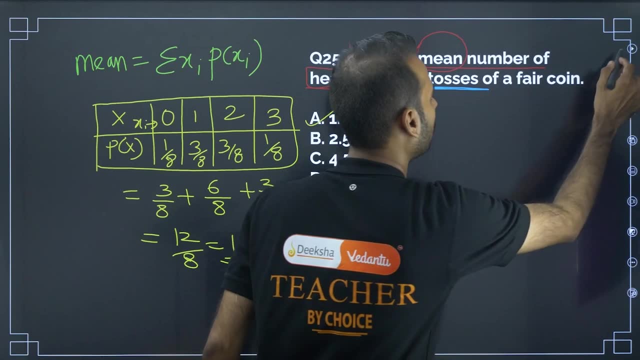 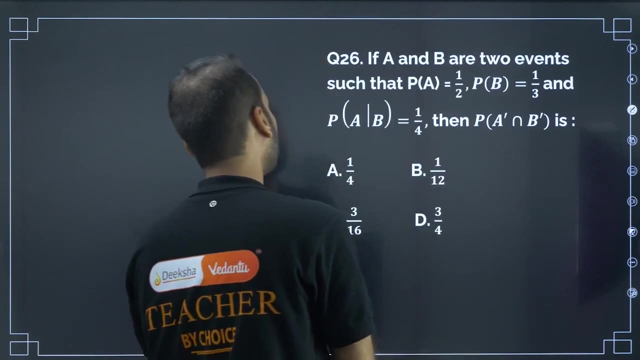 12 by 8 is equal to 1.5.. So answer is 1.5. very easy question, only this much hardly. it will take 30 seconds to solve this. moving on to next question, If a and b are 2 events, what are they? a and b are two events such that h p of a is equal. 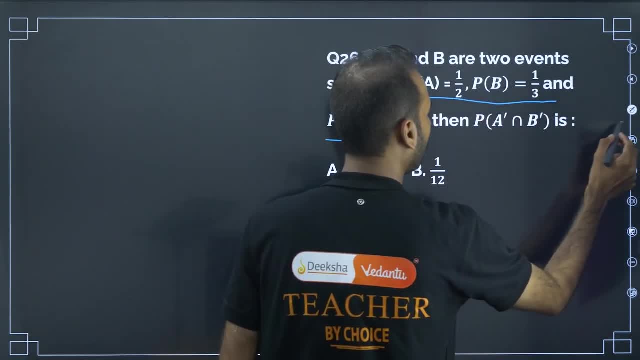 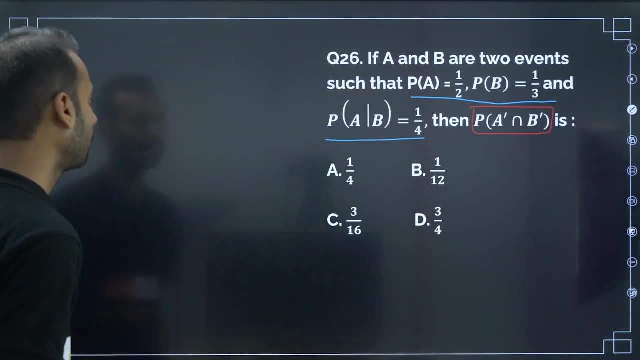 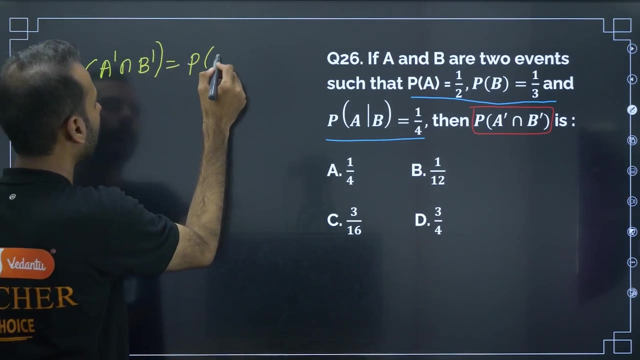 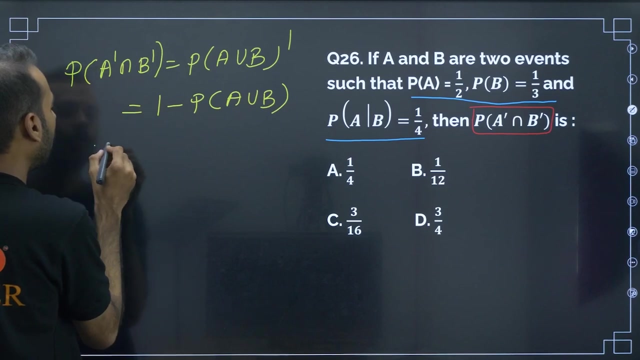 to this much and a p of a. then what are they asking? See here this focus on this. they are asking this: So how to solve this Probability of a dash intersection, b dash intersection? So we would think that is equal to probability of A union B dash which is equal to 1 minus B, equal to 1 minus. 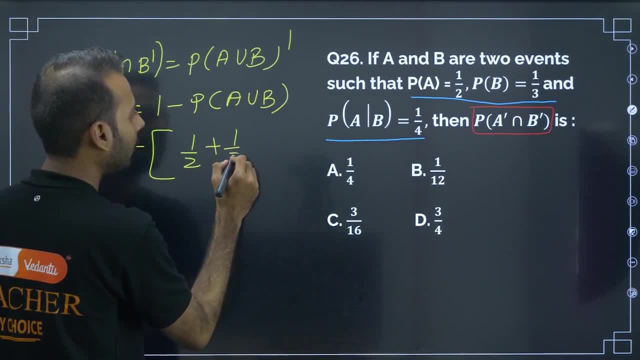 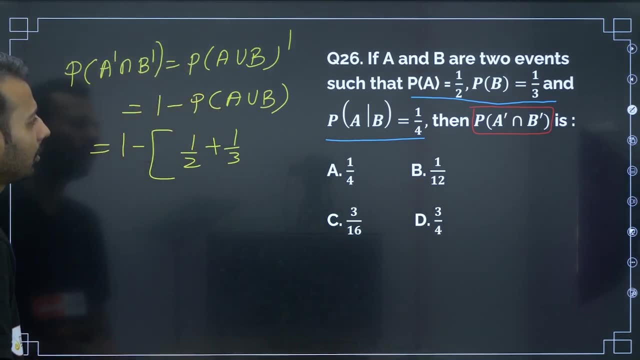 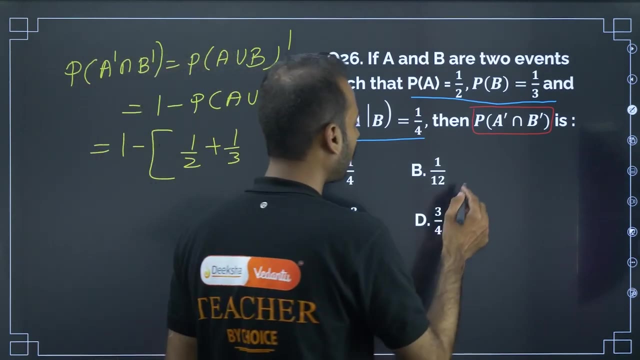 p of A union B is p of A plus p of B minus p of A intersection B. What is p of A intersection B: 1 minus p of A union B is 1 minus A intersection B. A intersection B is not available readily. 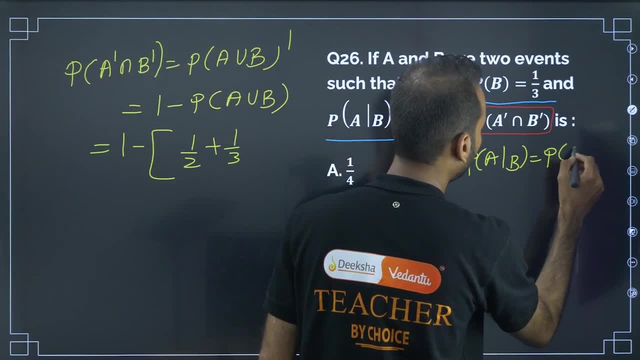 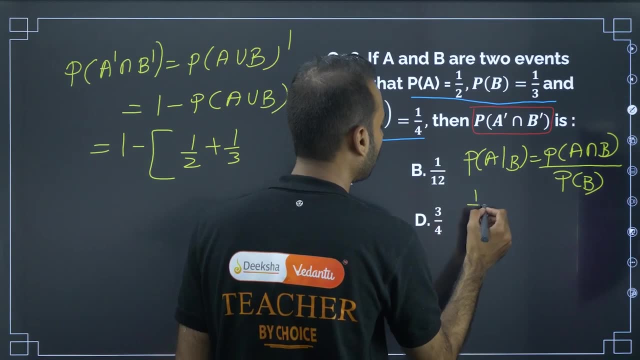 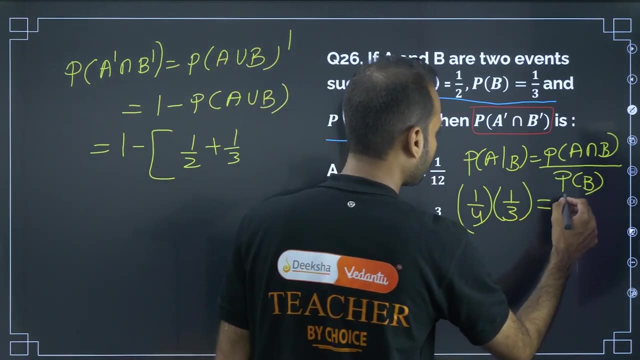 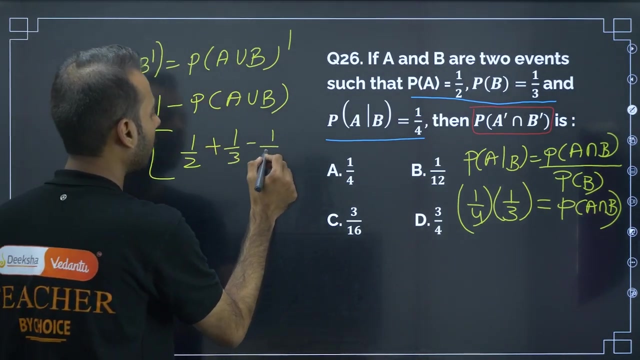 so probability of A given B is equal to probability of A intersection B by probability of B. So probability of A intersection B is 1 by 4, probability of B is 1 by 3, probability of A intersection B is not. Now, this is 1 by 12.. So if I go for simplification, 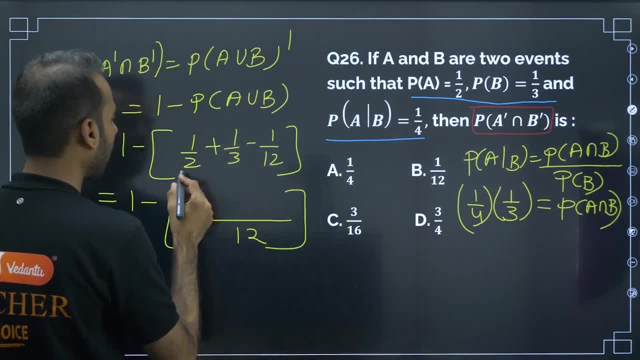 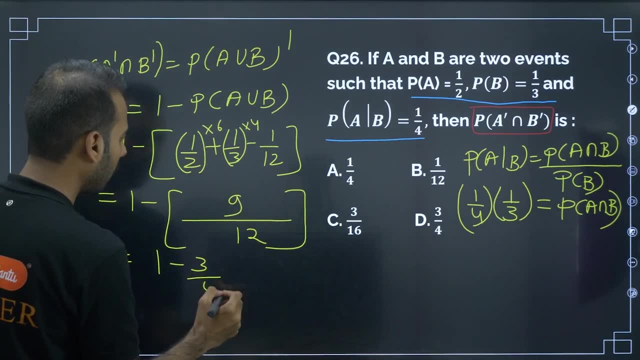 1 minus here it is 2 L. If I take calcium into 6 into 4, 9 by 12, 1 minus 3 by 4 is equal to 1 by 4.. So is there any such option? 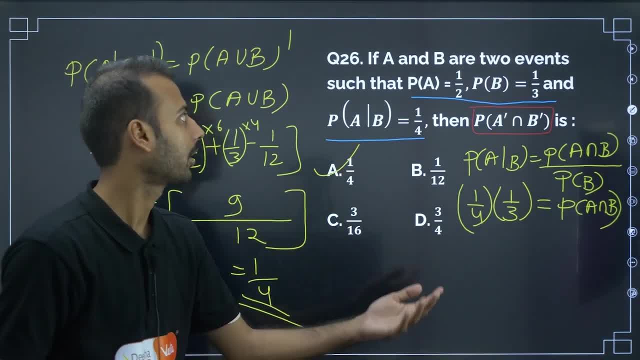 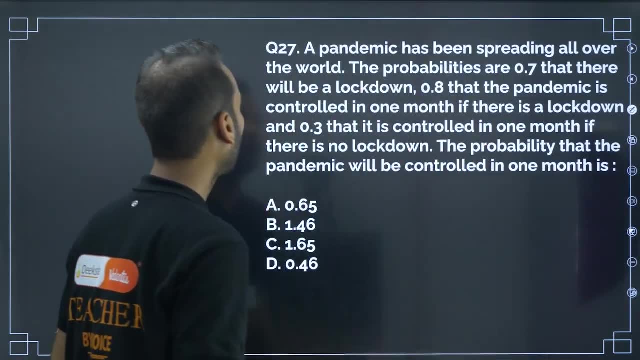 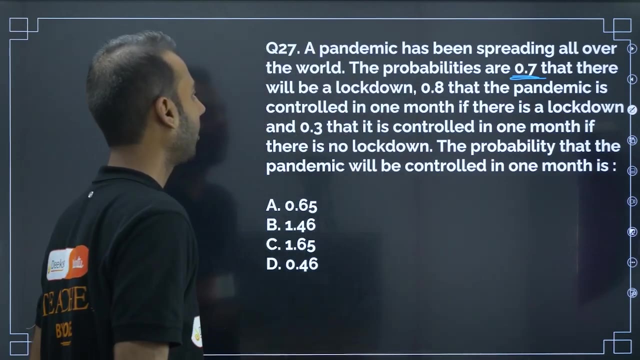 This is the answer. Again, easy question, hardly 30 seconds to solve this. Moving on to next question: A pandemic has been spreading. a pandemic has been spreading all over the world. pandemic has been. The probabilities are 0.7 that there will be a lockdown. probability of lockdown is: 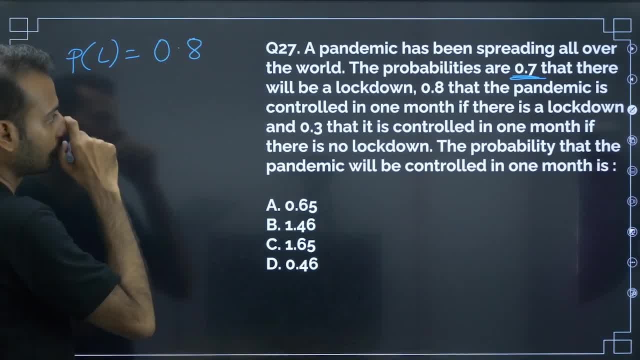 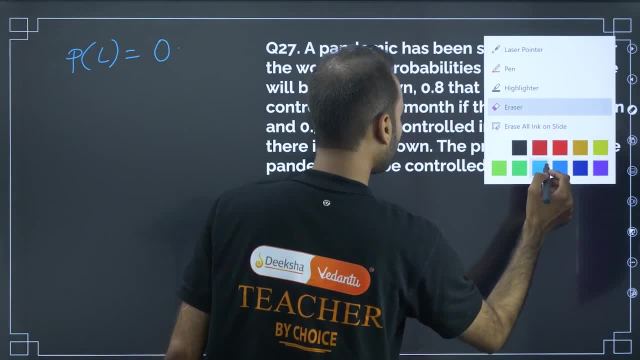 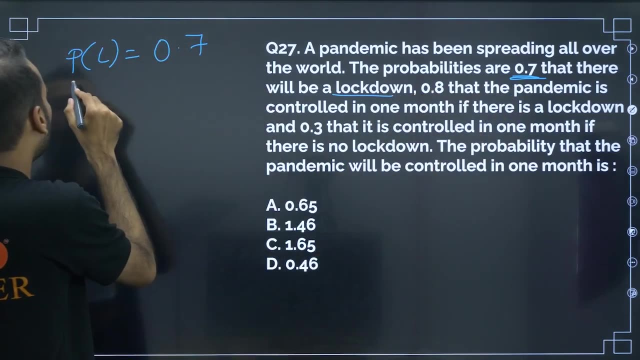 0.8, sorry, sorry, sorry, 0.7,. probability of 0.7, there will be a lockdown: lockdown: 0.7, no lockdown. no lockdown 0.8, 0.3.. 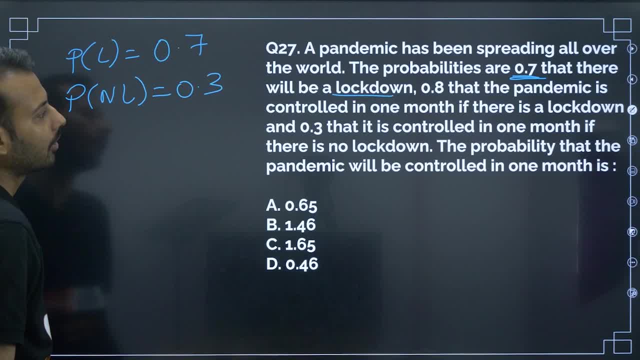 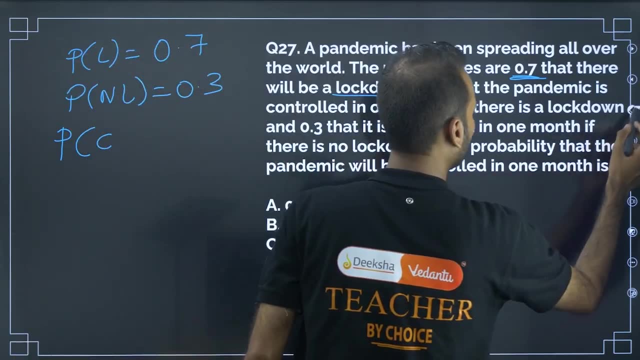 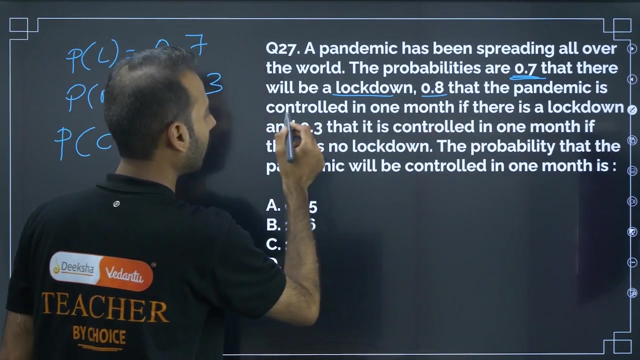 Lockdown. 0.7 means no lockdown. 0.3, 0.8. pandemic is controlled in one month. controlled in one month if there is a lockdown. So next point: you observe 0.8, that pandemic is controlled in one month if there is a lockdown. 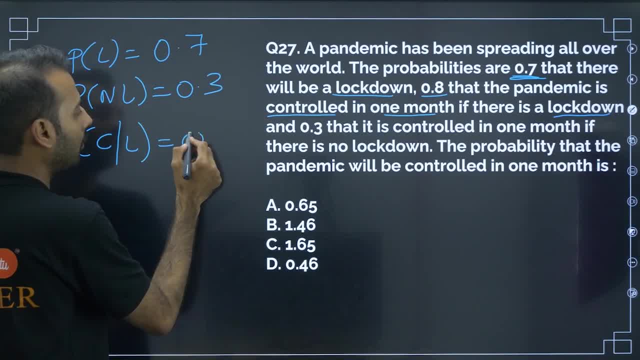 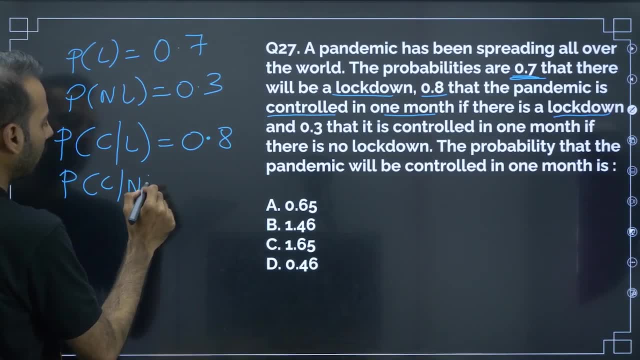 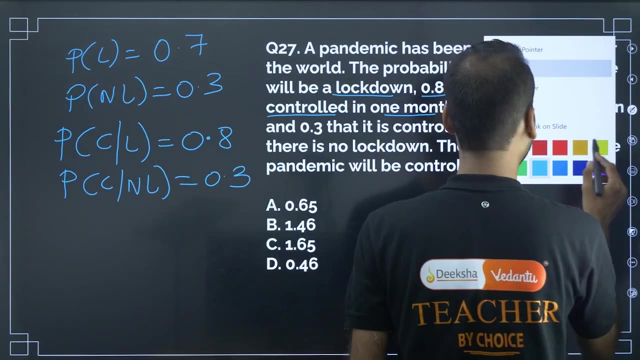 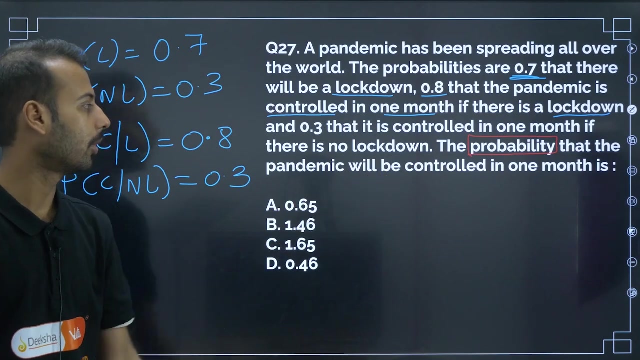 So controlled, given there is a lockdown, Lockdown is 0.8 and 0.controlled- no lockdown: 0.3, no lockdown. The probability that now go through the question, the probability that pandemic will be controlled in one month, the probability that pandemic will be controlled in one month, is so what? 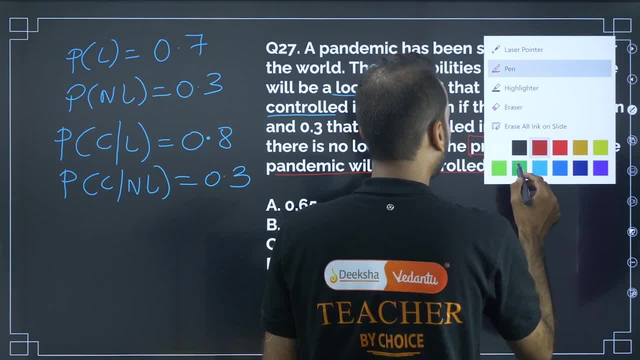 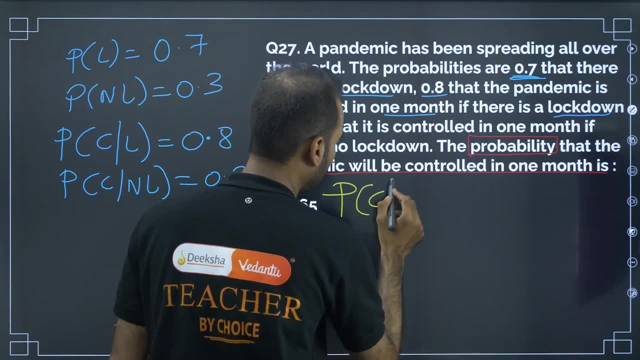 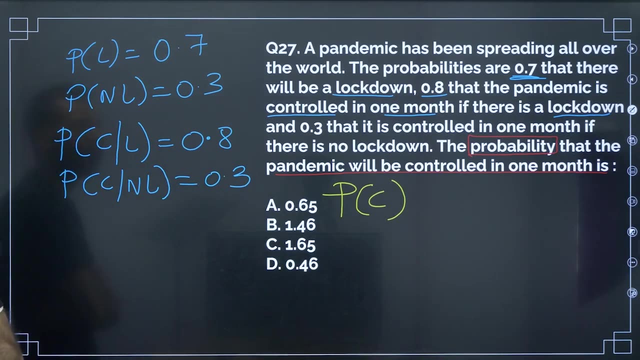 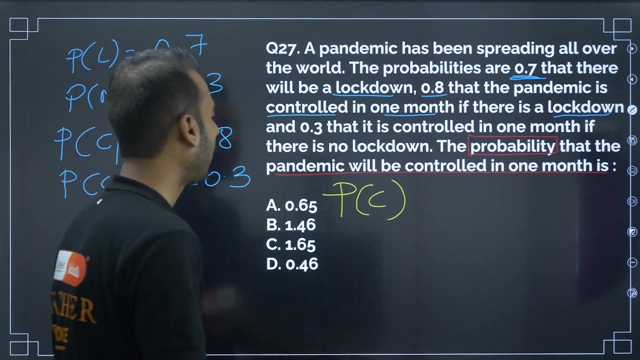 is the question. So the question is probability that pandemic will be controlled. controlled in one month. pandemic will be controlled in. pandemic will be controlled in one month. So probability of controlled in one month. Now, with the given data available, I can write total probability. probability of c given. 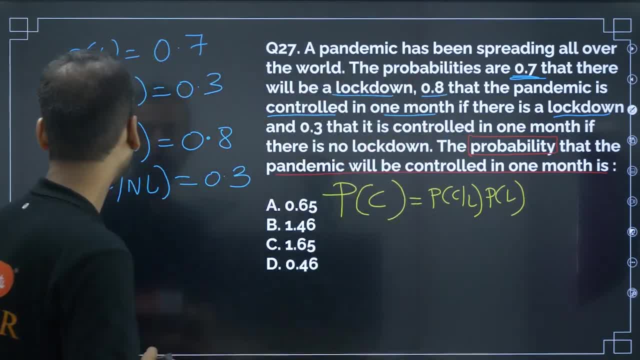 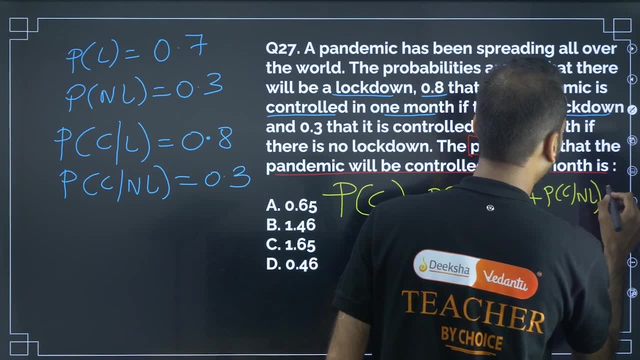 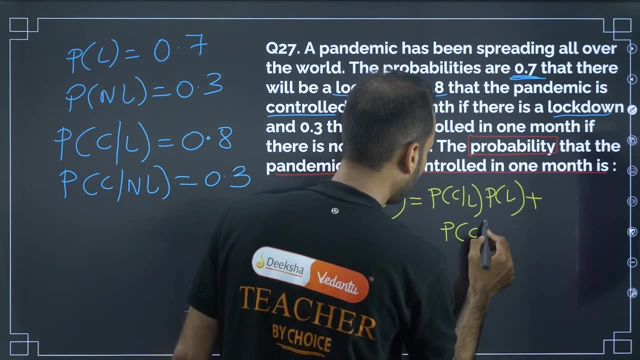 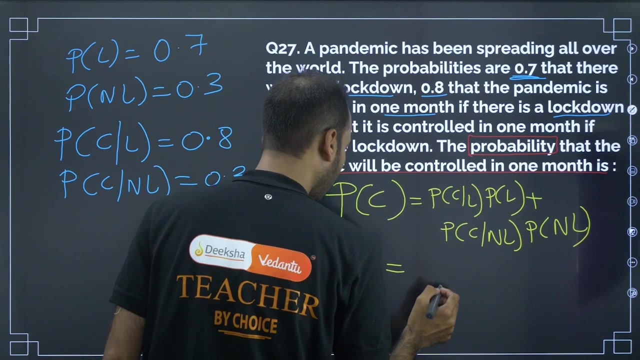 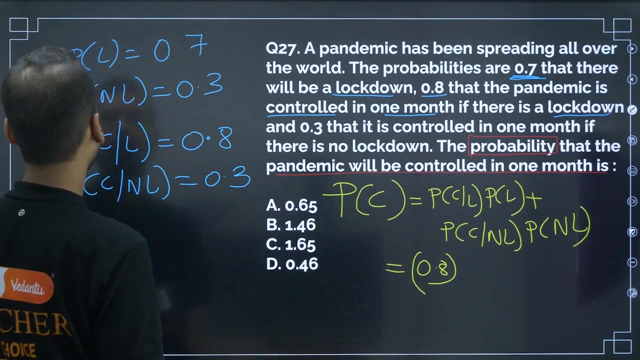 Lprobability of L. Can we be Now with this? we can write op. it is at L, Next N L. probability of C given N L dot probability of N L plus probability of C N L probability of N L. So probability of C given L is how much? 0.8, 0. point lockdown. 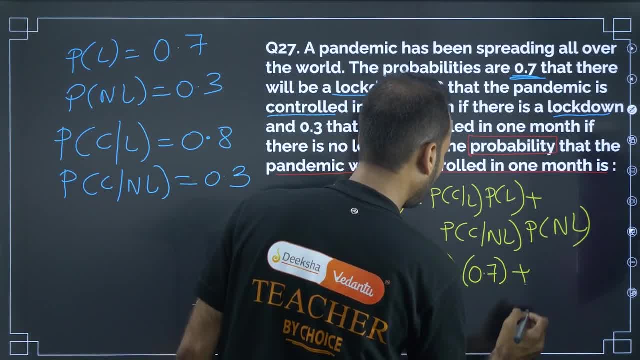 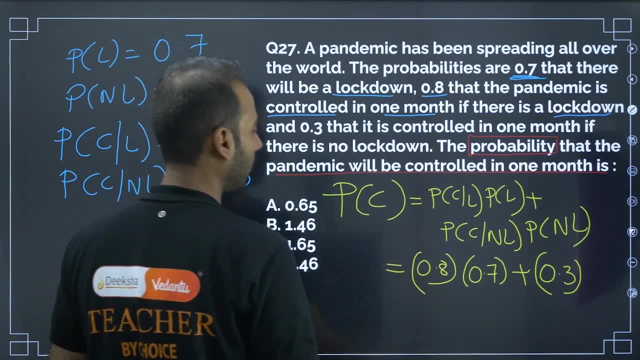 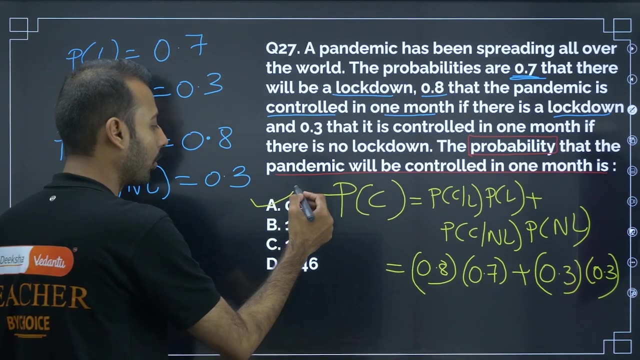 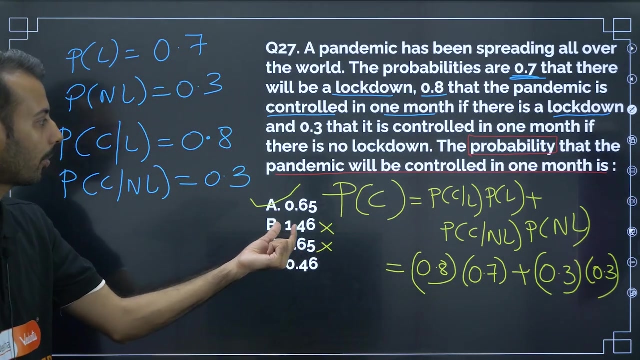 0.7, C given N L. C given N L 0.3, N L N L 0.3.. So if I multiply, if I simplify everything, I will get 0.65 as the answer. In any worst case. you should never, because probability. 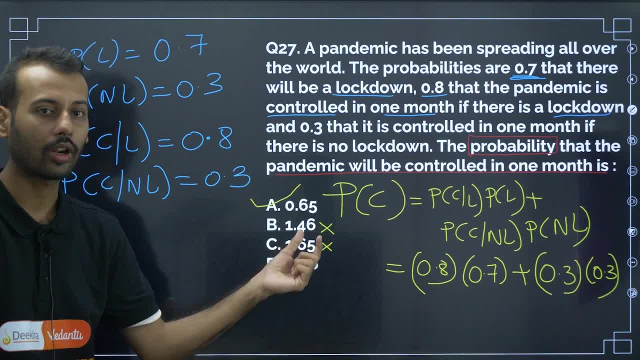 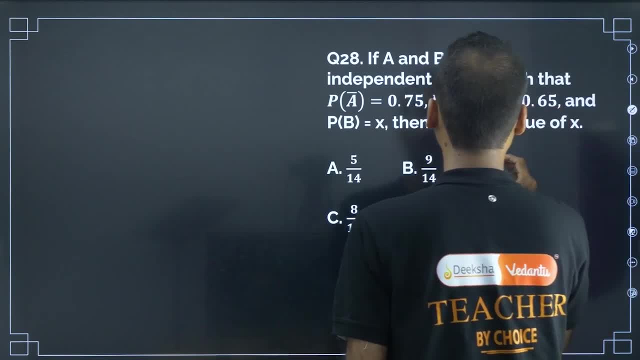 they are talking about probability and they are talking about more than one. How probability will be low. More than one? Not possible, not possible, So do not Next. moving on to next, If A and B are, if A and B are two events or independent events, such that P of A is this much, P of 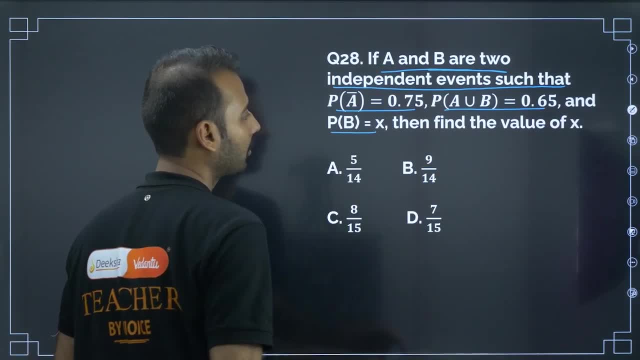 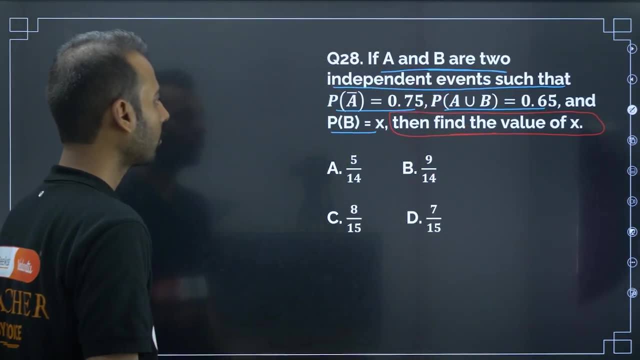 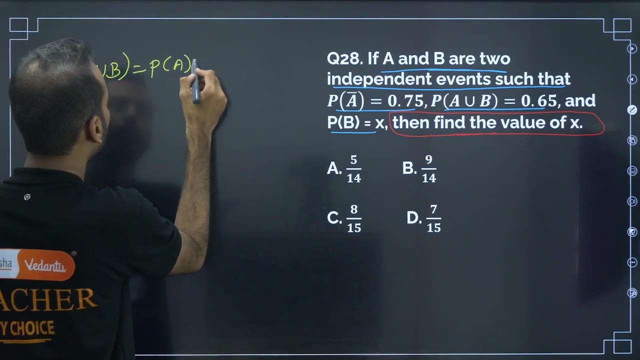 A union B is this much and P of B is equal to this much. then what are they asking? to find a value of x, Find a value of x. So P of A union B is equal to A. union B is equal to P of A plus. 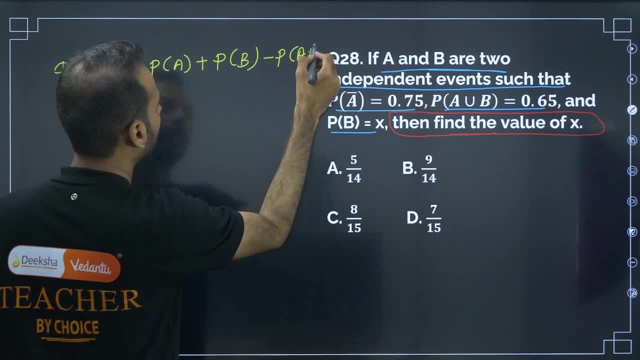 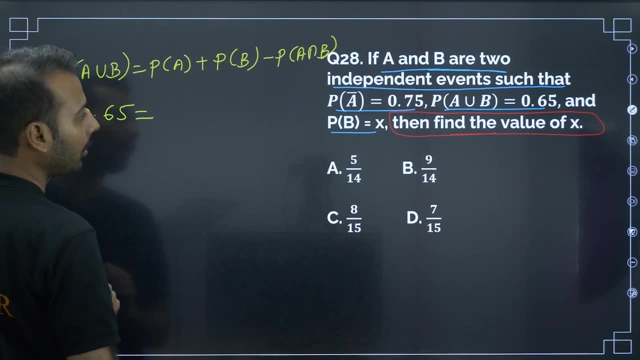 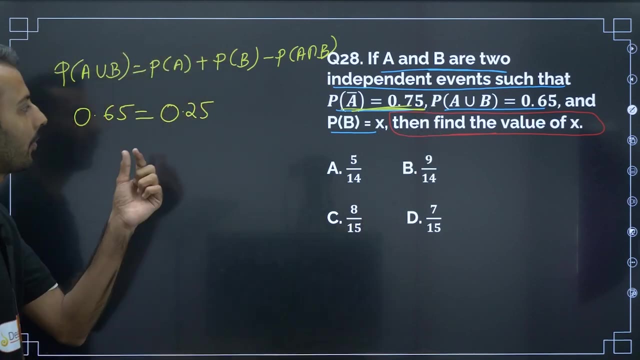 P of B minus P of A, intersection B. Now P of A, union B is 0.65, P of A is: P of A is 0.25.. See here: P of this is this much, So P of A will be 0.25.. Next, P of B is x minus. 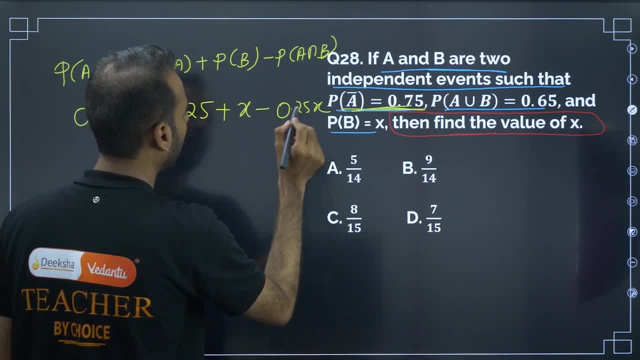 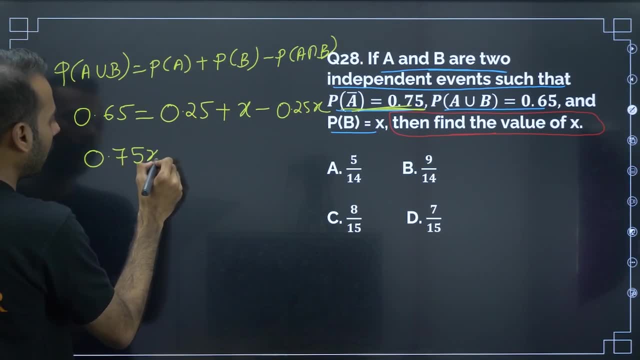 0.25, 0.25 x. Now, if I transpose that- this side, So this is this much. So if I transpose this becomes 0.75, x is equal to 0.4.. Next, if I simplify, x is equal to 8 by 15, x is equal. 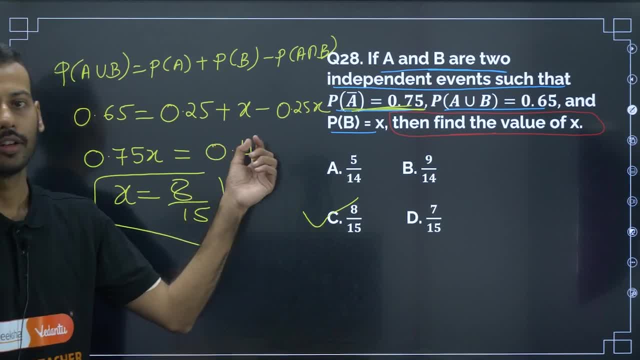 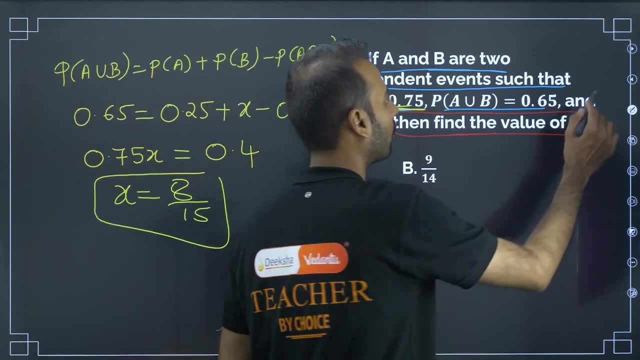 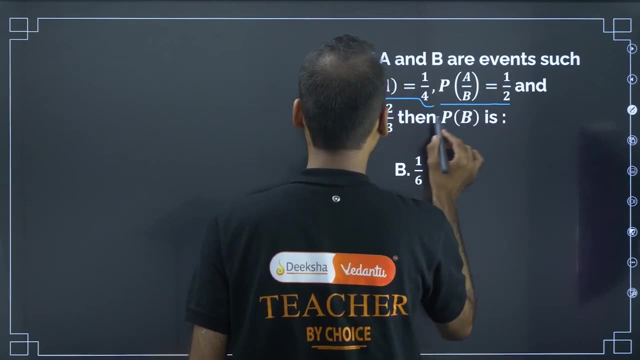 to 8 by 15.. So C is the answer for this, again only based on one theorem. So easy question, only hardly, hardly. it will take 15 seconds to solve this. Moving on to next question, if A and B are events such that P of A is this much, P of A given B, and then P of B is: 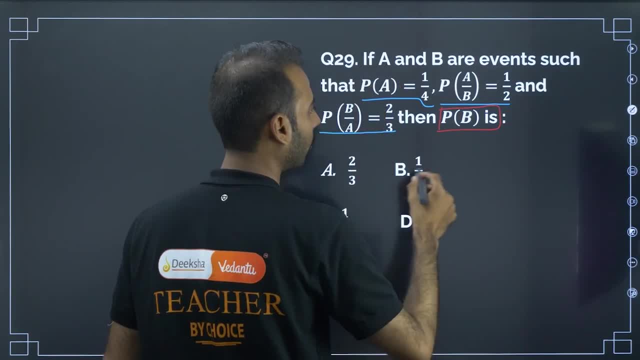 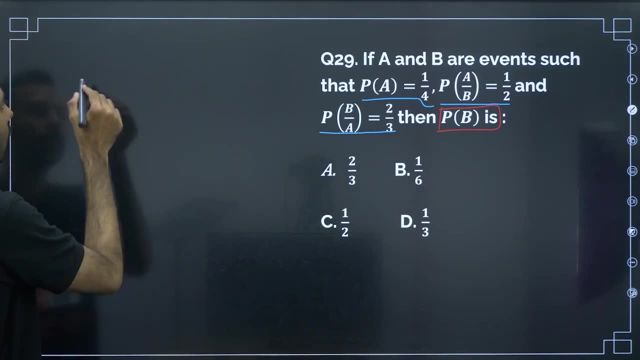 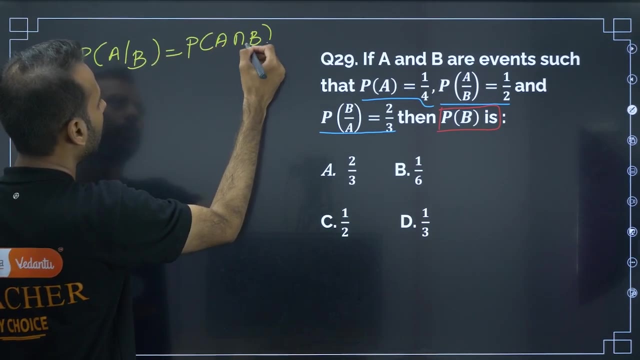 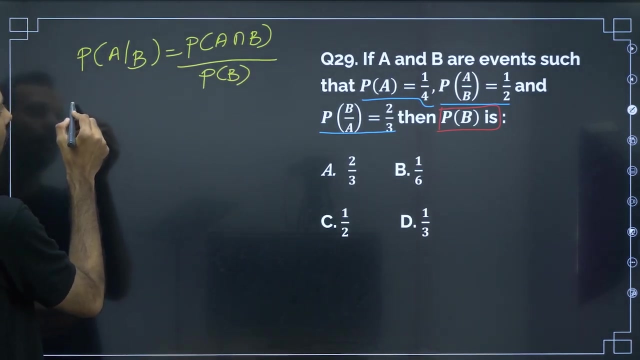 what is the question then? P of B is what? So how to solve? P of A and then P of B is now: probability of A given B is equal to probability of A. intersection B by probability of B. Ok, A given B is how much? no, before going to that, let me from here I can write: P of B is equal. 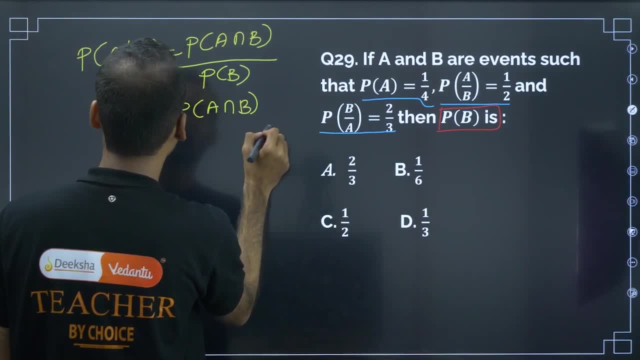 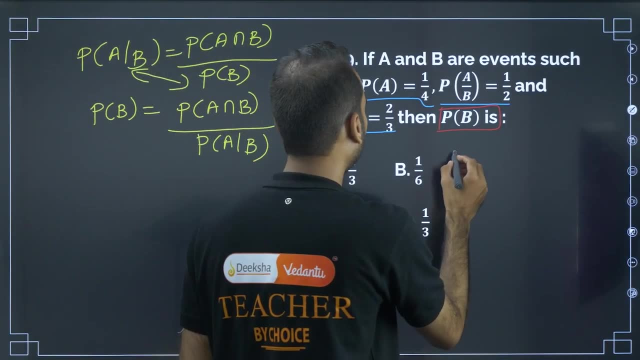 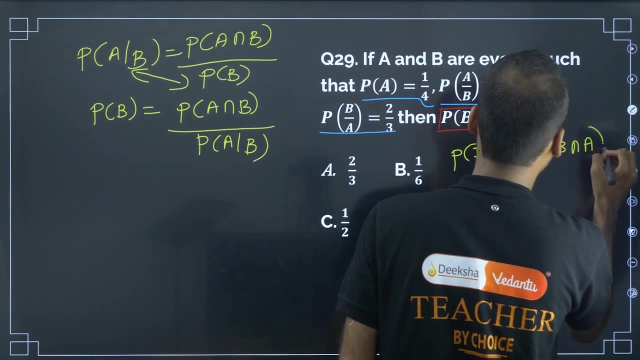 to P of A- intersection B by P of A given B. I am just interchanging their places. Next, P of B given A is equal to P of B, intersection A by P of A. P of B- intersection A by P of A intersection B. 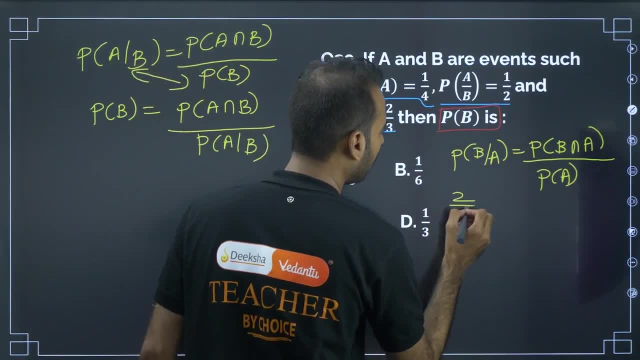 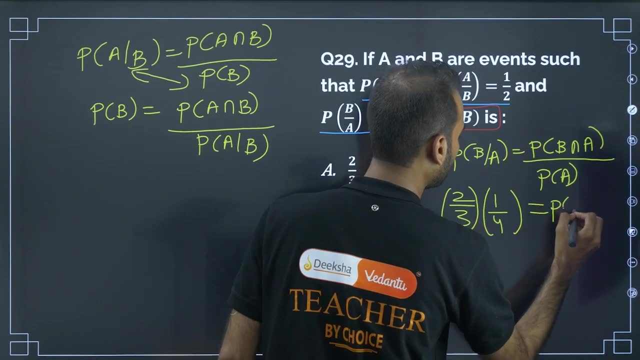 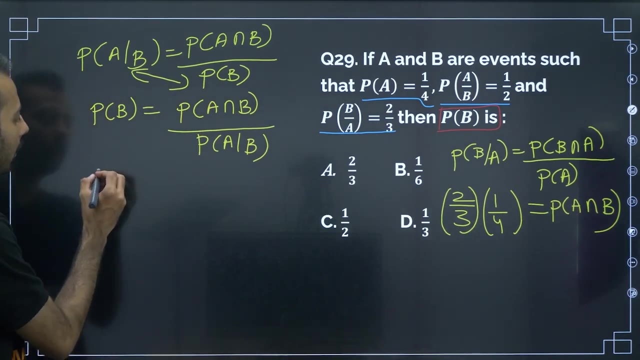 Ok, b given a is 2 by 3, p of a is 1 by 4,, 1 by 4, p of b intersection a is p of a intersection b, Just substitute that. so here we will get: p of b is equal to p of a intersection b. 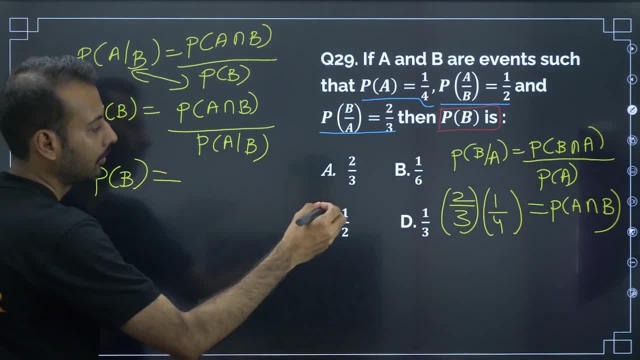 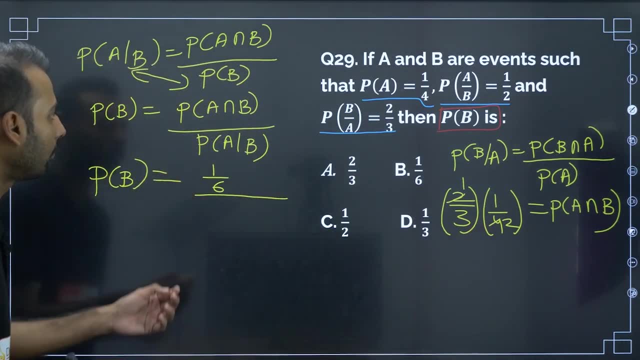 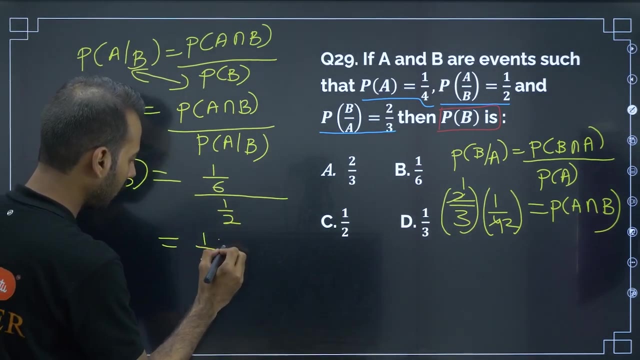 How much is p of a intersection b? It is already given. if I cancel this 1 by 2, 1 by 6, I will get 1 by 6.. Probability of a given b is so 1 by 6 divided by 2 by 1, probability. 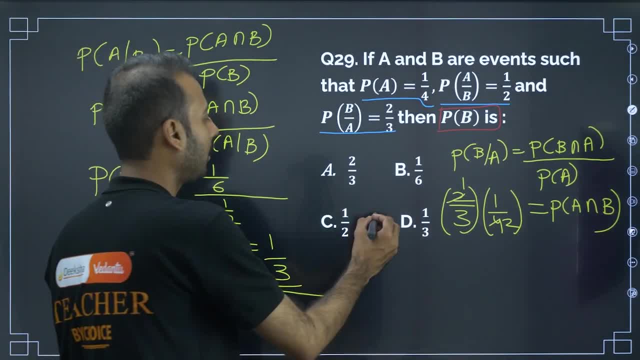 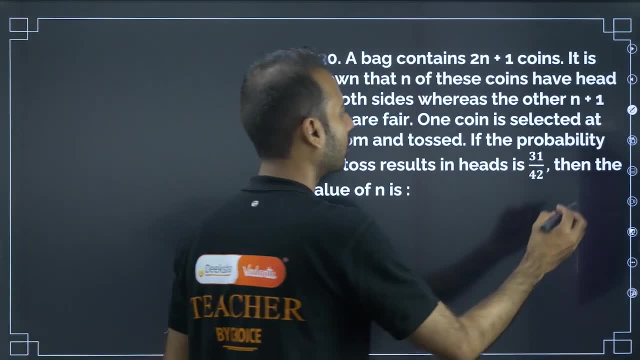 of b is 1 by 3.. So answer is d. d is the answer. Moving on to next question, a bag contains 2 n plus 1 coins. So some information they have given: a bag contains 2 n plus 1. 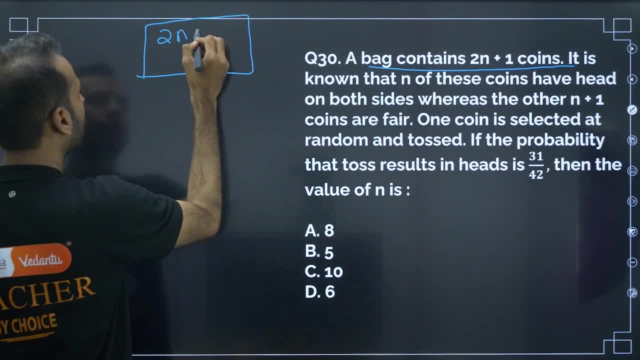 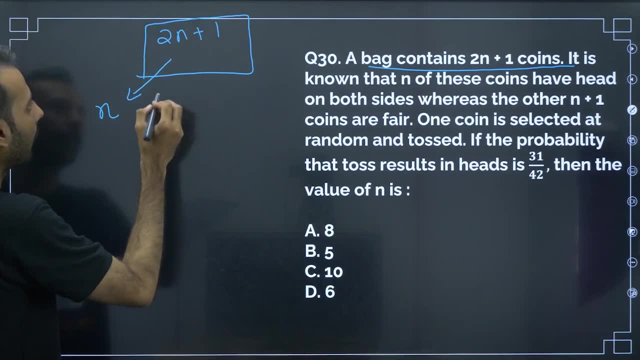 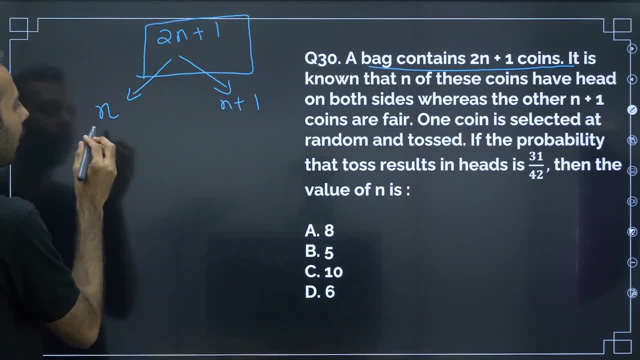 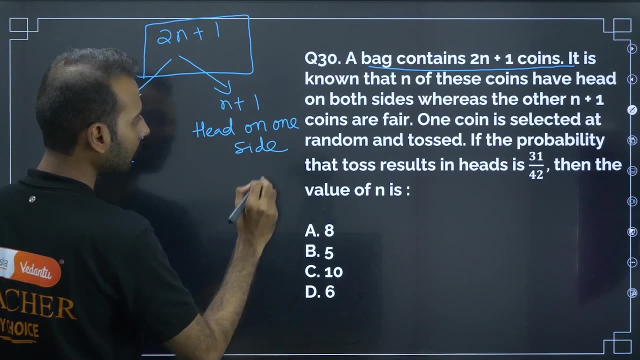 taking n here n plus 1 are left. n have head, head on both sides, head on both sides, head on both sides here, head on head on one side, on one side, And to see if we can bring this n there. n is there in the taken amen. n is there in. 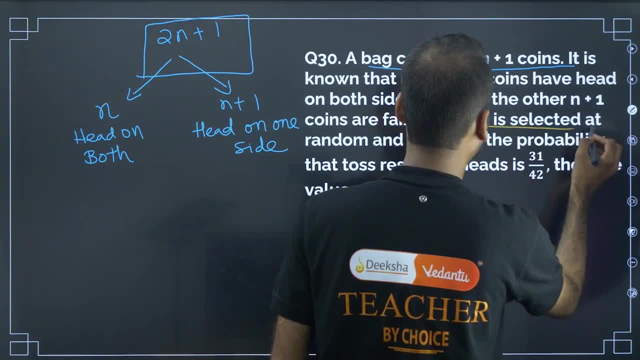 the taken amen n is desired, And when we divide this equal to 2 by 6, it is equal to 3, only 2 is given. n plus 1. here n is said because 1. often we have't selected n in either. 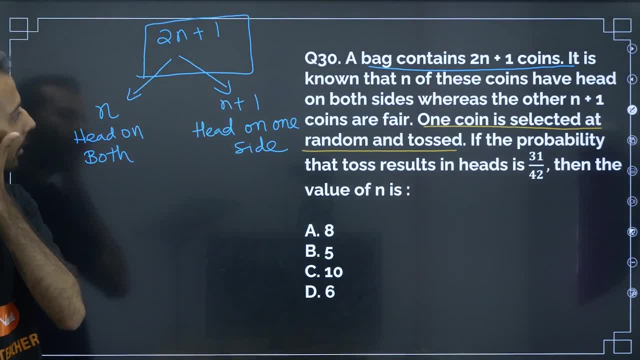 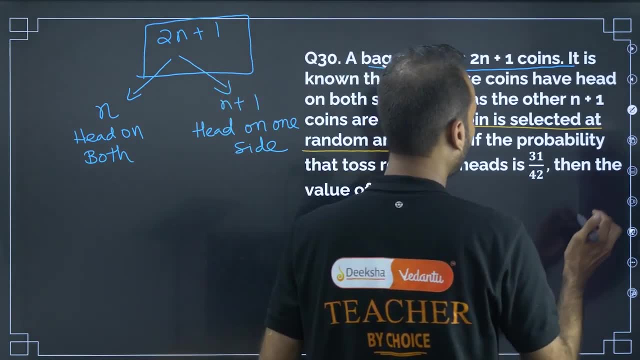 case. So in different cases, if we were going to線 the head, that means n is set at a distance from head to head. If the probability that head is not selected, we have 1 by 2 to be 1.. So this is the probability of heading in to action. Now, what we are doing? We are doing? we are doing one coin selected at random and tossed. they took 1 coin and they tossed a bag contains. this means one, one coin is selected at random and if the probability that tossed results, 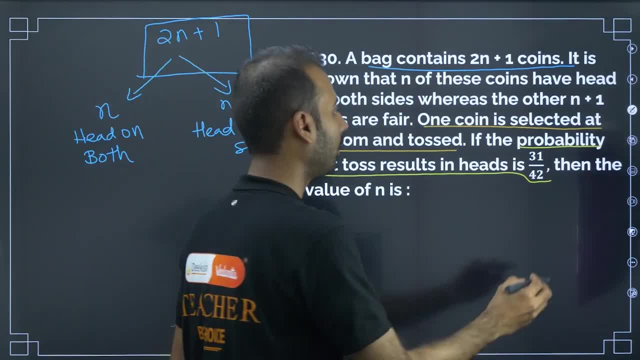 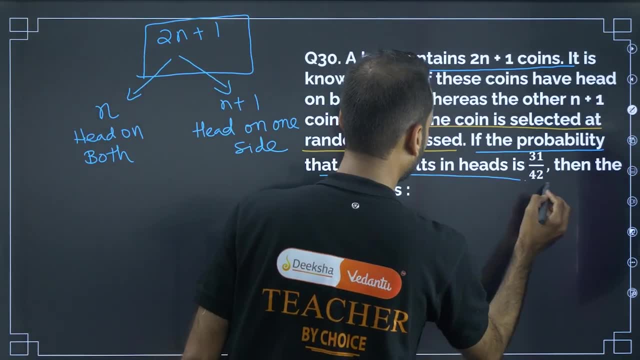 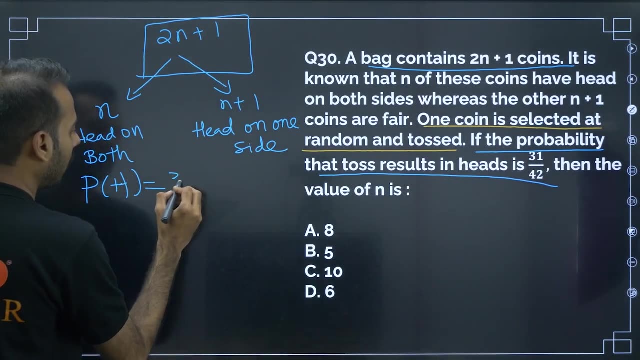 in heading is tossed. if the probability that tossed result in heading is ah, toss one coin is selected in head, is this much, then the value of n is and the probability cost result in head is: probability of head is: probability of head is 31 by 42, then the value of n is value. 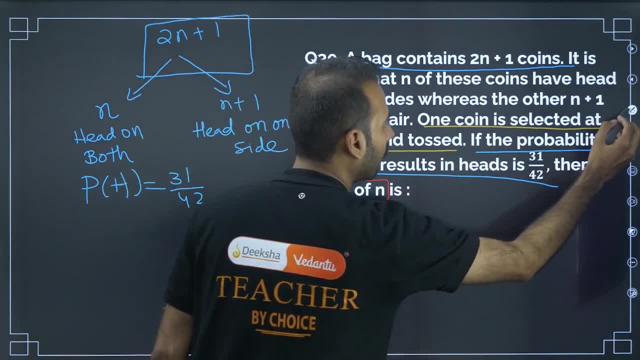 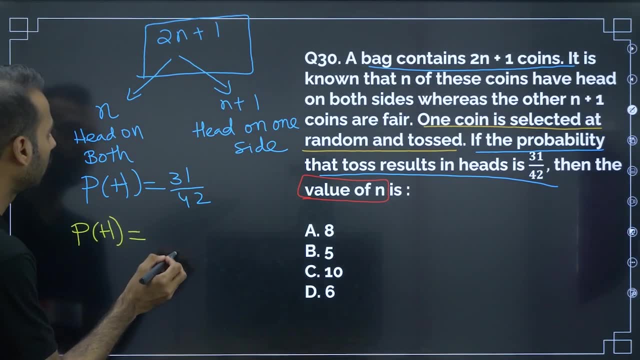 of n is. they are asking to find value of n. So how to approach this problem? Probability of head is equal to now, from here, if I name this as 1, if I name this as 2.. So probability of head is equal to n head on both sides, on both sides, n head on both sides. 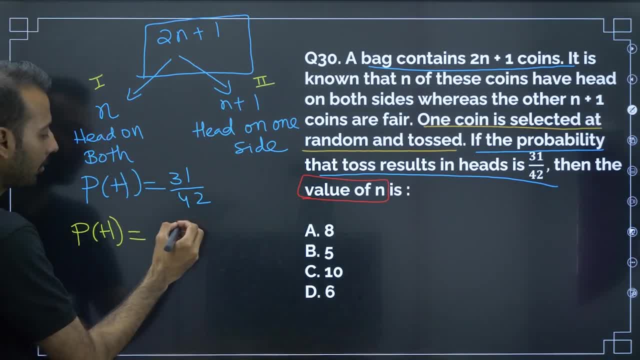 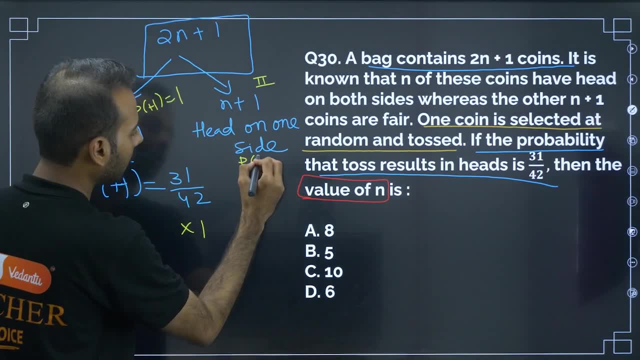 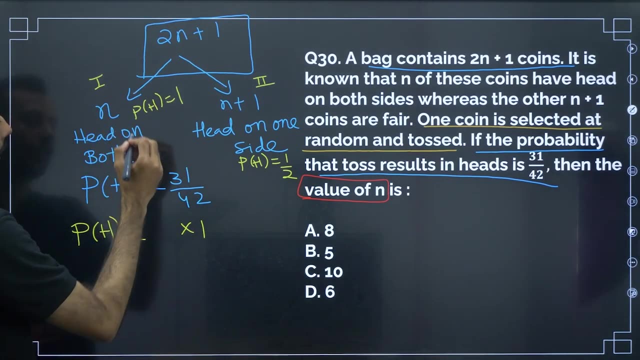 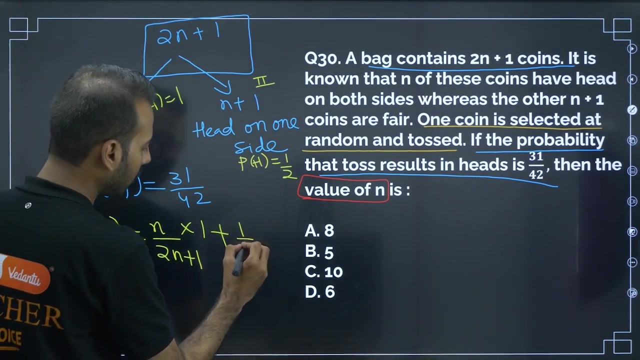 For this head on both sides means probability of head. here is probability. head here is 1. probability of head here is 1 by 2, probability of head here is 1.. Also, how many n? favorable n by 2, n plus 1. plus here head is 1 by 2, how many coins are there? How many coins are?